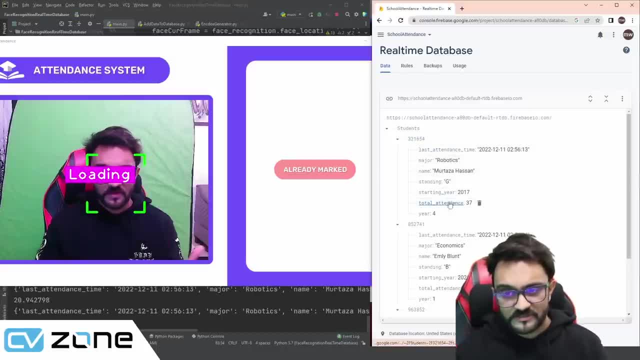 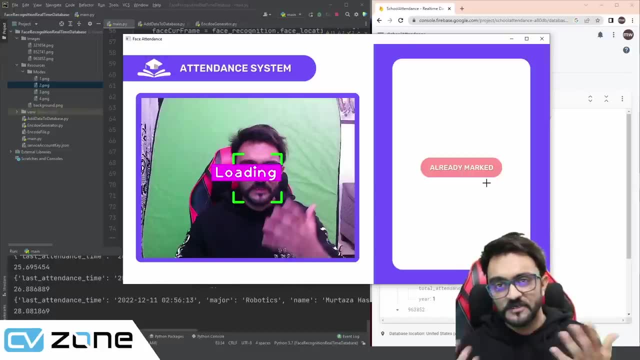 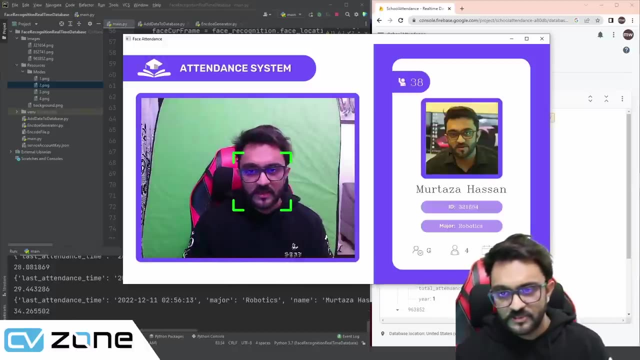 it has the attendance, time, major name standing, all of that information and, as you can see, it shows here that i have been already marked and i can mark only after 30 seconds. so if i hide my face and 30 seconds are gone, i can mark it again. it's loading, it shows my name, it shows the total. 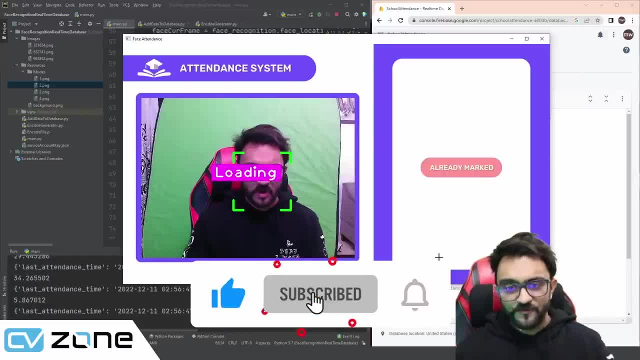 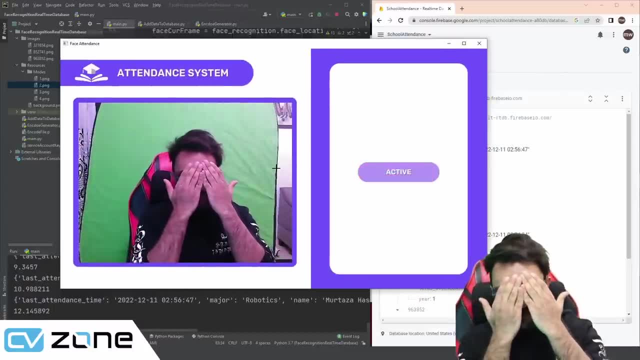 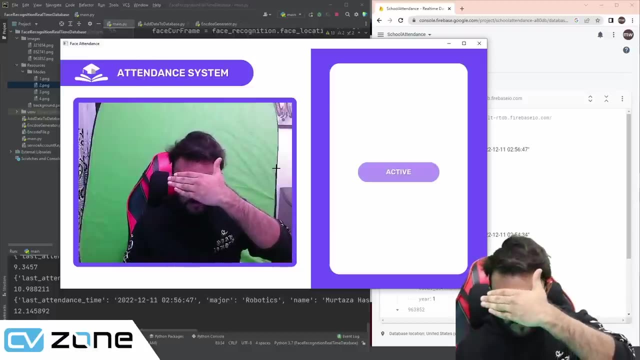 number of attendance and it says it has been marked. now if i come again it will say already marked, so it will not mark this attendance. so that's the basic idea. i will hide my face so that it can show you the status. so we already have other students as well. for example, we have emily. 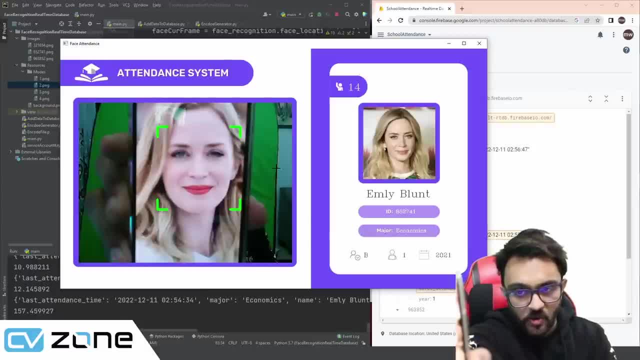 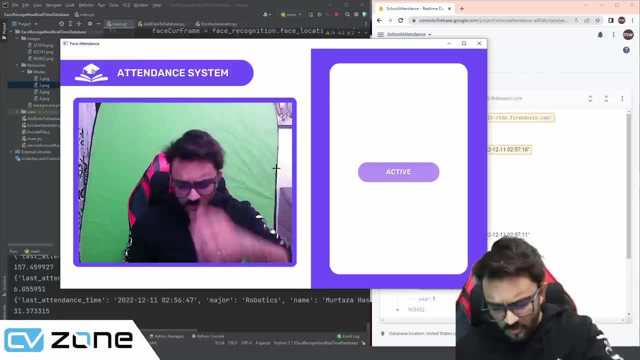 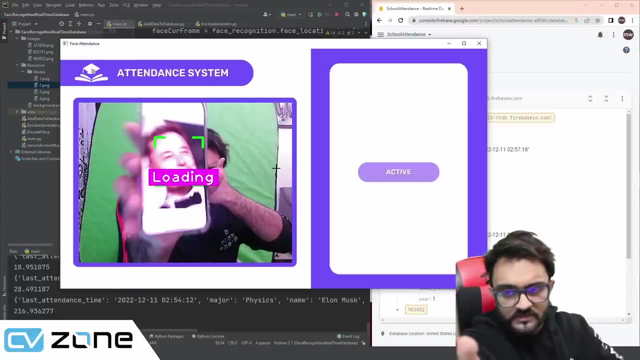 blunt. so if i bring in her image it says loading and it shows my name and i can mark it again. emily blunt was detected and her- uh, what do you call attendance is marked. we also have elon musk, so let me just google elon. so here we have the image of elon musk and there you go, it says loading. 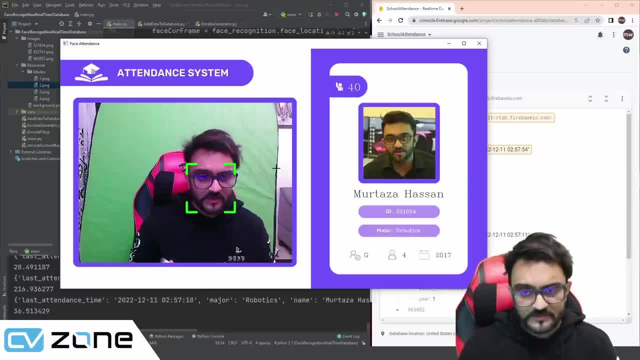 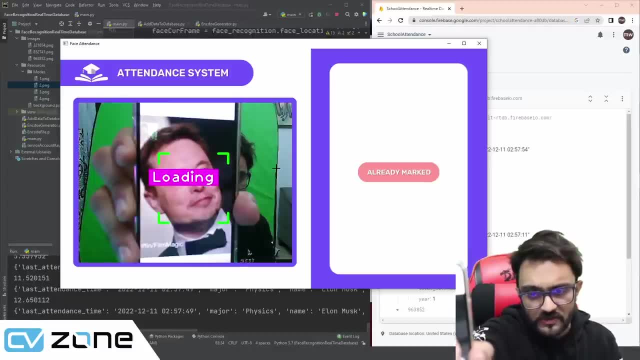 and elon musk is marked and if i bring it again it is not going to detect. it will say already marked. so if i bring it again, you can see it says already marked. so after an x amount of time you can mark it again. and you can see it says already marked. after an x amount of time you can mark it again. 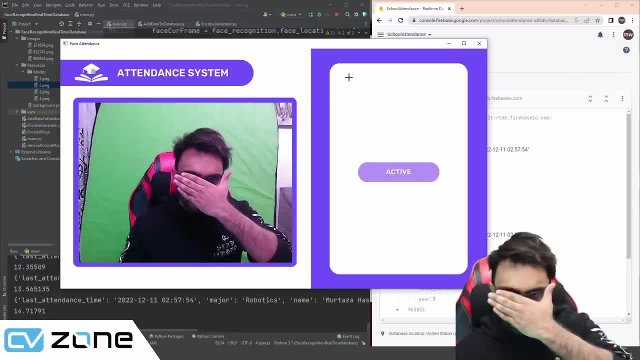 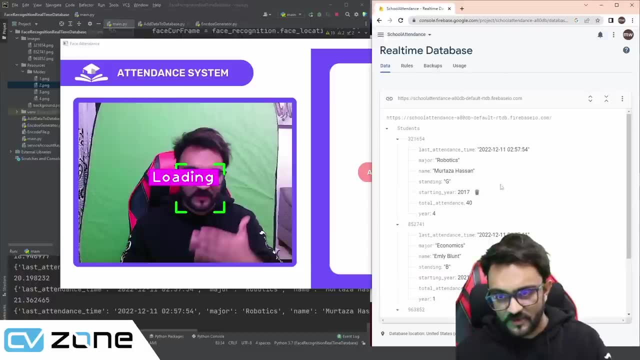 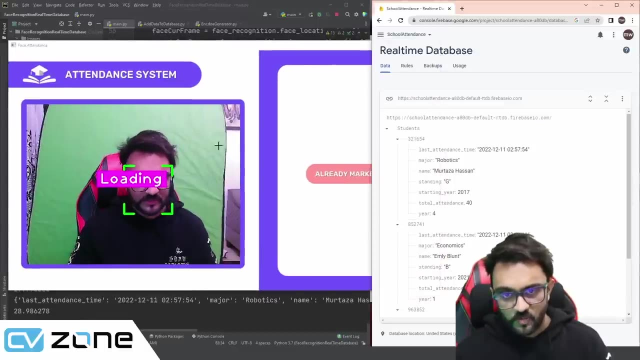 otherwise the system will not detect. so here right now you can see my face was detected. if I remove it it will say already marked because not enough time has been passed by. it's it's checking the time from here and if you see here you will see it updates in real time. so when over here it will update there you. 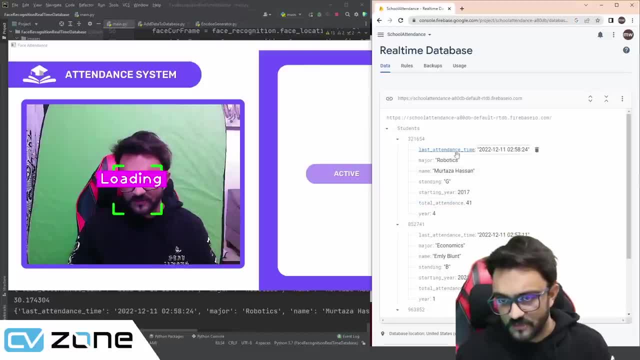 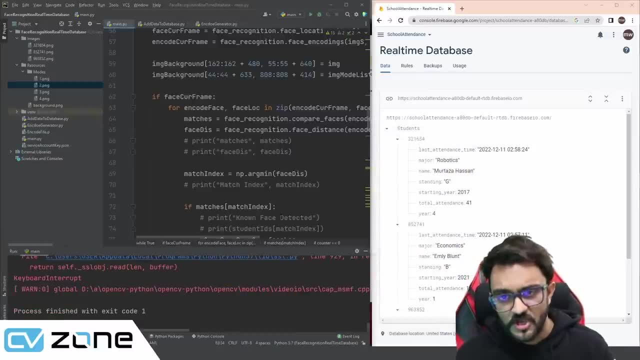 go so you can see the orange. the total number of attendance was updated and the attendance last time was updated as well, so this is an amazing project that you can use to implement it in real time, and if you want to learn how to create this on a web app, then you can check out our Kickstarter page, which is live right now. 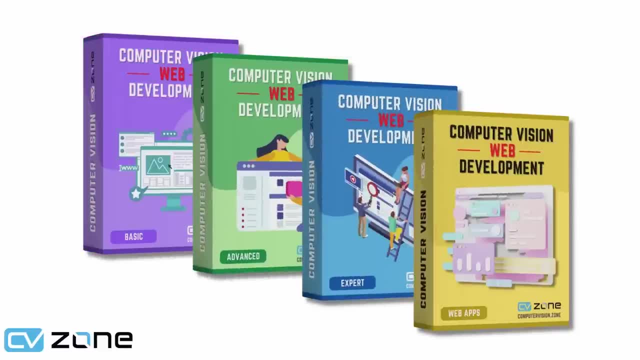 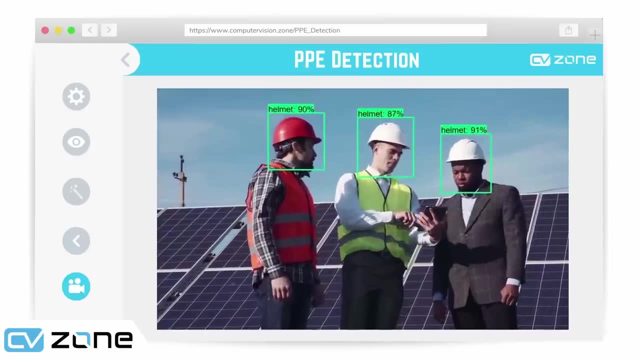 with the world's first web development course for computer vision, which will teach you all the basics of computer vision, along with all the basics of web development. so we will integrate both of them and we will create more than 30 web apps to create these amazing projects. so here you can see, it is a. 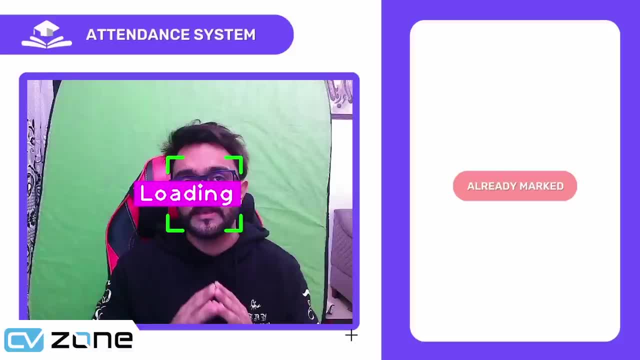 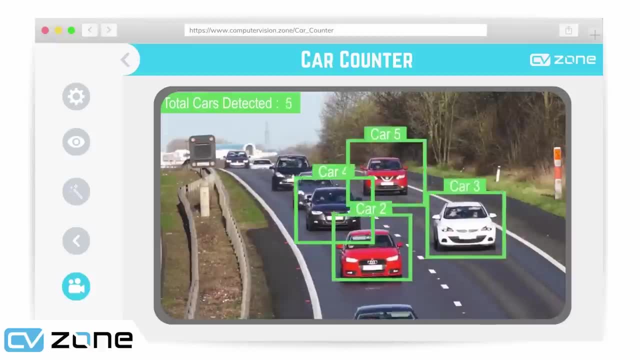 little bit laggy because we are not using asynchronous functions. we're going to need a lot of time, so I'll show how to do that in a minute. but but on the web development part, we are going to use asynchronous functions, so it will download the data and it will show you the real-time webcam feed at the same time, so it will not be. 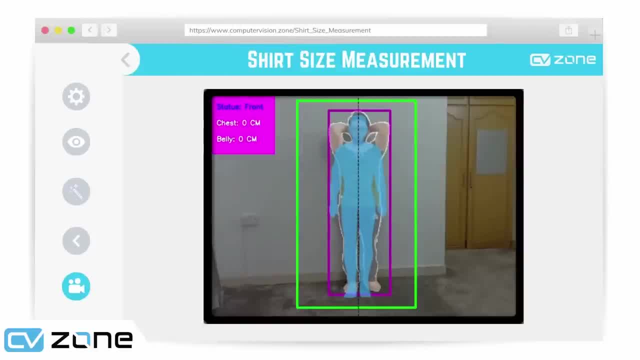 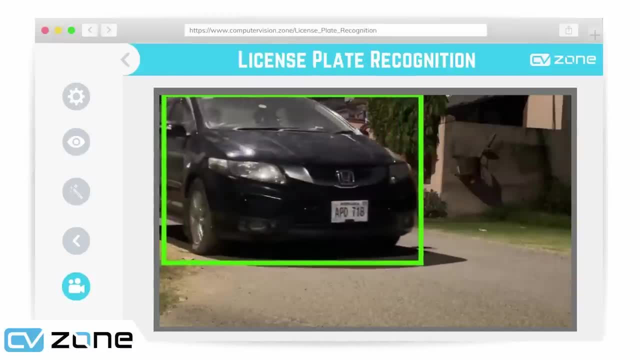 in a series function. it will be parallel, it will running side by side. so this project is also part of the web development course. so if you wanted to implement it on web, do check out our kickstarter page. otherwise, you can do it in python as well and create your interface and add these graphics. 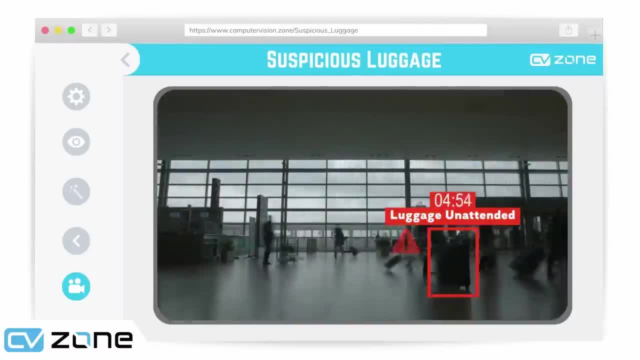 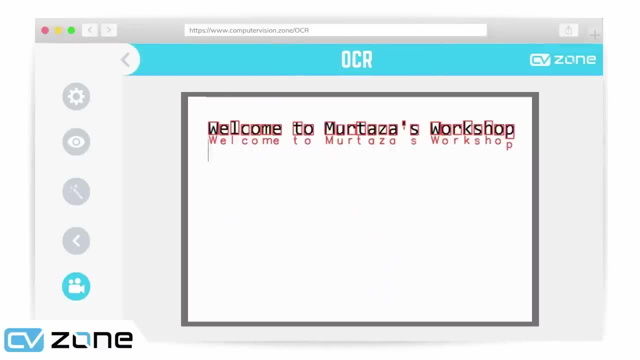 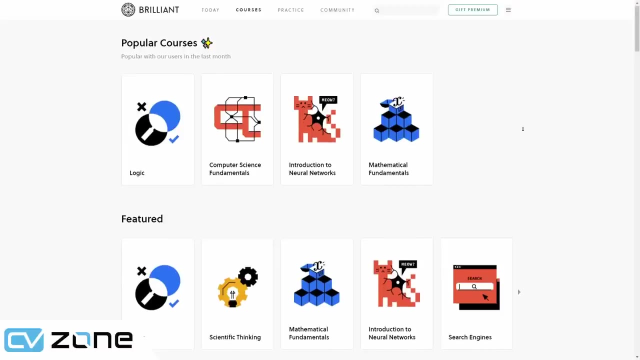 and add this real time. and all of this is for free, of course, but our premium course for web development is paid and it is 30 off right now on kickstarter, so do check it out. so let's go ahead and create this project. this video is sponsored by brilliantorg. the most significant way to learn. 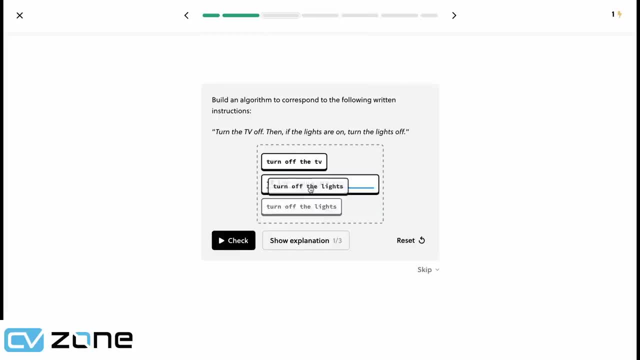 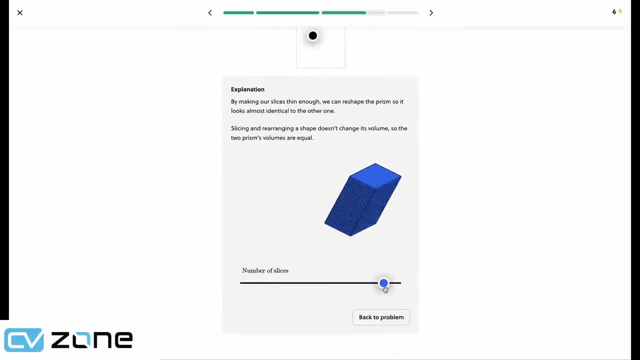 anything is by doing it for yourself. brilliance. engaging hands-on lessons will let you learn six times more efficiently through interactive learning that you can do by viewing lecture videos. they're interactive and they're free to use, so if you want to learn more about how to use them, 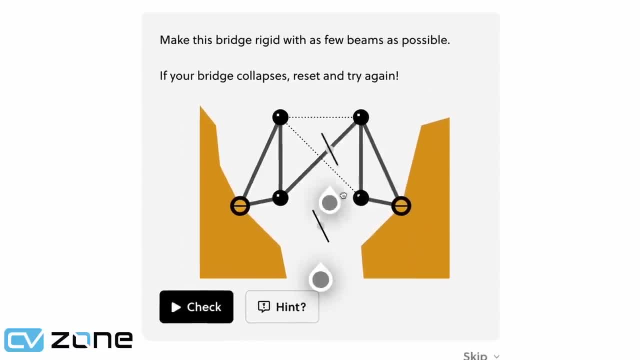 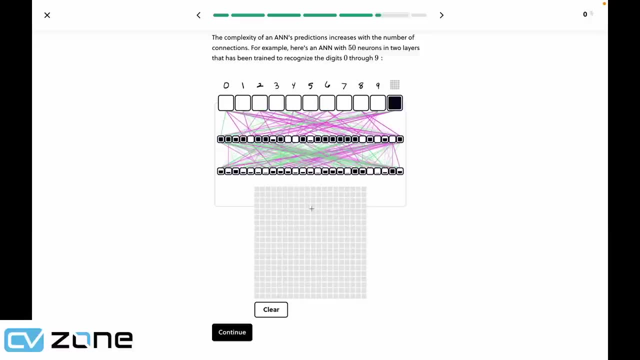 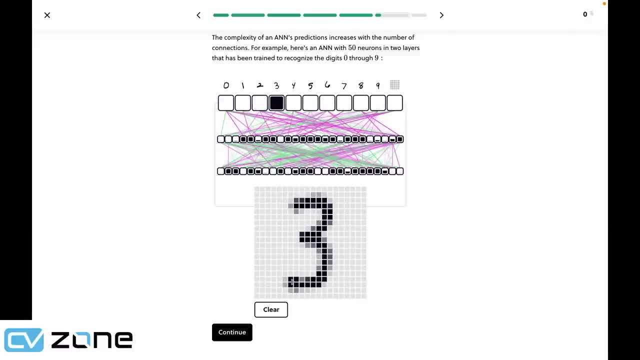 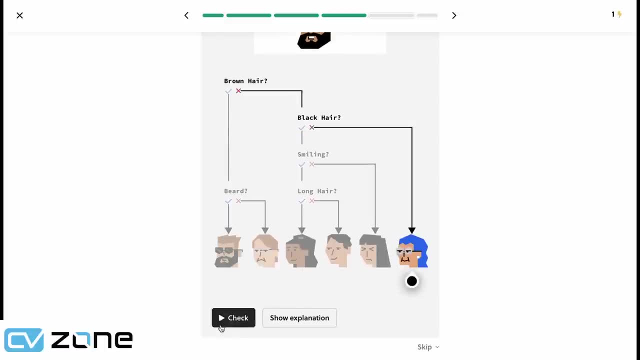 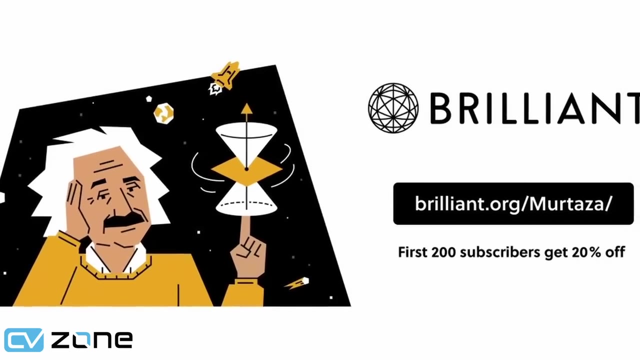 rigorous mathematics. explore the internal workings of artificial neural networks through practical testing. design innovative algorithms that a computer can process quickly. enroll now and learn anything of your interest. check out the link brilliantorg murtaza to get started for free with brilliance interactive lessons. the first 200 listeners will also get 20 off their annual 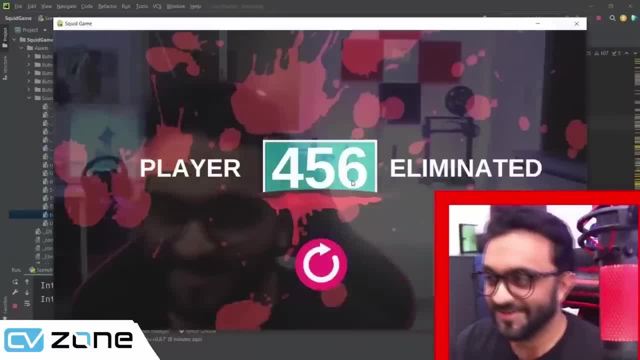 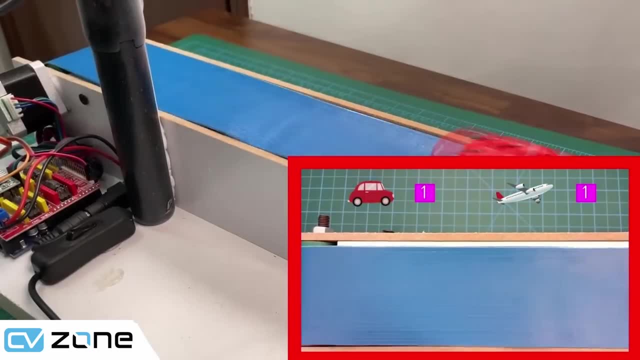 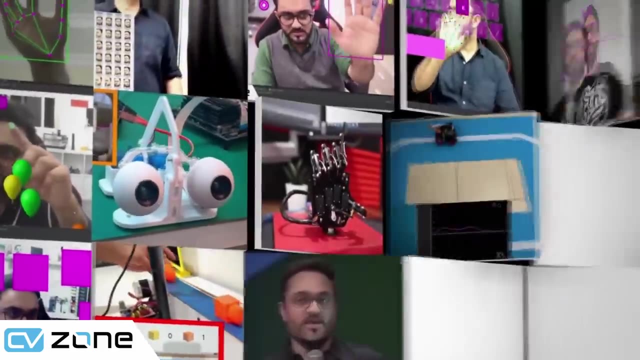 membership. if you would like to level up your computer vision skills, do check out our premium courses that are available on our cv's own platform. links are in the description. so, without further ado, let's get started. so today we are going to create a course that will help you to. 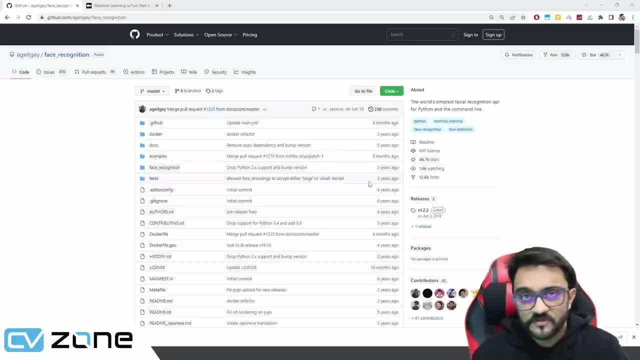 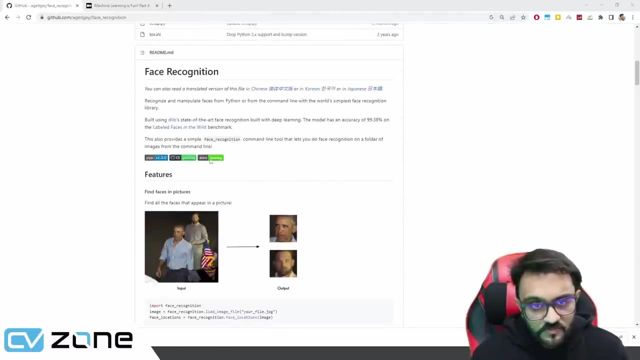 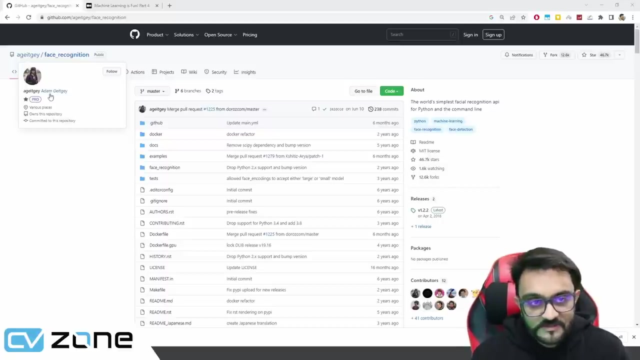 create this face attendance system that can be used for schools, for employees, for a company and so on, and what we are going to do is we are going to use this face recognition library. now you can see, this is the github page and, uh, thanks to mr. what's his name? a get key adam. okay, his name is. 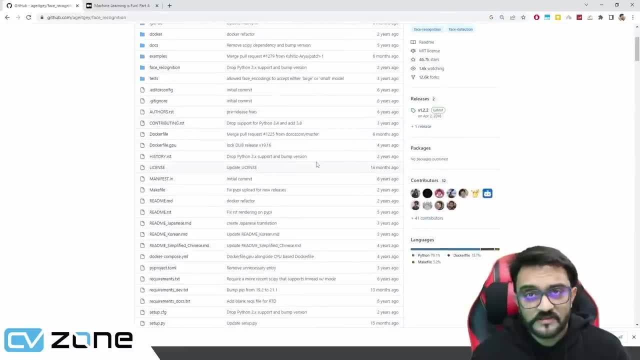 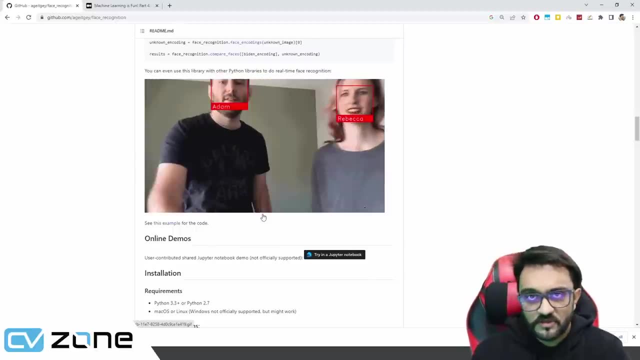 adam. so thanks to adam and all the contributors for creating this library, and we have done a previous video on this. but today what we are going to do is we are going to take this technology, we are going to take this library and we are going to integrate it with a real-time. 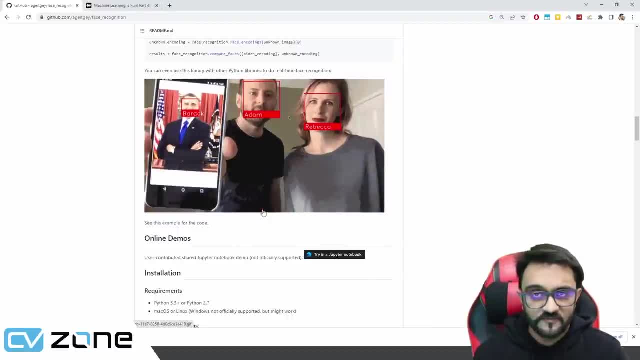 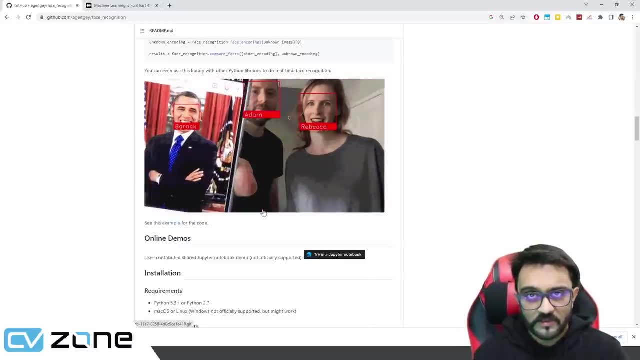 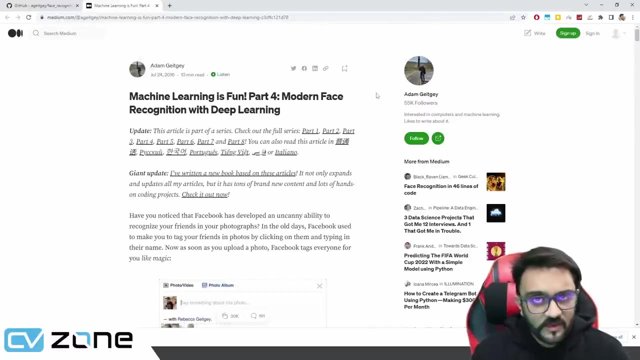 database so that we can upload all the data on a server and then, when we are running the software, we can download the data, we can view it and we can upload more data to it, we can update it. and there's also this medium article that you can read again, by adam: 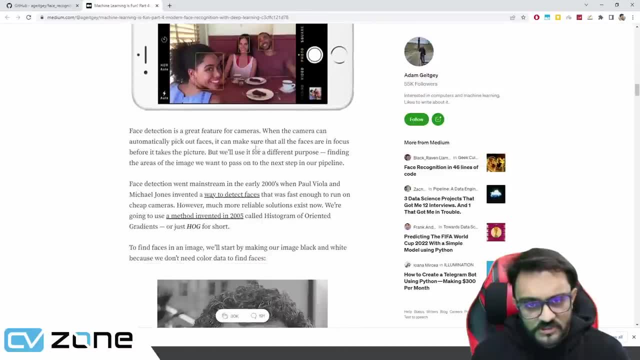 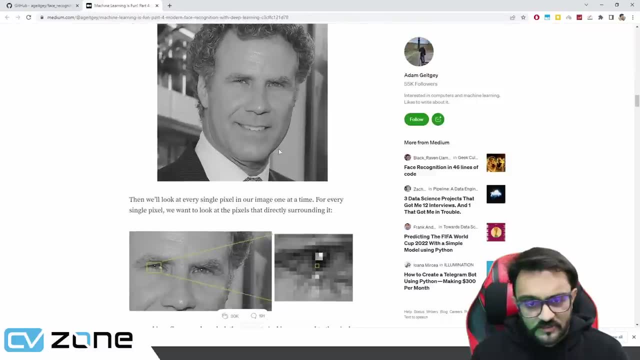 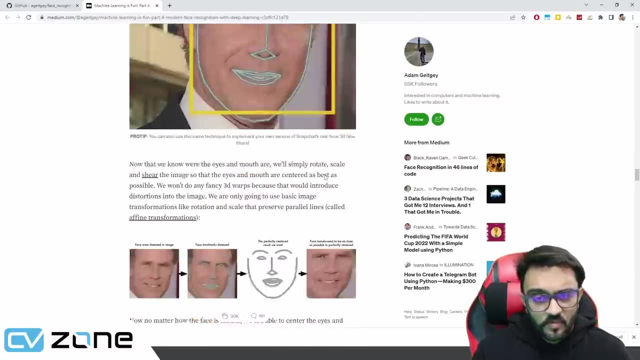 it explains how this face recognition library works. it is pretty good to see how it works. it uses face recognition- sorry, face detection- then it uses these features. it extracts and creates these encodings which you can see at the very end over here. so it will create these 128. 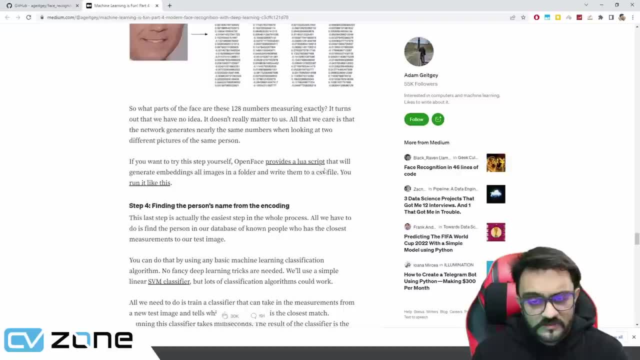 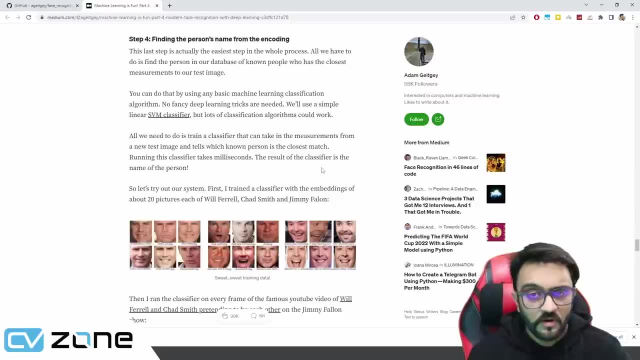 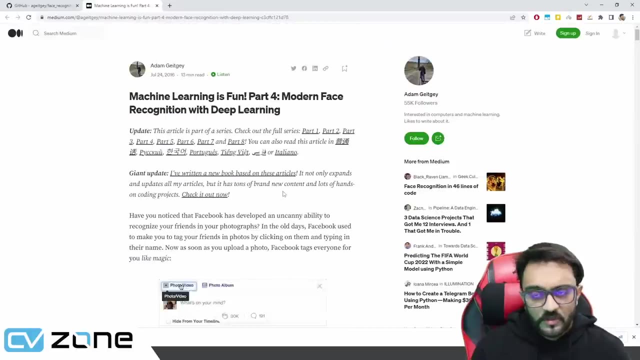 measurements that we will call as the encodings, and based on these encodings we can use a machine learning model to actually compare which of the two faces match with each other. so they are using svm classifier to you to do that. so you don't really have to go through all of this and read it out, but it will be better if you do, if you. 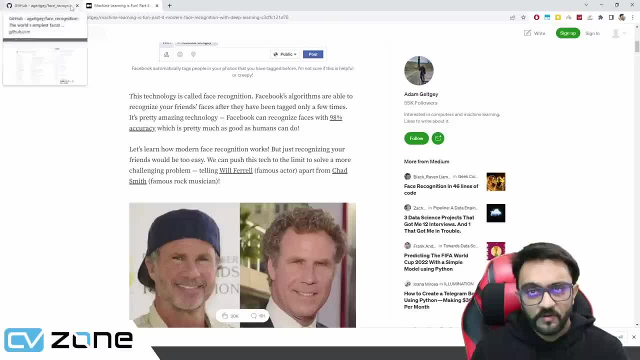 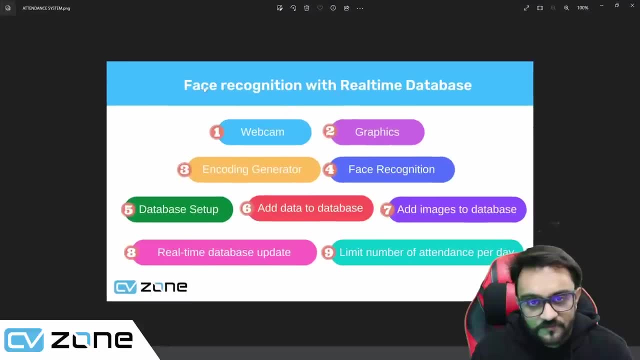 understand the underlining principle of the library, so it will be useful for you. so what exactly are we going to do? we are going to follow these steps. so face recognition with real-time database. first of all, we look at the webcam, we will import our parameters and then 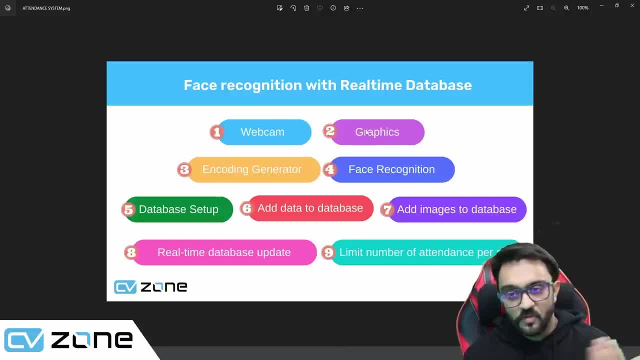 we will run our webcam, then we will add the graphics, so we have an interface in which it will show whether it's active, whether we are detecting the face loading and all this stuff, and then we will create an encoding generator. so this has to be done once. so, for example, if 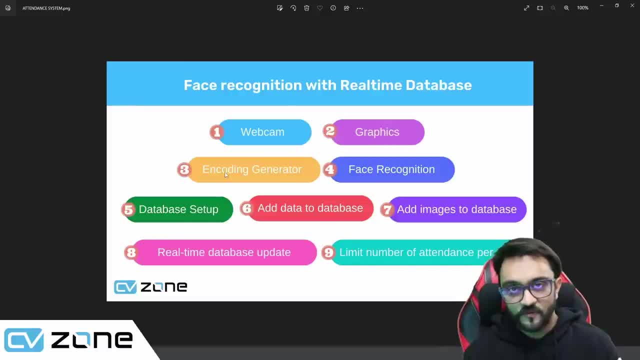 you have three faces, three students. you have to do it for all three of them and then you have three Stunden. you have to create the encodings with three student's methods in this descent guide. so you run it once it will generate the encoding for all three of them and whenever you have a new student you will have to create the encodings. 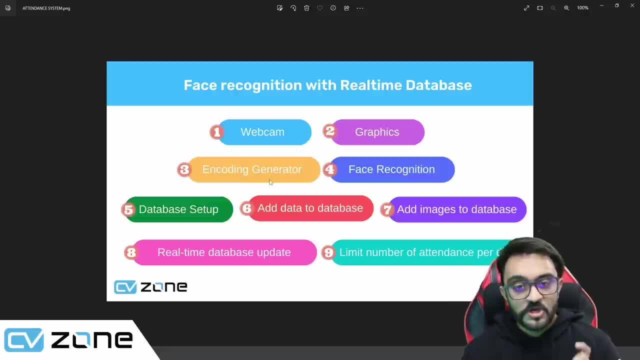 again. so you'll have to update them, so you will run this script, so this will be a separate script. then we have to do this face recognition. so the encoding generator is going to generate a file in which we will have all the encodings and it will be able to detect the faces. 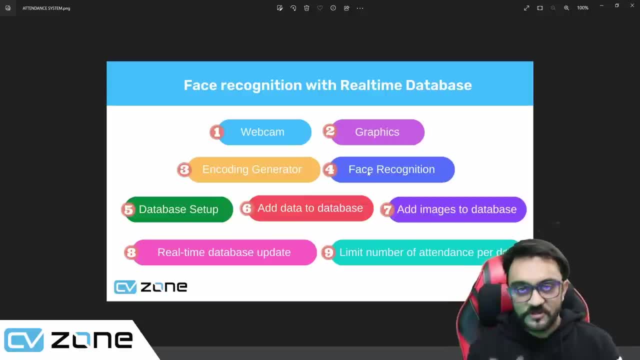 So you can put both of them in one script, but that is not very useful, because every time we have to run you should not be generating the encodings, because they are pretty much the same each time. Then the next step is basically the database setup. 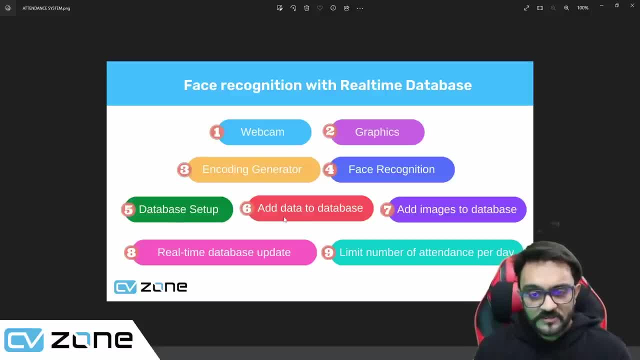 So we are going to set up our database so that we can send in and we can receive the values. Then we have to add data to the database. Again, we will create another script for this, in which it will become easier to add the data. 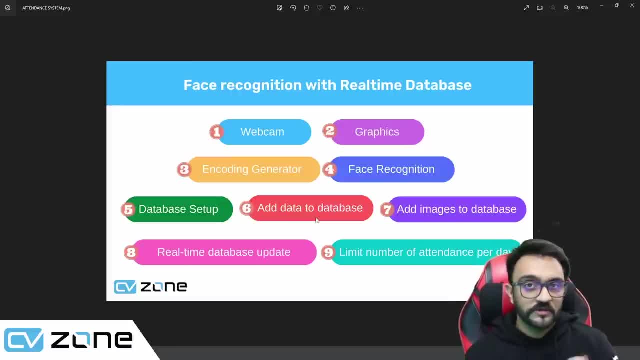 Otherwise you can actually go to the website, you can go to the database itself and you can manually add the entries. But that will take some time. so instead of doing that, we can just create a script and we can just copy paste. 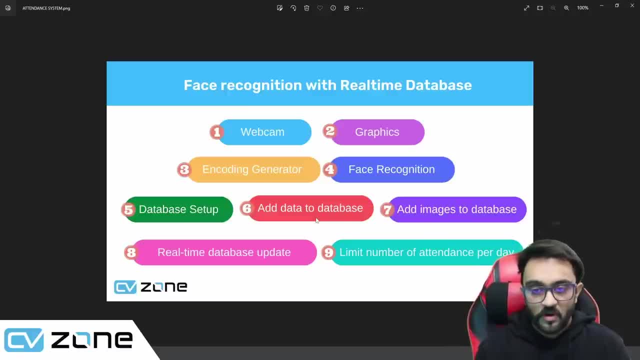 for each student and change the data and we can upload it all together at once. And then we also have to add the images, So images are stored in a different place than the data itself. So the database is stored in our real-time database and the images are stored in a storage bucket. 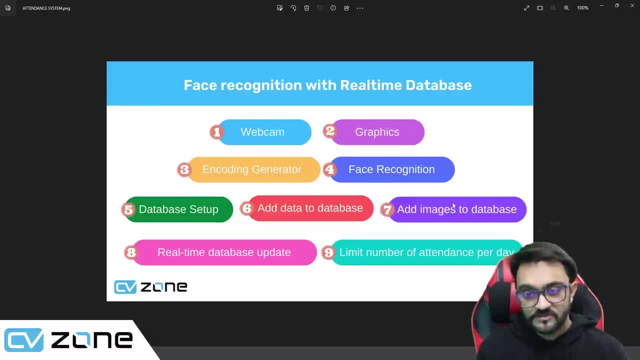 So these two are separate, so we will handle them separately. But at the end of the day the results will be shown simultaneously. Then we have to update the database. whenever there is an attendance, whenever there is a face detected, we have to update the database. so we will do that. 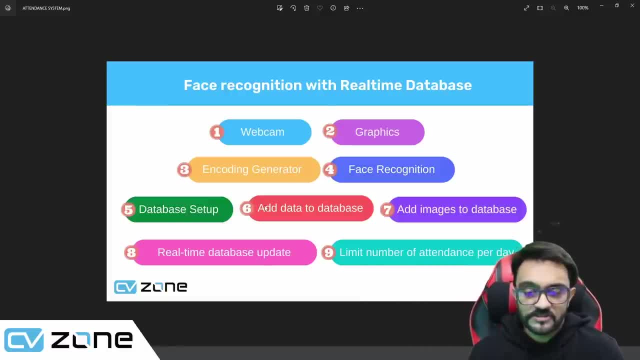 And then, once we have detected the attendance, we will not take another attendance until an X amount of time. So normally it will be one day, So 24 hours, or the next day you can take attendance. That's the idea, But for simplicity we are going to give it a limited time. 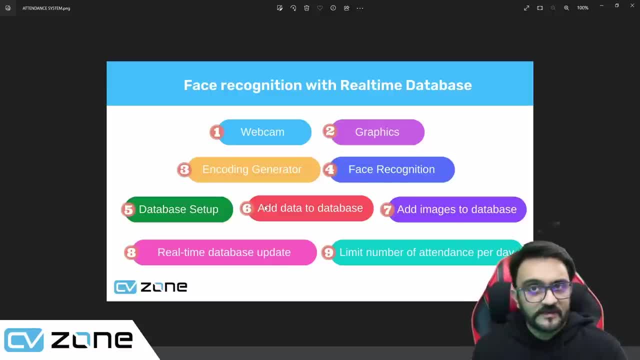 for example, 30 seconds. So after 30 seconds it can take the attendance again, because we just want to see the effect. I don't want to sit here 24 hours, just to show you that it works right. So that's the idea. 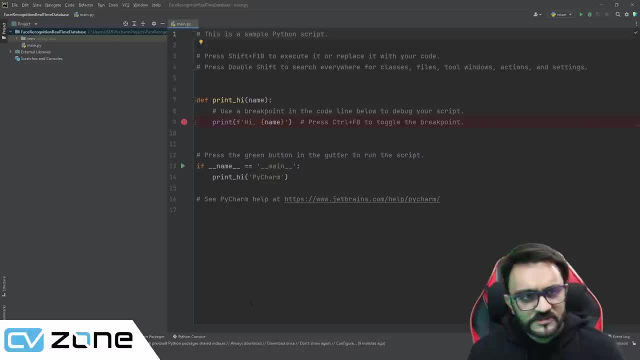 So let's go ahead and get started. So the first thing we have to do, we are going to import all the images, the resources, everything the files, and then we will start with the installation. The installation is a little bit tricky. 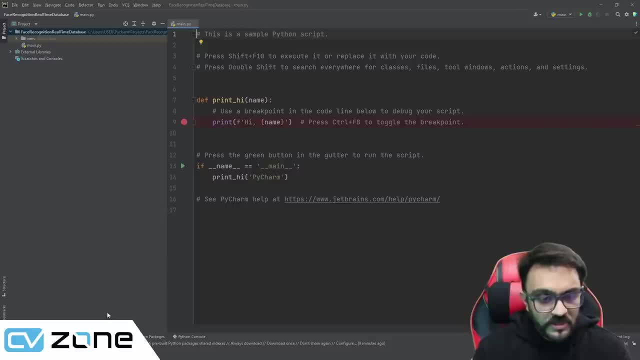 but it's not that difficult, but I'll show you how it's done. So let's bring in the resources first. So what exactly do we need? So, first of all, we are going to create here a new directory and we will call it resources. 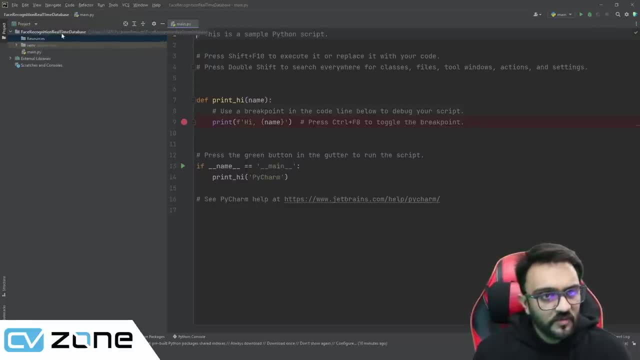 Resources. Now, these are the sources. Then we can also create another one by the name images, or we can do it inside this. So let's create it outside, So we will keep it separate. So images, And within these images we are going. 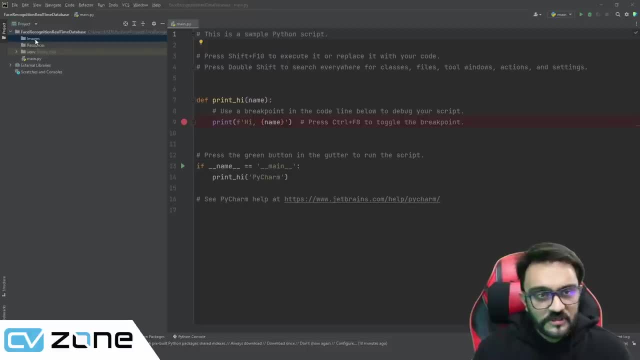 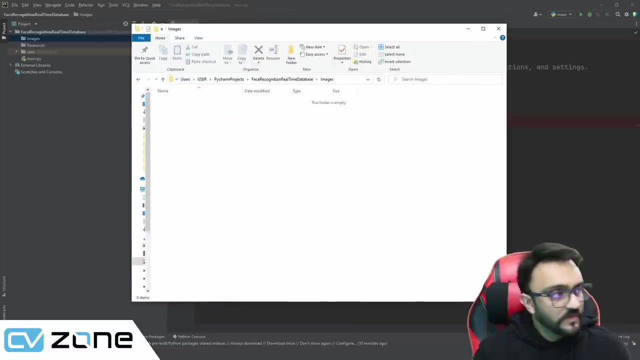 to add our three faces, or three students that we are going to detect. So let me open this up. So open in Explorer. I will just drag and drop the images so we can see them as well. There you go. So these are the three images. 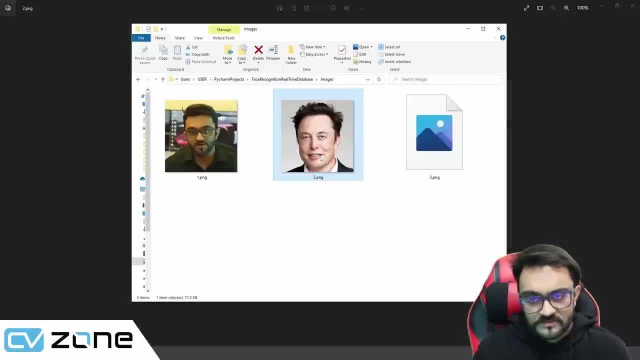 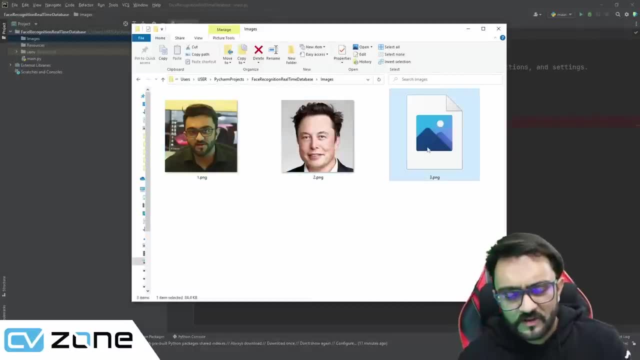 Why is this not showing? So this is Emily Blunt, This is Elon Musk And this is yours truly. So what can we do is, instead of writing one, two, three, we can give them IDs because, based on the ID number, 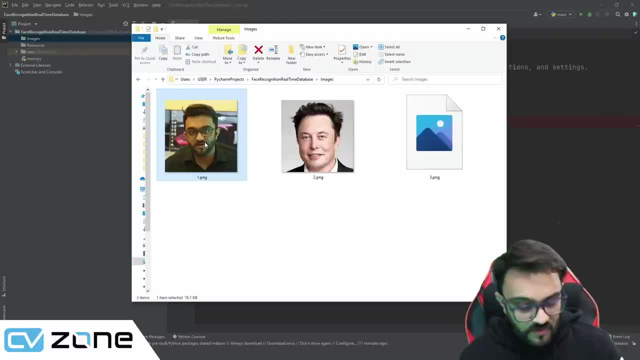 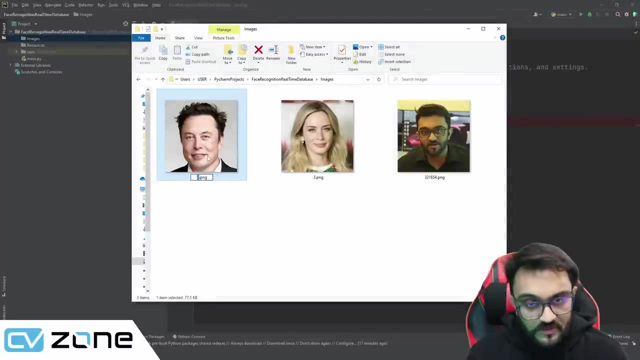 the student should be detected, not based on their name, because name can be detected, It can be similar, but the ID number is unique. So here we are going to give unique IDs. So 321654, that's my ID, And then we will give it to Elon. 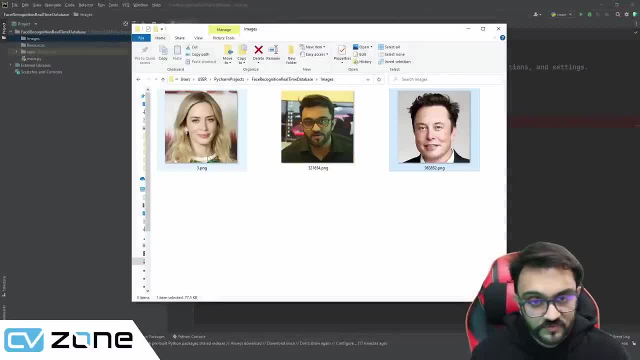 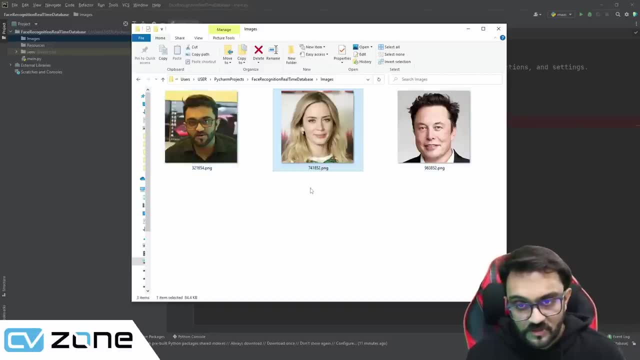 Let's give him the ID 963852.. And then, for Emily, we are going to give 741852.. So these are the- or let's change that- 852741.. Yeah, So these are the three IDs that we are going to use. 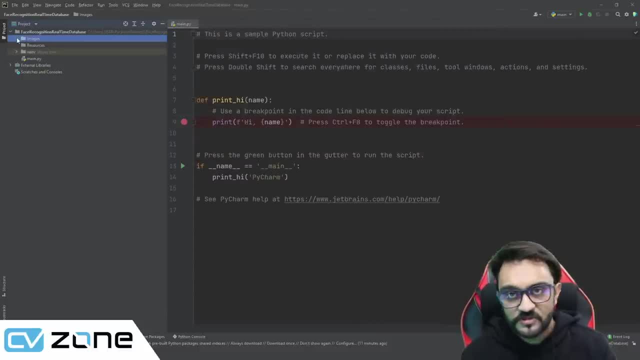 Now we have the images in the images folder. So these are the three students. If you wanted more, you can add more as many as you want. Then the resources in the resources folder, we are going to add. we are going. 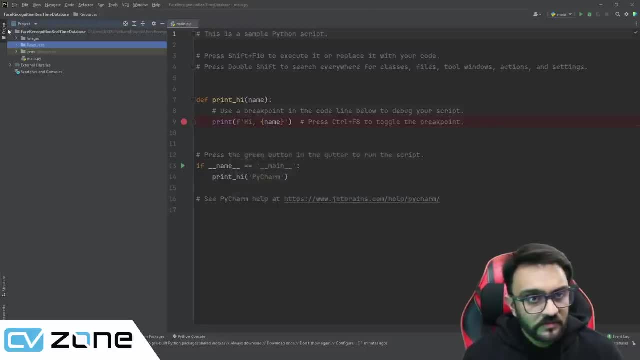 to add background and the modes. So let me open that up and show you what do I mean. Let's open that up. Let's open that up. Let's open that up, Let's open the Explorer. So here in the resources, we have modes. 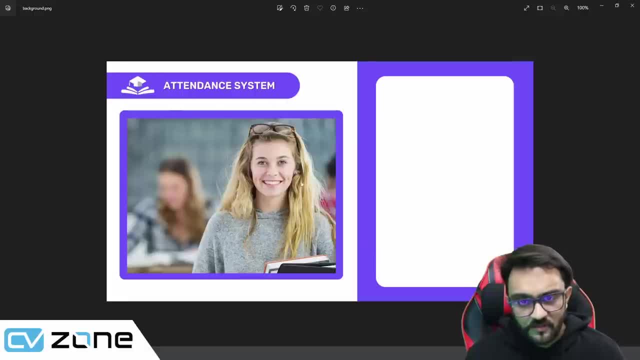 Actually, let me show you the background first. So this here is our background. So this is the attendance system graphics. Here is the webcam that will be displayed And on the right-hand side you will have the information of the student. So you have the image and all that stuff. 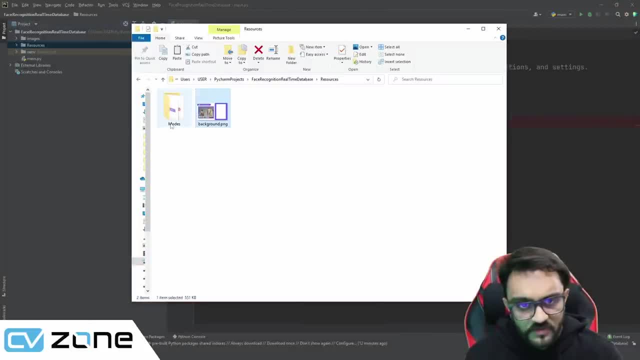 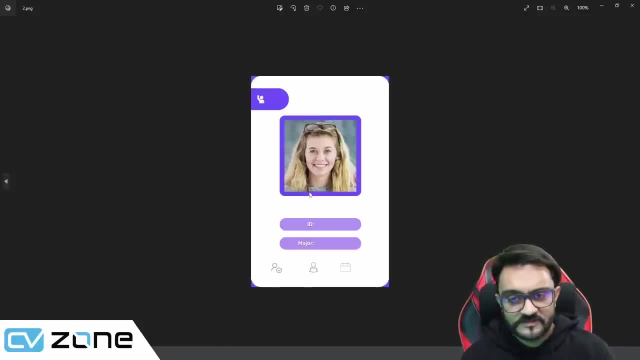 And where does that come from? That comes from the mode. So here, if you click on mode, so these are the modes that we will see. So the first one will be active. The second one will be of the actual student. It will have the image. 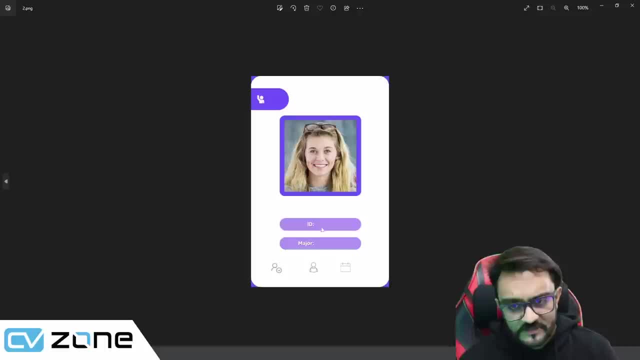 This part. here is the total number of attendance. This here is the ID number. This here is the major. Then we have these three. This is which year did they join and how many years have they been in the university. And this one I actually forgot. 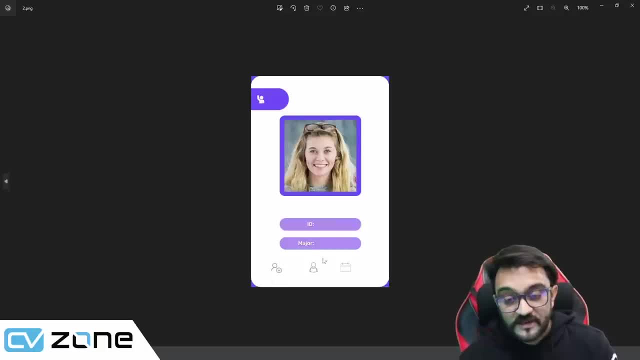 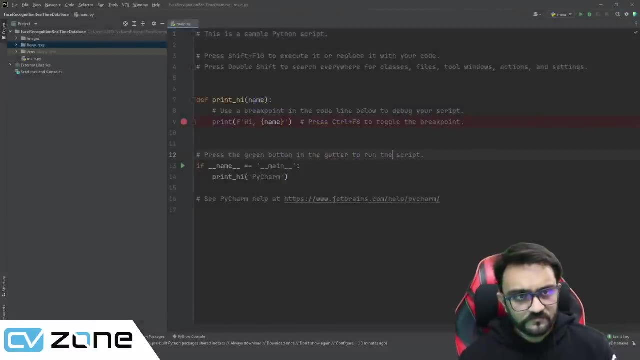 What was this? The standing of the student? Is it good standing, probation period or bad, or whatever you want to write here? So it's just for showing that you can add lots of different parameters and you can actually display this information. 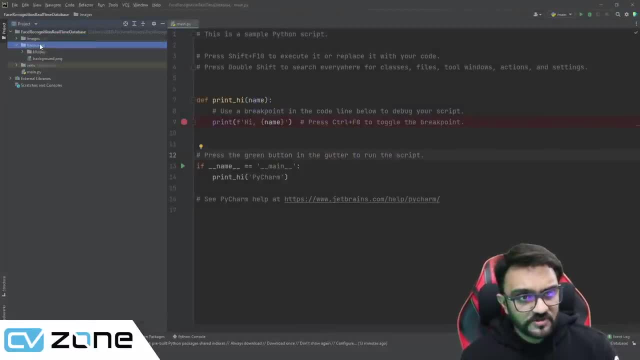 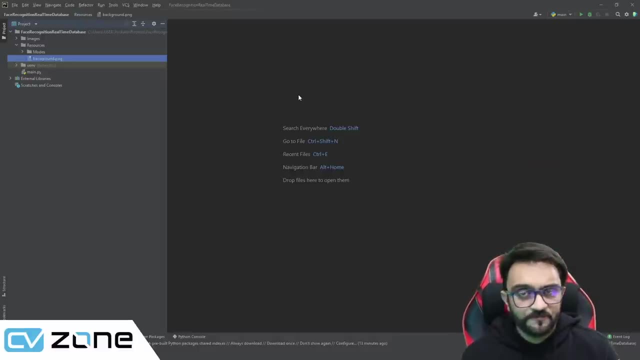 OK, so now that we have our images and we have the resources folder with the modes and the background, we can move on to installations. Now for installation, what we need is we need a C compiler, Now the C compiler, the easiest way to install the C compiler. 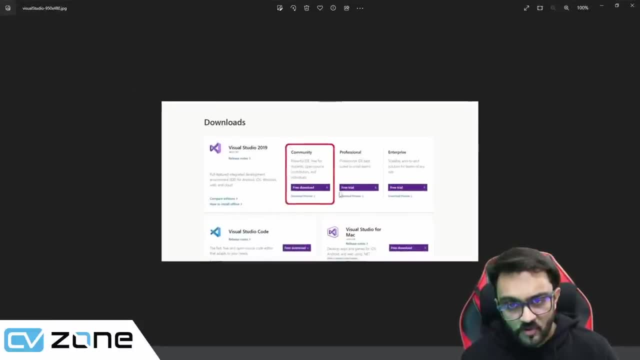 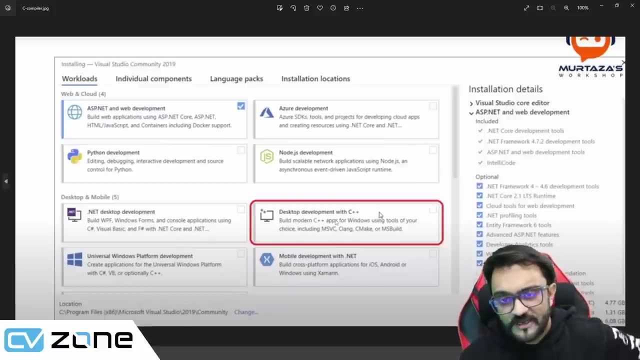 is to go to Visual Studio website. You can go to Downloads and download the community version, which is available for free, And when you are installing it, make sure you select the desktop development with C++. So we need the C++ compiler and this is the easiest way. 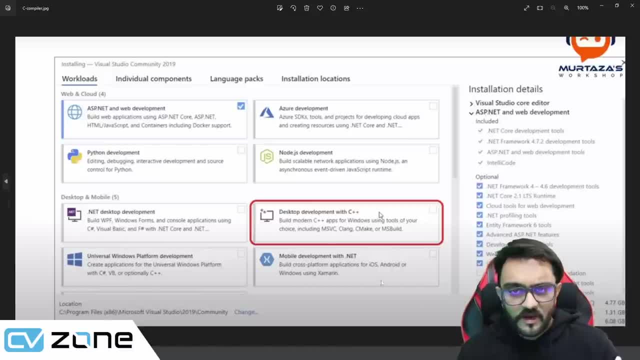 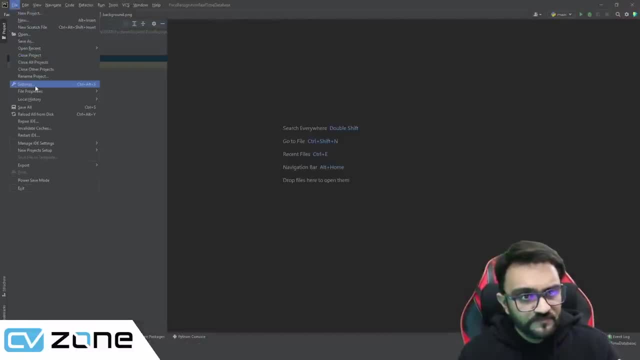 to install it. So just go ahead and do that. It will take a while because it's quite large, And then, once it's done, then we can go on to File Settings. By the way, the project name is Face Recognition. 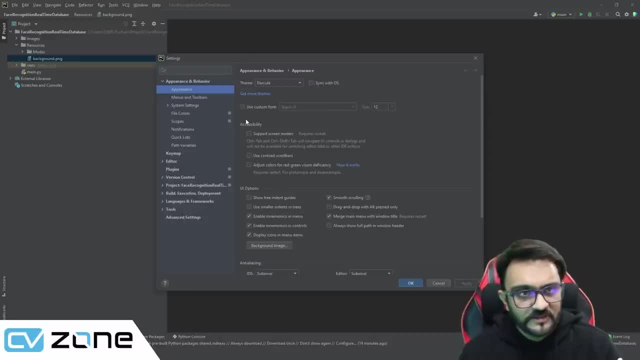 OK, So this is Face Recognition Realtime Database. So this is the name of the project. This is using PyCharm. If you're not familiar, this is one of the best IDEs for Python. OK, so here we have the project. 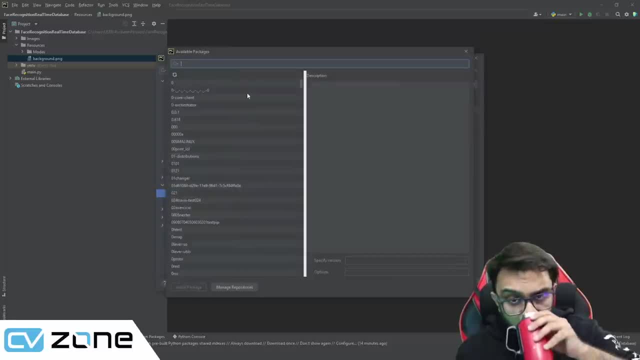 We'll go to Python interpreter and we are going to Add. So here, first of all, there's a list of libraries we have to install And make sure you install it in the same order. So first of all, we are going to install CMake. 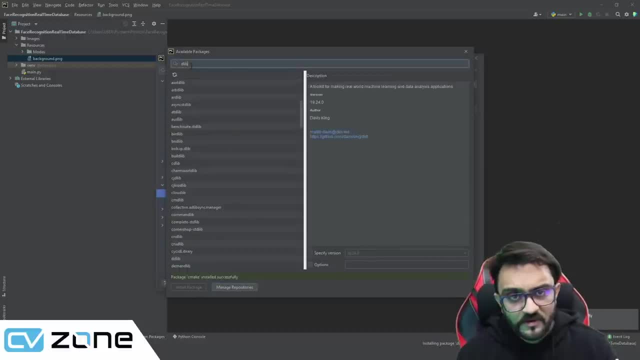 Then we are going to install Dlib, Then we are going to install Face Recognition. Where are you? Face Recognition? OK, let me just type it: Recognition. There you go, Face Recognition. What else do we need? We need CVZone. 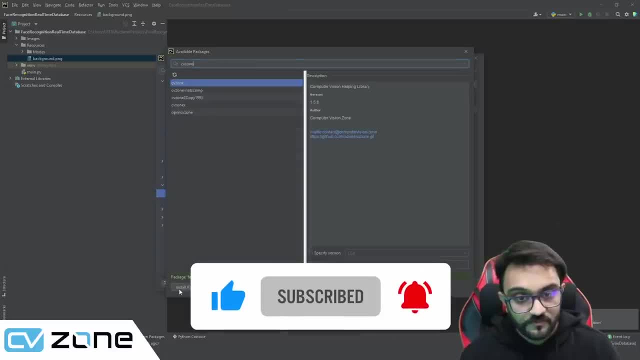 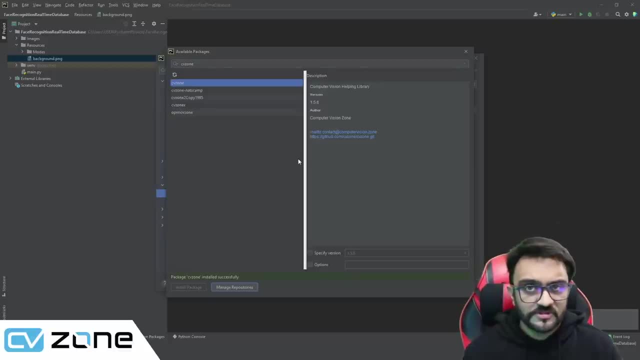 CVZone, CVZone. There you go. So the CVZone is going to install OpenCV and it will install OpenCV, OpenCV, OpenCV, OpenCV, OpenCV. It will also install NumPy. If you don't want to install that, it's up to you. 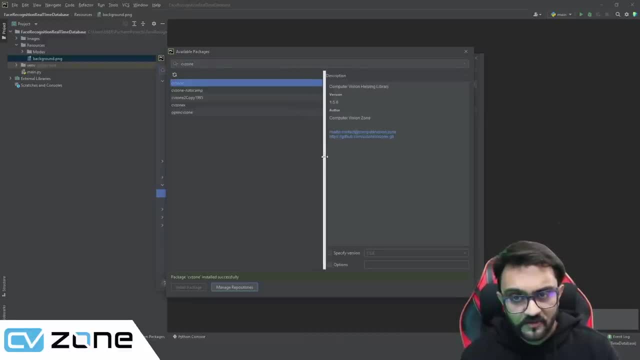 You can just go ahead and install NumPy and OpenCV separately. The reason we are using CVZone is because we are going to take advantage of one of its functions, which will give you a fancy rectangle, So we are going to use that. 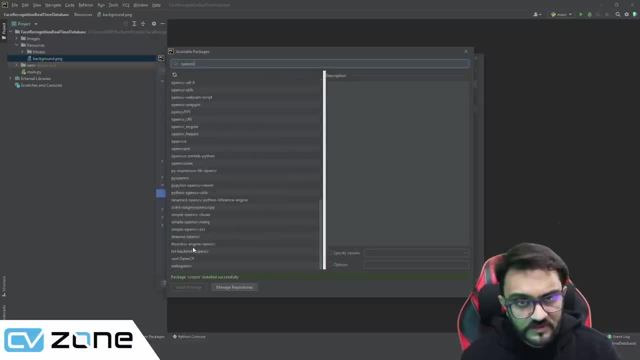 And we will go to OpenCV. I believe it will already be installed, But we are going to change its version and we will downgrade it to 4.5.. 4.5., 4.6., 4.6.. 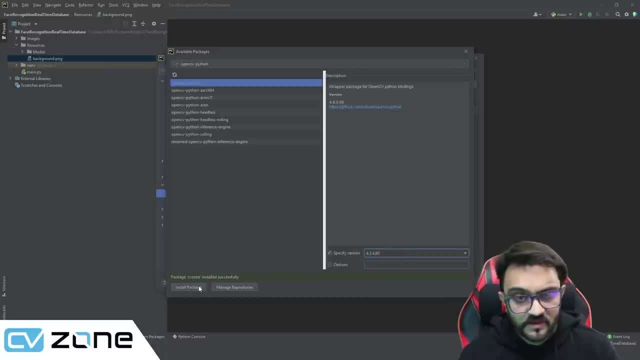 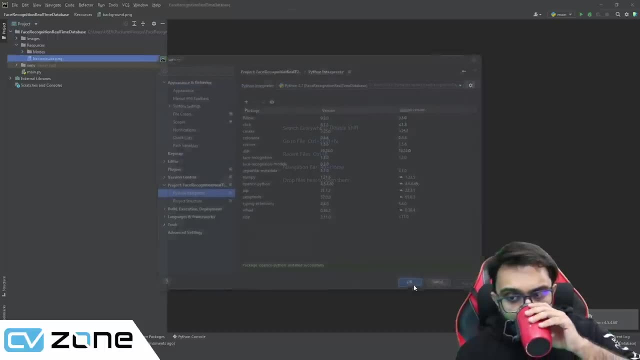 4.6. 0. 0. 0.. This is a little more stable than the newer ones. That's why we are doing this. Otherwise, if you want to stick with that, it's fine as well. I believe all the installations are done. 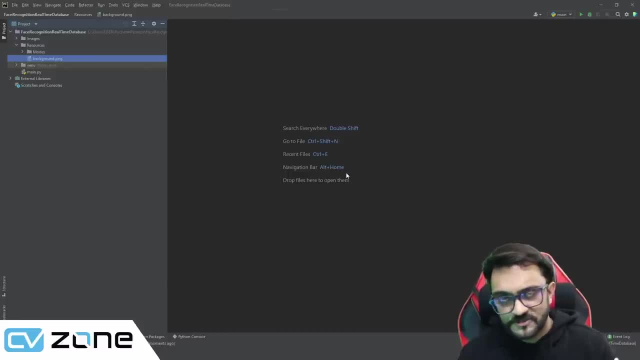 I'm using Python 3.7.. If you are using a later version, that's fine as well, as long as it doesn't give you an error. So if it does, the specific version of Python I'm using is 3.7.6.. 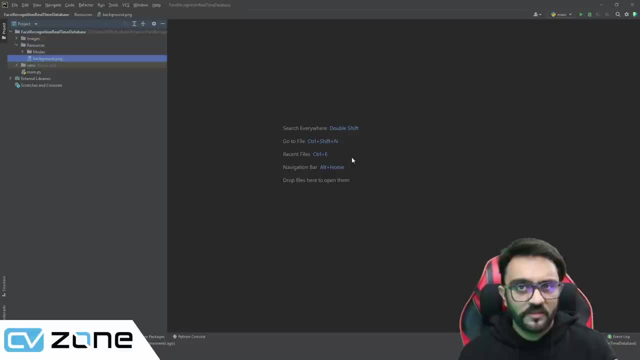 you can upgrade if you want. i believe it will still work with higher versions- 3.8, 3.9- but if it doesn't, you can always come back. so these were the installations. now, what we are going to do, we are going to create a main, main project file. and in this file, what happened? oh, there's already. 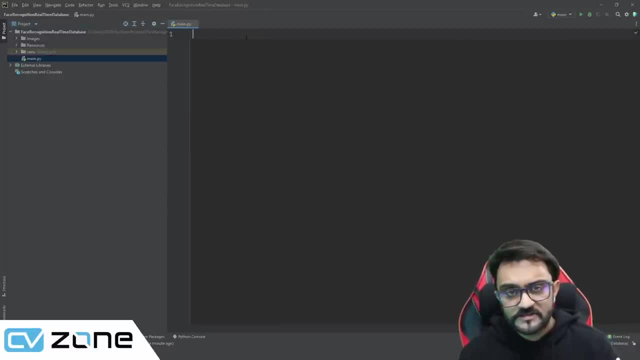 a main, my bad. so we are going to delete that and in in this file we are going to add all the code with all the real-time database and everything working. now the rest of the code that we are going to use will be separate and different scripts and we will name them differently. so here what we can. 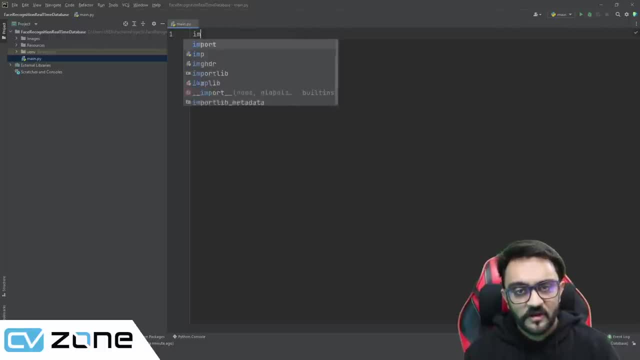 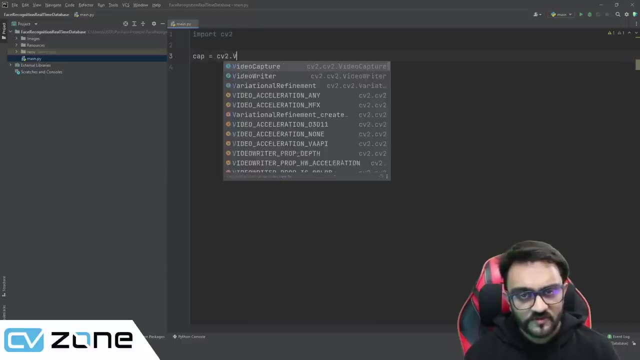 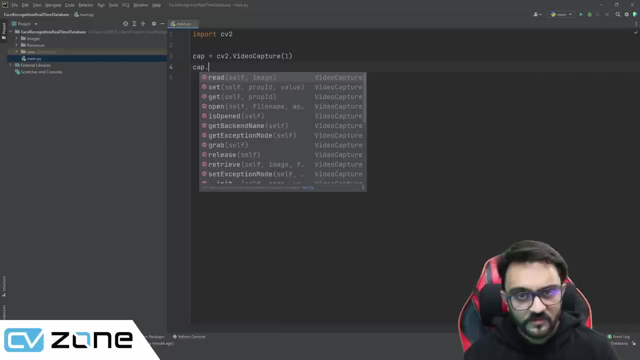 do is we can start with the webcam. so here we can write import cv2. then we will write cap equals cv2, dot video capture, and i am using multiple cameras so i will write one, but you can write whatever you are using, okay, so over here do we need to set? let's just set it, just in case. oh, actually. 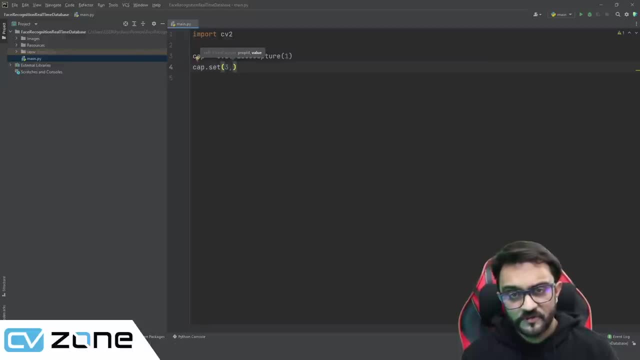 we do need to set it. so, uh, the width, we should be one, two, eight, zero, and the height should be: the height should be: number four is 720.. so we have to specify this because we are using graphics and the graphics are based on these dimensions, so if it increases or decreases, you have to change. 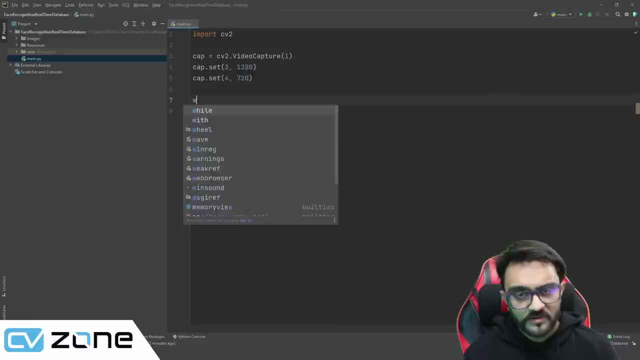 those as well. so then we are going to write, while true, we are going to write success, image equals cap dot read. and then, once it has read, we are going to write cv2 dot- um, i am show. and we are going to write let's say display or let's say face. 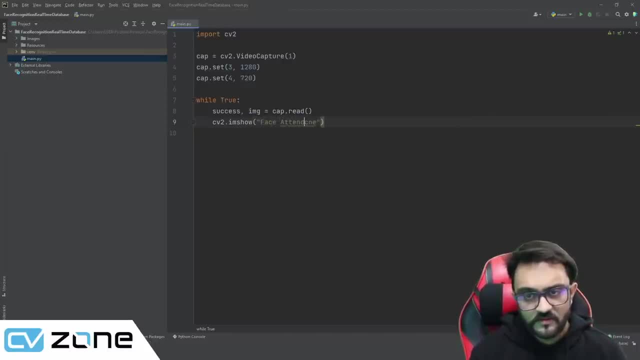 attendance: uh, 10 tens, if i can spell it right. and then we are going to write image and then cv2 dot weight key and we'll give a one millisecond delay. so this is pretty standard, you can say. is the boilerplate template code for running a webcam. 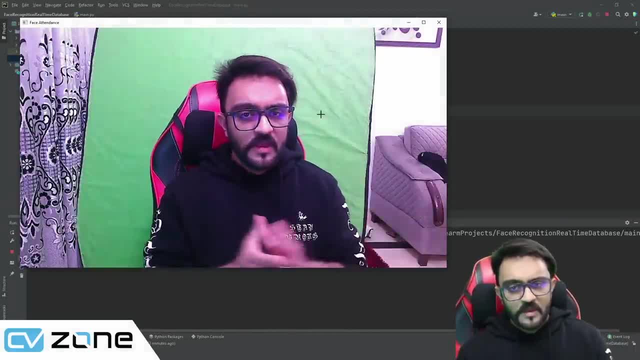 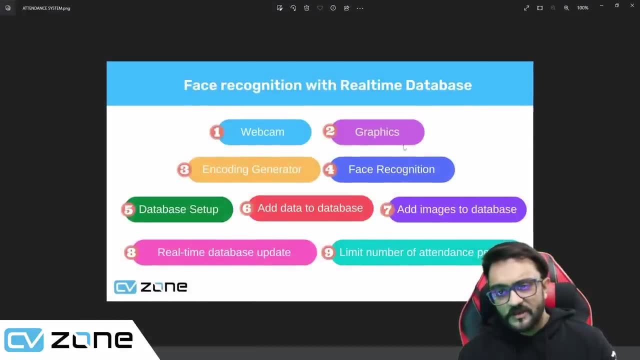 so let's wait for it. and there you go. so now you can see me and the webcam is running fine. so now let's go ahead to the next step. we have done the first part, which is webcam. now we have to do the graphics, so let's import the graphics. 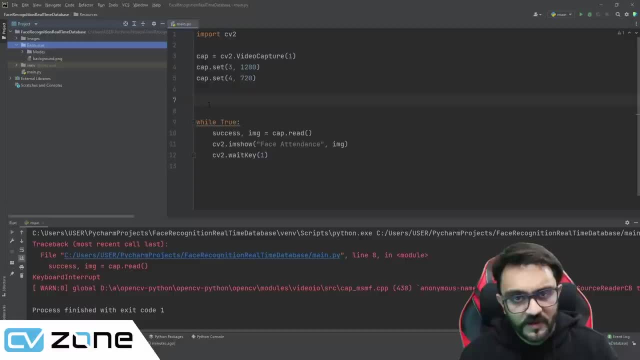 so we have our graphics in the resources folder in the background. so we are going to write here: image, background, cv2 dots. i am read: we are going to give in the resources and background dot png. it will load the image and then we simply have to display it. so we 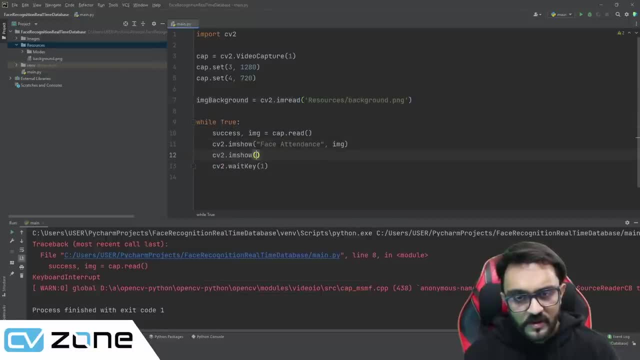 will go here and we will write cv2 dot. i am show and we are going to write here face attendance, then come on and then we will write image background. so this will be the actual output that we are going to use. so here i will change this name and we will write here: webcam. 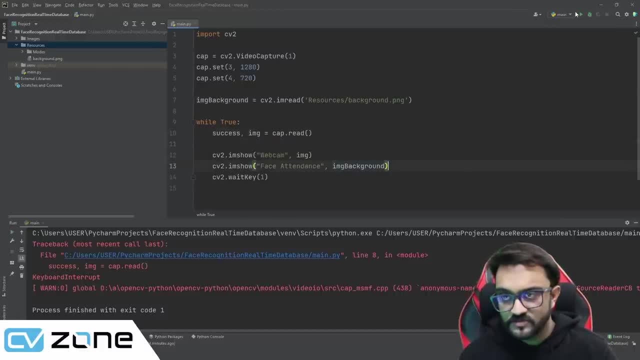 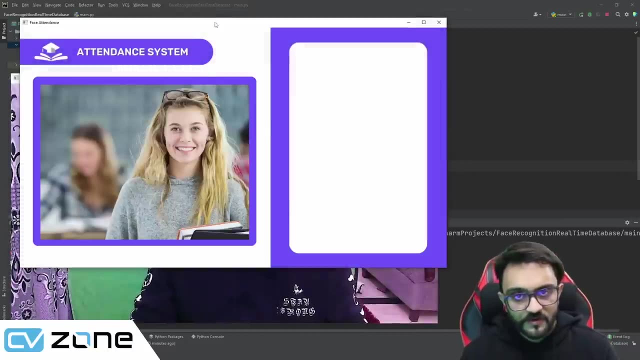 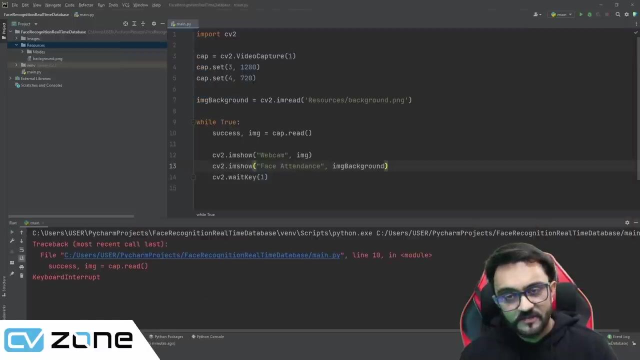 so now we have the webcam and we have the image background, so let's run that and see if it works. there you go. so this is the attendance system and this is our webcam. it's running fine. so that's the idea. actually, i made a mistake. now i recognize it. 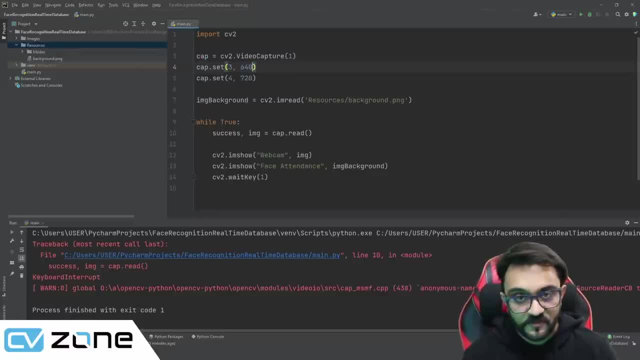 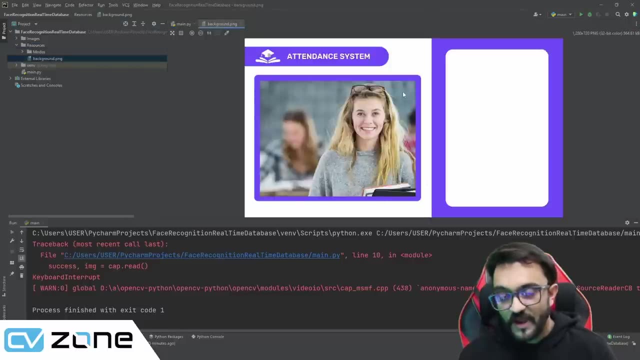 this is not supposed to be 1280 by 720. it's supposed to be 640 by 480, because that's the next thing we are going to do. if you look at the image background, this is the part where we have to add our webcam image, and this is 640 by 480. the complete image is 1280 by 720. 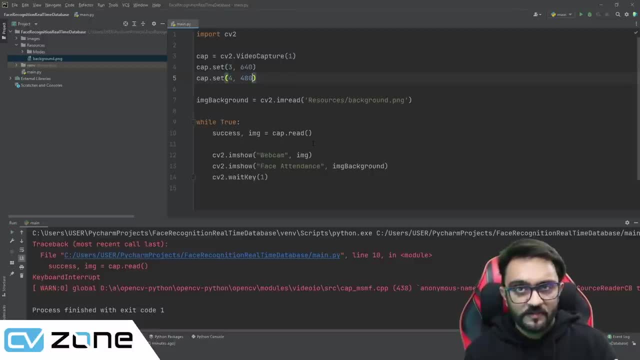 that was the mistake. so now what we have to do is we have to take our webcam and we have to overlay it on the background, because we don't want to display these two things separately. so how can we do that? it's very simple: we will simply write image background. 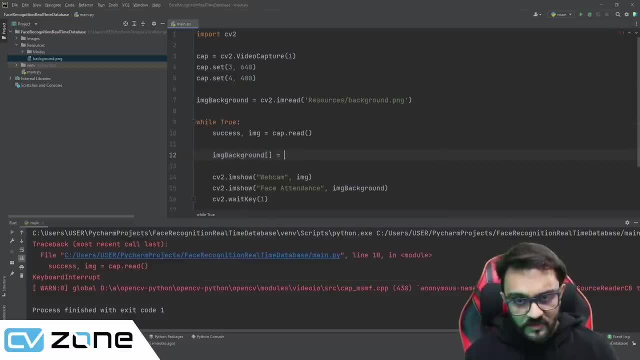 at what exact point equals image. so what are those points? so we have the starting point and the ending point now. i have already checked that earlier and i have written it down, so here what we will use is 162. so that's the height, the starting point of the height: 162, then 162 plus 480, that's. 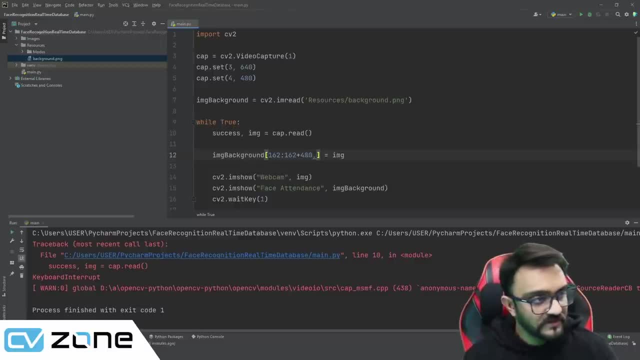 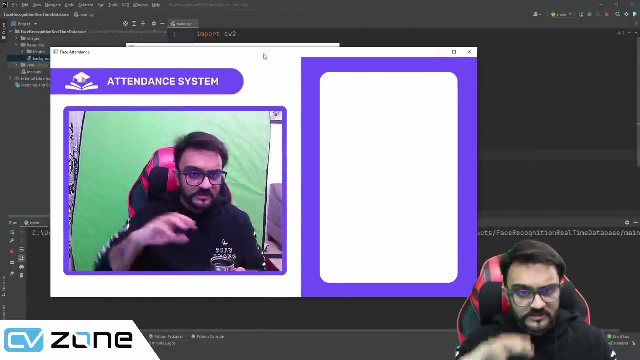 the last point of the height, then the starting point of the width is 55 and the ending point of the width is 55 plus 640.. so that's the basic idea. let's run that again and see if it works. and there you go. so now we have our attendance system. you can see the webcam running. 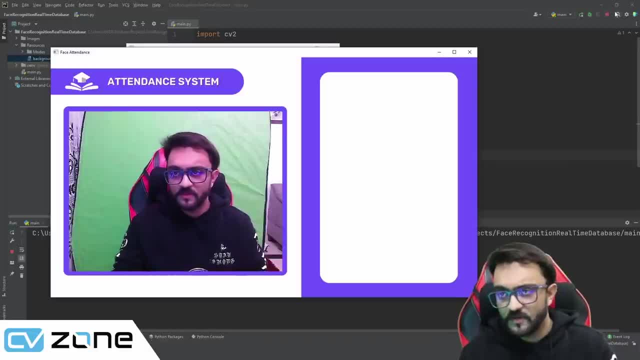 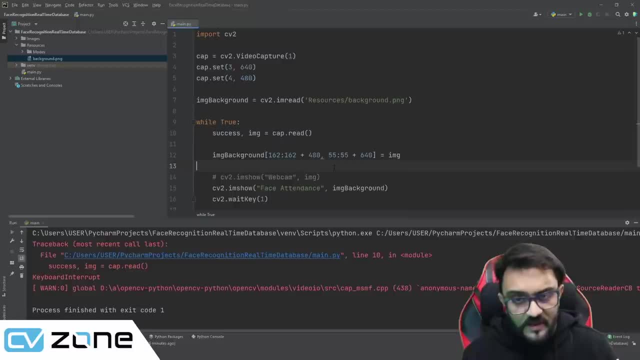 in real time and we have overlaid the webcam image on our graphics. so this is good. now we can actually hide this. we don't need that, and what can we do next is basically bring in the modes, so we should have the ability to change the modes. the modes are basically active. 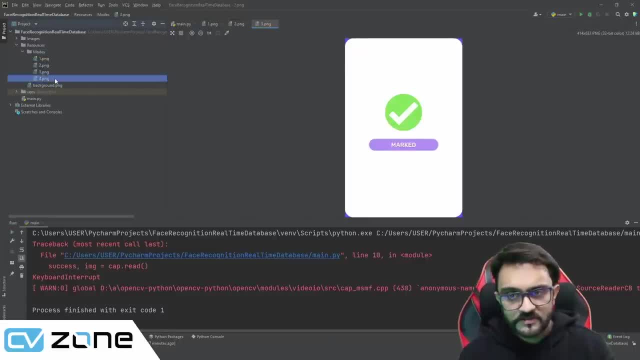 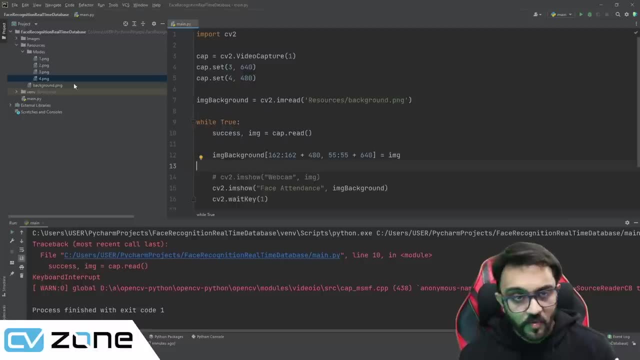 then the information of the student, then marked, and then already marked. so these are the four uh modes that we can use. so let's go ahead and import all these images so we can do it one by one or we can just give in a loop and it will store it in a list, so that's. 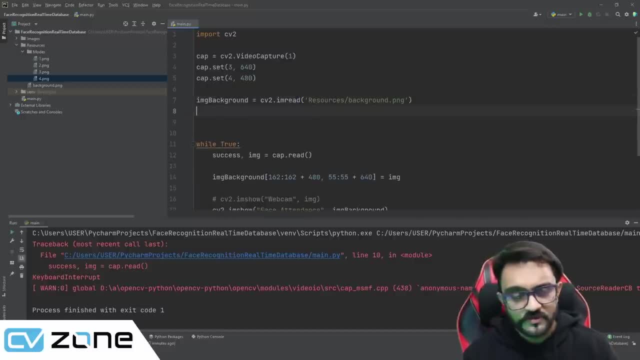 a little bit better to do. so that's why we are going to import it as a list. so for the list, we are going to simply give in the path, so you should have a path, and then you should have the for loop so we can write here folder, for the mode path equals. we are going to write resources. 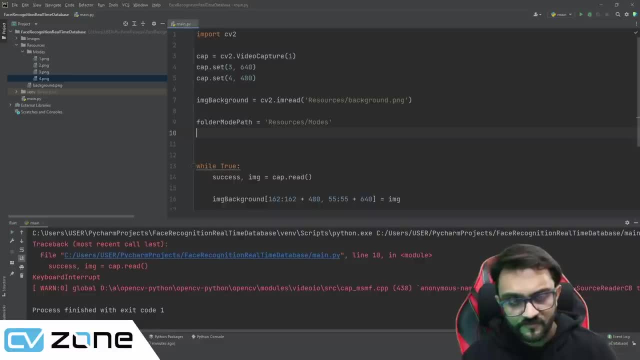 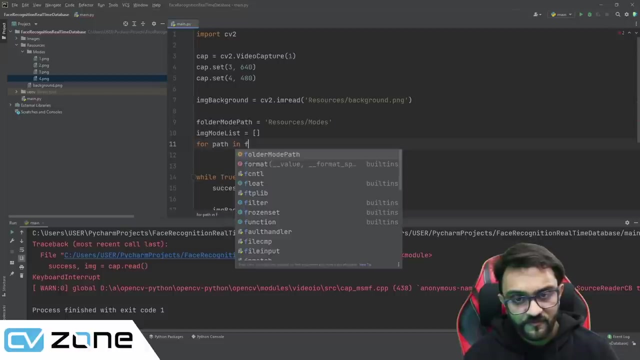 slash modes. so this is our folder mode path and then the the list that will contain all the images. we are going to call it uh. image mode list equals empty, and then for the for loop, we are going to write four uh paths in folder mode path. um, no, no, no, no. what are we doing? folder mode path. folder no. 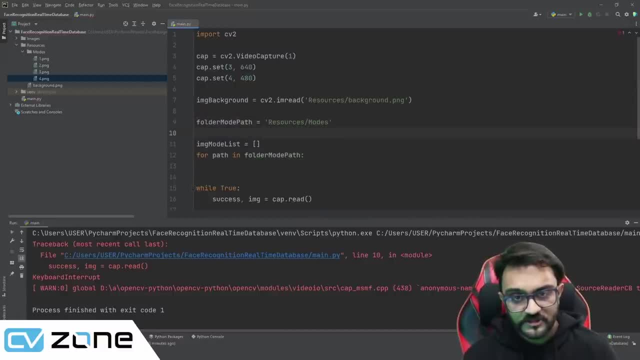 actually i forgot that we actually need another path. so we need mode path equals os dot list directory, and then we will get the name of all these- uh, what do you call images? so if you are confused, like i was 30 seconds ago, then let me show you what exactly i mean. so if i print this out- uh, mode path list, you will see that. 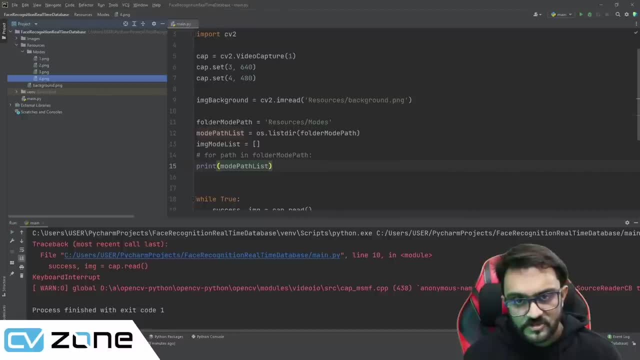 it will contain 1.png, 2.png, 3 and 4.. so the reason we gave this is so that if you're changing in, uh, you have different folder structure, you can simply type it here instead of writing it here. it doesn't make a big difference, though. 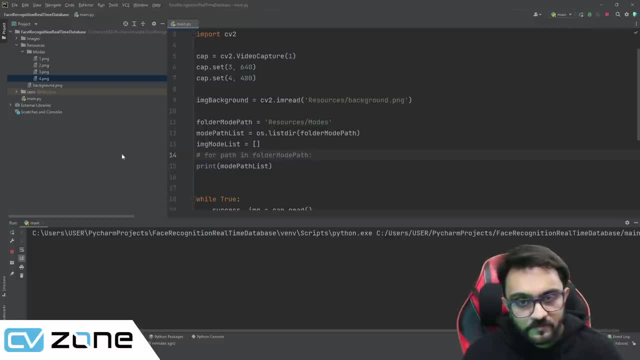 so there you go. so it contains all these names: 1.png, 2.png, 3.png, 4.png. so now we can take this part and we can add it to folder mode path and it will give us the complete link of the image. so that's how we can import. so that's why we need this. so we are going to remove this for path in. 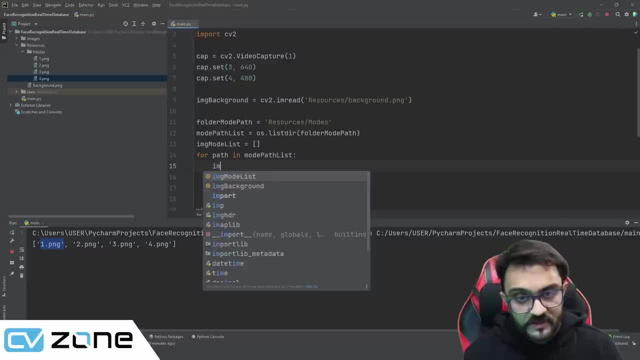 mode path list. we are going to write image modelist listappend. We are going to add it to our list. What exactly are we going to add? We are going to add an image that we imported, So image cv2.imread. that's how we import it And what exactly is the? 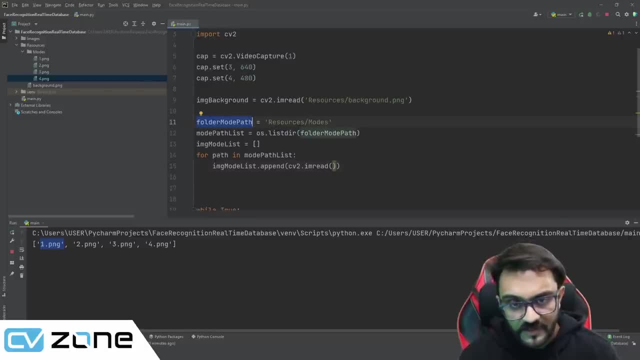 path. The path is this: folder mode path plus this path. So we are going to write ospathjoin and we are going to write folder mode path and path. So that will add the images to our folder. and just to make sure, we are going to write print the length of image mode list. So that will tell. 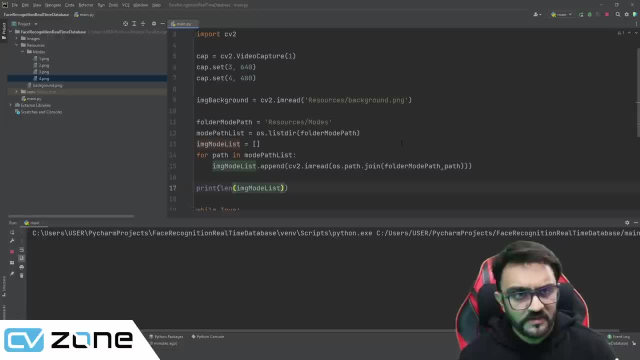 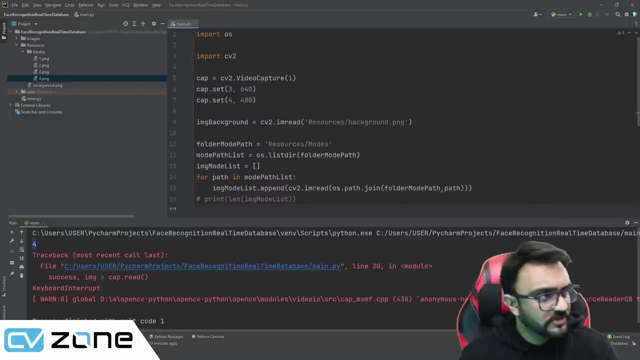 us whether we have imported all the images or not. It should be four images. There you go. It's giving us the value of four. It means we have imported all the images correctly. Let me just hide it out so that if you want to test, you can test it as well. Now, it's good if you actually comment it. 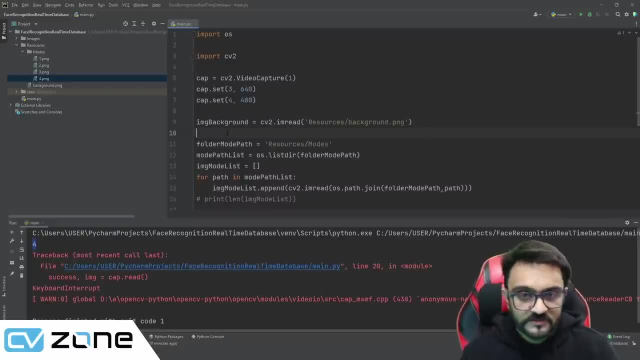 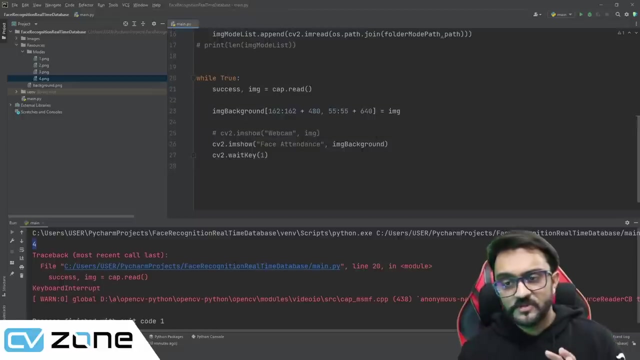 out, not comment it out, if you comment it. So here we are going to write: importing the mode images into a list, right? So that's what we are doing. Now what we will do is we will add this to our what do you call background image. So we'll. 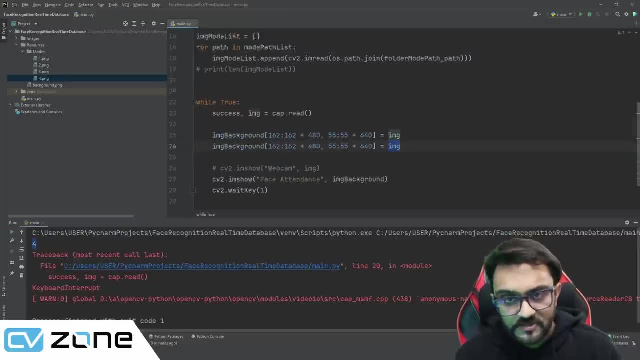 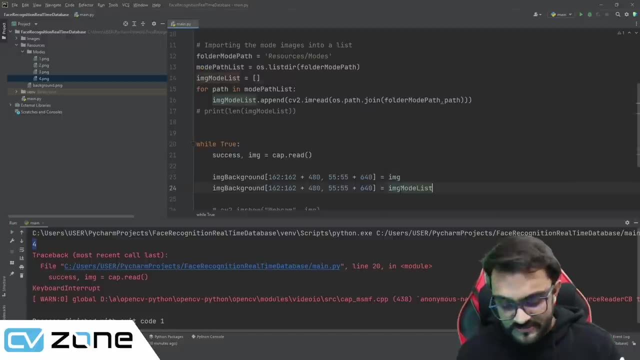 copy this part, we'll paste it And instead of image, this time around we will have one of these images, the ones which are in the image mode list. So image mode list at any instance. So, for example, we'll put zero, so it will give us active, Then it will give us image. We can. 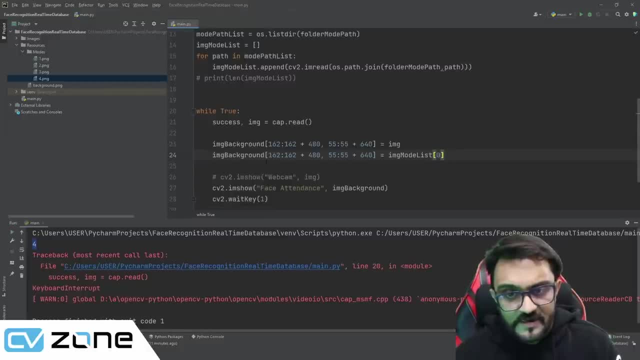 actually test it out. So that's the idea, And then here we have to change the values because it's not the same position. So what exactly is the position? Let me check. So we have 44, then 44 plus 633.. And 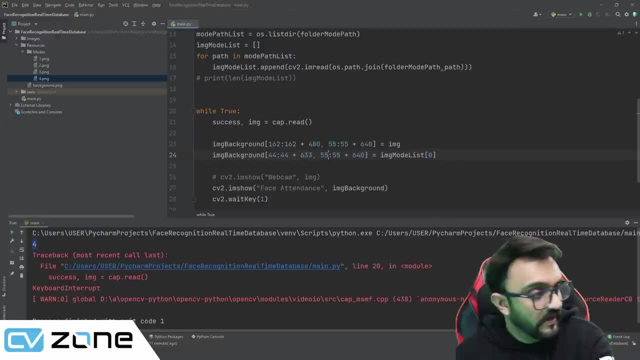 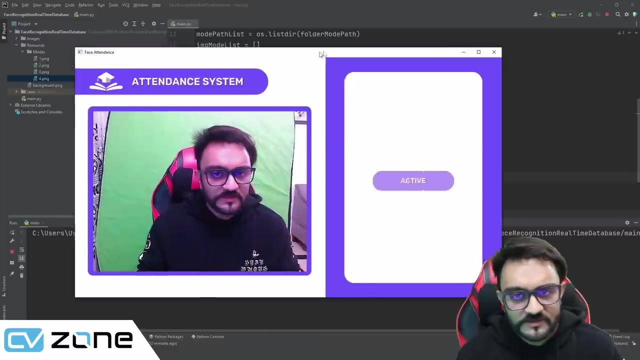 what happened there? Nope, 633.. 633.. and then we have 808, 808, 808 plus 414. so again, you can check it yourself. so here you can see. now we have the active mode and what we can do is we can check the rest. so if i put one here, 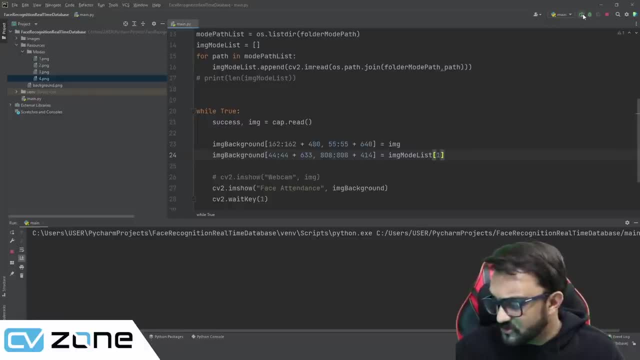 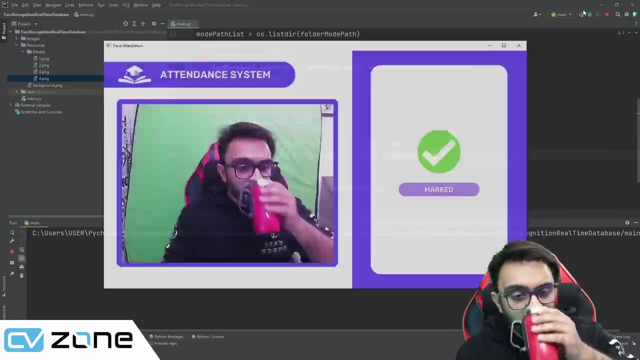 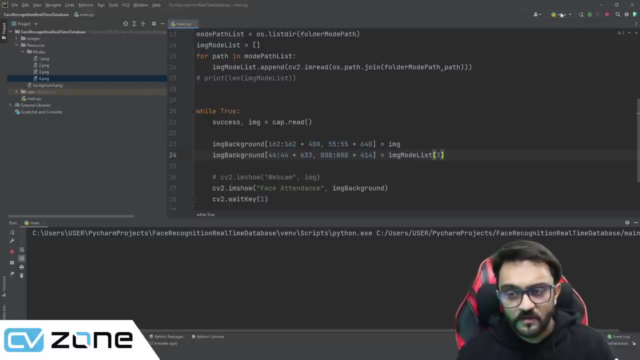 it will give us the next mode, which is for the student. it will show the image and the data of the student. there you go, and then what we can do is we can put two, and it should show us marked. there you go, it's showing us marked, and then, if we put three, it will show us already marked. 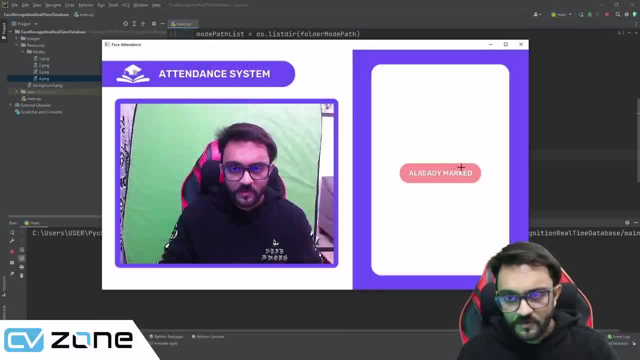 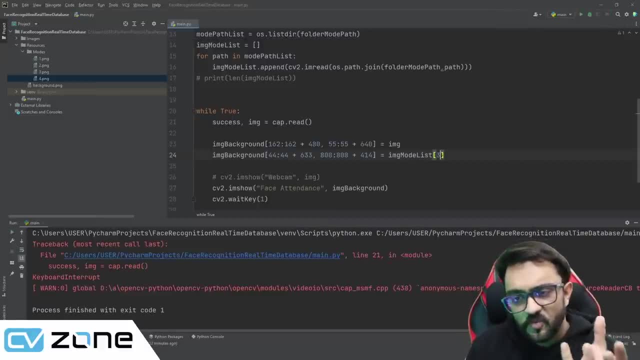 there you go. so these are the four images, the four modes that we are going to use. so now, what exactly can we do? we can simply add a new image and we can see that we have a new image, and we can see that we have a new. 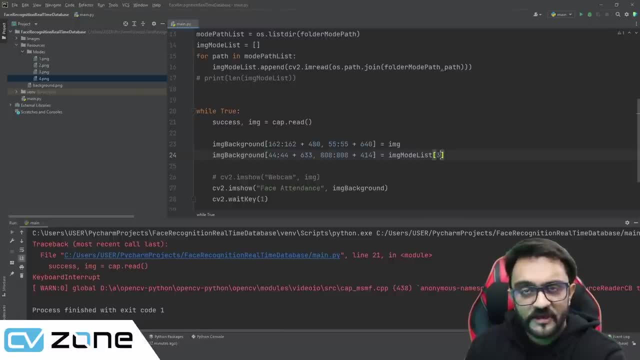 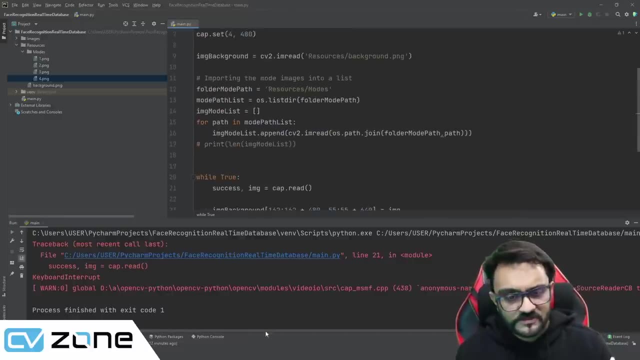 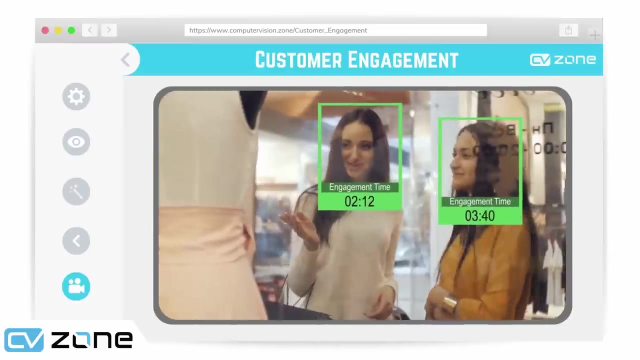 dynamic value. here we can add a variable and based on that variable it will show us the stages. so that's how simple this is. so this part- pretty much for graphics and for the webcam- is ready. the world's first computer vision web development course is here. the power of computer vision now. 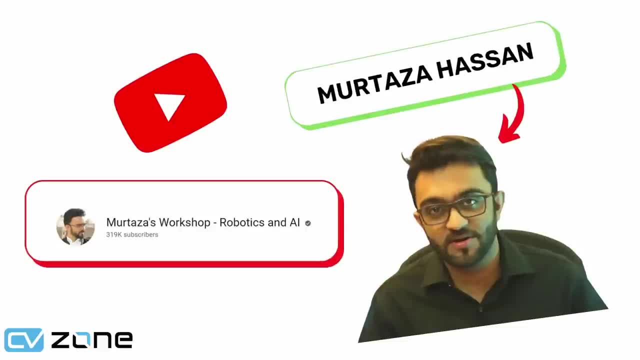 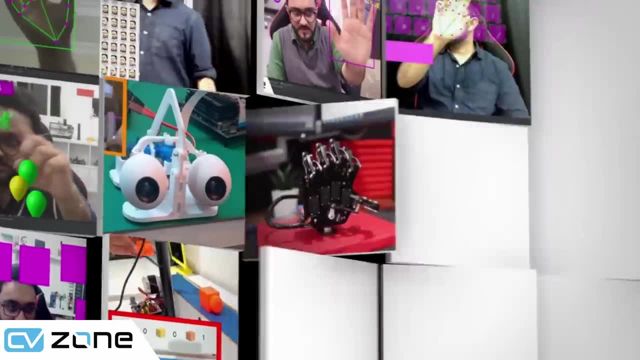 goes into the browser. hey everyone, this is murtaza from the youtube channel murtaza's workshop, which has now over 300 000 subscribers, thanks to all of you. i have been working in the computer vision for the past nine years and have found one big problem: while it's easy to create computer vision, 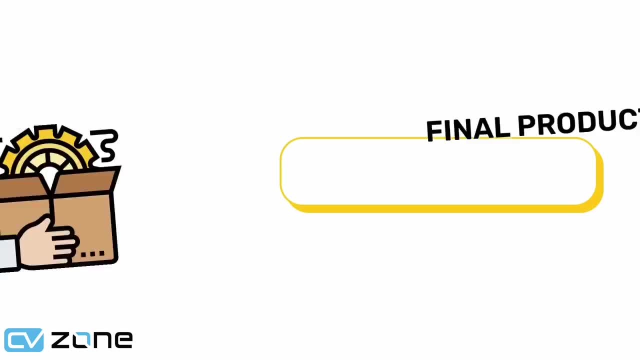 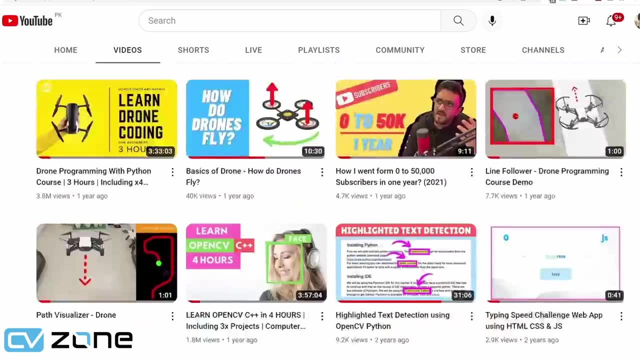 projects, it is very difficult to bring them to the market as final products. trust me, i have over 100 youtube tutorials on computer vision with python which are excellent to get started, but providing it as a solution to a company is extremely difficult and not effective. so now comes. 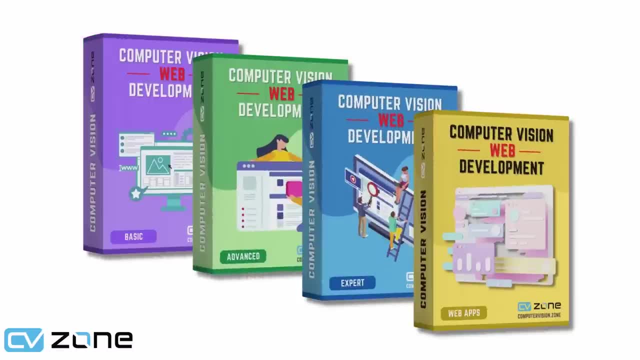 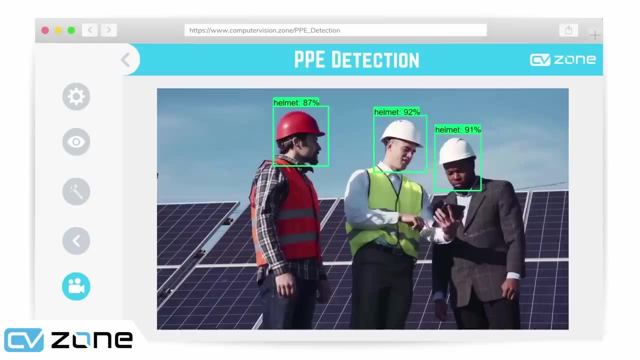 the solution. we have created the world's first computer vision web development course. here you can create your own computer vision web development course. here you can create your own computer vision ideas and deploy it to the web as web apps. this will allow you to create solutions that can be. 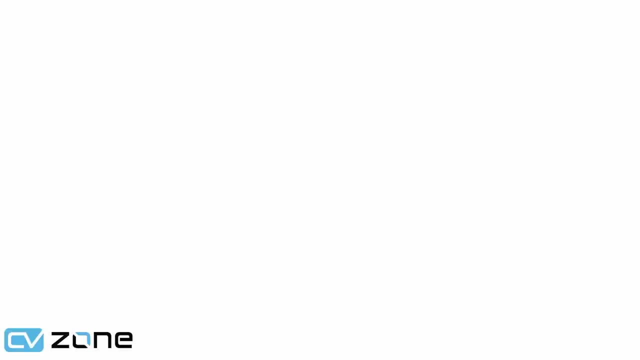 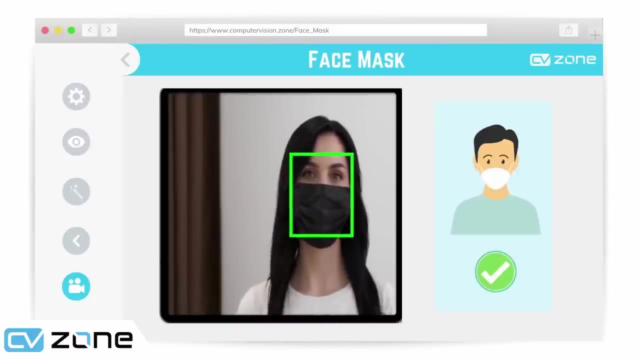 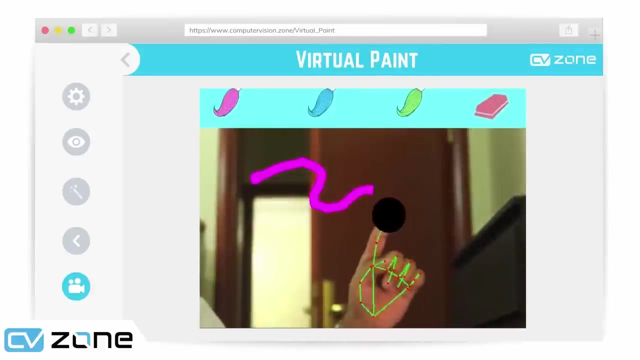 shared with anyone with just a web url, no installations, no running behind library versions, whether you are creating a mass detector for a small company or a traffic analyzer for a governmental project, using computer vision web development, you can create and deploy your computer vision algorithms at ease, while maintaining and scaling them. but what exactly can? 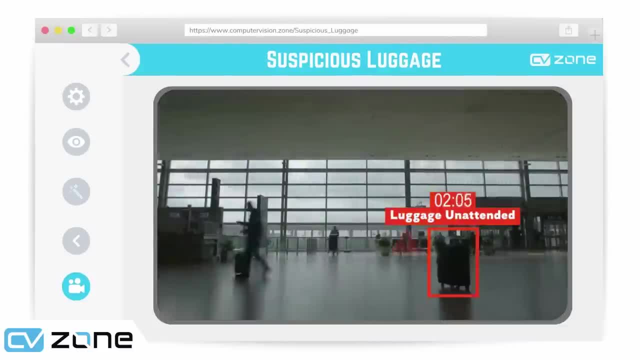 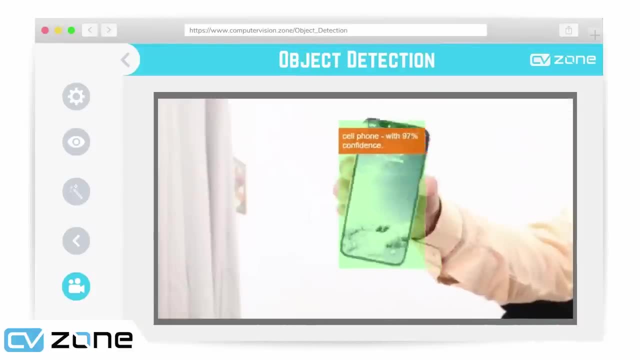 you do in this web app, you can create a system that will get the best results for you. within a few minutes of your knowledge and experience, you can create a web app that will give you access to every Windows program in your computer. you can create different controllers, for example. 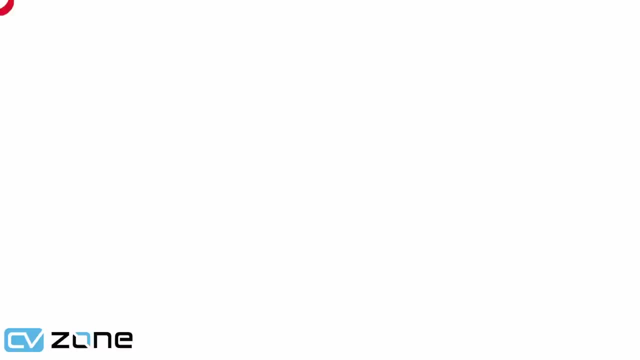 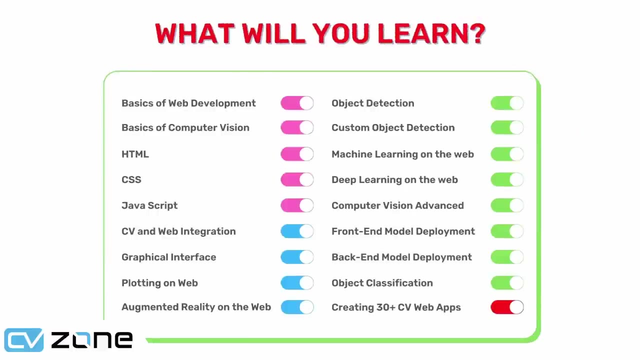 you can create your own computer vision web app as well. you can create your own web apps with a free telephone service and keep up with the web app that you are creating as a community. we have carefully designed this course to take you from the very basics of web development right up. 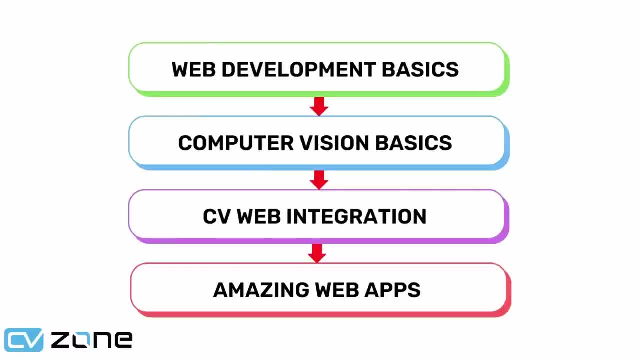 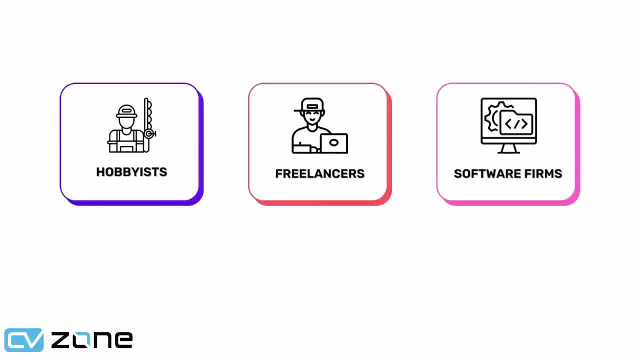 to the point where you can create your own computer vision web apps at ease. this course was created. as This course is not a purchase, but it is an investment. We have designed it for hobbyists, freelancers and software firms that want to level up their 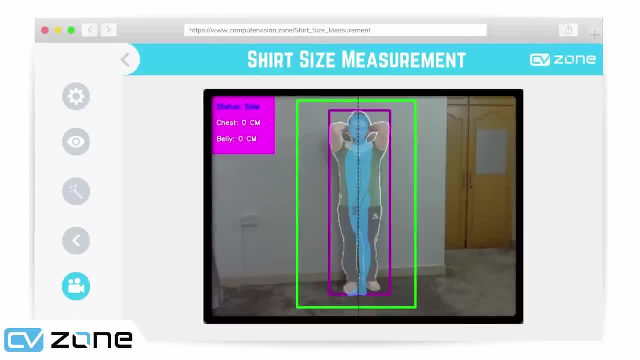 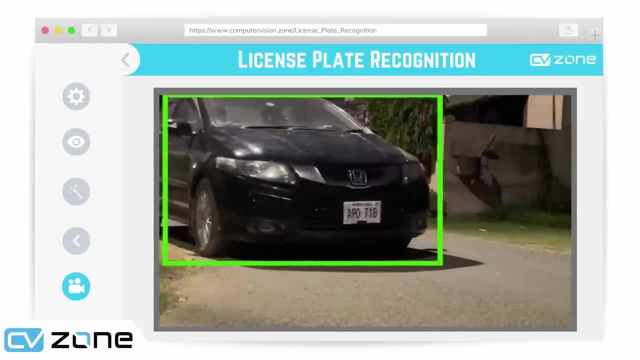 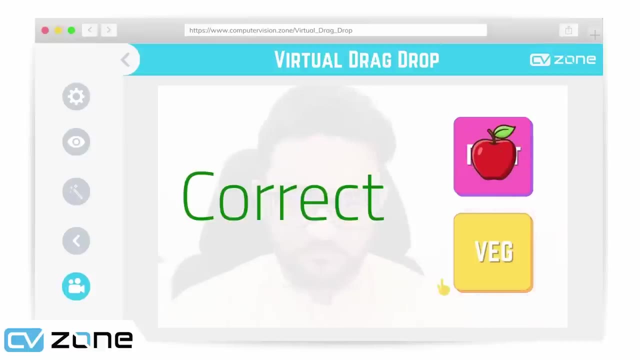 computer vision services. Imagine providing an automated shirt size measurement to a clothing company or customer engagement statistics to a shop owner, or creating a license plate cloud-based recognition system. This course is meant to monetize the skills that you learn. So what is included in this course? 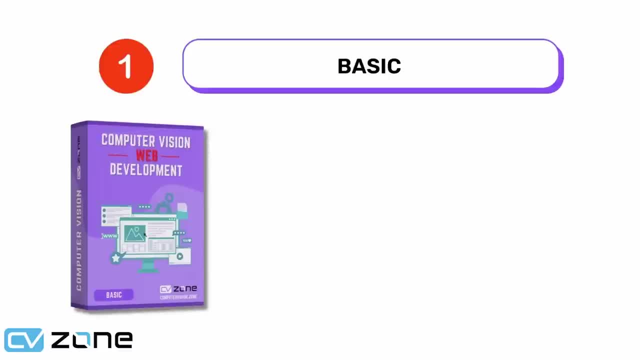 We have split this course into four parts. In the first part, Computer Vision- Web Basics, you will learn the basics of web development, including HTML, CSS and JavaScript. We will go through the integration of computer vision and web development, along with the OpenCV basic algorithms. 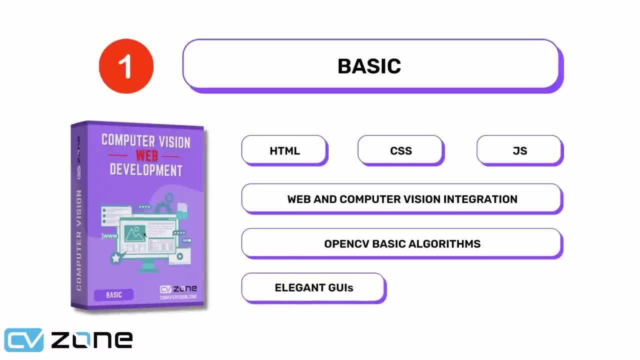 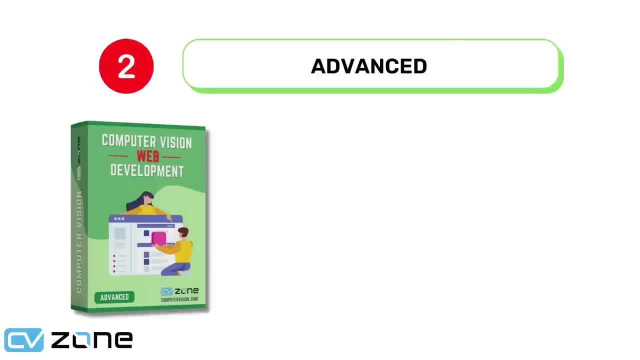 We will also look into creating elegant graphical interfaces for your web apps. This part will include three projects. In the second part, Computer Vision Web Advanced, you will learn face detection, body detection, hand recognition, face mesh detection, body segmentation and much more to create some. 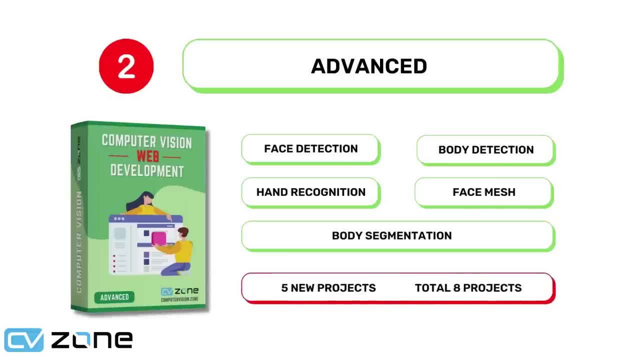 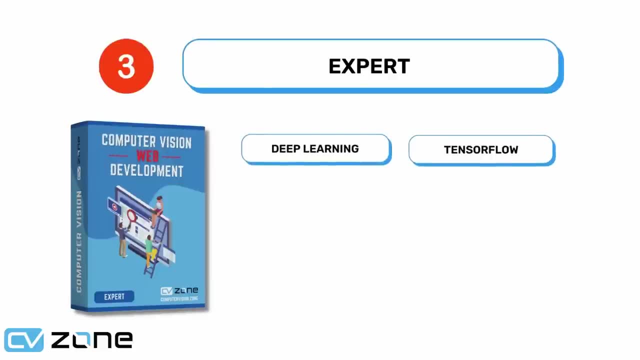 advanced projects. Here we will create five projects to solidify what we have learned In the third part: Computer Vision Web Expert. we will learn the basics of deep learning with TensorFlow on the web. Here you will understand the fundamentals of object classification and object detection. 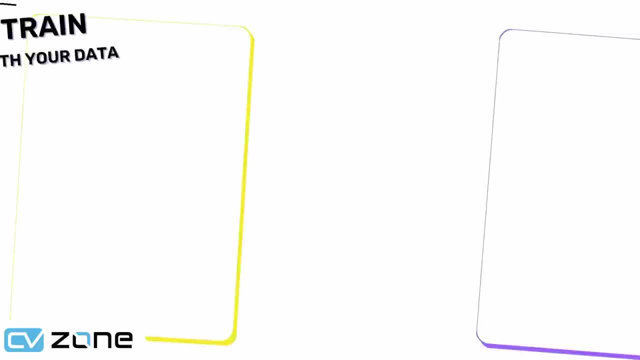 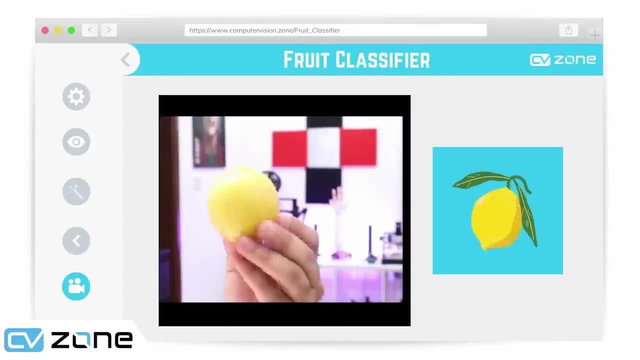 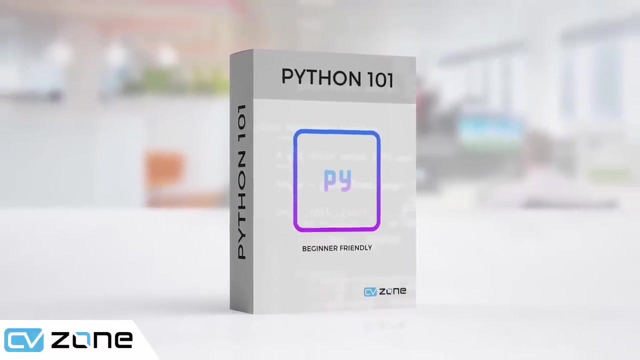 You will use pre-trained model for testing and then learn to create your own models from your own dataset. This will allow you to create object classifications. We will also create three projects in this part. This part will also contain a free Python course that will make it easier for you to. 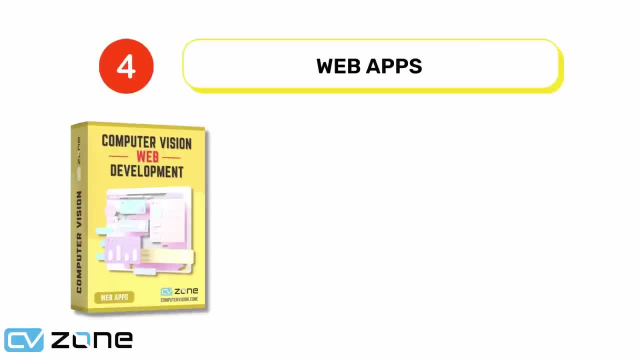 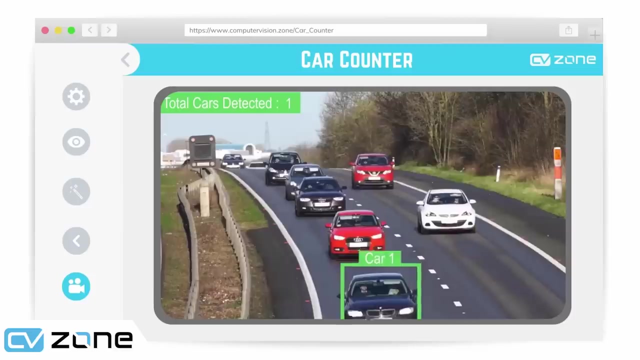 create your own models. The final part, Computer Vision Web Apps, is dedicated to commercially viable projects. We will create more than 20 web apps to get the maximum exposure to real-world applications. These will include automated shirt size measurement, customer engagement, car counter, face attendance. 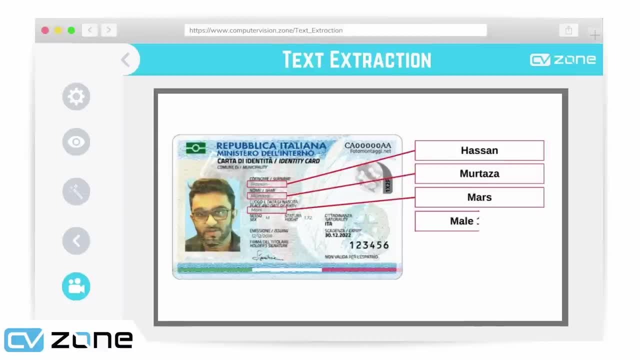 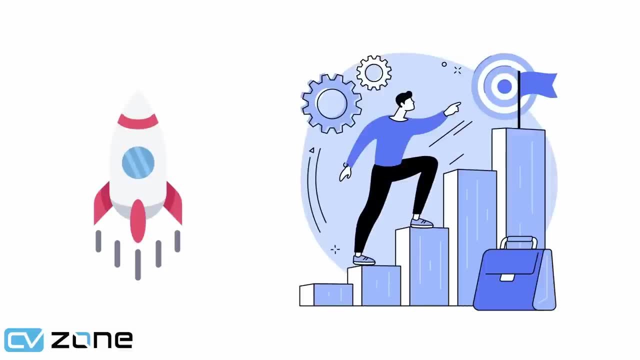 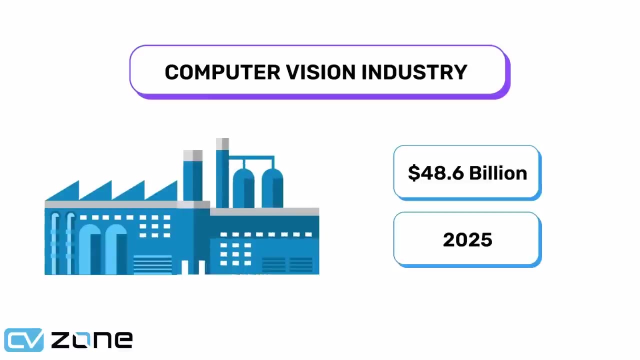 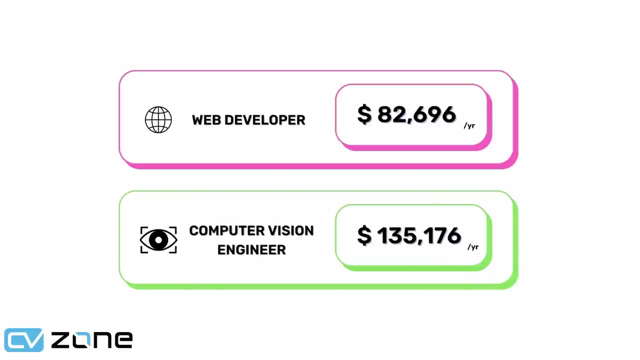 and more. This course is meant to boost your career to new heights. The computer vision industry is expected to be worth $48.6 billion by 2025, with the average salary of a web developer being $82,000 and for a computer vision engineer being $135,000. 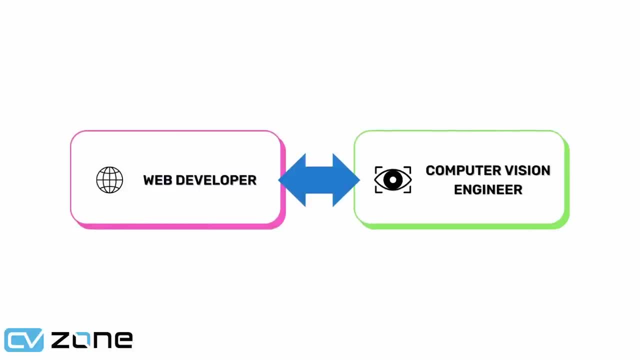 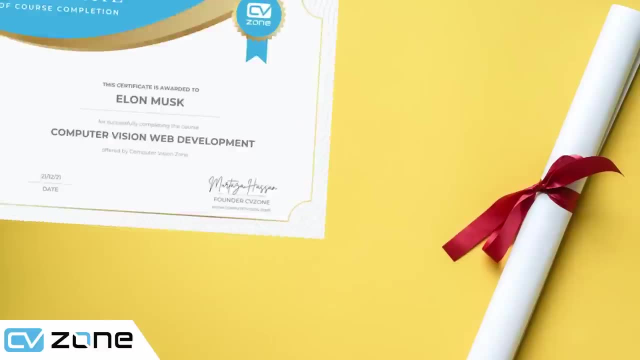 in USA. The merger of both these technologies is a deadly combination that will soon be in great demand, So it's best to get on this train in the early stages. We will also provide certificates of completion so that you can proudly add it to your resume. 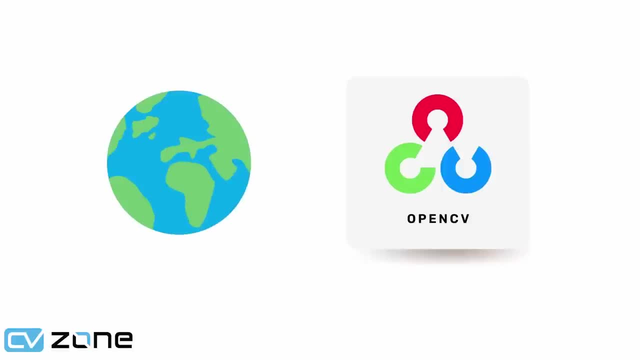 We will be using the world's largest computer vision library, OpenCV, along with the most popular deep learning framework, TensorFlow, so you don't have to worry about the latest tools and technology. And don't worry if you are a beginner who is unfamiliar with HTML, CSS and JavaScript. or even an intermediate programmer who has these skills but needs some polishing. We will also provide certificates of completion so that you can proudly add them to your resume. We will be using the world's largest computer vision library, OpenCV, along with the most. 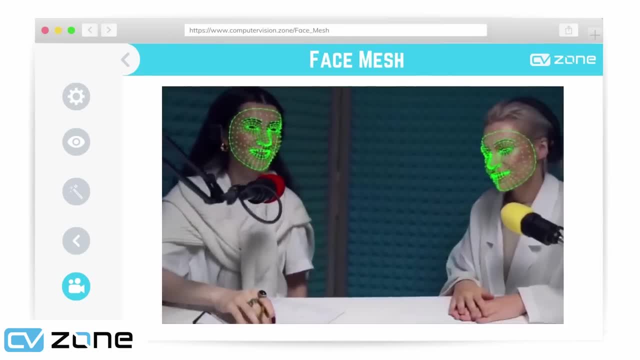 popular deep learning framework, TensorFlow, so you don't have to worry about the latest tools and technology. We will also provide certificates of completion so that you can proudly add it to your resume. And don't worry if you are a beginner who is unfamiliar with HTML, CSS and JavaScript. 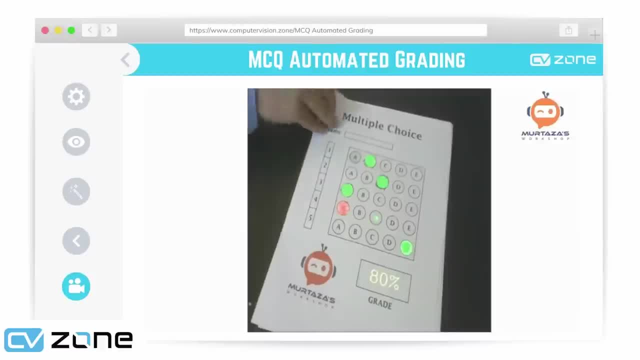 or even an intermediate programmer who has these skills but needs some polishing. We have got you covered. We created crash courses that will teach you the basics to get started, And only for our kickstarter backers we will be providing free HTML, CSS and JavaScript. 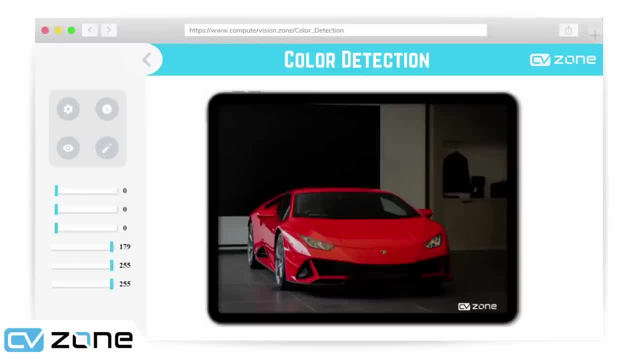 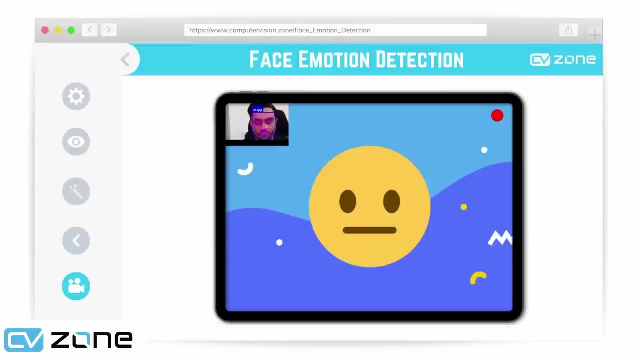 ebooks along with their video courses to get you started. There is a reason why this has not been done yet on a large scale. It is very difficult to create lots of commercial projects that are optimized to run on the web. Not only that: going through all the bugs and finding their fixes takes a lot of work. 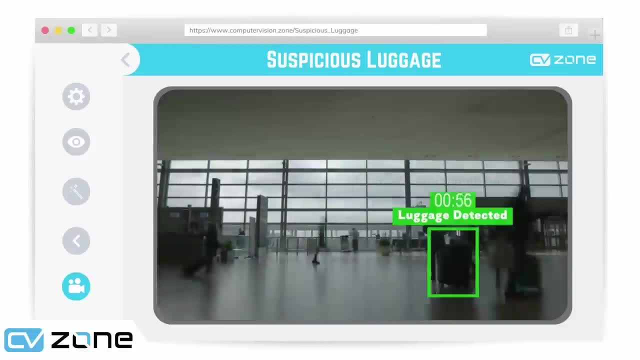 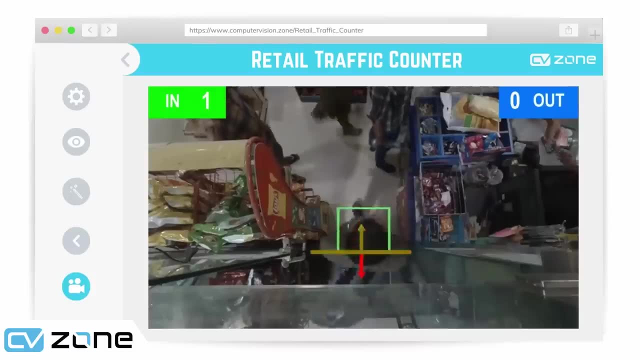 But we took the first step and started working on it. So let's get started, And now we need your help to bring it to reality. We have written the code for almost 70% of the projects and the basics, And now we need to start production. 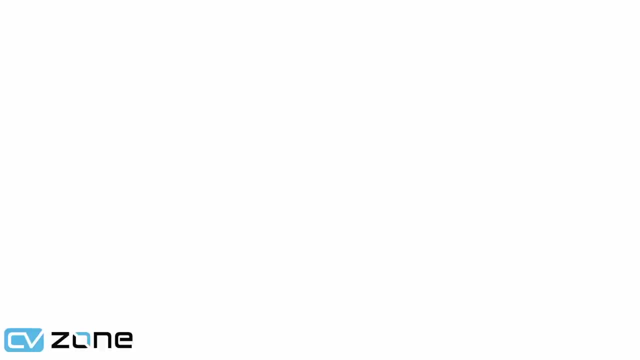 Although this is a challenging task, we are not new to this arena. We have delivered 8 high quality and information dense courses prior to this course that have been sold in over 75 different countries. We are confident that we can deliver this course, but need your help to do so. 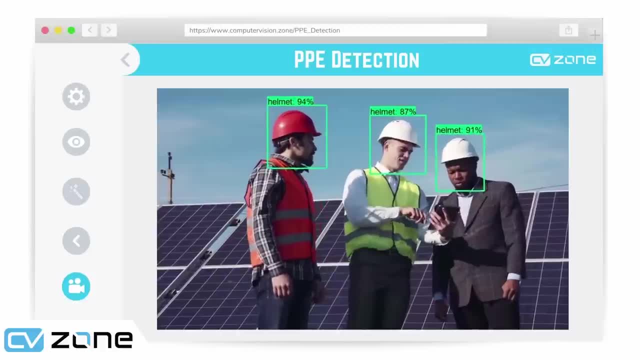 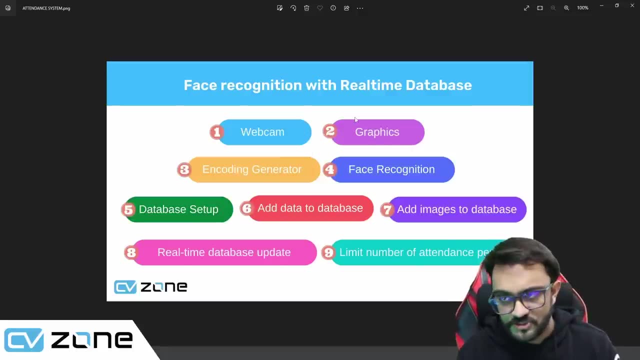 So please join our kickstarter campaign by taking a pledge or sharing our mission with others. So these two are done. Now we are going to move on to the encoding generator. So we have to encode, We have to generate the data for all those 128 measurements and we have to store it in. 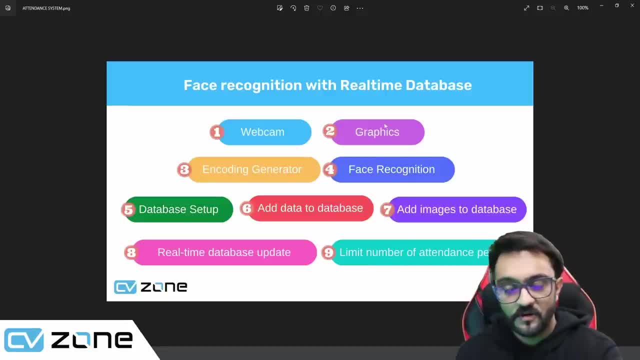 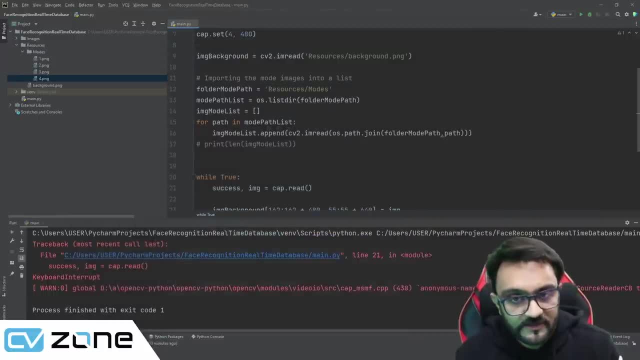 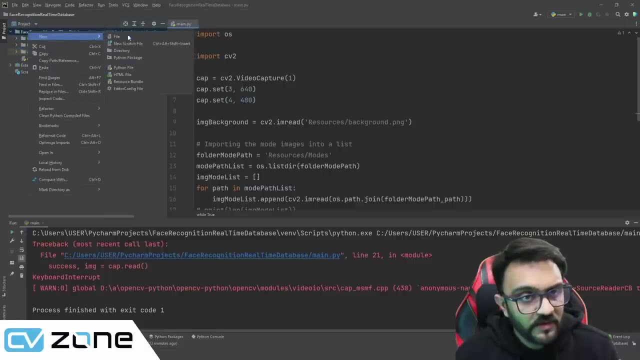 a file and that file we will import it in our face recognition and then it will display whether it has detected that face or not. So that's the main idea. So here what we can do is We can create a new file And we are going to call it. 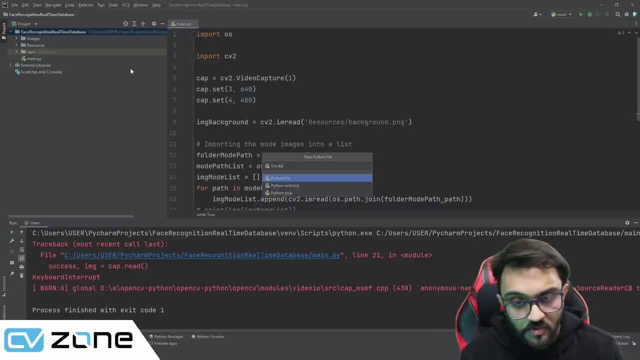 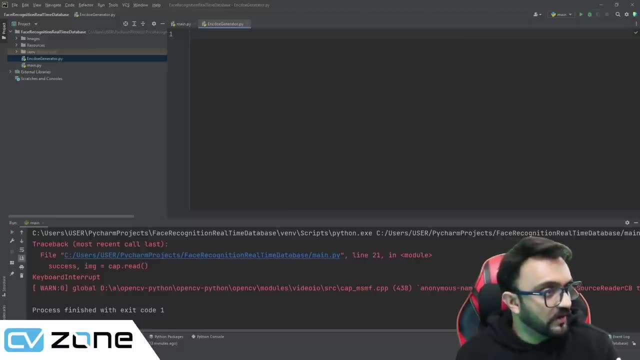 encode generator. So in this encode generator we are going to generate all the code that we need, The encodings that we need of the faces. So here we are going to import CV2 and then we are going to import face recognition, and then we 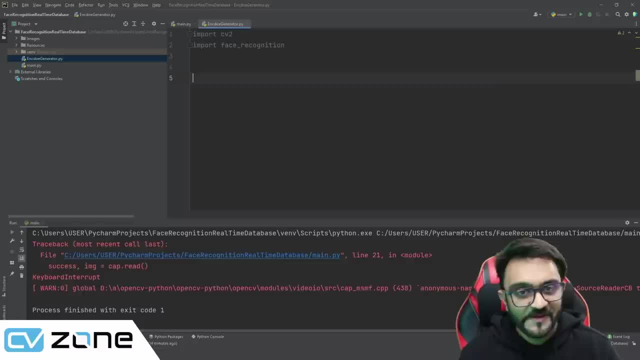 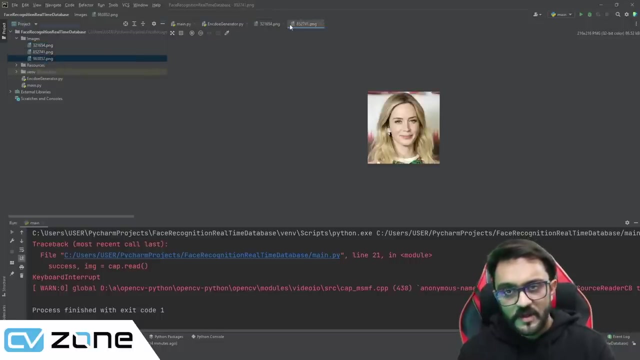 are going to imports, nothing else. okay. so now we need to import all the images once we have the images. the images I'm talking about are the faces, so we have to import these faces. once we have these faces, we are going to encode them one by one, and once we encode them one by one, we are going to store them in a list one. 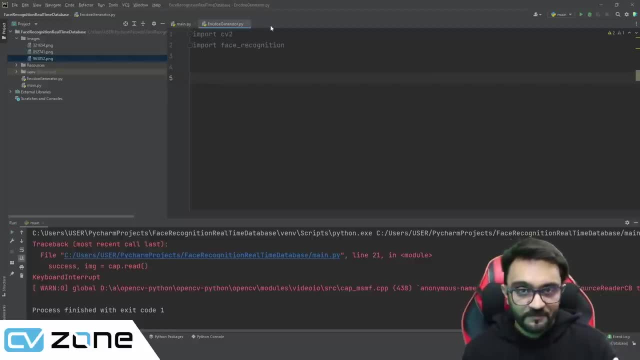 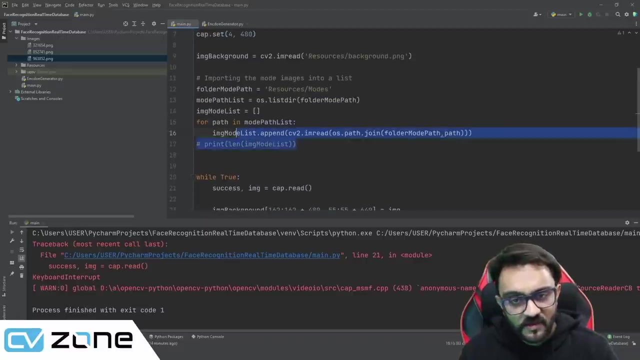 by one, and then we are going to dump it using the pickle library so we can import pickle. so yeah, that's the idea. so here the first thing we will do is we are going to import all the images, and this will have pretty much the same standard as we did earlier for importing the bold images. so here, if we paste it, 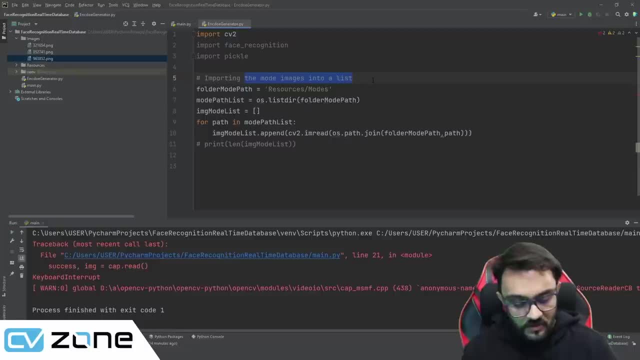 out. so here we can write: importing the student images. there you go. so what exactly is the folder folder path? you can see, here is the folder folder path. and you can see, here is the folder. let's just remove the mode so it is images. so we don't have to write anything. 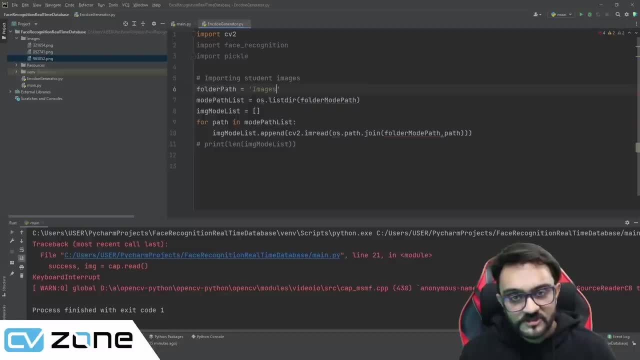 else we'll just write images and from the images we are going to get the list of directory. so let me import OS as well, and then we will get the list of all the images. so so here we are going to write image list, here we will write image list, and here we are going to write. 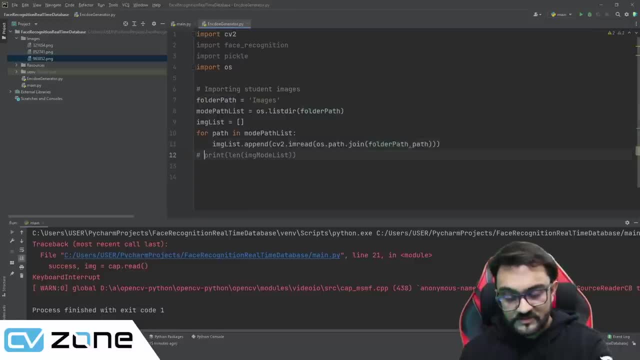 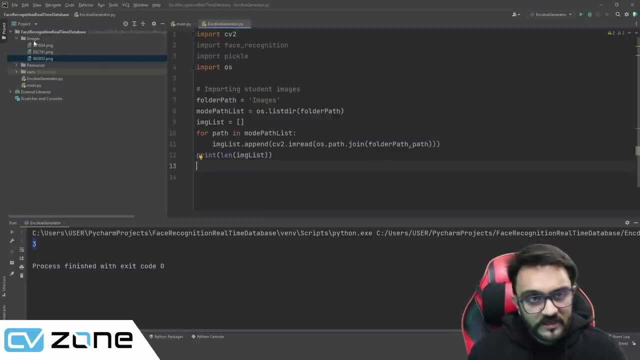 folder, folder paths. so if we run this now, let's see if it imports all the images. we have to change this to image list. okay, so we are importing three. now one more thing we have to do is to import the ids as well. so here each image has an id on it, so the name of the image. 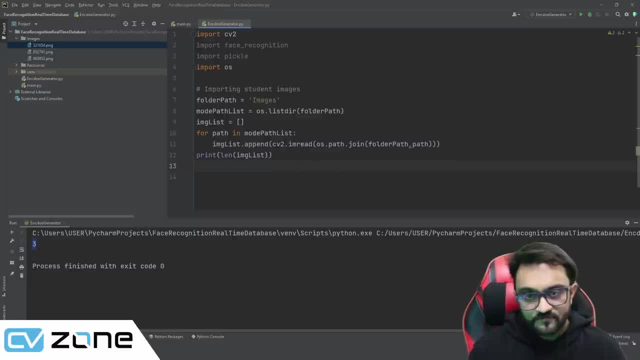 is basically the id, so we have to extract that. so what we are going to do, we are going to write here: student ids equal empty. so here, when we are importing, we are going to import the name. so here we already have this. if we print out, if you write here: print. 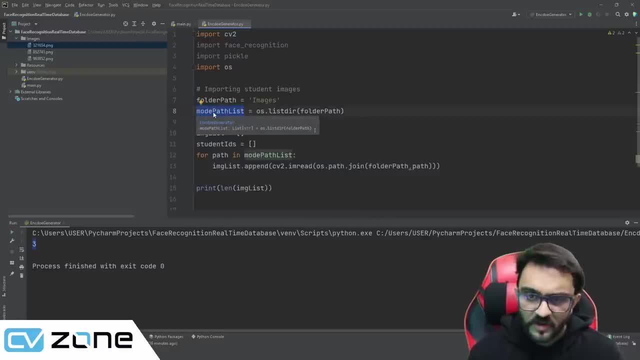 print mode path list. why is it mode? we need to remove that path list, okay, and then we write here path list. so here we will copy and paste and let's see what do we get. so here we are getting all the names. so what we need to do is, first of all, we need to get 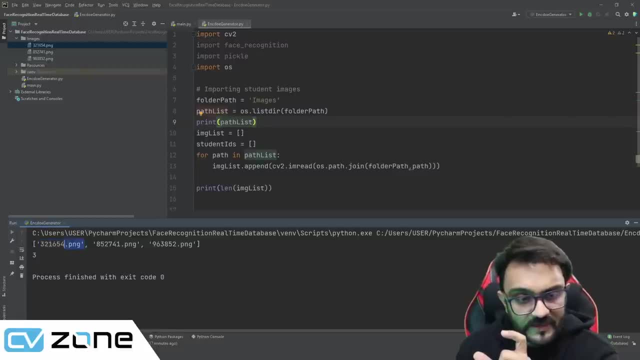 this name. right, we need this id part so we can get this part. it's very easy. all we have to do is we have to write: uh, what was it? path, path. that is exactly what we will get- this dot png. but now we have dot png, so we need to remove that. so if i, if i print this: 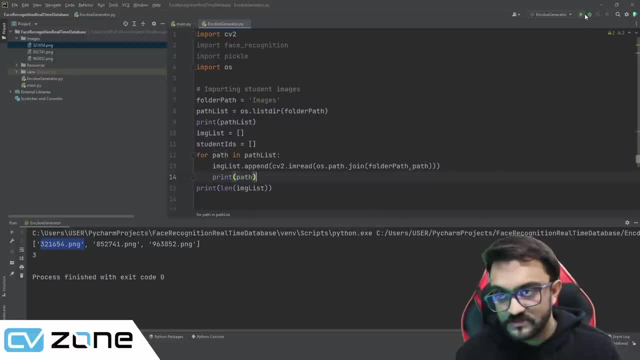 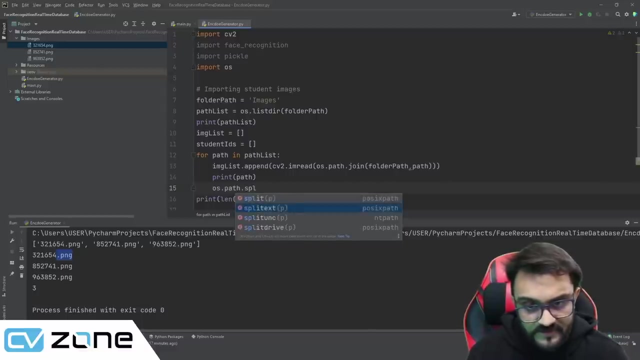 let me show you. if i print this, so it will print all of them with the path, with the png, dot png. so we need to remove this dot png. so how can we do that? we can do that by os dot, path, dot, split text. so here we can write os dot, path, dot, split, split text, and here you have to, given the path. 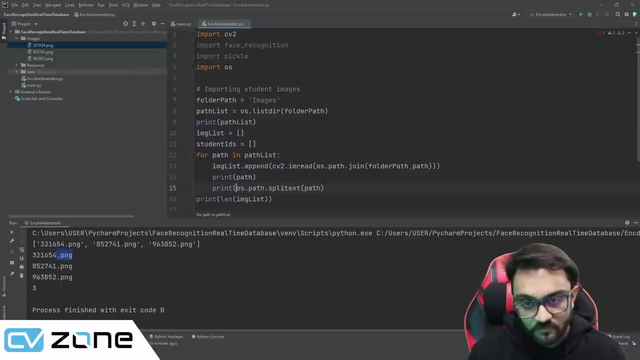 so let's print that out. there you go. so now it has split it up into two parts, one with the id and the other one is dot png. so which one do we want? we want the first one. so the first one to get it. all we have to do is we. 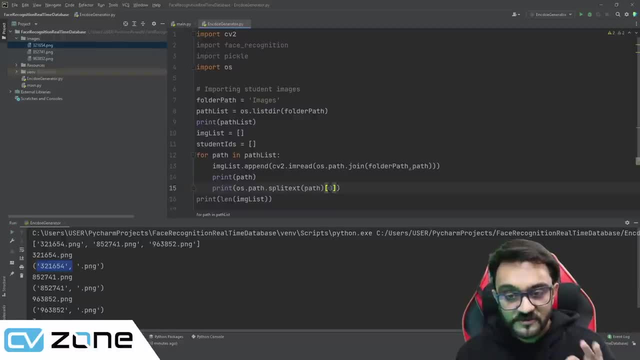 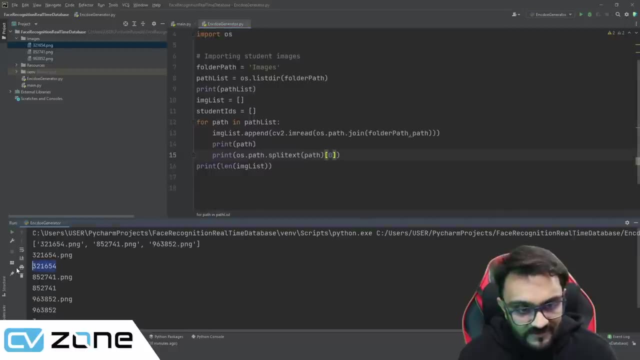 have to put here zero. so that is the first element. the zero is the first element, right? so if we want to split it up into two parts- one with the id and the other one is dot png- we run this now. now you are getting the exact value: three, two, one, six, five, four. so we have. 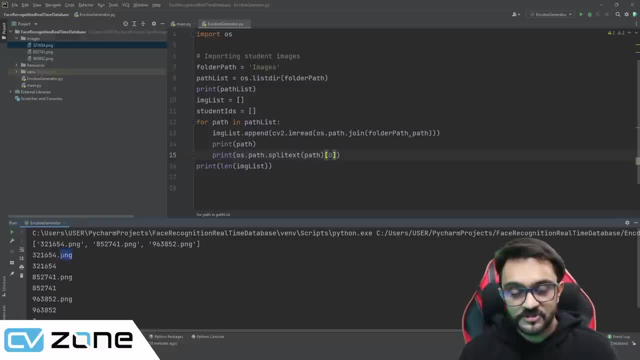 removed the dot and we have removed the dot png. the reason we are doing this and we are not just saying get the first six letters, is because the numbers can change. it might have three digits, it might have 10, so this is the correct way to do it. so now that we have this, all we have to do is we: 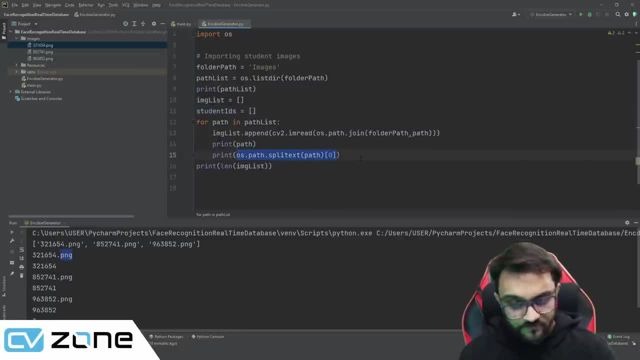 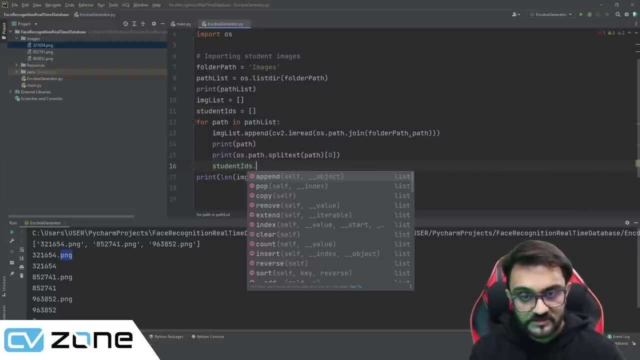 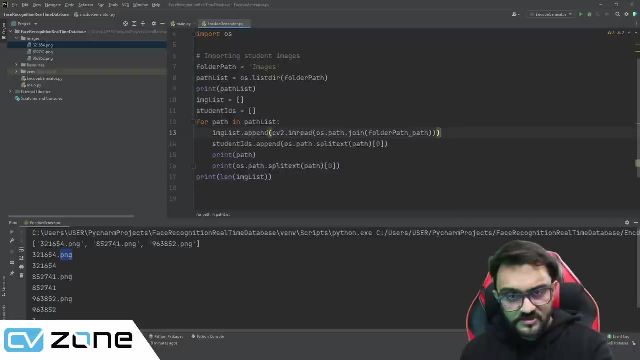 have to put it in student ids. so we are going to copy this and we are going to write here: uh, what is it? student ids? uh, student ids, dot append. and we are going to append all of this so we can remove this. we can paste it here. uh, just for your reference, i will keep it and i will comment it. 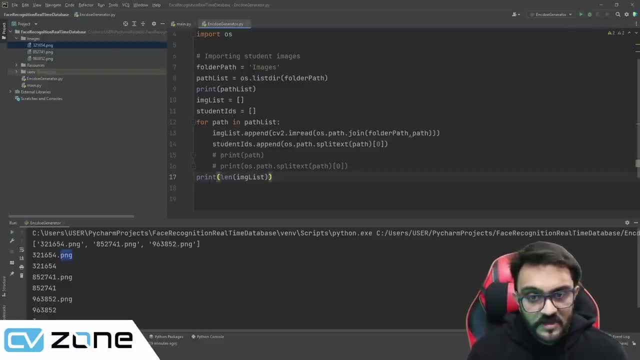 if you wanted to see, you can see it as well. so again, we are going to check, uh, the student ids if they are important correctly. actually we can print the whole id thing so we can write here student ids and let's see if it is imported correctly. so here you can see it's extracted properly and we are getting. 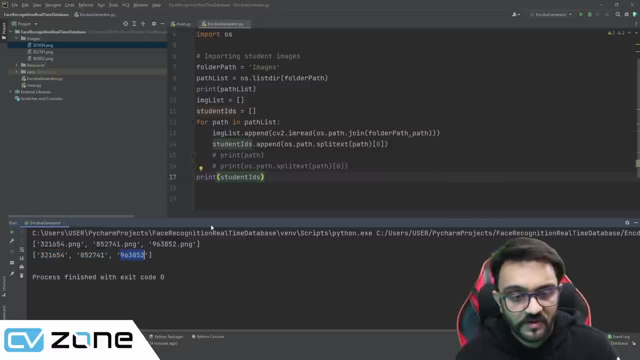 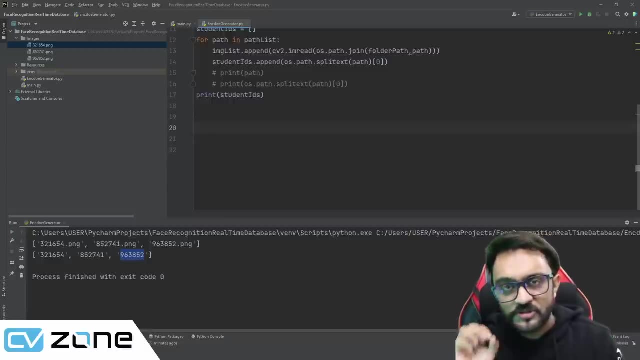 the names or the ids of our students. so now to run the encodings, to create the encodings, we are going to create a function, so we are going to send in the list in this function and this function will generate all the encodings and split out. 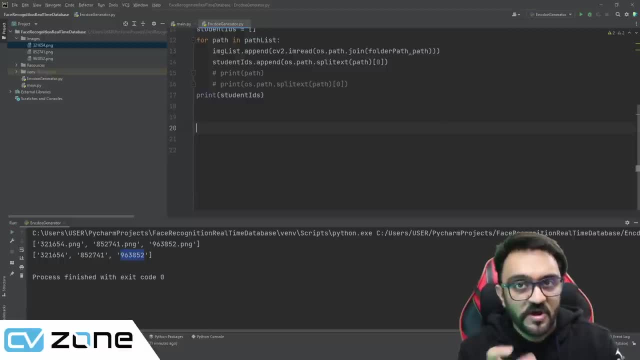 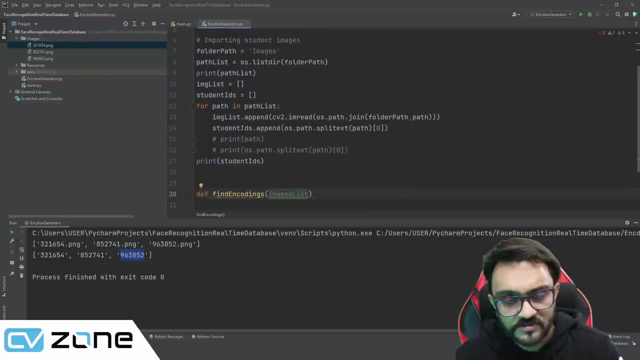 or split out a list with all the encodings. so we are going to write here find and go codings and we are going to give in the images. so ima, images list. let's see, or did we name it? yeah, it's already there, image list. so we will just call it a little bit bigger, a little bit different. so images list and. 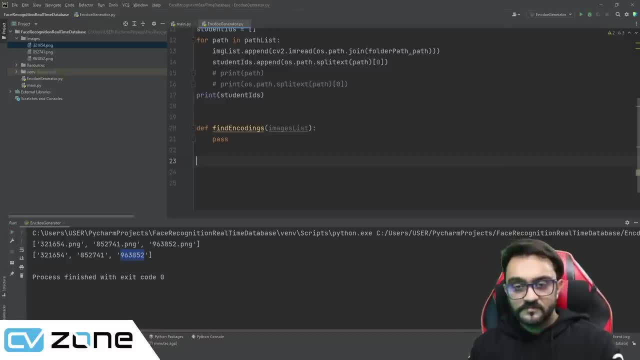 we are going to write here: pass and we are going to write here: pass. so what exactly are we going to do? we are going to loop through all the images and we are going to encode every single image. so we will say for image in image, images list. 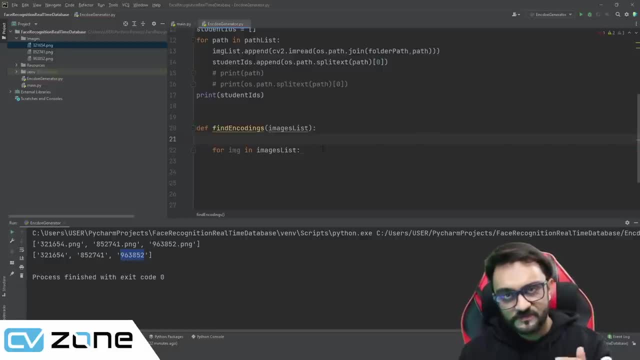 first of all we we have a few steps: how to encode. the first step is to change the color, so the color space, just to make sure we are going from bgr to rgb, because that is what the library uses. so opencv uses bgr, the face recognition library uses rgb. so we have to convert. 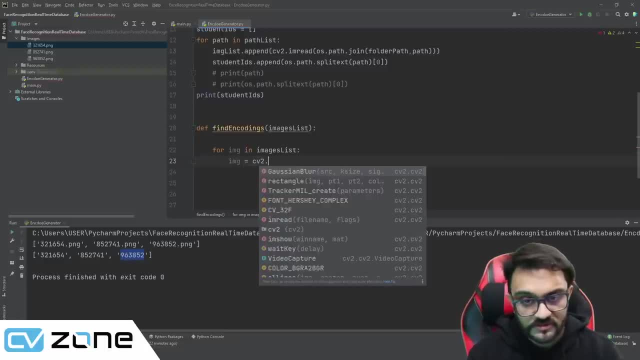 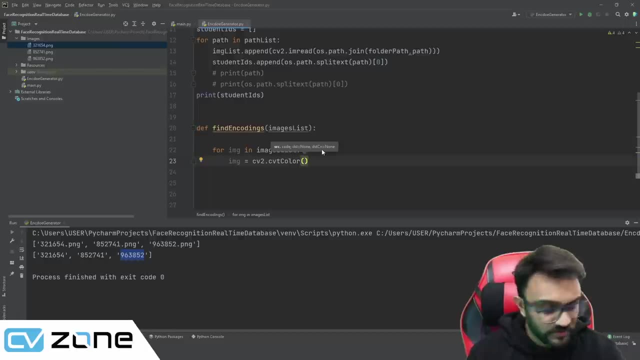 it. so we write here: image equals cv2 dot color: cv t color. and we are going to write image and cv2 dot. cv2.color underscore bgr2 to rgb. there we go. so now the first step is done, we have converted it. the second step is to find the encodings. so we will write here: encode equals face recognition. 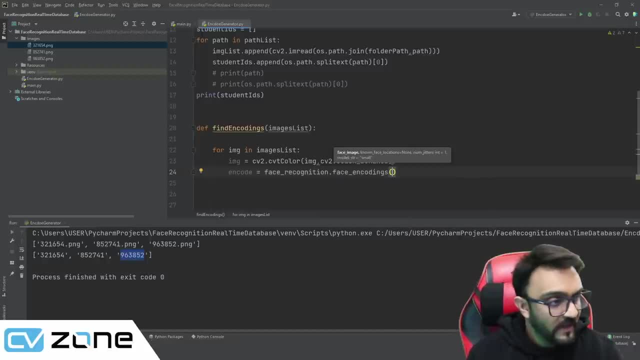 dot face encodings, and then we are going to give in the image and we are going to get the first element of this. so this is how exactly you can find the encodings of that image. now, once we have that, what we have to do is we have to put it in a list. so we will write here: encoding- encode list. 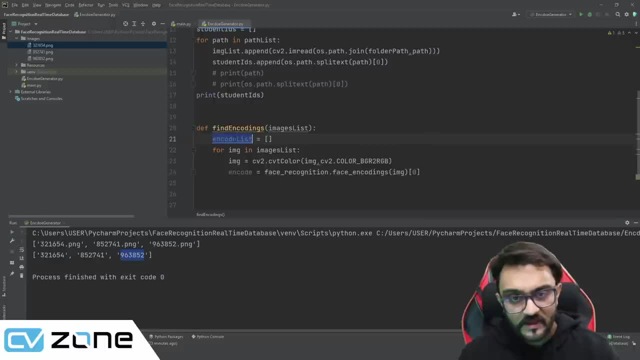 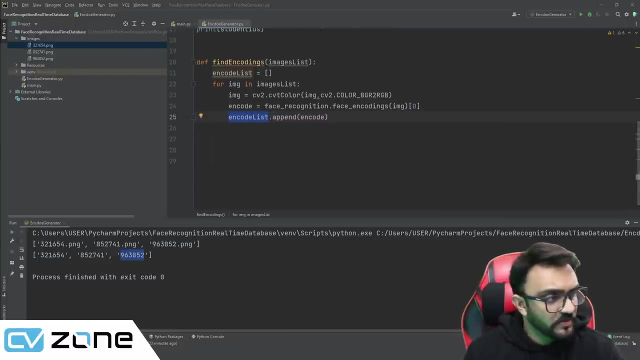 equals empty, and we are going to write encode: list dot. append encode. so it will loop all, or loop through all of these images and it is going to save it. you now, once we have that, uh, what we will do is we will return this. we are going to write here: 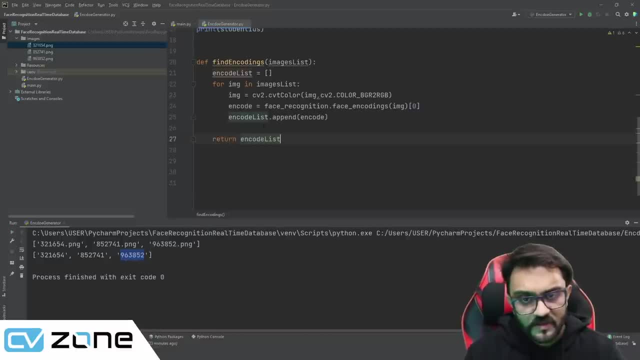 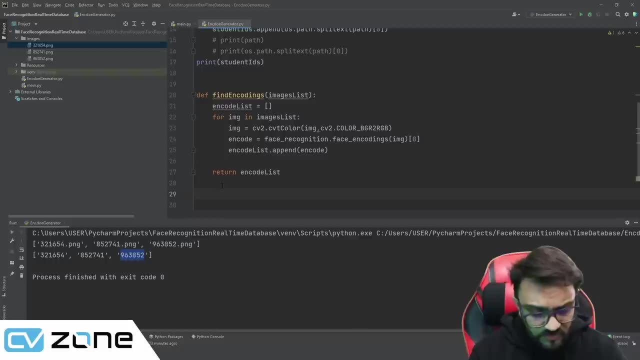 return encode list and that will generate all of our encodings. so here let's call this function. so we are going to write encode list known, so all the known faces equals find encodings for all the image list. so this will generate the image list and it will 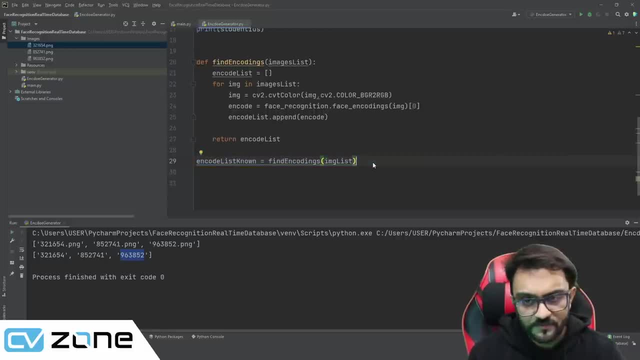 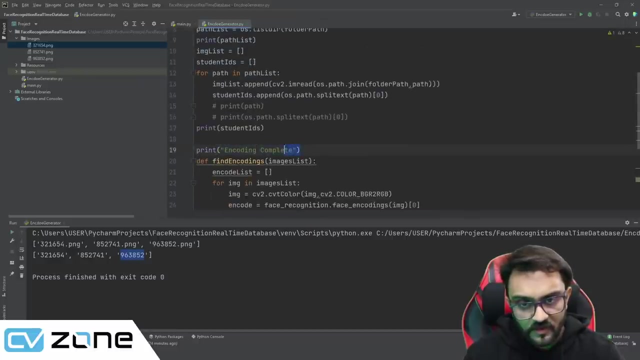 save it here and then we can simply write here: print encoding complete, and above we can write here: uh, above that, sorry, above, here we can write: encoding started, dot, dot, dots. so here the encoding has started, here it will generate and then encoding has completed. so if there's a lot of images, this will take a while, so it's better to show it like this: 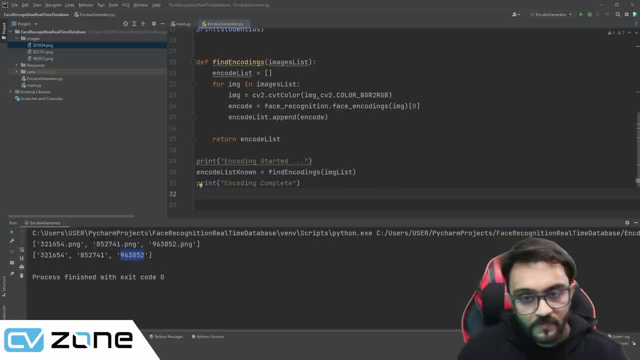 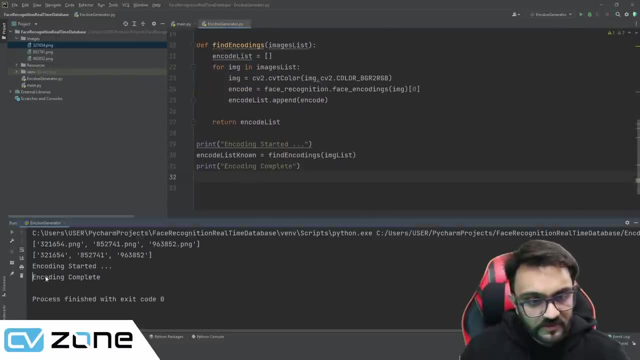 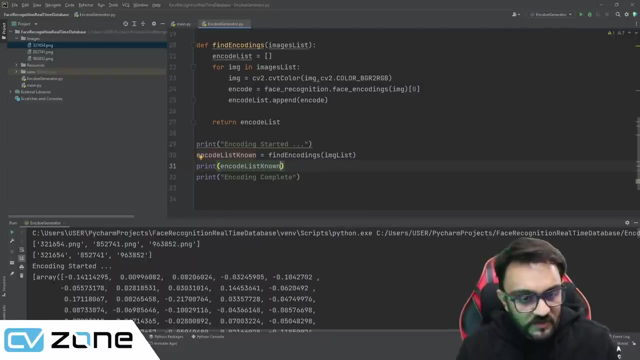 okay, so that's the idea. let's plate and let's see if it works. encoding started, encoding complete, so that's very good. we can actually print out the encode list known just to see what exactly does it output. so there you go. we have some values here that we can see. we have an array of all these. 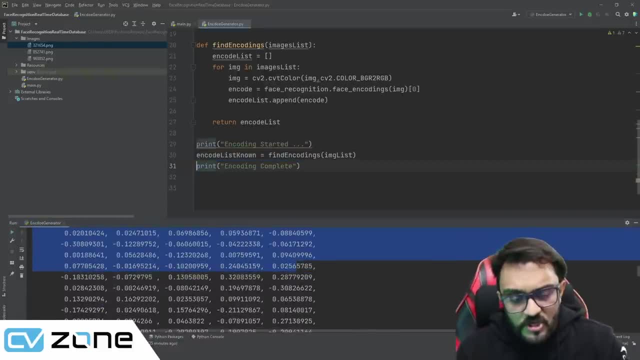 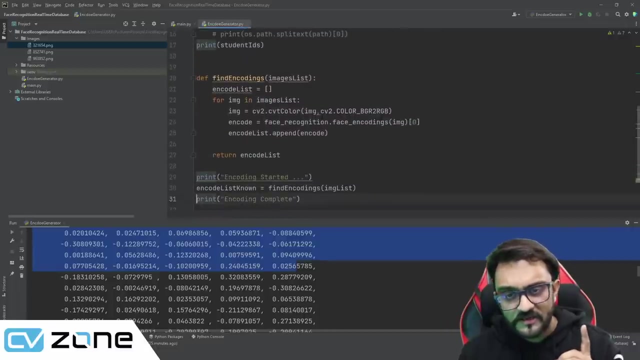 different values. so that's good, so it means it's working. so what's the next step now? we need to save it in a file. we need to save it in a pickle file so that we can import it when we are using the webcam. so, um, but when we are saving it in a file, we need to save two things. one is the encodings. 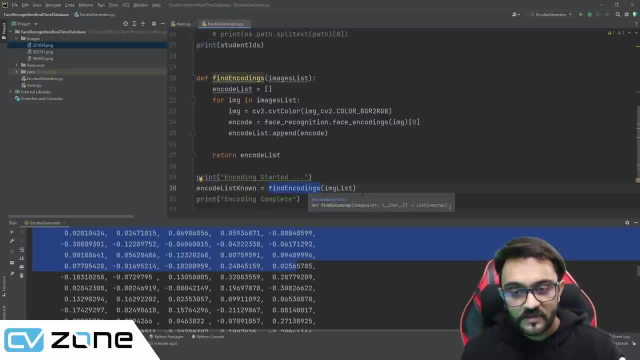 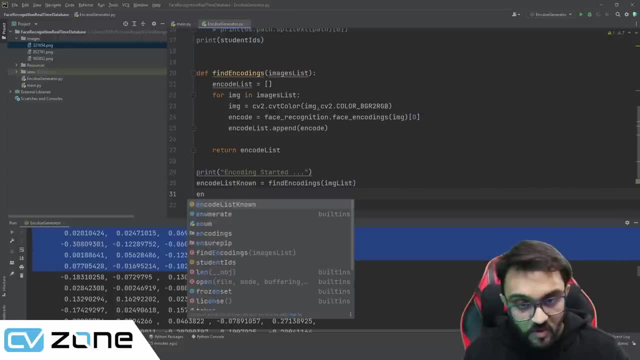 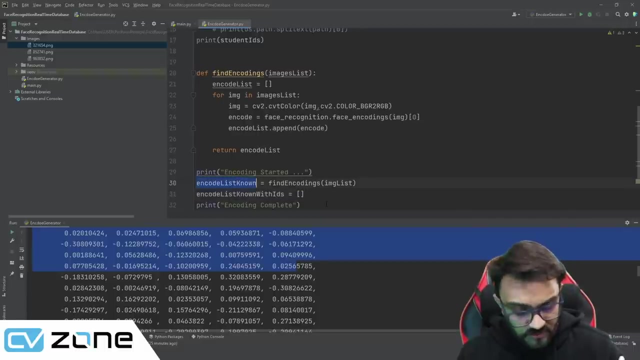 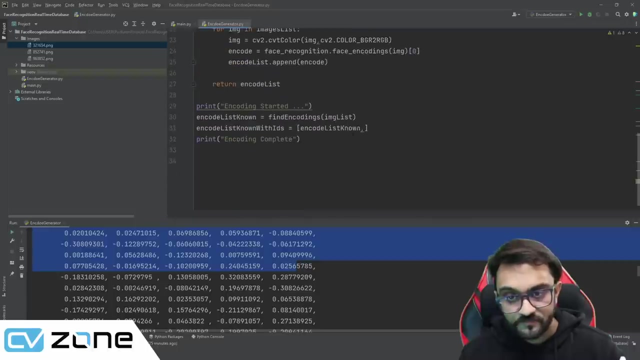 and the other is the names or the ids. so which id belongs to which encoding right. so we need to tell that. so we will write here: encoding list known with ids equals. we are going to put encode list known and then we are going to put so, uh, student ids. so these are the two lists that we need to store it, uh, in our file. so we are going. 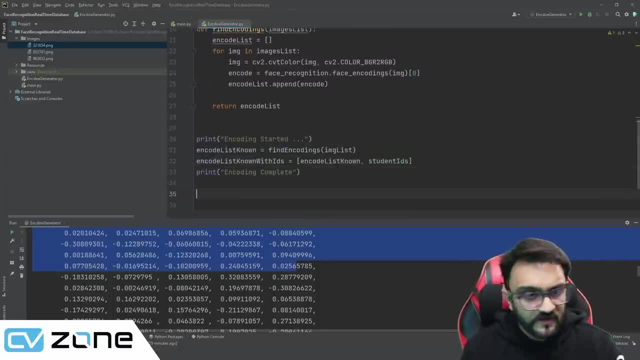 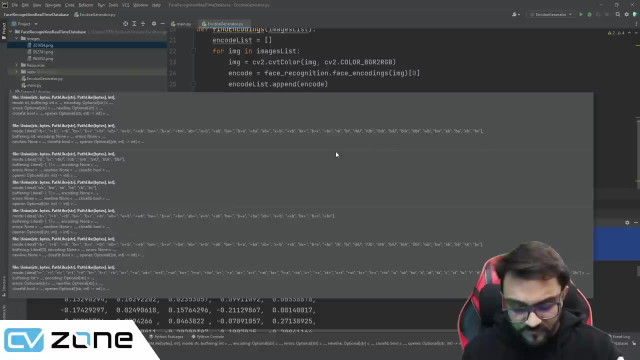 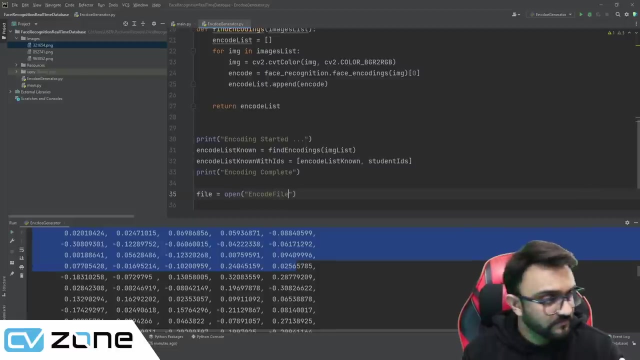 to generate this pickle file. so how can we do that? it's very simple. you have to write file equals open, and then you have to give in the file name so we can write anything. let's write: encode, uh. encode file, dot p, and then we have to give in some. 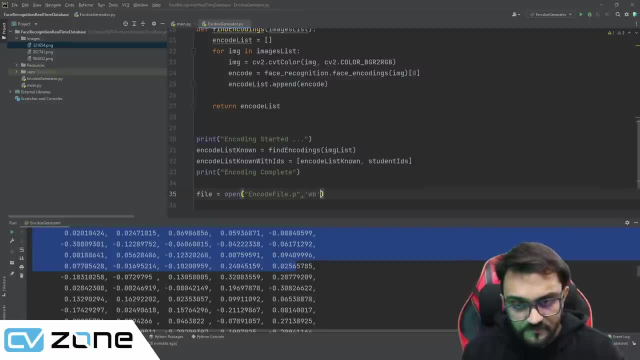 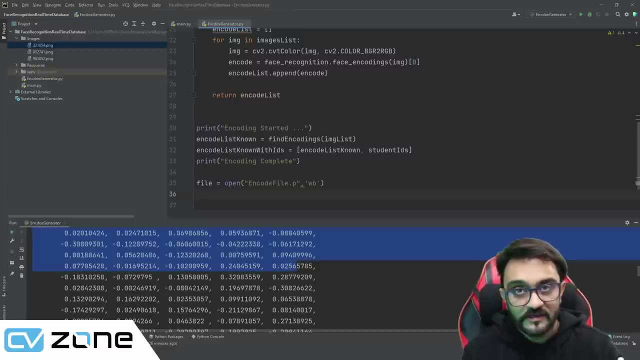 permissions. so we are going to write w b and then we have to send in or dump the lists in this file. so we will write here: pickle dot dump and we are going to dump encode list known with ids and we are going to dump it in our file. then we simply can close. so we'll write here: file dot close. 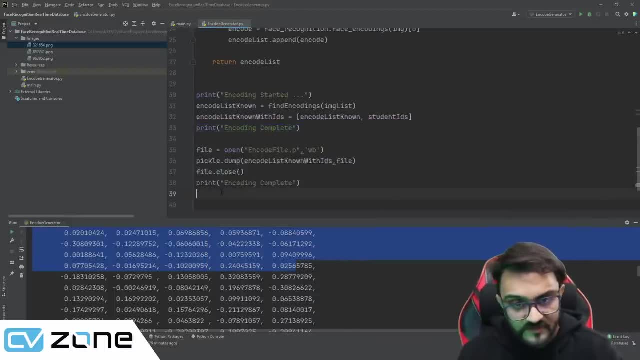 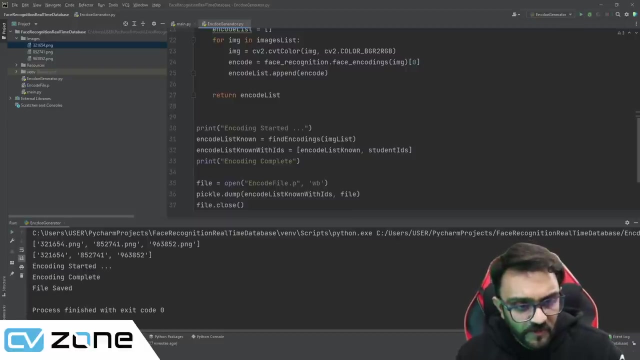 and we are going to write file saved, file saved. so that's the idea. let's see if that works. there you go: encoding started encoding complete file saved. so if we look at our directory you can see we have encode file dot p. so this is the basic idea behind encoding. now we have. 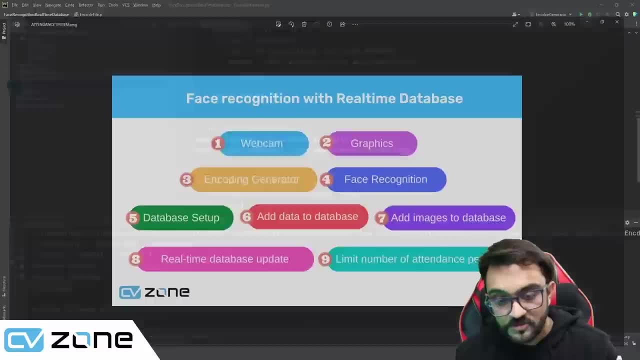 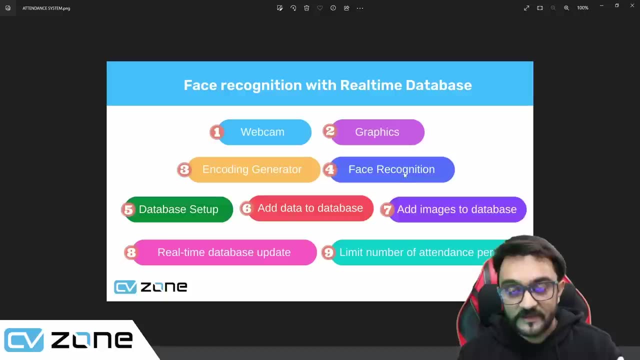 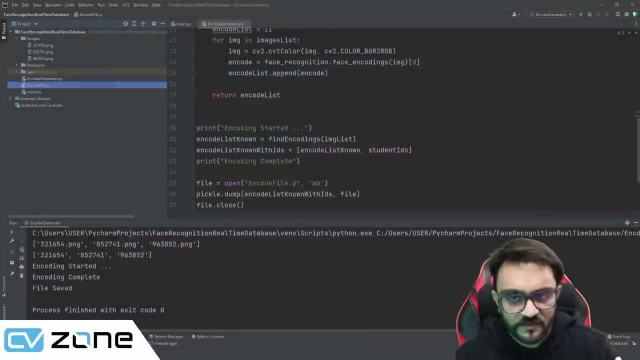 extracted all the encodings and now we will go into the face recognition part. so in the face recognition we are going to take these encodings and then we are going to apply it to see whether we are detecting any faces that are known or not. so how can we do that? it's very simple, it's very 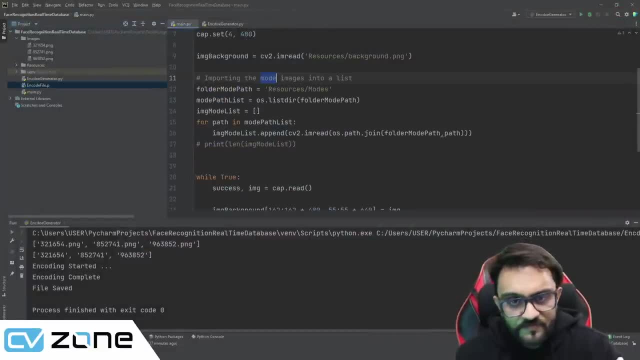 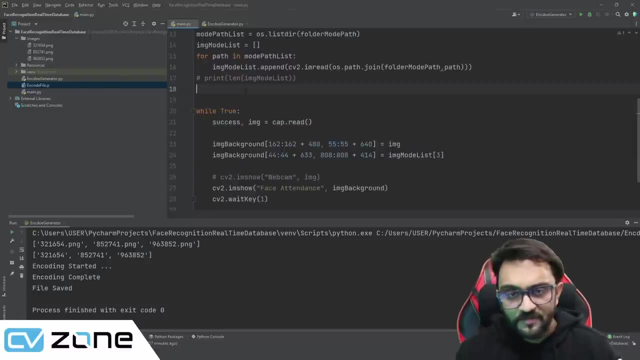 easy to follow. so let's go ahead to our main file and we are going to go to our encode file and then we are going to import it here. so here, after importing more images, we have the while loop and before the while loop we are going to write: import the encoding and coding file. 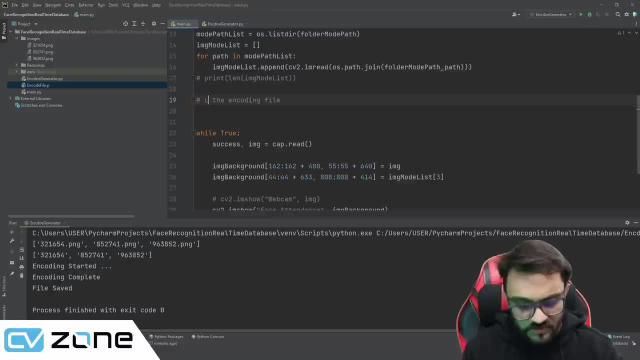 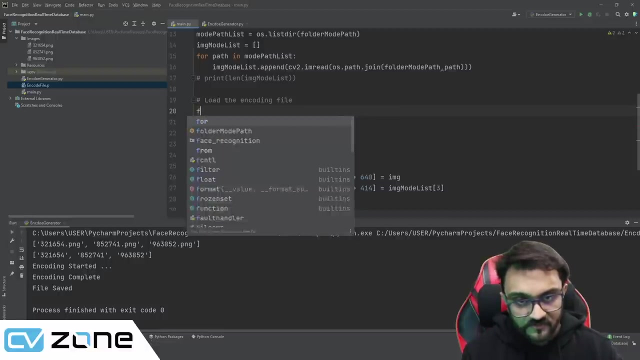 or let's- let's not call it import, let's call it load- load the encoding file. so the loading part is pretty much similar to the encoding file. so let's go ahead and import the encoding file. so first of all we have to open the file. so we will write in умon file. so first of all we have to. 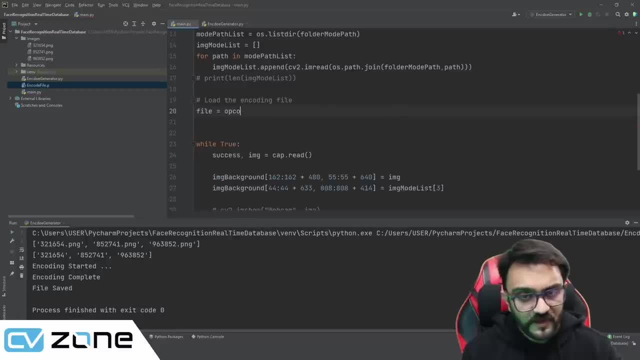 write file equals open. which file do we want to open? we have to give in the name, so here we will write and code: file dot p. and then we have to give in some permissions again, so we will write our B, so this is for reading. and then we are going to write encode, encode in encode. so that's actually. our main file and then check and if we have, if we have any code here, it will say: include erased ecg s nossas, the file, dot file, such that if you look, we have our tag. Second, clear was our icon and we will save this process at the way we want, and then this is all done. so see how that is. 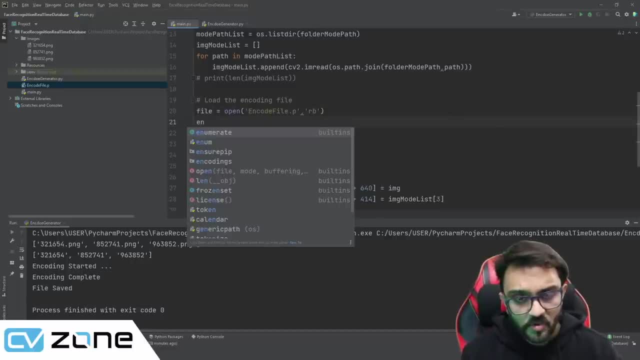 exciting. first we both have our profile fill in, so we have the file and after this we will write the diagram. we see the number of thewearlist on our site. we will say requesting that we and code lists with IDs. did we write the same name and code list known with IDs? 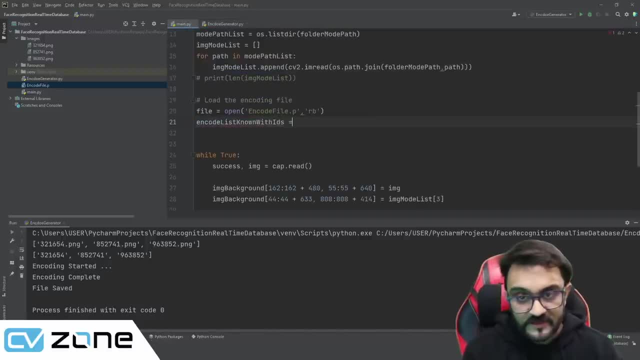 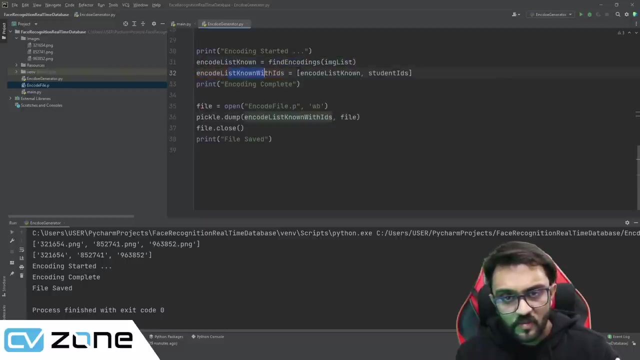 so let's just copy that and code list known with IDs equals pickle dots load file. so this will add all the what do you call lists, all the information, into this encode list known with IDs. now we need to extract. we need to extract it into two parts. so the way we converted this, we added these two into a single. 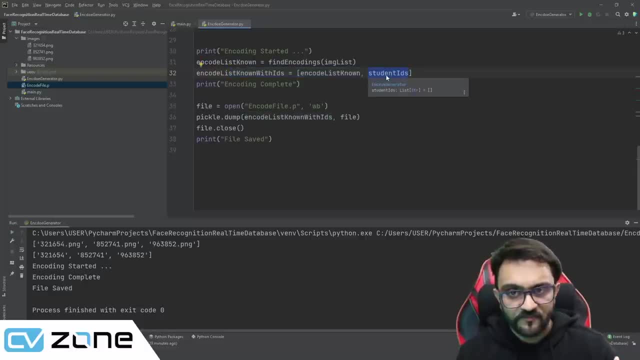 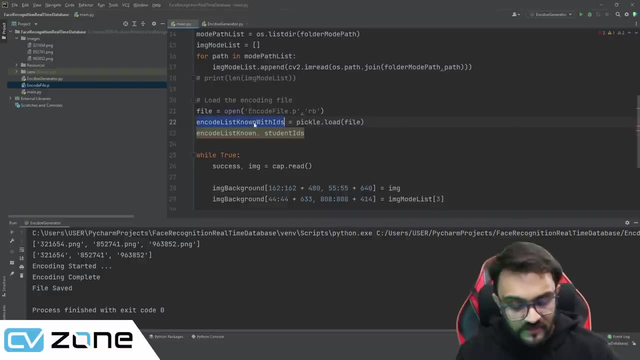 list we right now we have to separate them from the list. so again, we will copy this and code list known and student IDs equals encode list known with IDs. and before we do that we can simply close this. so we can write here: file dot. close. there you go. so. 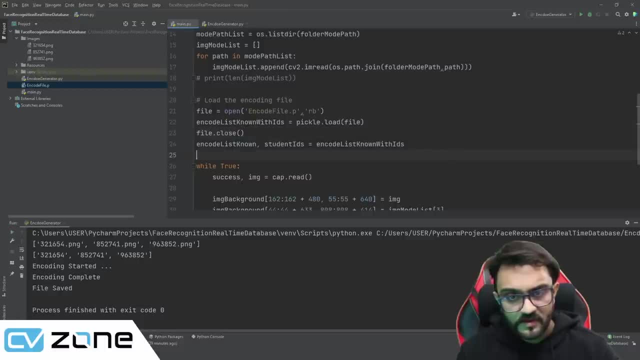 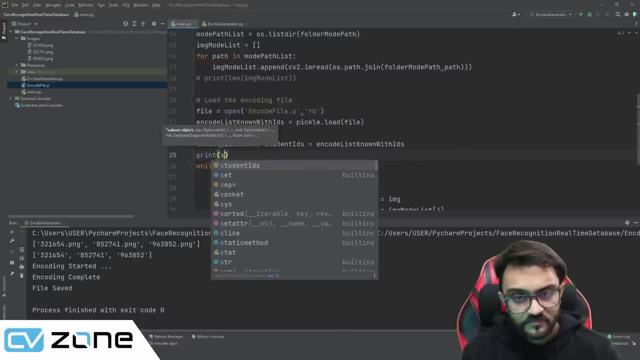 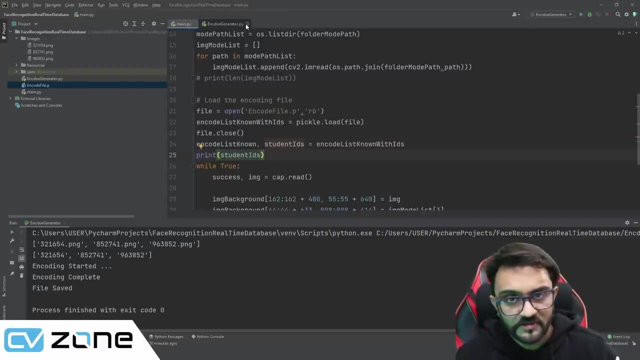 that's the basic idea behind this. so let's run this and see if it prints. prints student IDs. let's see if we have extracting the correct. we are running code generator. we need to run main again, so let's run that. there you go. so now we have the three IDs of all the students. so that's good. 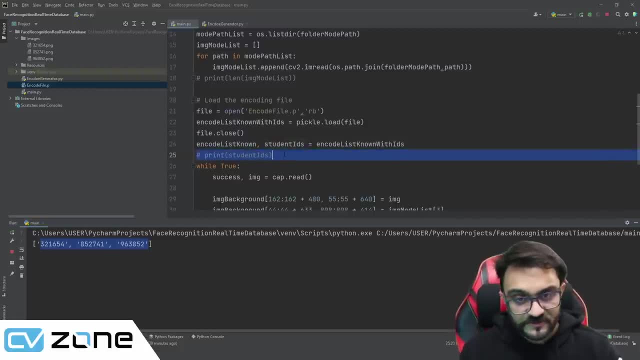 and it means it's working. so I will keep this here just for testing. so if you wanted to, you can test and we can also add something like this: we can add negative color and I need to understand its loading, let's say loading encoded file and code file and core file loaded. there you go, so just 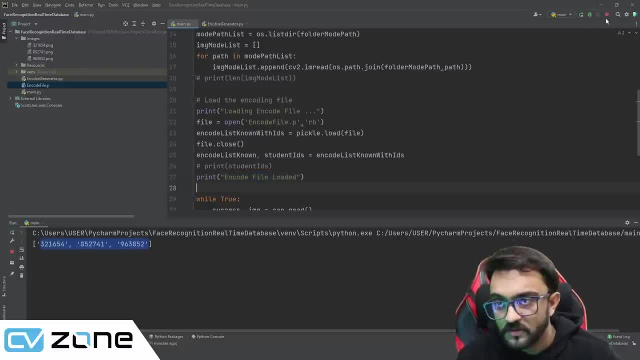 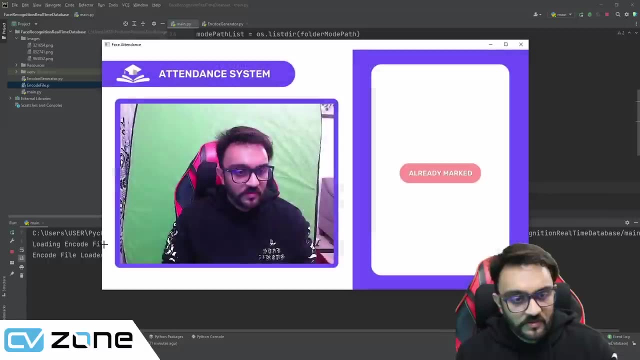 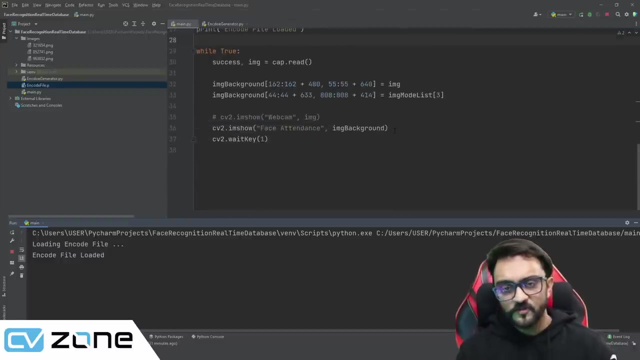 just just to make it a little bit more more interactive. so here it will say: loading encoding file: encoded encode file loaded. there you go. now what we have to do: we have to take these encodings and we have to check in with the new faces whether any of these match or not. so this is very simple. it might seem a bit complicated. 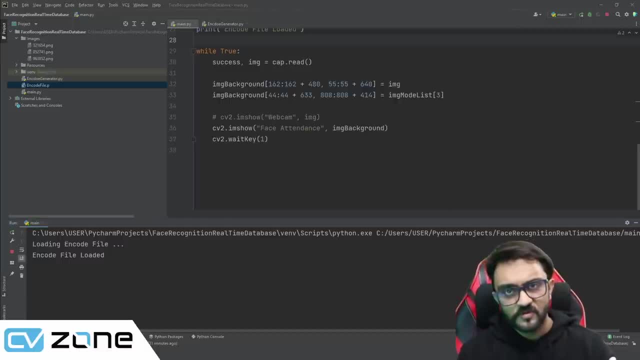 but actually, in reality, it's very simple. all we have to do is we have to write a few lines of code, so let's go ahead and do that. so the first thing we have to do is we have to, uh, make our image a bit smaller, because it takes a lot of computation power, so we will squeeze it down, we will scale it. 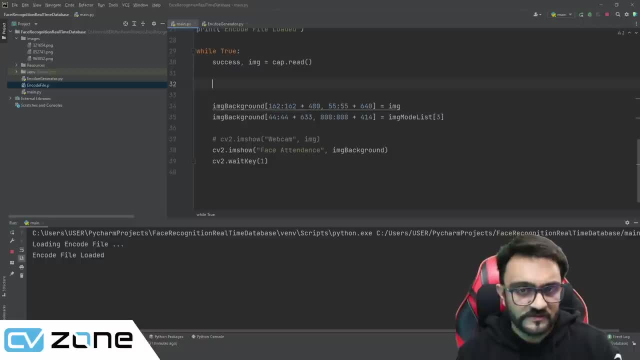 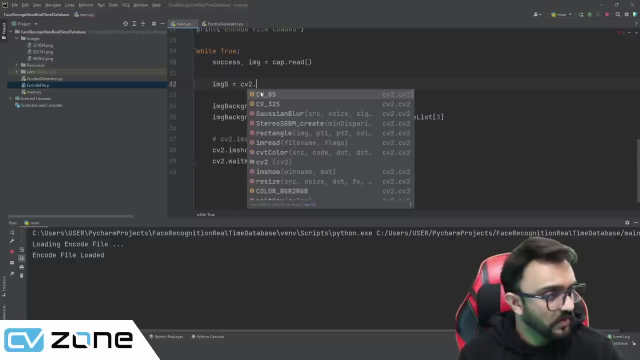 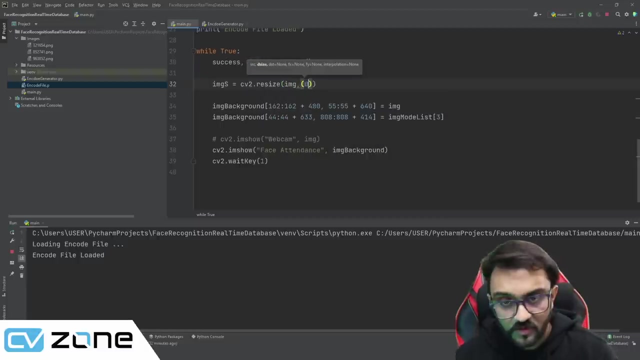 down to, uh, one fourth of the size. so here we are going to write that our image small cv2 dot, what was it size? and we are going to resize our image and we are not going to give in any actual numbers. what we are going to give in are the scale values, so not the pixel values. we are 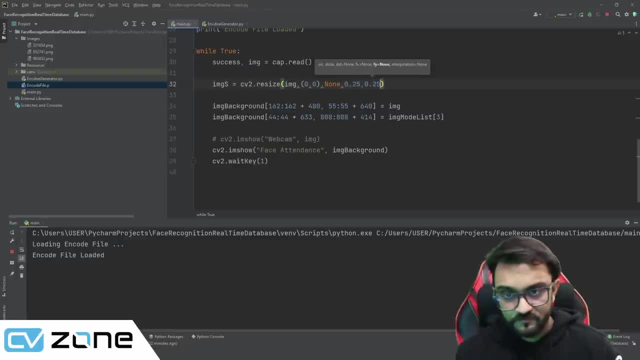 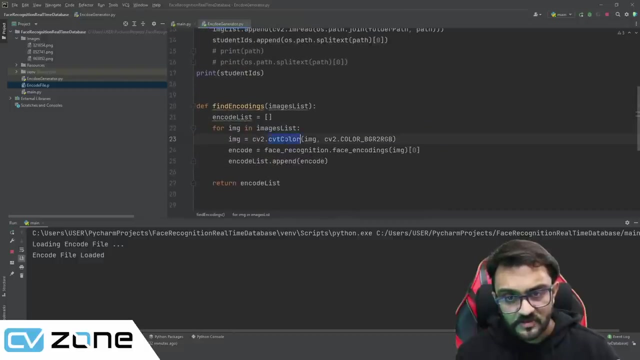 going to give in the scale value, so 0.25 and 0.25. so this is the smaller image. and again, if you remember, we have to convert it into rgb from bgr. so here we can just simply copy and paste. so where was it so cvt color? you can copy that and paste it here and we will write image: small equals. 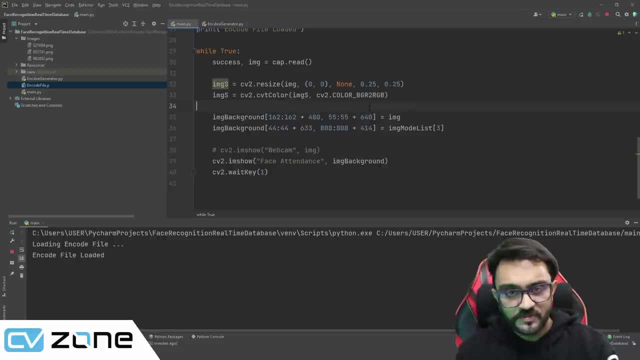 this image small, so bgr2, rgb. so this, this step is very important- of conversion, otherwise it will not work properly. so once we have done that, now we need to feed in the value to our face recognition system. it will detect and then it will give us some output. so we need two things. the first one is the 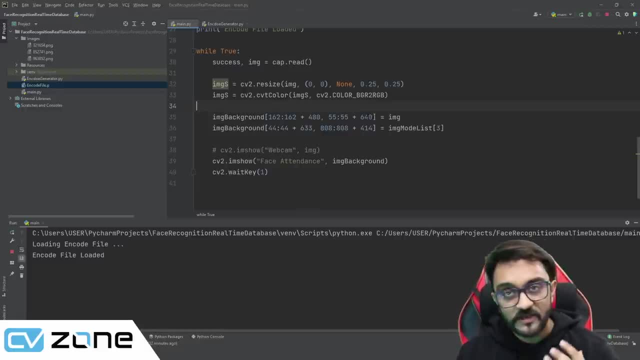 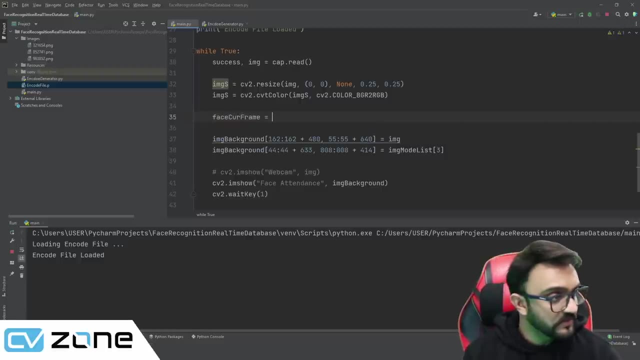 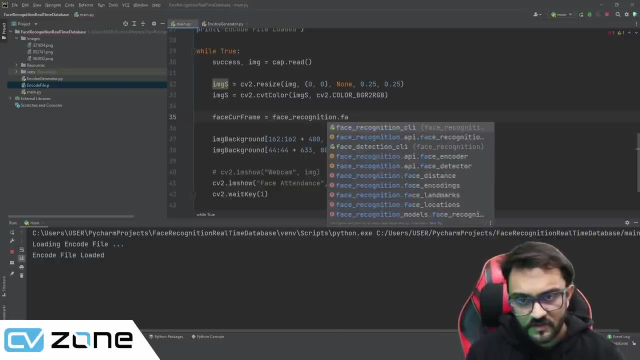 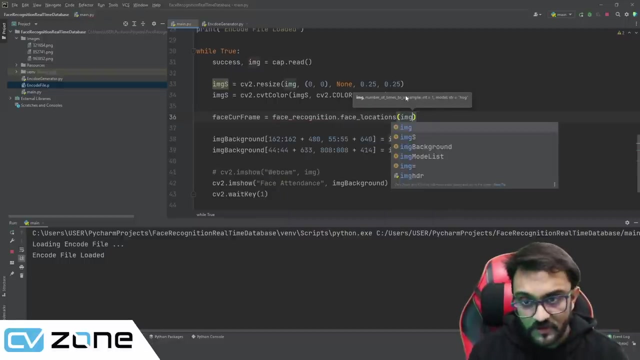 faces in the current frame and the second one is the encodings in the current frame. so here we are going to write face: current frame equals face recognition dot. face locations, face recognition dot. why is it not showing dot. face, hello locations. yeah, there you go, and we will give in our image small, and then, once we have the location of our images we need to. 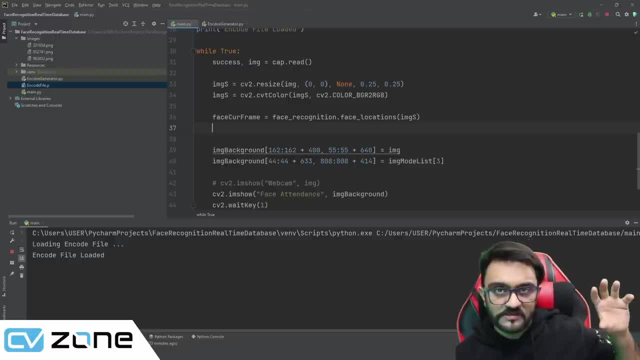 find their encodings. so we have the previous encodings of our known faces. we need to find the encodings of the new ones and then we will compare. so this is for the new ones. so we will write here and code: uh, encode current frame equal. and we will write here: face recognition. 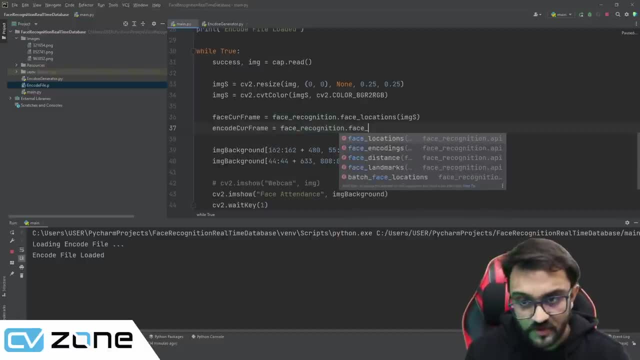 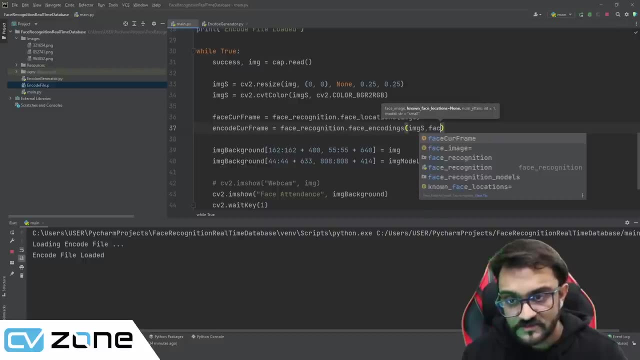 dot face underscore encodings and we will give in the image small and we will give in the face current frame. so these are the locations and these are. this is the image. so go ahead and find, because we don't want to find the encoding of the whole image, we want to find the encoding of the face. so we are. 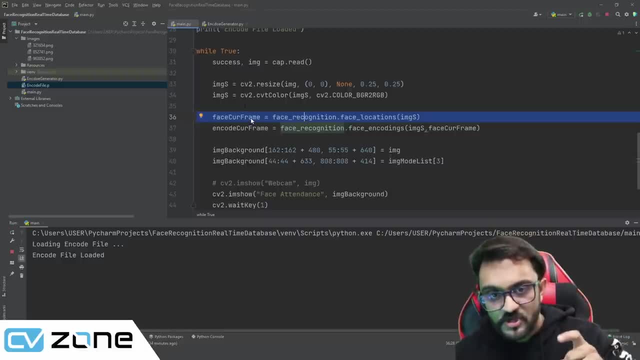 giving the location of the faces and we are telling that this is the image, extract it and find the encodings. so that's the ideal condition of what we are trying to do. so if we want to go back to the ticaacom once we have that, then we can go into the next step, which is actually let's. 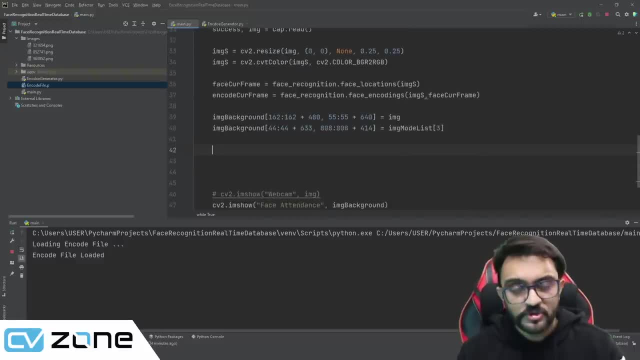 write it below this and we are going to loop through all these encodings and, one by one, we are going to compare it with our generated encodings whether they match or not. so we are going to write for encode face and code face and face location base, lock in and codes current frame and faces current frame. so what? 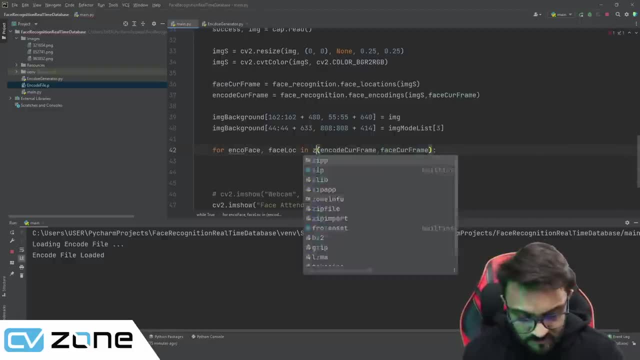 exactly is happening here? we need to write here zip, because we cannot. we cannot unzip using the for loop. we want to use a for loop for both of these lists at the same time, so we have to use the zip method. otherwise we have to unzip the for loop and then we have to unzip the for loop and then we have to. 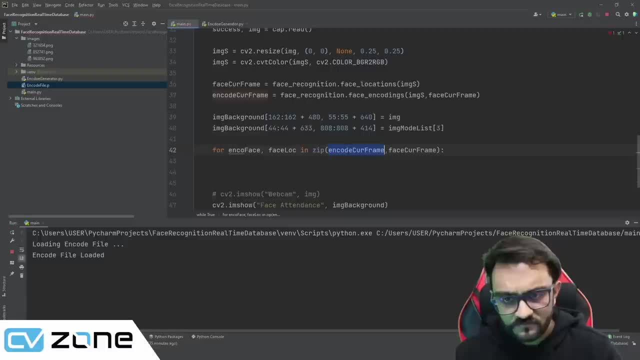 write two different loops separately. so what we can do is we can extract the information one by one. so the extracted information of this will go in this and the extracted information of this will go in this. so that's the basic idea. now we need to find the matches. so matches equals face recognition dot. compare. 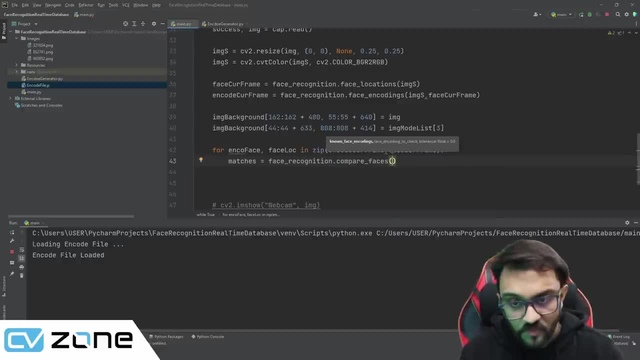 faces and we need to compare it with the encode list known. we are going to compare our current face. our current face is this one. why is this like? encode c, o, d, e- what is wrong with my spellings today? and code face. so we need to write: 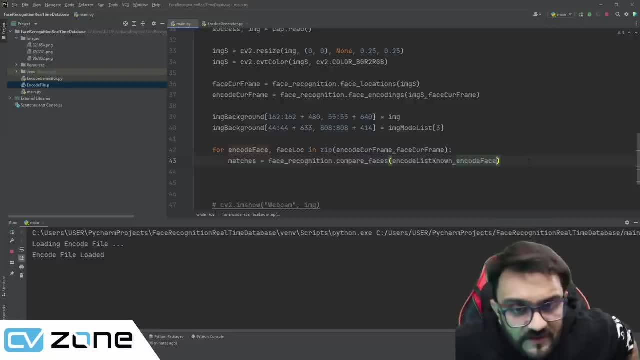 that. and then again for the distance, we can find the face distance as well. uh, the lower the distance, the the better the match. so we will write here: uh, face distance, and here we will write face distance. so again, encoding list node and encode face. now this will give us a list of: uh. actually, let me show you so because i, if i explain it, 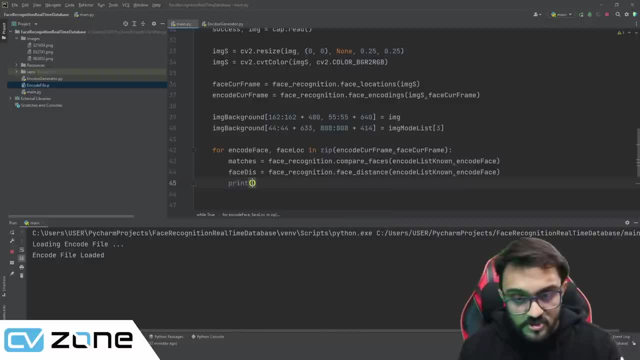 will be complicated. let me just show you what exactly are we getting. so this is matches, and then we will. we will print matches, so let me put this as a string so you can see what is happening. yeah, i was using the wrong key. okay, this is matches and this is face. 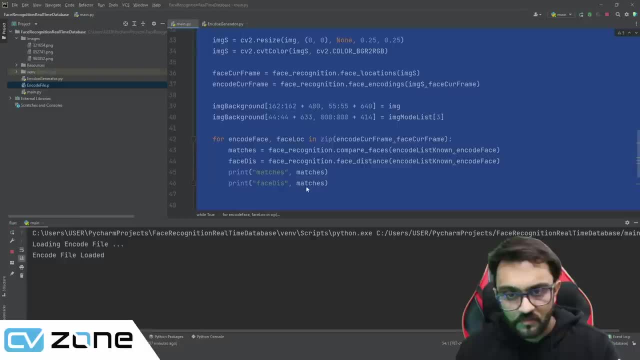 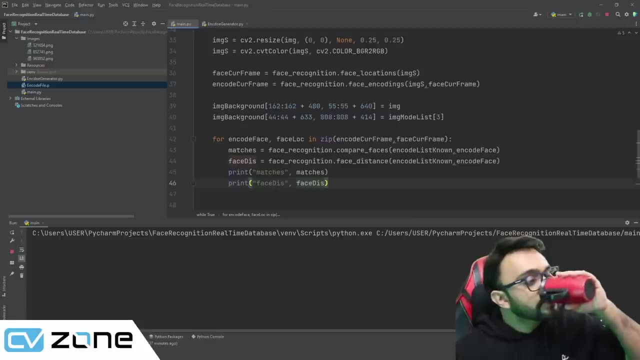 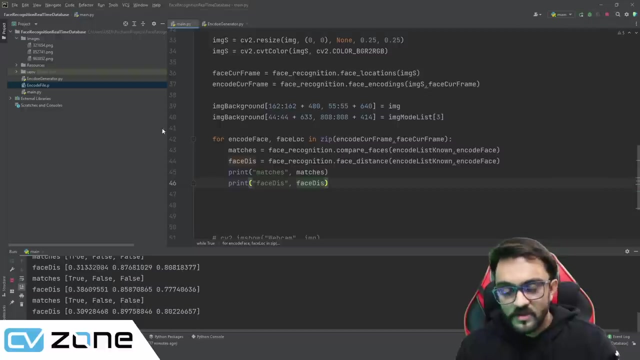 distance, okay, so let's write here face distance. so let's run that. there you go. so now you can see both of them have three, three values, because we have total of three images in the known directory, because our encoding generator generated three images, three encodings, so it will match with all three. so let me just go in the 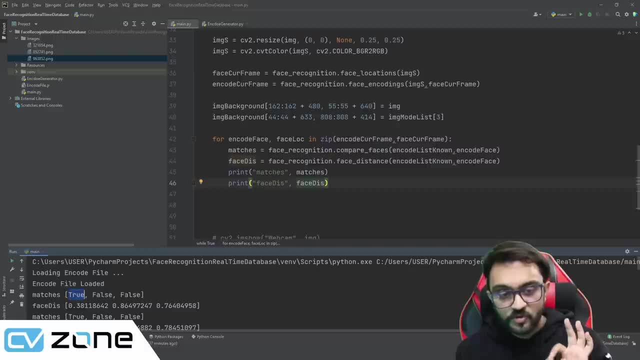 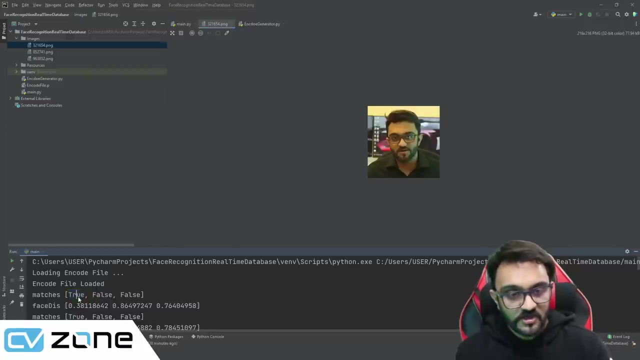 very beginning. so now it will first give you true or false matches, whether my face, the current face from the webcam, matches the first image from the images that were generated. so here it actually matches my face, so that's why it's saying true. it did not match with emily blunt, it did not match with elon musk, so that's why it is giving false. 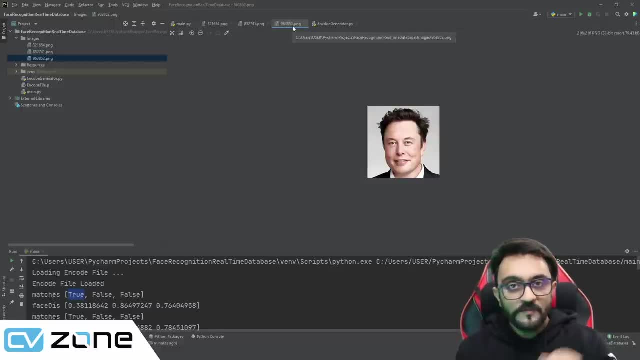 now how good of a match it was will be given by the face distance. so the lower the face distance, the better the matches. so here it's 0.38, here it's 0.38, here it's 0.76. so it is matching with the other faces, but only 0.8, only 0.7, but with my own face. 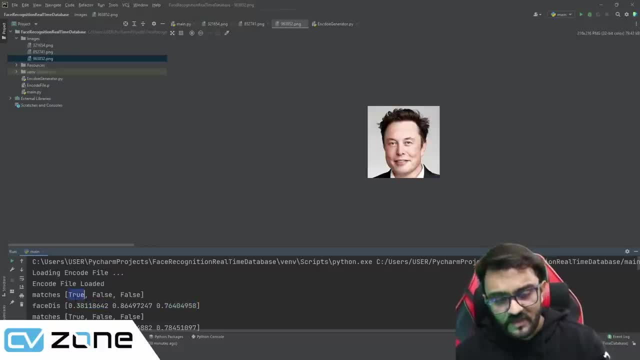 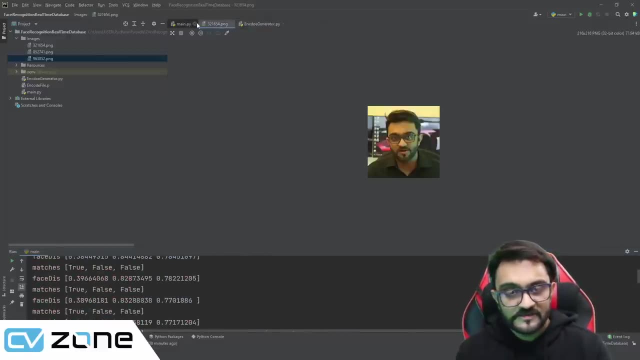 it matches 0.38. so that's why it's giving here true and for the others it's giving false. now, if i bring in the image of, let's say, elon musk, then it will give uh, the second one or the third one. the third one it will give true, because that is the face of elon musk. so let me run that and let 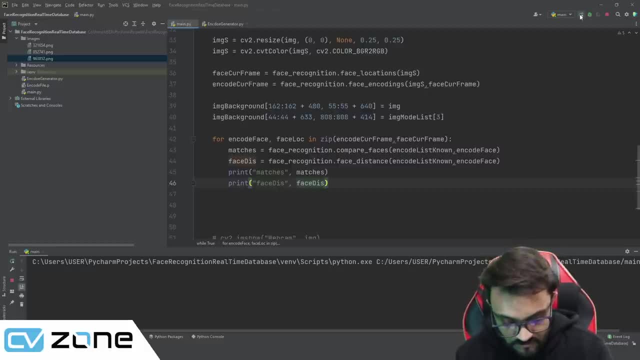 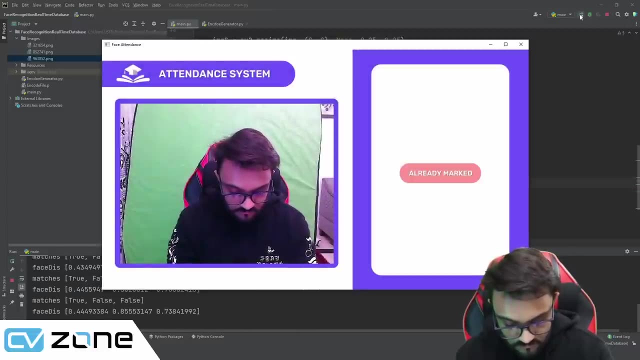 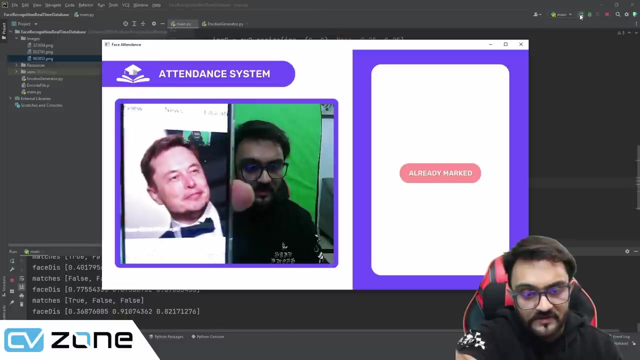 me bring in my phone and i will open an image of elon. uh, let me open elon musk. there you go. oh, it went back. okay, there you go. so here. if you see elon musk now, at the end it is going to say true. 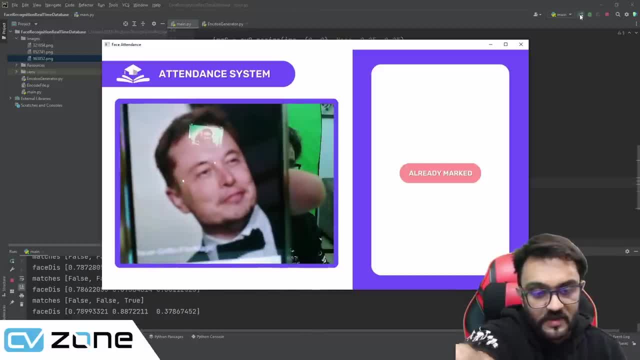 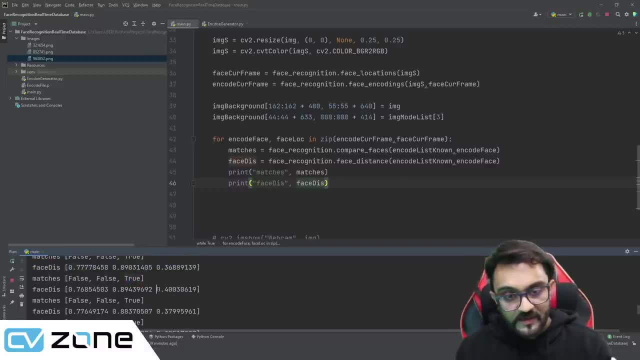 let me push it here. there you go. now it's stable. and the last one you can see here. you saw that it is showing the last one as true and the least value is 0.4, which is of the third one as well. so this means it is matching with elon musk. so that's the main idea. so how can 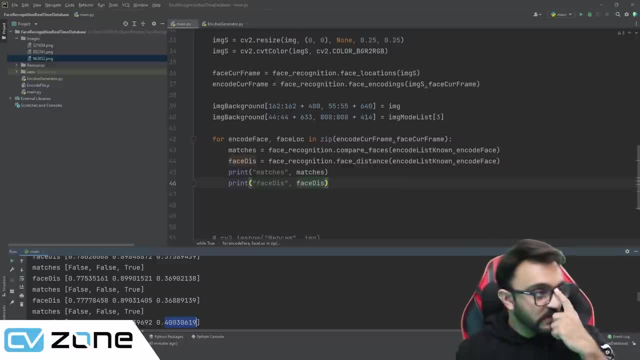 we extract this value and how can we make use of it? so the first thing we will do, we are going to get the index of the least value, the least value. so, whether it is 0.3, 0.8, 0.7, which one of these is the least? 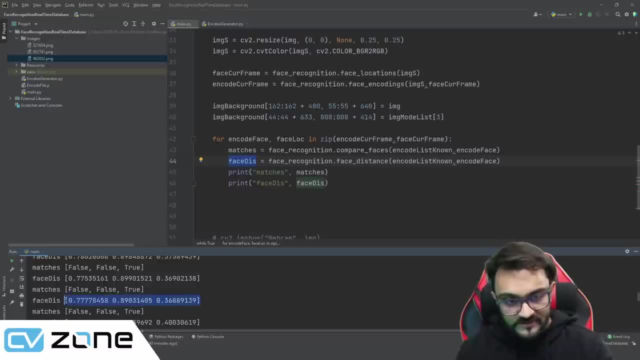 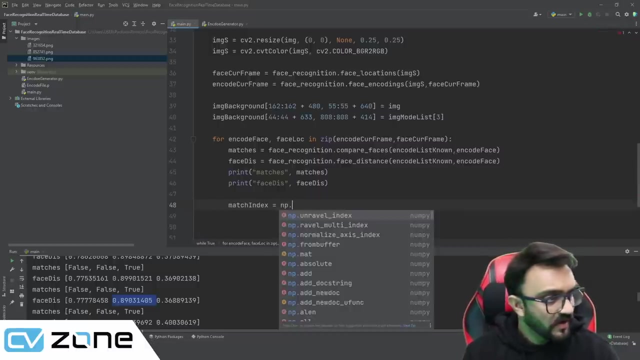 we want the index, which means, for this instance, we would, we would need the value 2, because this is 0, this is 1 and this is 2. so how can we get that information? we will write here: match, index, equals, numpy, dots, arguments, arg, minimum, and then we are going to give in the face distance. 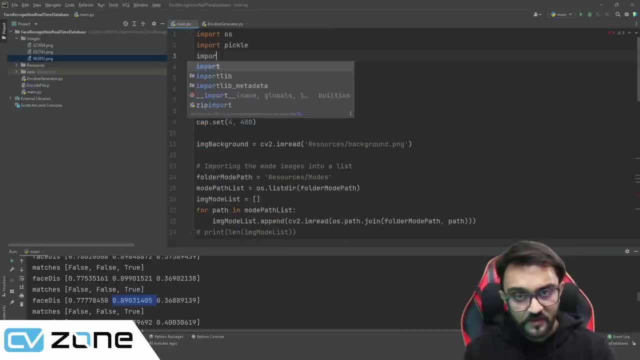 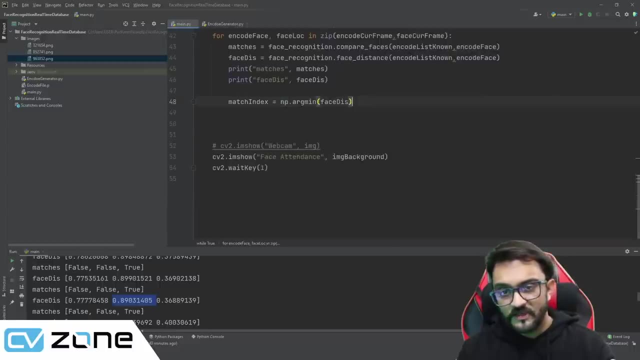 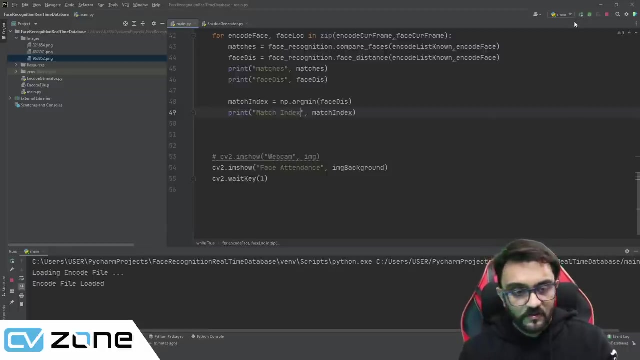 numpy is not imported, so we'll write here import numpy as np. there you go. so now it will give us the value index value. let me print that out. so here we will write match index and we will write here match index. in my case it should give 0. there you go. so match index is 0 because it's detecting my face. 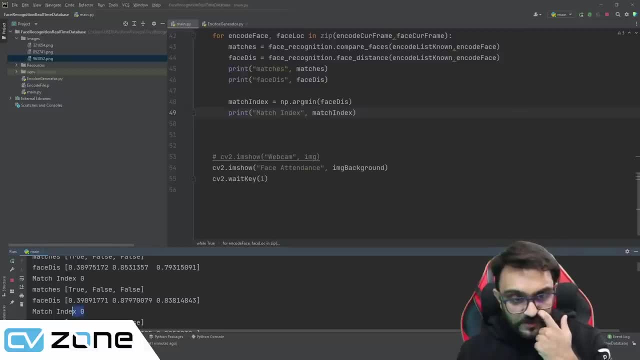 and my face is the first one. so it is giving the value of 0 and this is the least value. now, once we get the 0 value, we will write match index. we are going to check it, uh, in the matches list. if that value is true, we will say face detected. 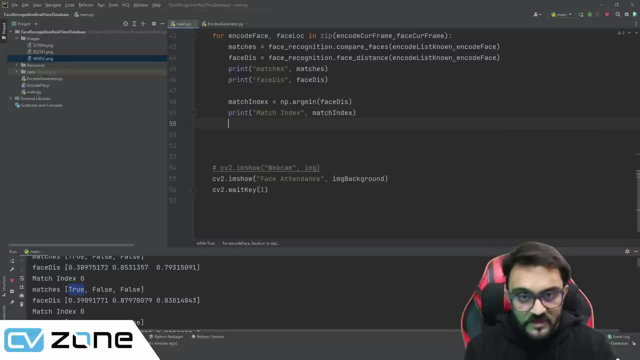 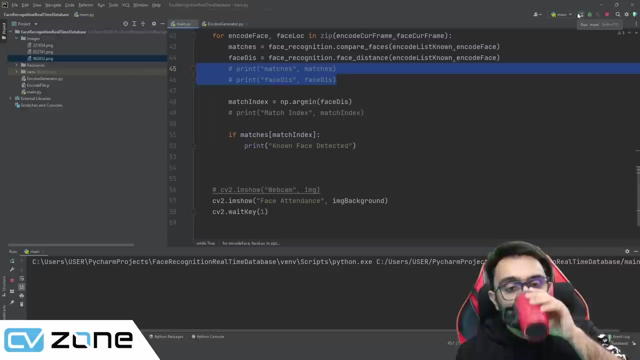 the correct face is detected. so that is our criteria. so how can we say that we can say: if matches at match index is true, then we will print a face. let's write known face, detected data set. there we go. so let's remove these so that it's not confusing. 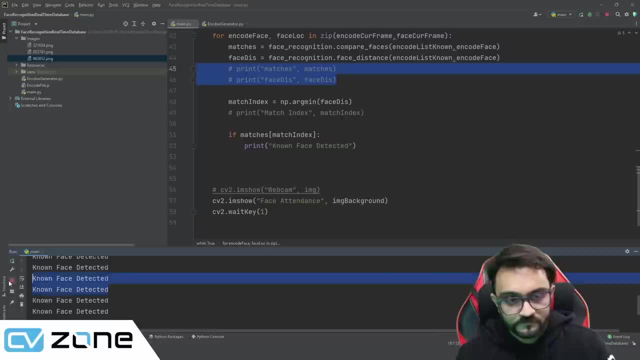 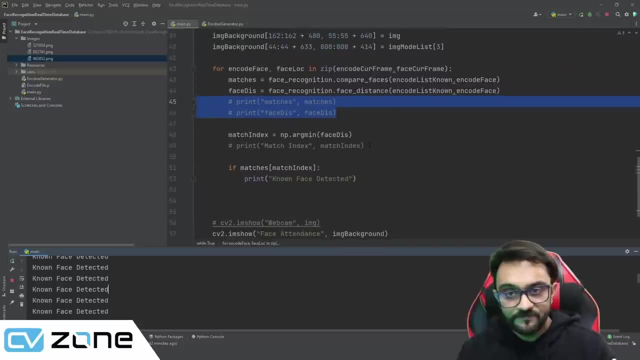 and then so it is saying: known face was detected. that's the idea, and to make sure that we are getting the correct one, what we can do is we can print out the id of this one so that, um, we do a, we have the correct information of which one was working, so for which one was detected. 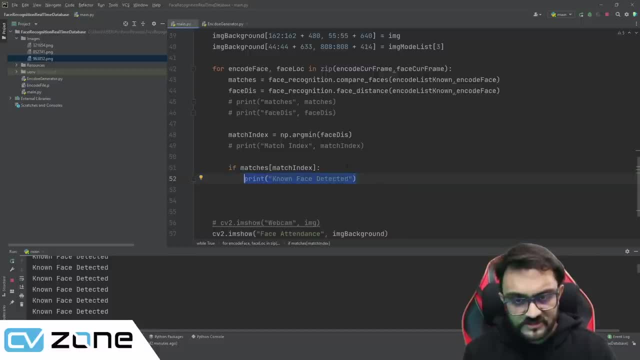 so here what we can do is from the list. what was the list name? it was student ids, so student ids at match index. so we can print that. there you go. so three, two, one, six, five, four. three, two, one, six, five, four is the correct id. that was. 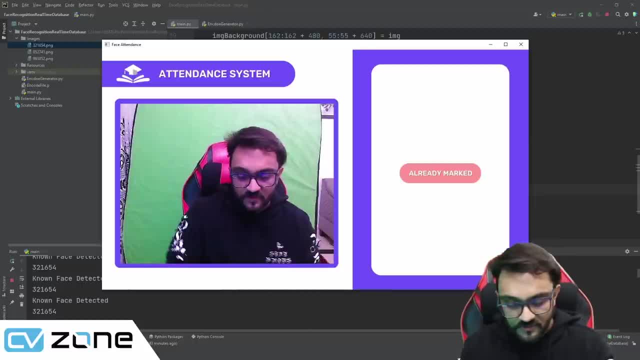 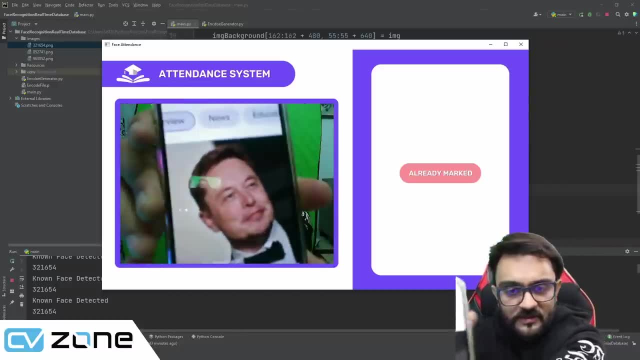 detected. uh, let's check for elon, or let's check for emily blunt. actually elon is already open, so let's check his. so there you go, and let me bring down the value so we can see. so here it's showing nine, six, three, eight. 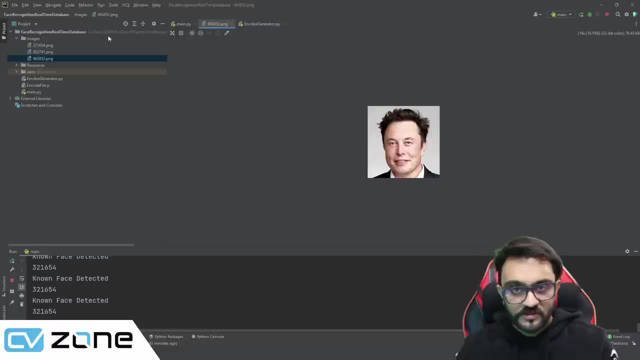 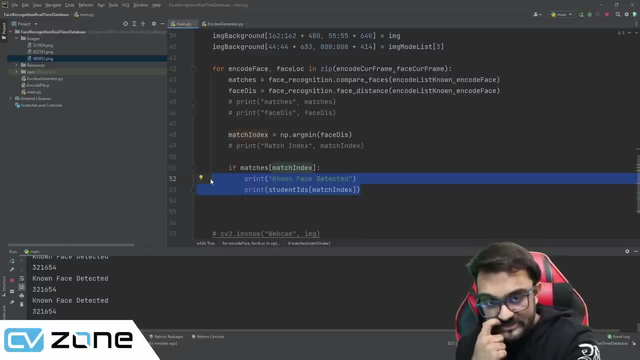 s two. so here nine, six, three, eight, five, two is elon, so that is correct. now this is a a little bit weird, that what we are doing, so what we can do instead is we can actually show the face and show the name so that it looks a little bit better. so we have printed this out. 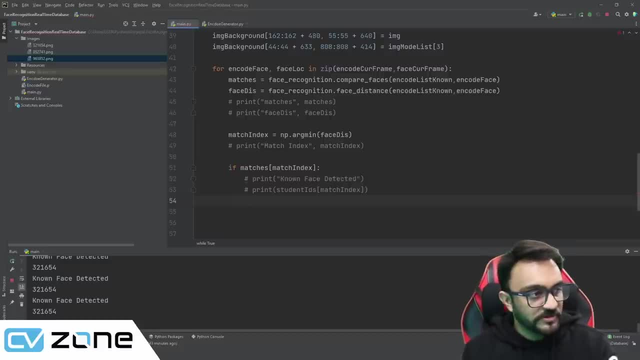 we have comment the commented this out, and what we are going to do next is we are going to draw the rectangle around the face. so, at least we know it, something is being detected now, uh, what we can do is we can use the normal rectangle, uh, provided by opencv, or we can use cv zone. so the cv zone rectangle is a little bit. 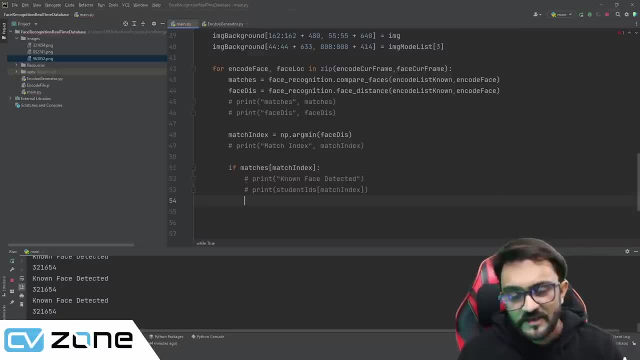 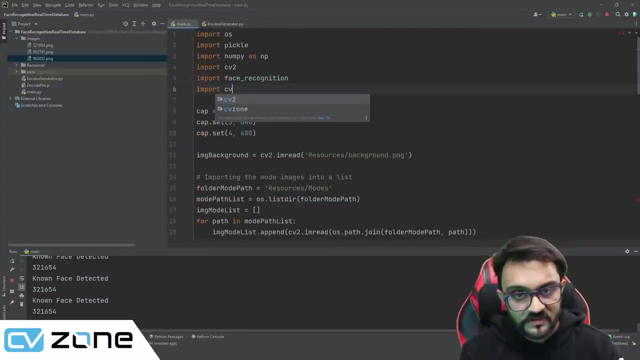 fancier, so we are going to use that. if you want to use opencv, it's fine as well. you can simply write cv2 dot erect rectangle and you can use that. or you can write cvzone dot. um, we did. we import cv zone. no, uh, import cv zone, import cv zone and we are going to write cv zone dot. 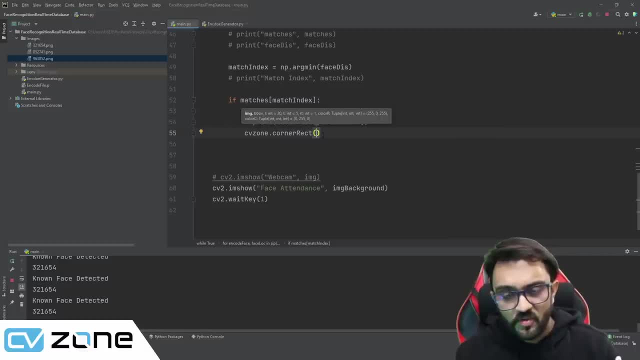 uh, corner rectangle, so that's the idea. so, uh, to fill in this, we need the image, so image background, and then we need the bounding box. so the bounding box, information, is what we need. the rest you can remove or you can keep. you don't have to give any other information. but if you want to, uh, we 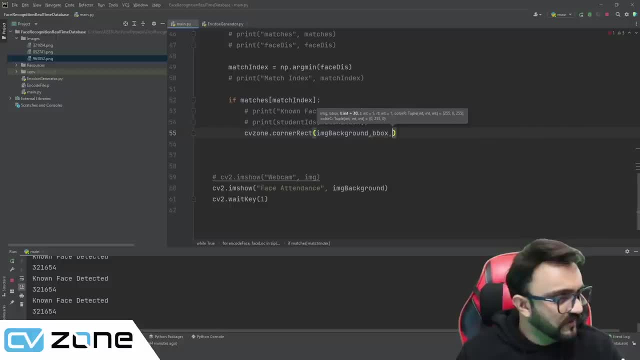 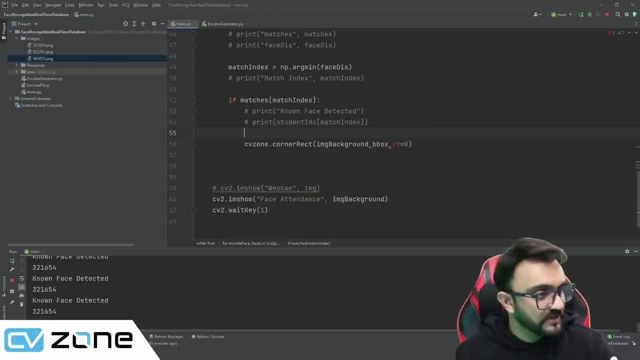 to use this we need the bounding box. so the bounding box information. what we can get is from the face location. so how can we get that? let's write it down here. so it is very weird. it is y1 and then x2, and then y2 and then x1. 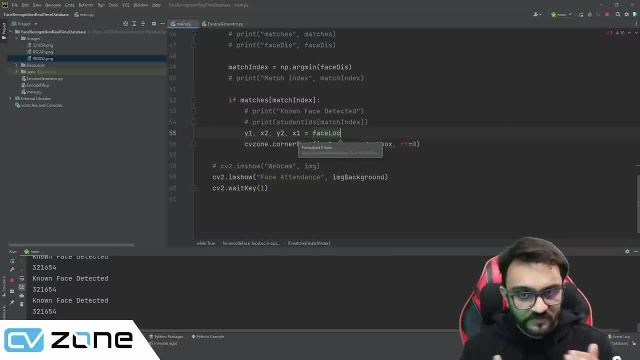 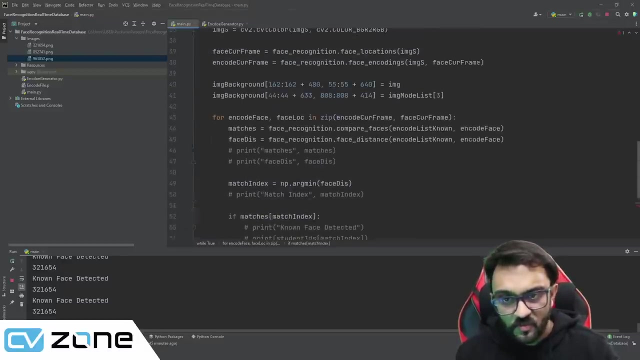 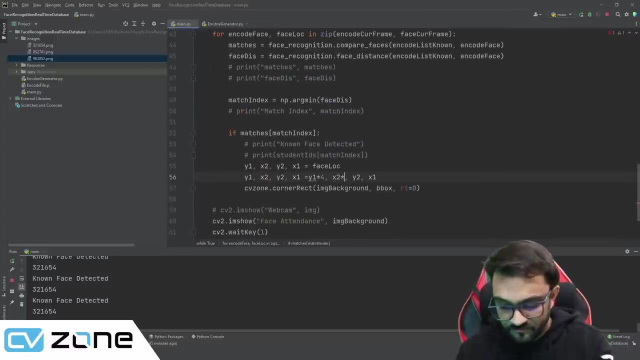 equals face location. so that's how they mapped it, so we have to use the same same idea. so then we are going to copy this and we will paste it twice, and the reason being: we have to multiply it by four because we reduce the size by four, one fourth. so now we have to multiply it by one, uh by four, so that it is uh matching. 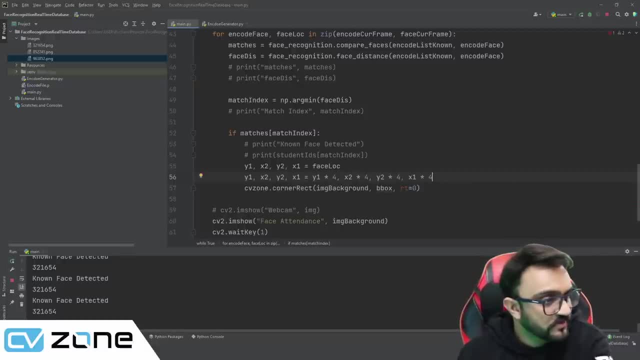 so all of them are multiplied by four. so that is well and good. now we can simply put our rectangle. so how can we create the bounding box information? so first of all, to to have the bounding box information, let's just write here: bounding box equals to have the monic box information we have. 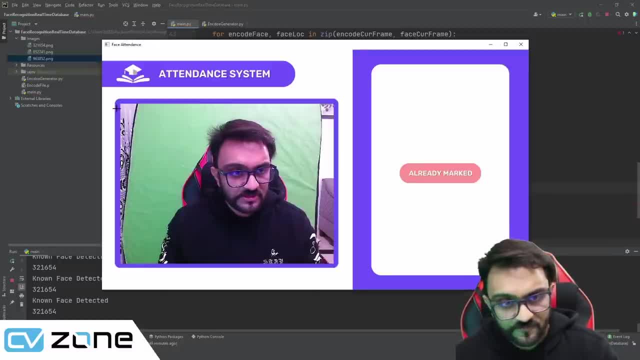 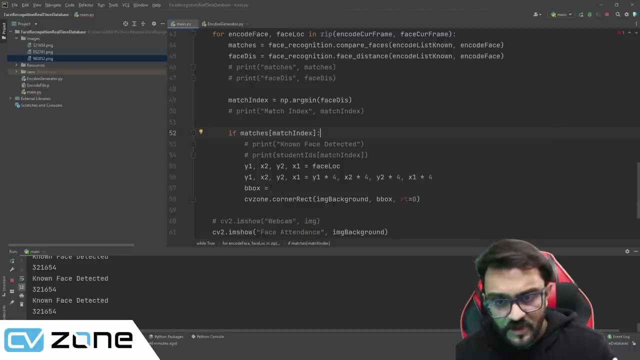 to uh remember that our image is not starting from zero. this is zero of the image. we have to add an x and y value which is for starting from here, then our images starts. so here we are putting it in image background, not the actual image. so we have to give in that offset. 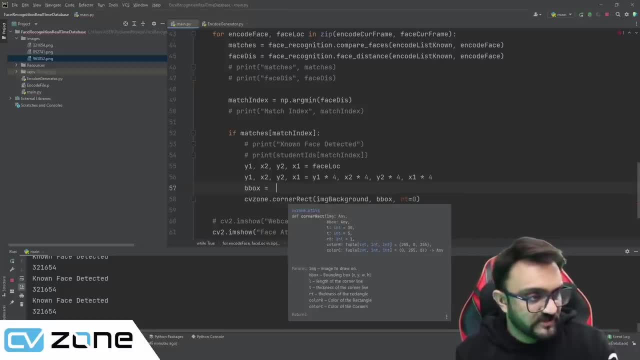 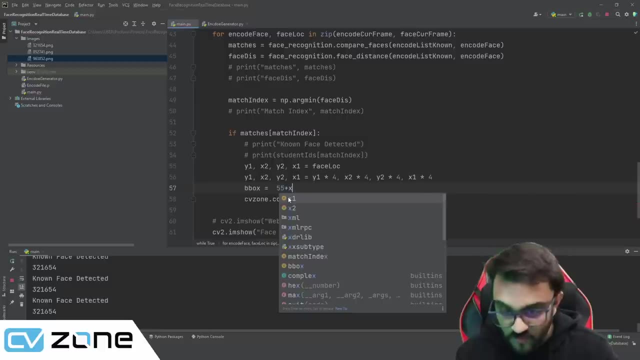 so what is that offset in the x direction is 55 and in the y direction it's 162.. so we are going to write 55 plus x1, then we have to again give 162 plus y1, then we have the x2 and y2. 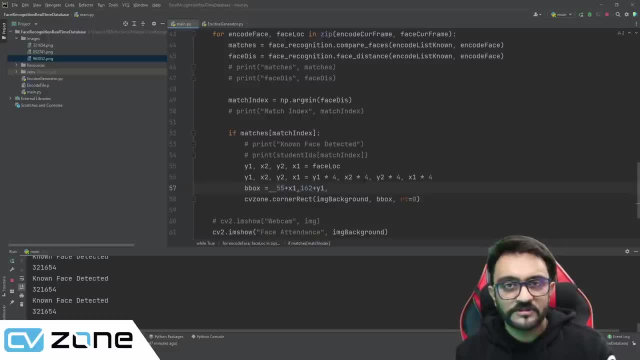 but we need the width and height. when we are talking about bounding box, it includes x, y, width and height, not x 1 y 1, x 2 y 2. it's not like that. so what we have to do is we have to uh get the x2 minus x1, so x2 minus x1, and then y2 minus y1. 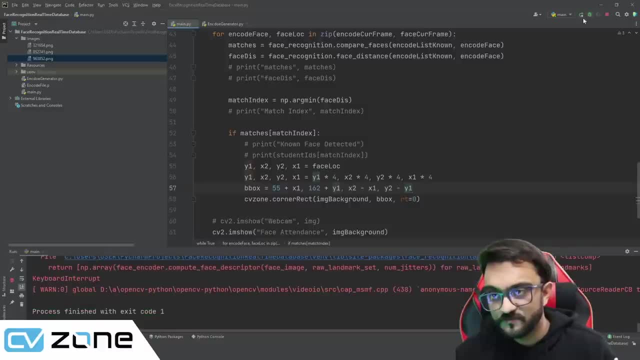 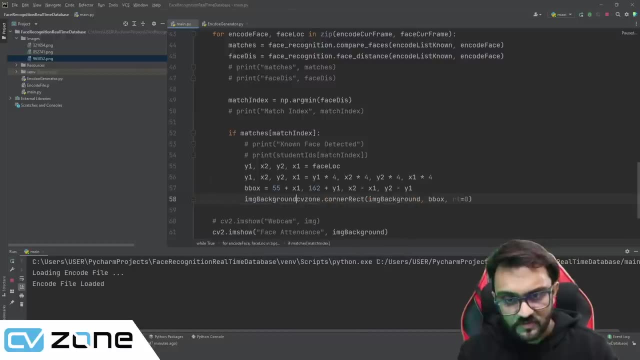 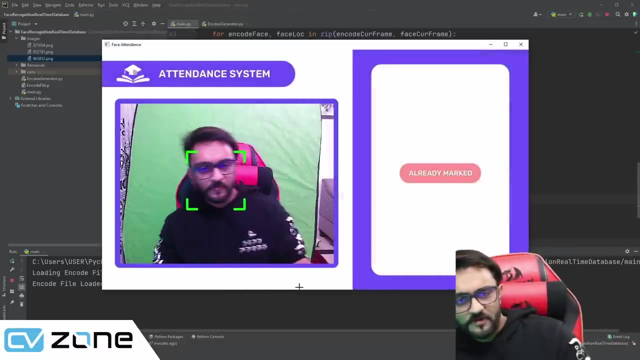 and that should give us the bounding box. so if we run this, we should have our bounding before, did we? no, we have to put it back. so image background equals this. there you go. so now, if we run it, it's should have the rectangle around. there you go. if i move, you can see the fancy rectangle. 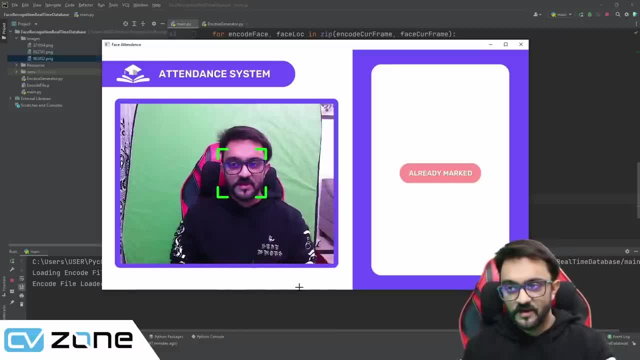 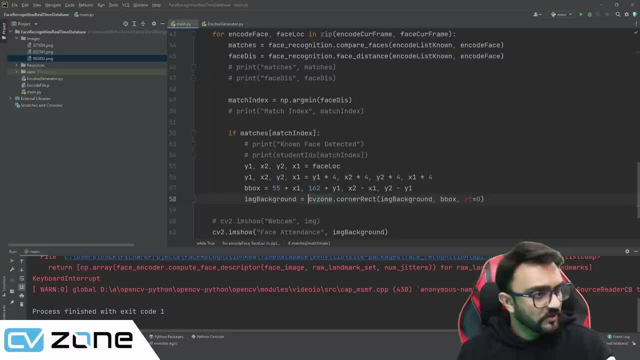 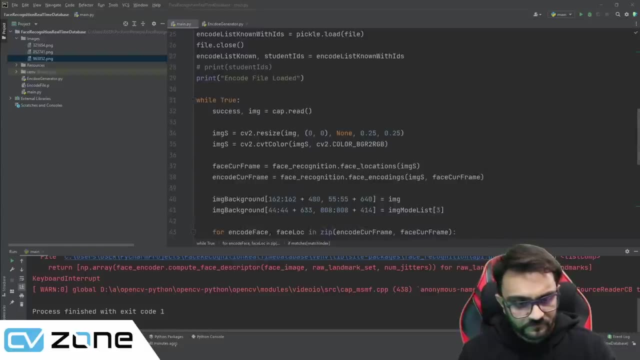 again, it's up to you. if you wanted to change it, you can use the opencv rectangle as well. it's um, it's fine, okay. so that's the basic idea and, so far, what we have done. let me go back to our image tings. and we have created the web cam. uh, we. 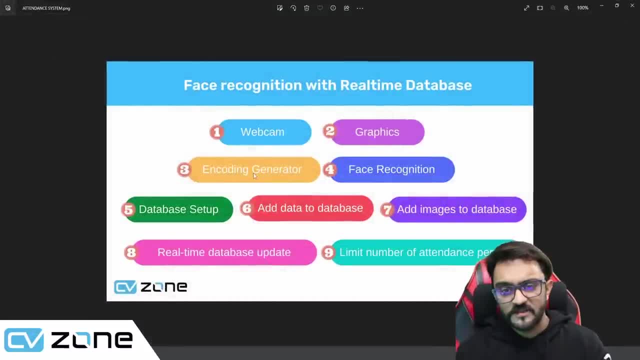 have started the webcam, we have added the graphics, we have created the encodings, we have done the face recognition. so the next part is the interesting part where we will start the database setup. so we are going to add our database and then whatever information we are getting. 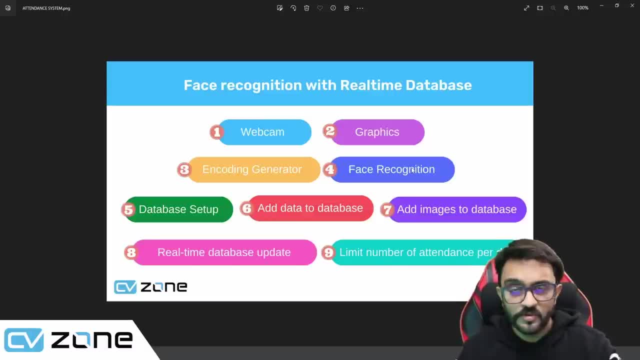 we are going to upload, we are going to download and we are going to do all of these different things. so now the database that we are going to use for this project is basically firebase, and the reason we are using this is because it's real time, It's very easy to set up and you can. 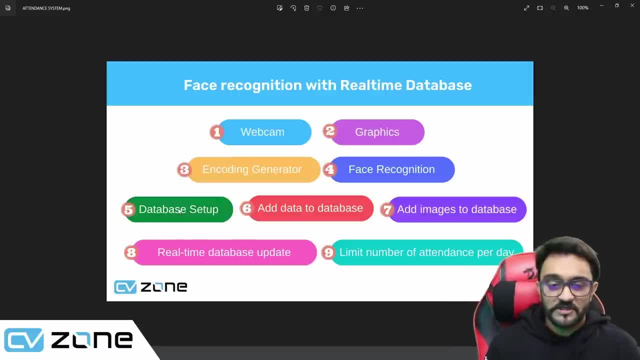 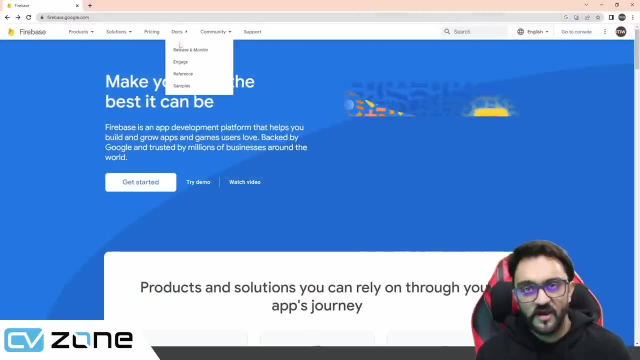 actually use it in real projects. I have seen it being used in mega projects as well, And the best part is that you can scale as you go along. It's very easy to scale this database, So let's go ahead and set it up. So we are going to go to Firebase and then you have to log in. It's free. 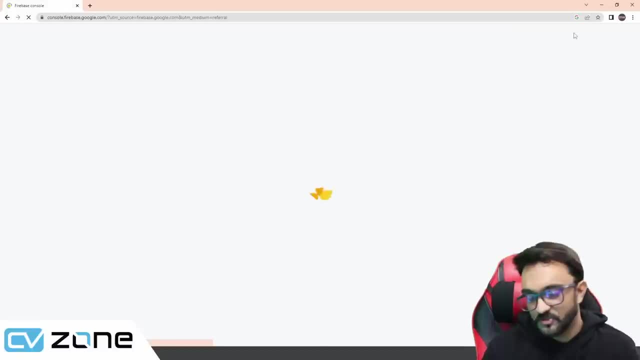 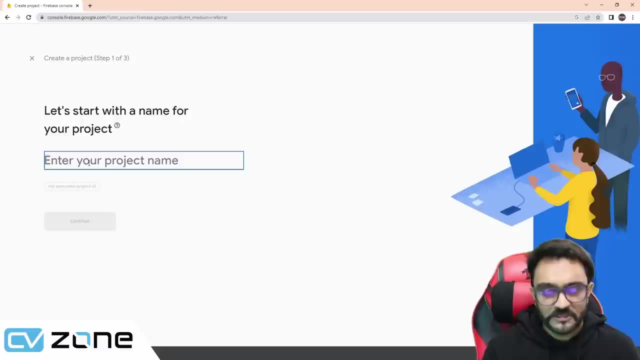 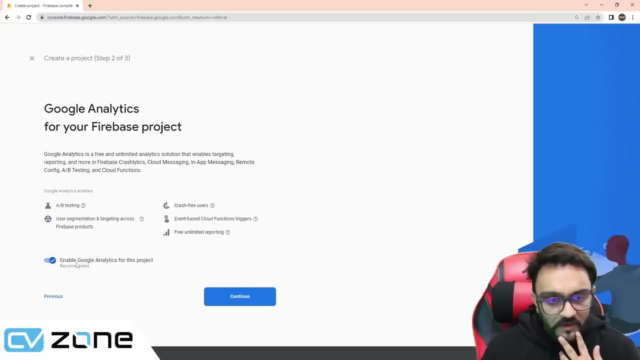 to use. So just go to Google console, Sorry. go to the console And here you are going to create a new project. So add a project here. Let's enter the project name, We will call it. what should we call it? Space attendance- real time. There you go And we will hit continue and we will enable. 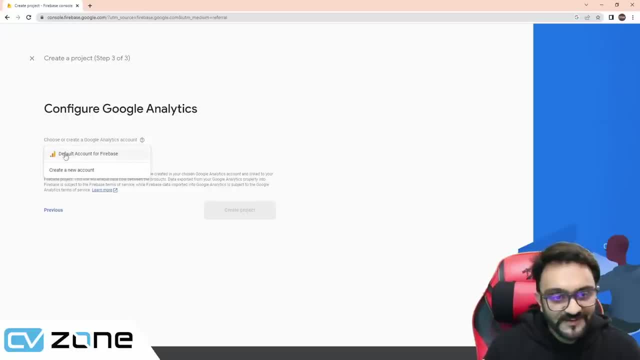 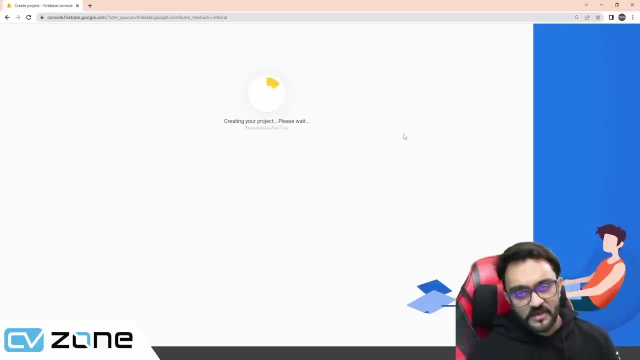 everything, No need to be shy- And then default account And we will create the project. So let's wait for it to finish And what we can do is, by the way, what we have to do is we have to create one file that will actually upload all the data to the. 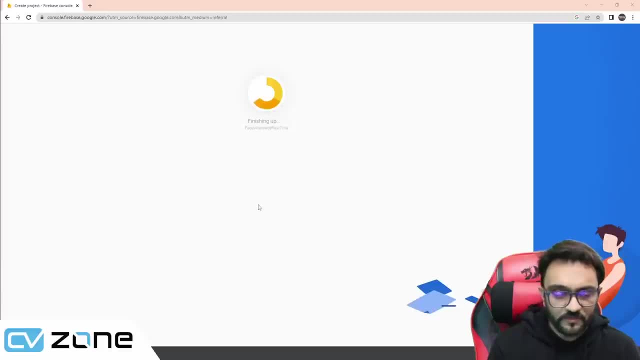 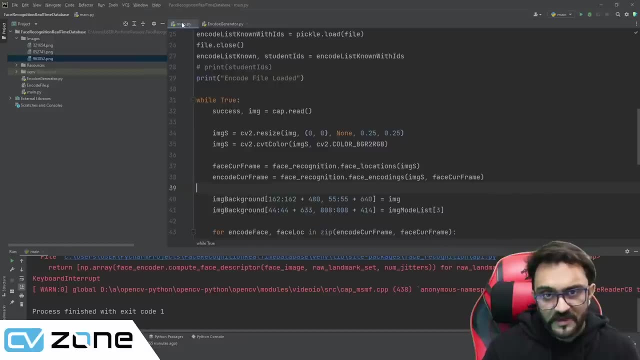 server And then the other file. it will actually help us download the code, So the other file will be basically what we are using so far. It's the main file, So we can download the data from here and then we can upload the information of attendance. updated attendance. 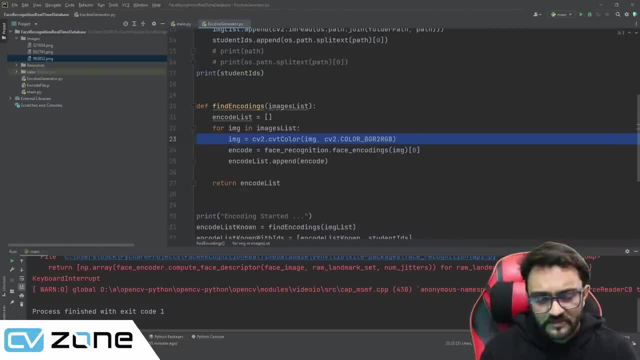 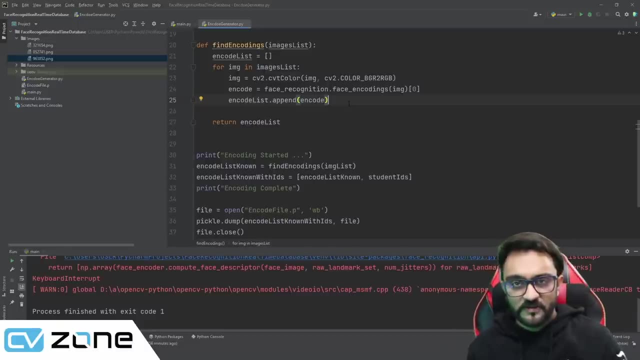 from here. But for the generation of code we have to add the images. So these images, once we store them, once we have uploaded them, we should be able to access them, Because if you look at the resources folder in the modes here, you have to show the image of the correct student, So that's. 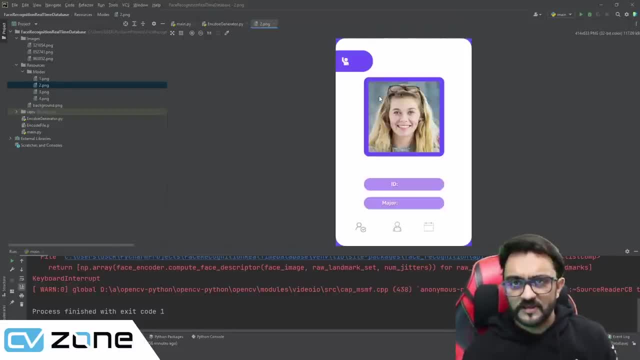 that is detected. if you don't want to show the image, that's fine, you don't have to use the storage. but if you do want to show that, you have to upload the images as well. and doing it manually again it's not a very good thing then. 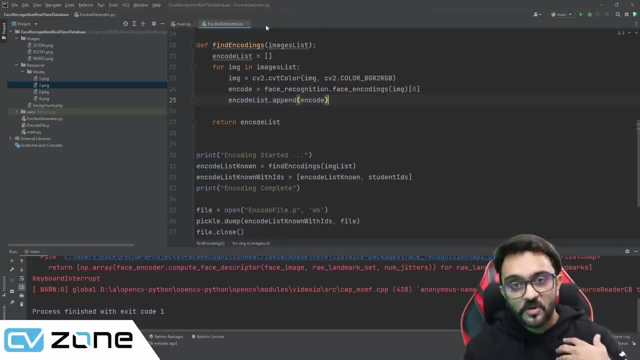 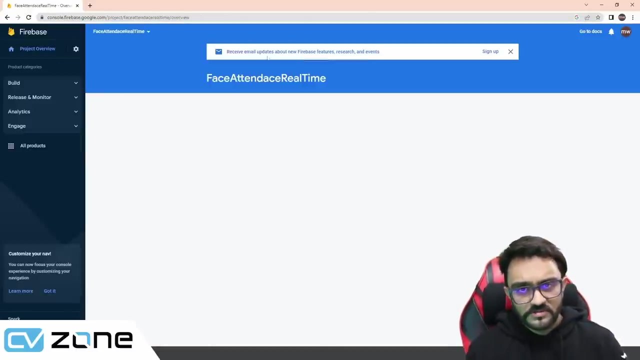 why exactly are we coding if you have to do it manually? so we will upload the images man automatically and then we will download them automatically and it will display it based on the face detected. so that is the idea. now it's the project is ready, we will go to the console face real-time. blah, blah, blah. 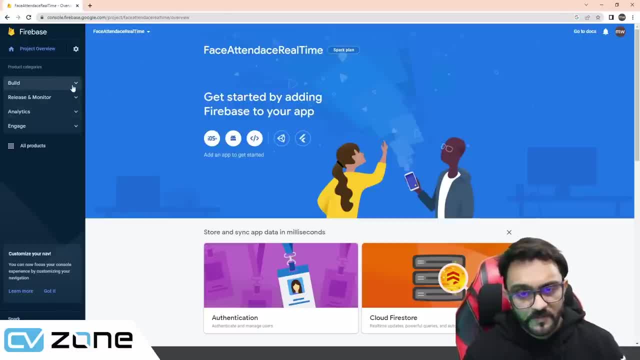 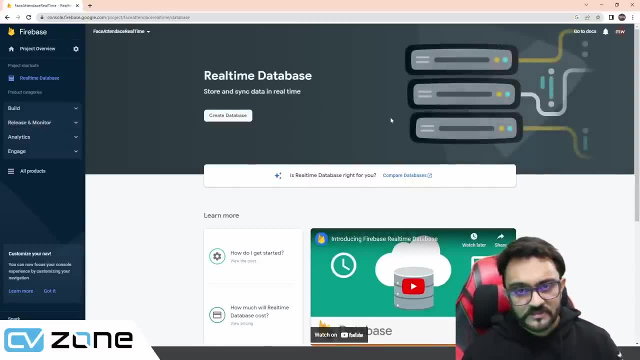 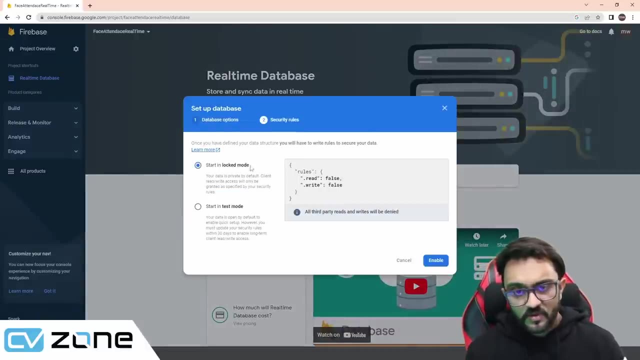 and we will close this here. we will click on build and we are going to go to our real-time database. so here you can see. we are going to click on create database and it's United States. that's fine, we are going not going to start in. 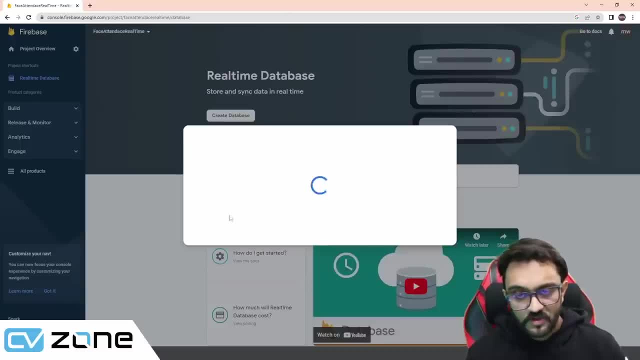 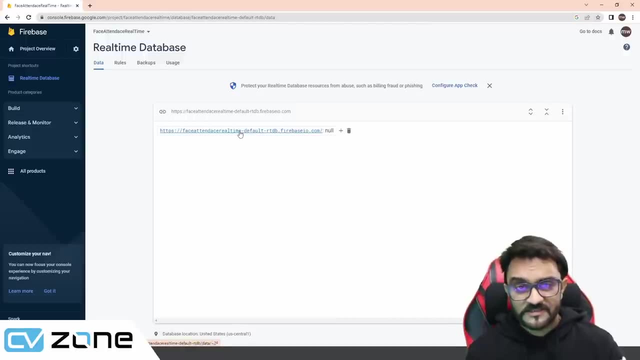 lock mode. we are going to start in test mode, we are going to enable it and here you go: you have your first database setup. that's how easy it is. by the way, this uses a JSON format, and that is exactly what we are going to use for. 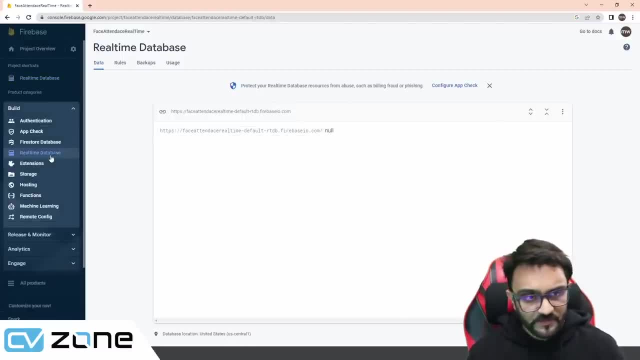 our project as well. so here we have the build and in the build we have seen real-time database. now we need to link it. we will do that, don't worry, don't go ahead. then we also have storage. so if you click on storage, you are going to. 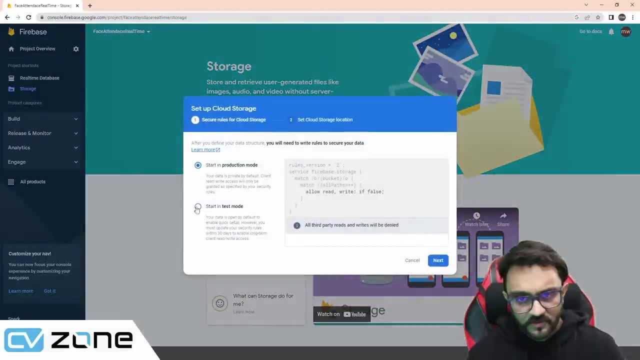 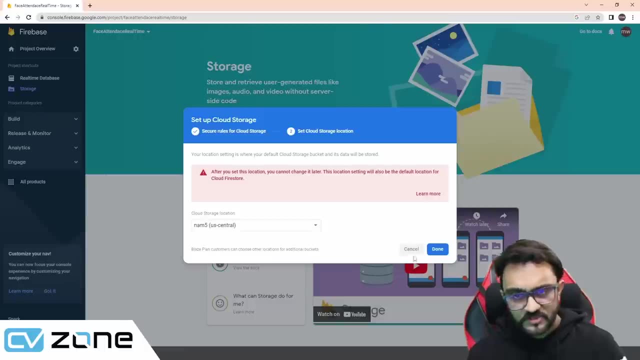 see your storage. we are going to click on get started in production mode. no, we need it in test mode. we are going to click Next and after this location is set, you cannot change it. blah, blah, blah, you will move ahead. so it's creating our storage bucket in which we will store all these files, all the faces, all the 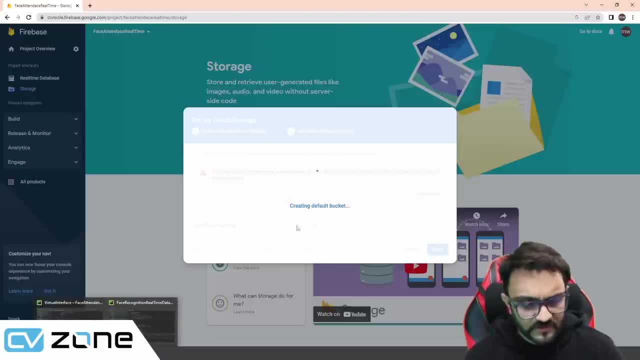 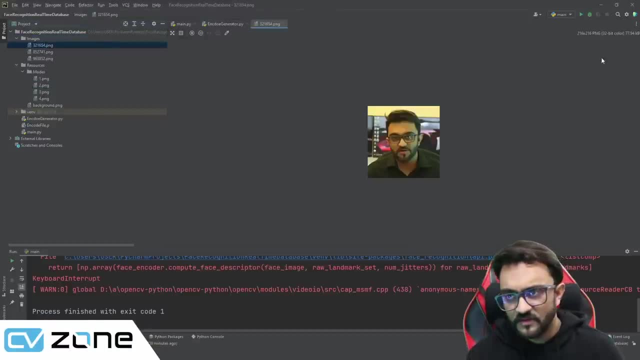 images. now, these images, by the way, they have a particular size they are. they are 216 by 216, I believe, 216 by 216, so all of them are the same size. so if you don't know how to do that, you can go to kenva or you can you open, paint and crop the image and make it. 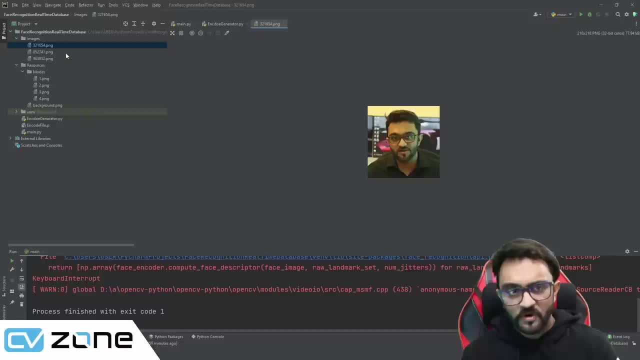 smaller. so exactly 216 by 216. so all of them are same. so it will be easier for us to use. otherwise we have to add some code to check what is the size of the image. then we have to crop it manually and not manually. we're using code and 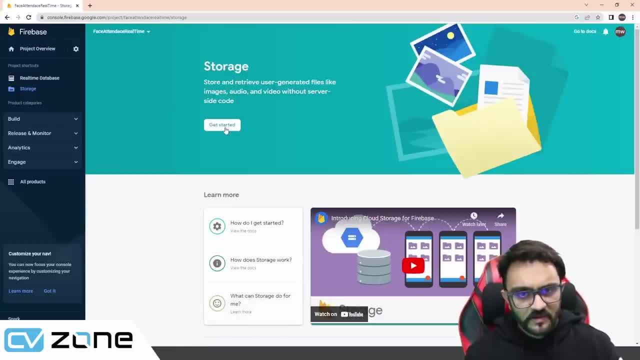 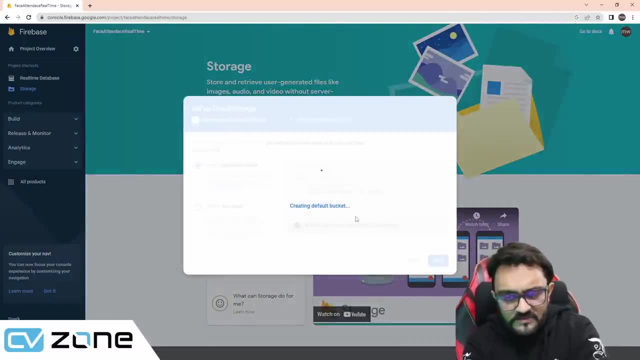 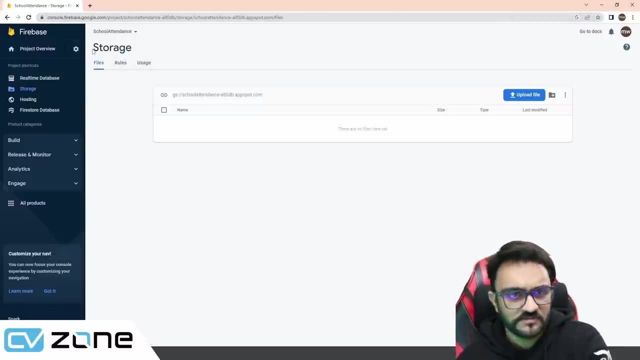 then we have to do so. try to avoid that. what happened? it didn't great- great default bucket, so it's creating. let's wait for it to create and then we will start uploading stuff on it. so I was facing some issues with the other database. I'm not sure why it's not able to create a new database. it's not able. 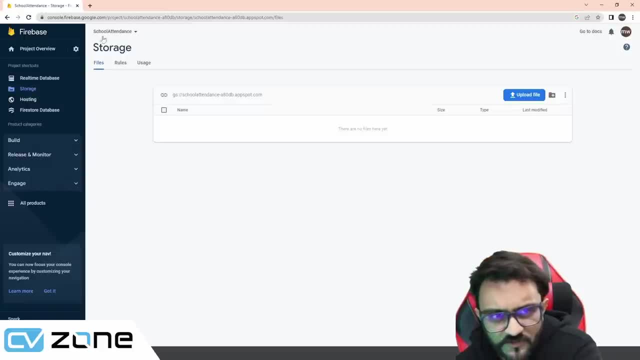 to create a new storage, so this is the old one. the only difference is the name: school attendance. the rest of it is pretty much the same. it's a real-time database as well. there is nothing inside it, and if you click on storage, you'll have this storage now. this is the link to the storage and this is the link to. 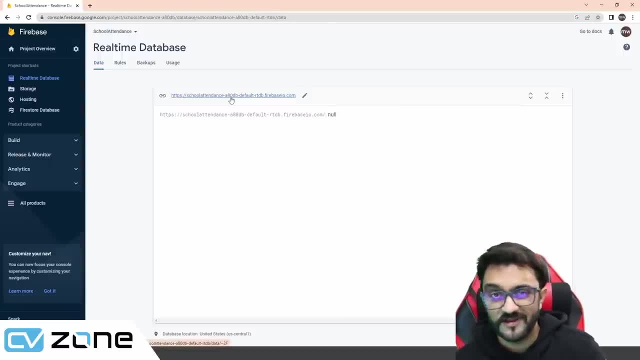 the real-time database. don't use these links, use your own, create your own, otherwise it will not work properly. so once we have this, we have the storage and the real-time database. what we need to do is we need to go to settings, project settings. here we need to go to service accounts and, in the service, 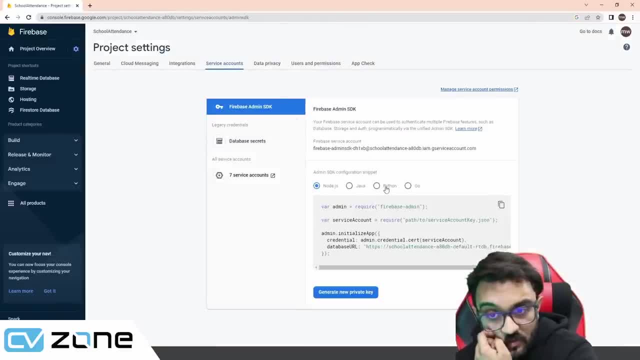 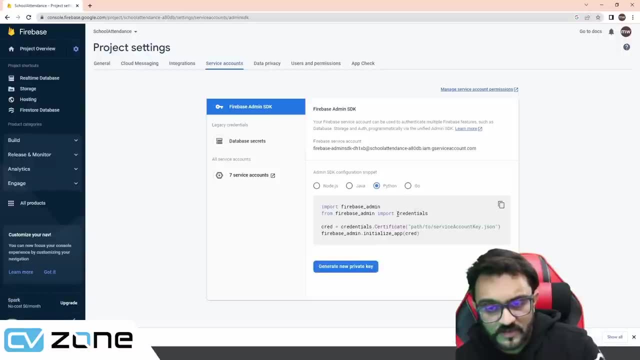 accounts. we are going to go to Python, Python, and here we will generate new private key. so we are going to create, and this will create our private key, and then we have to copy this code and add it to our Python code so that it runs. so this is. 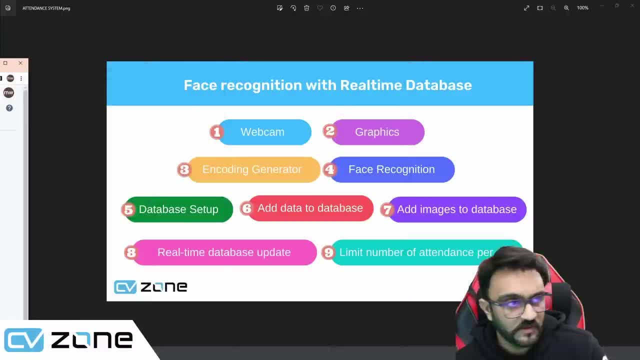 basically, they're telling you how you can use this. so let's put that to one side, then we'll open this up and here, what exactly are we doing? we need to add, we need to set up the database. once we have that, then we need to add data to a. 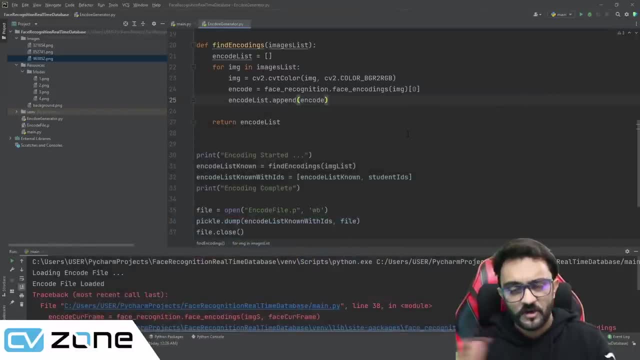 database. okay, that's good. so the the images we are going to do later on. first of all, we need to learn how to add data to the database, so we will click on Python file and here we are going to write: add data to database. okay, so we. 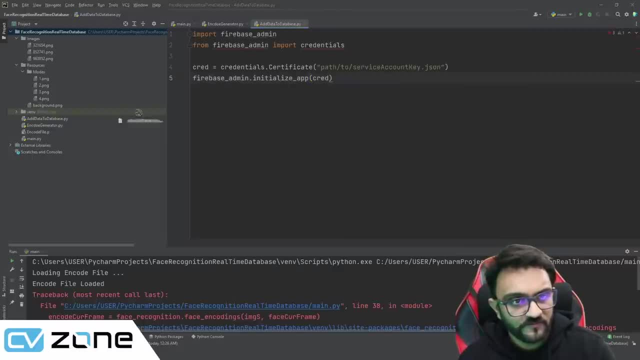 will copy and we will paste the code. then we have to just drag in the secret file, so, and we can just call it this- service service account key. so this is basically the service account key. you can see it here. it contains all the confidential information, so don't share it with anyone else. and you can create your own. 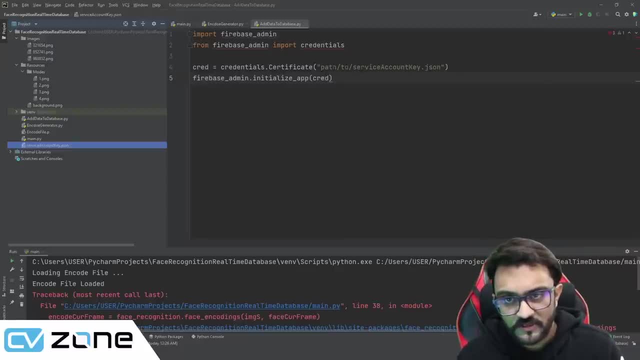 for your own database, as I have shown you. so it's going to use this file, dot JSON- and what we have to do is we have to import these as well, the firebase admin and the firebase admin package. so we'll go to file settings and we are going to add: 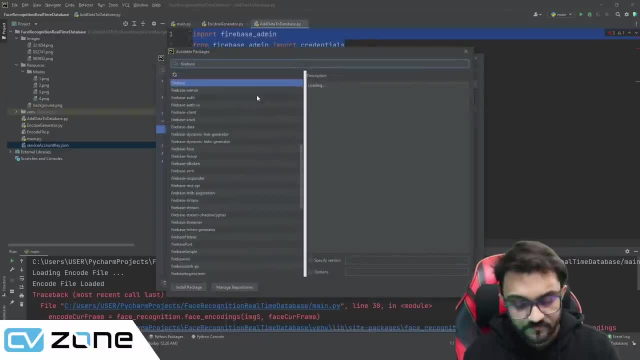 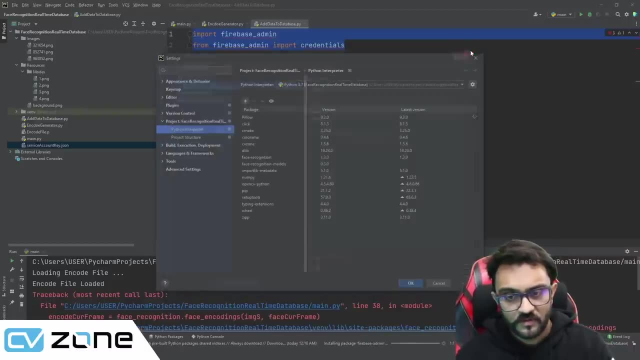 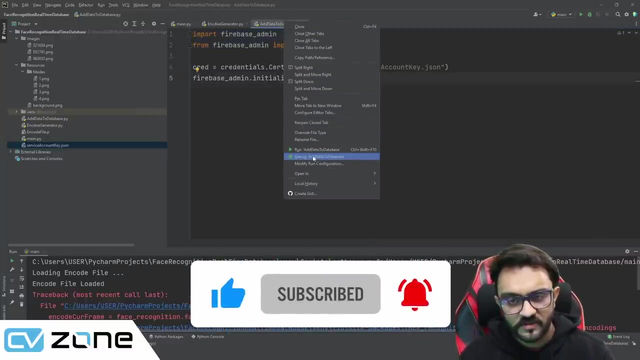 firebase dash admin. so we are going to install that, we'll hit close and we'll hit okay. so now the package has been installed successfully and we can move on. so if I just run this now, nothing is pretty much going to happen. actually it gives an error. 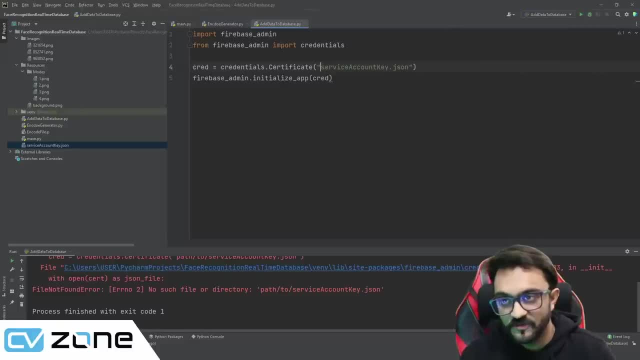 because the path is wrong. so we will just remove that. so it's directly in the same folder as this file, so we do not have to write any path. so here, service account key and the add data to database is in the same folder. so we all we have. 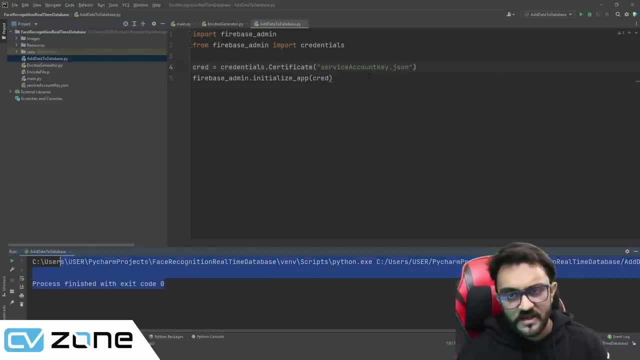 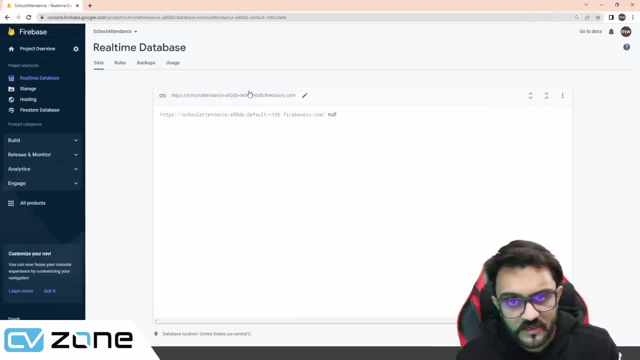 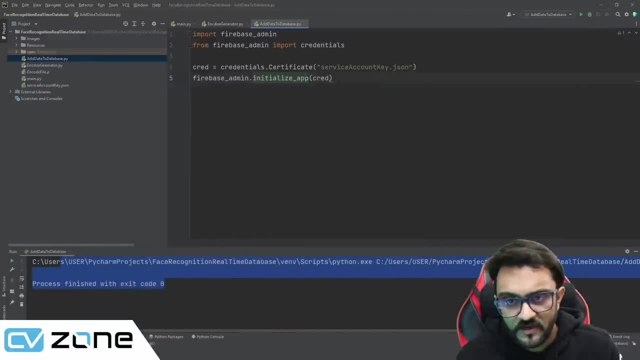 real-time database. so if we go to real-time database and let's close this here, it will show this link we have to copy. so here we can click copy reference URL and then over here we have to paste it again. we have to paste it as JSON format. so we are going to put brackets and within. 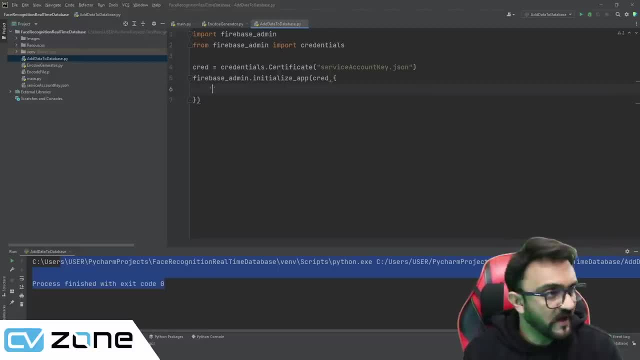 those brackets. we have to tell what value it is. the value is basically data base URL, and then we have to give in the URL of this. so that's the idea. there you go, so that is pretty much it, and then we have to create a reference. so what exactly is going to? 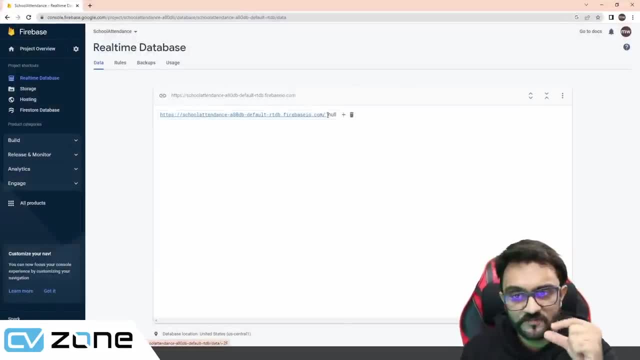 happen. this is our main directory and it has null right now. inside there's no values, there's no format, there's no data. so what we will do is we will add a format, we will parent directory, which will be students. inside that students directory, we will have the ids. 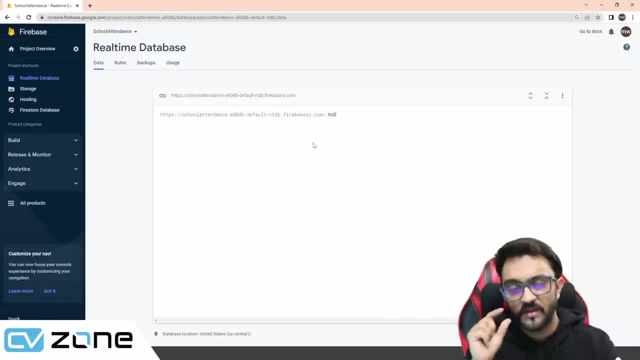 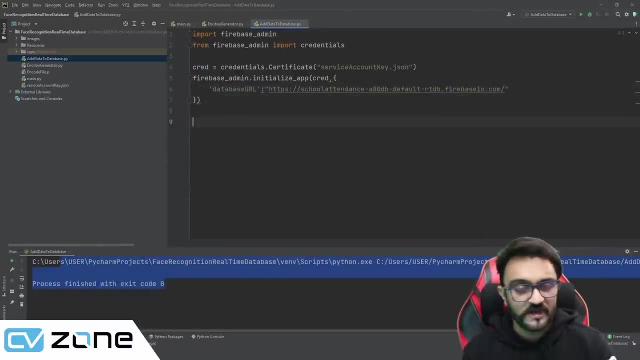 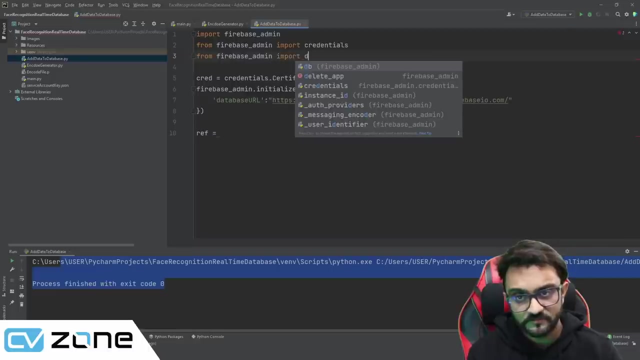 of all the students and inside those ids we will have the values of all the required things, so all the required information. so first of all we need to create the reference for this, so we will write: reference equals db. so we need to create the database reference. so we will write here from firebase admin import db, and here we will write: 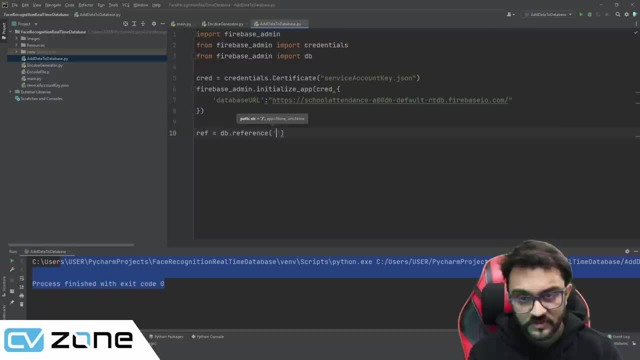 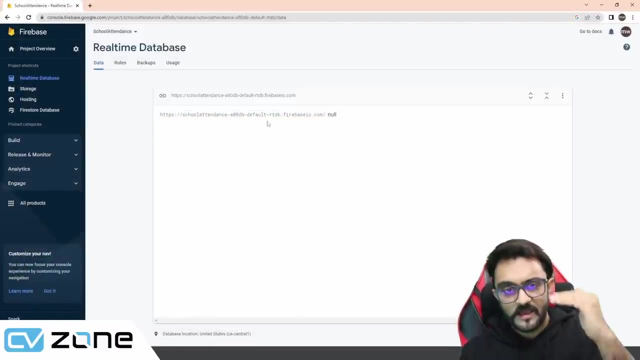 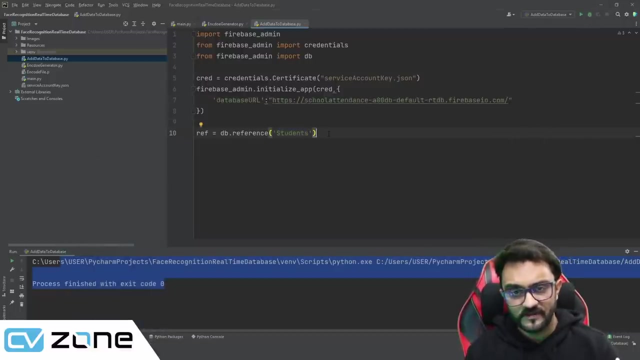 db dot reference and we are going to give in the path. so students. so this is basically the path, the reference path of our database. so it will create a students directory over here and inside that we will have all the ids of the students. now what we have to do is we have to add the data. so the data we will write, data equals. 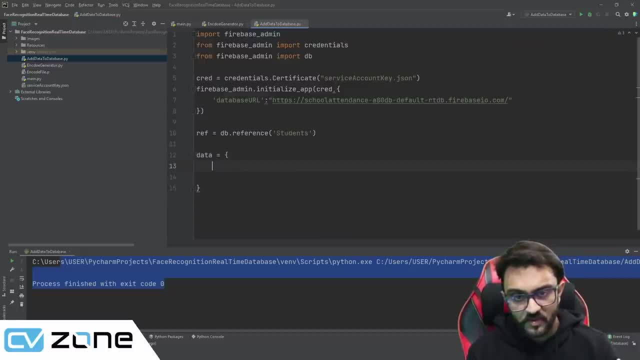 again, it's json format, then we have to give in the value, and if we want a value within a value, then we will. i will show you how it's done. so our value will be based on our student. so here we have images, so this is the id. so, as i mentioned earlier, it will be based on id, so we will write. 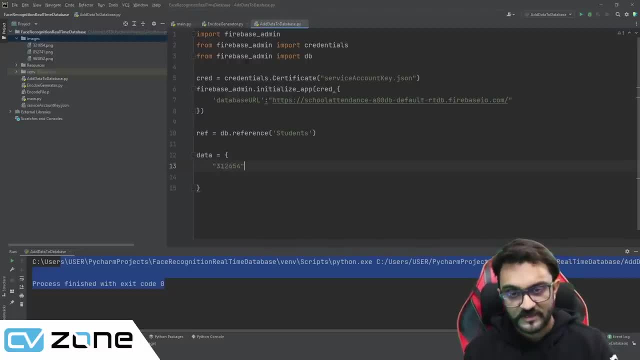 here: 3, 2, 1, 6, 5, four, so that's the ID number and in this we will have another JSON. so within this we have another JSON which is the value of this, and inside that we will have all the information of the student. so, for example, we will have name and the value. 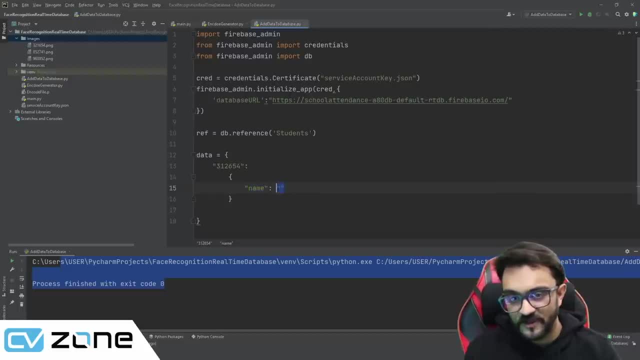 of the name. so this is called key and this is called value. in JSON format we have key and value, so this is the key and all of the information inside will be the value, and within that we have another key, another value, another key, another value. so that's how it works. so my name is Murtaza Hassan, and then we 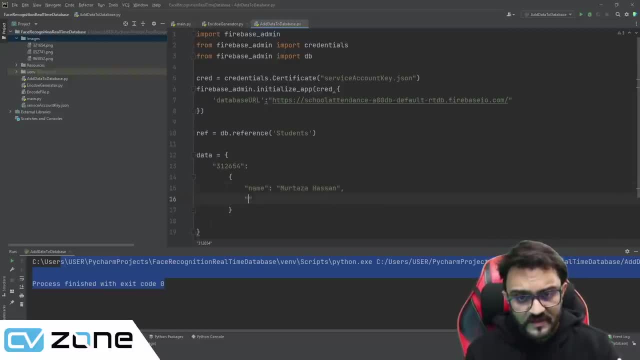 have to give in a comma. if we have more values, then we have major. so major we are going to give robotics- that's what I did and the spellings are wrong. so, very good, robotics. and then we will give starting year, starting year, and that is basically 2017. 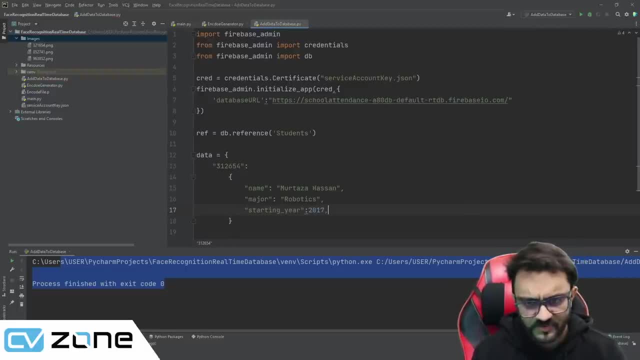 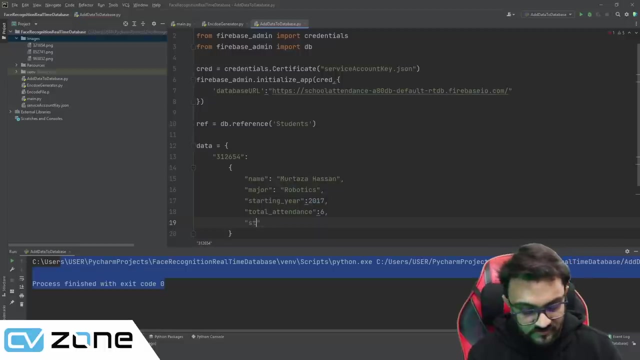 let's say that was not my starting year, though I'm old now anyway. so then we have total attendance, total underscore attendance, if I can spell it right. no, I cannot total attendance. let's say I already have, let's say, six attendance, and then we have standing. well, I'm a good student, I was a good student, Stan. 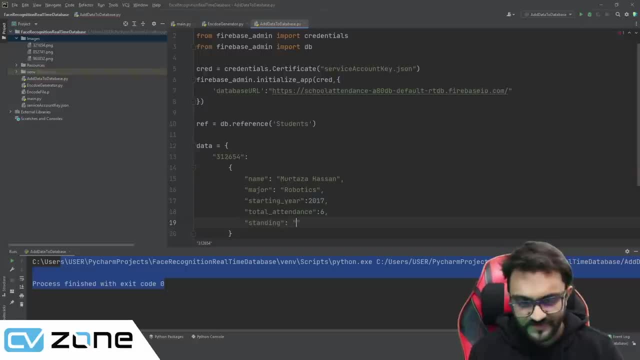 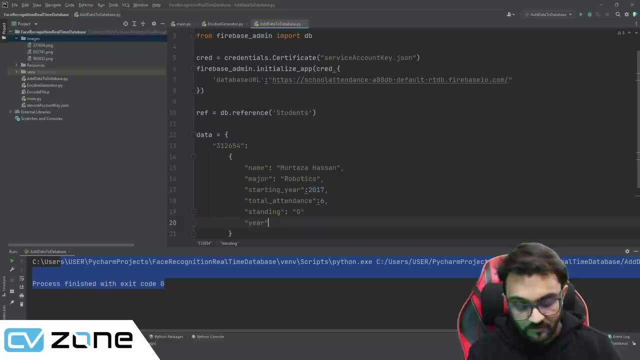 the only thing I can't do is I can't spend so. so I'm going to put g for good, and then for here we have year number four, and then we'll put comma again. I forgot it here, that's why it's giving error, and then we will rekey. so R and T. 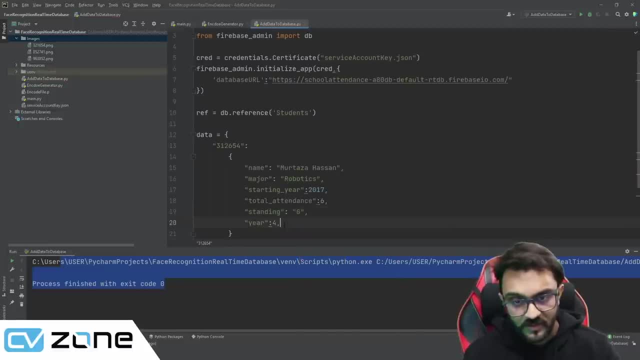 which is will be between r and a, equal to zero two. and closing, since that could depend on the Britain spell of these words and what I don't know, if they are not correct to that novel. So we have in the final nation, in the year um, so that this question is written by me, so we 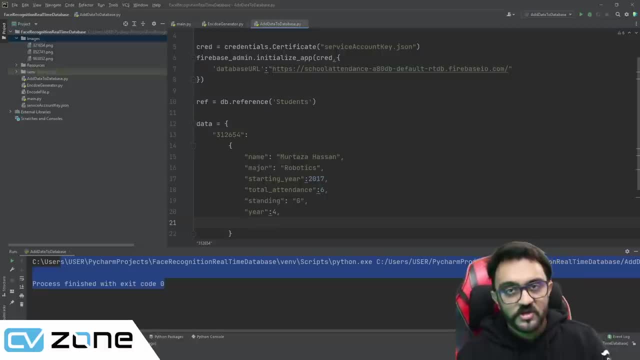 we will write last attendance time, so this will be the time that was attended last. so last time, for example, the student attended at the date of 24, and the next day they can only do another attendance. so that's what we are going to do. so here we will write last last underscore attendance. 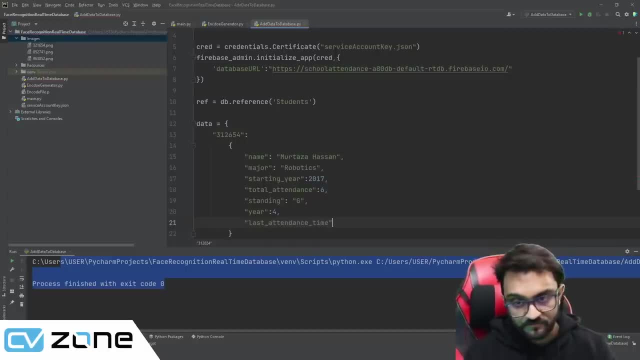 uh, underscore time, then we are going to give in the format, so it will be the first one will be here, so 2022, and then we have to give in month and then we have to give in the date. so let's put 11, and then we have to give in the time. so 0, 0, let's say 5: 4 and let's say 3: 4. so this is the time. 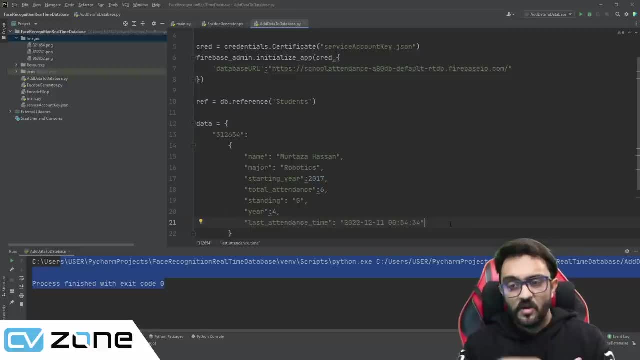 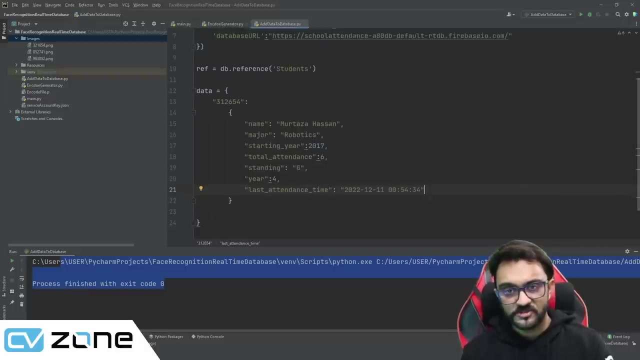 so this is the date, this is the time and you, based on this, we will check the date and time right now and we will minus it from here and then we will see whether the time is enough to count another attendance or not. so this is just a random value i've put. so now, this is for one student. so what i want to do is i want to show. 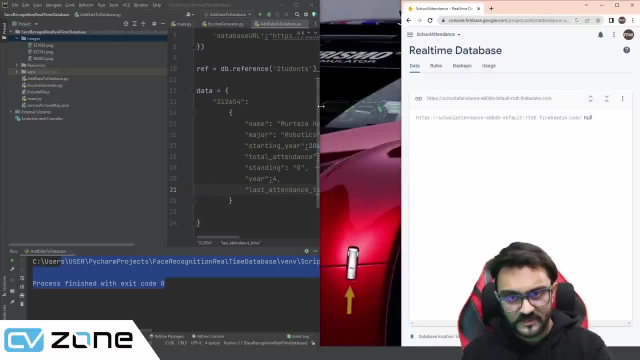 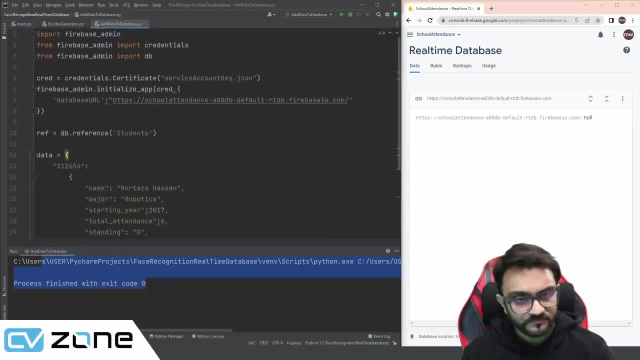 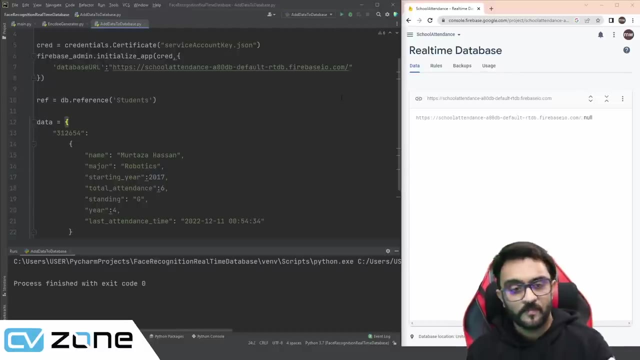 you this in real time. so i have put the database on one side and i've put this on one side. let's just remove this and there you go. so now, if i run this now, it should real time update over here. so let's click on add and let's wait for it, and nothing happened. 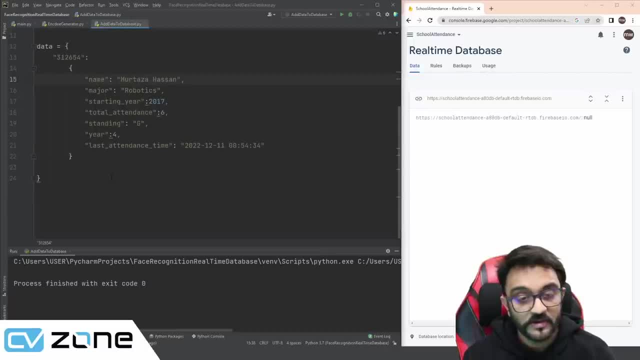 why did that happen? so, oh yeah, sorry, i just went too far. i have to add, we didn't actually send the data, we just wrote it and i got excited. uh, what we have to do is we have to send it. so we will say for key, key and value. 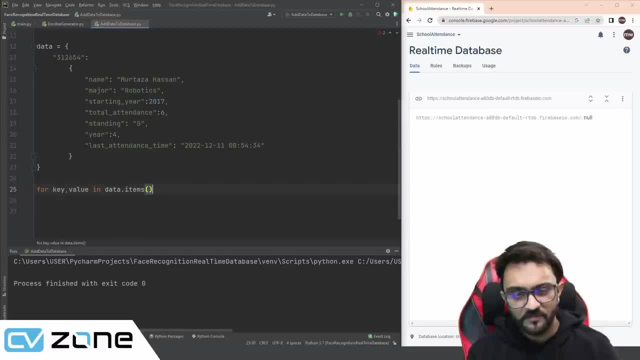 in our data. so we will write data dot items. uh, basically it's a dictionary. so, uh, in python it's a dictionary, but it's a json format. so that's how you um unzip a dictionary in python. so we will write reference dot- child. so if you want to send the data to a specific directory, then you have to use child. 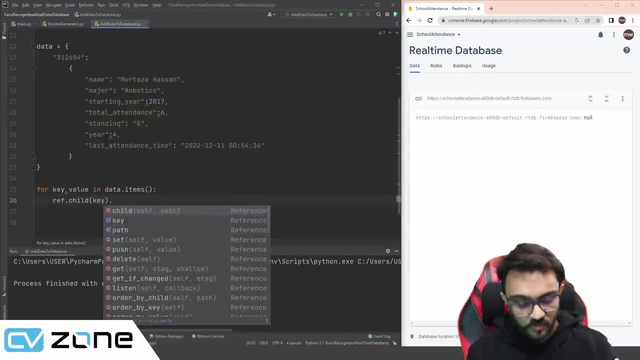 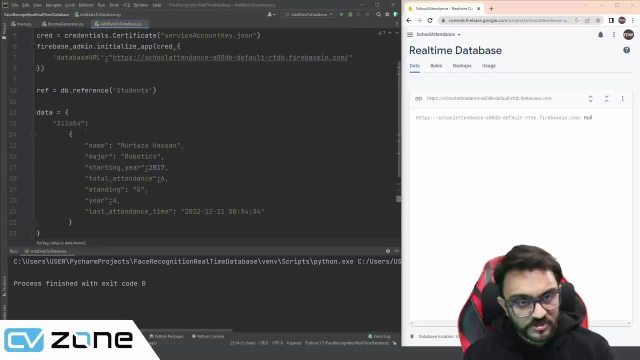 and we will put it in the key. and what value do we put? we will write set. we will write set value. so it will take the key and the value. so this will be the key and all of this will be the value. and then this will be the key and all of this will be the value. 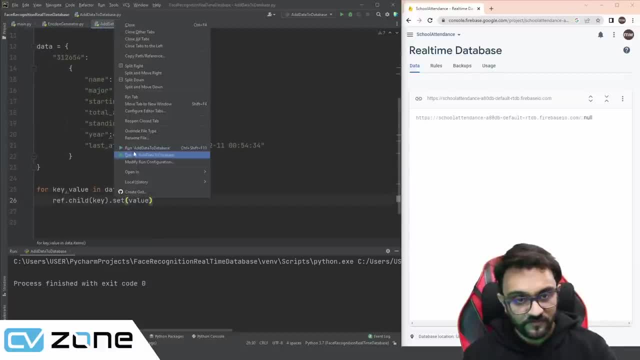 so, yeah, that's pretty much it now. if we run it, hopefully it will turn up here. there you go. so it created students. that is the folder, let's call it folder. and then inside that folder we have another folder which is 312654, which is my id and 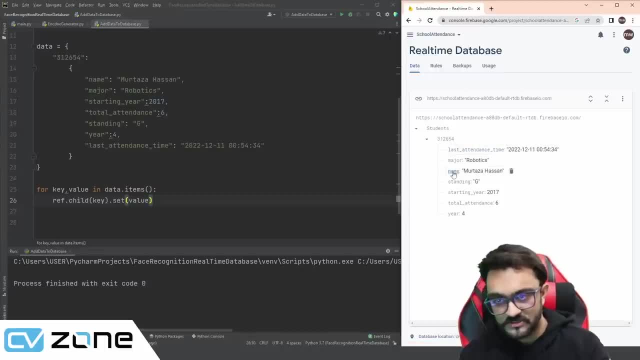 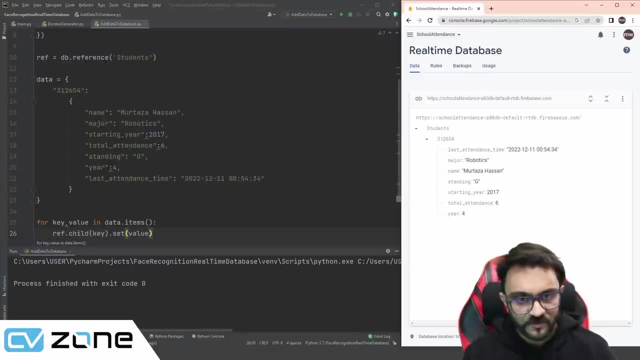 if i open that up, it has last attendance time, which is this: robotics, the name, the starting year, attendance and all that. now if i change anything, for example, if i change my name and if i only write murtaza and i run it- it will only update this part. oh sorry, this part- the name. 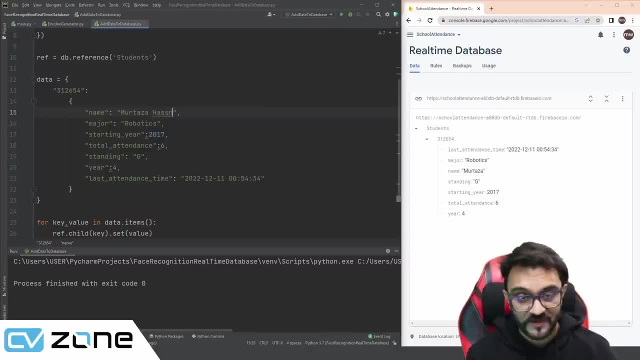 so that's how it works. so that's why it's real time, it's good and it's fast. so if i write there, hassan, and i update it now it is updated with murtaza hassan. so again, if i have more attendance, i can add seven to it and it will automatically update the total attendance. 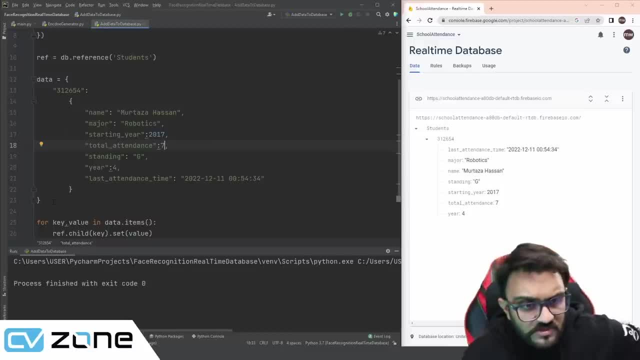 to seven. so that's how it works. so now we can just copy this part, this part, and we can paste it twice. and don't forget the comma, because for every other value we have to add a comma to it. so that's how it works. so now we can just copy this part, this part, and we can. 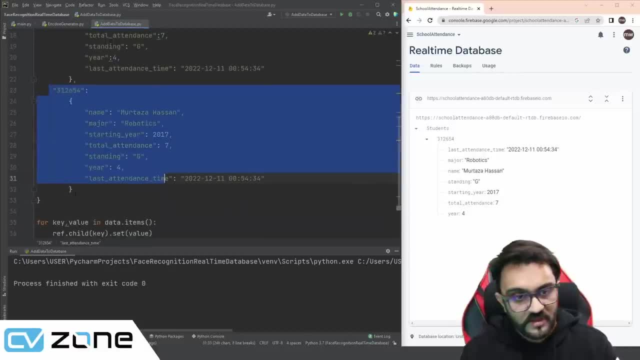 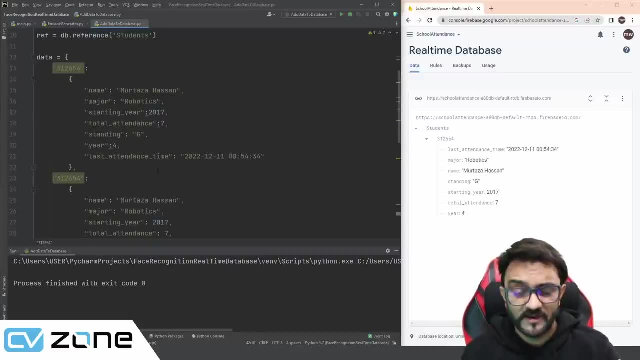 add a comma, so this is the next one and then we have another one, so this is the one after that. so this basically normally is done through an admin panel, so when the admin actually registers a student they will add it or initially the information in their database. this is: this is: 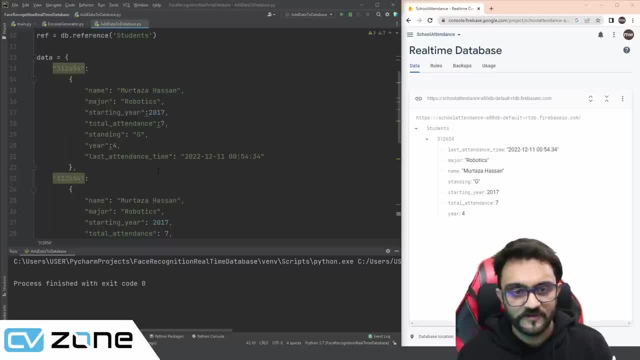 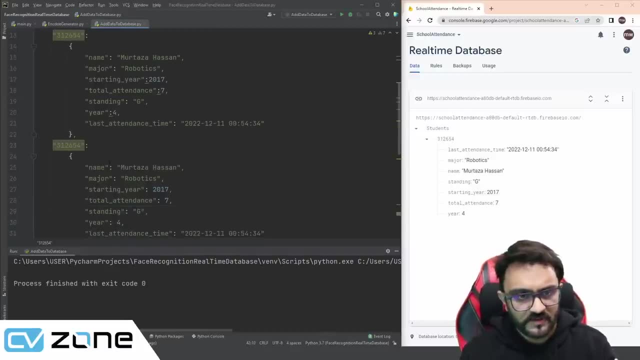 what we are doing using a python script, so you can create a graphical interface for this to for adding as well, but you will need to use a pygame or tinker to actually create that. so, uh, then we have, uh, the other numbers. what were they? let me check, because i forgot. 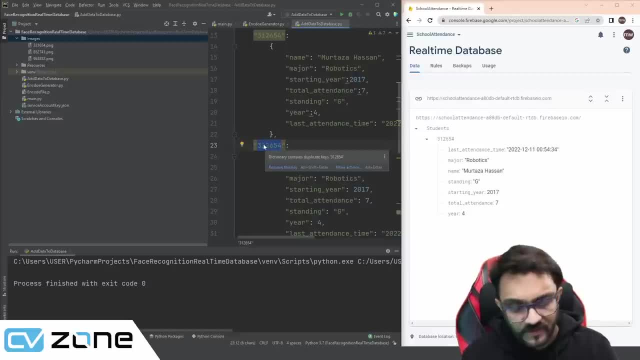 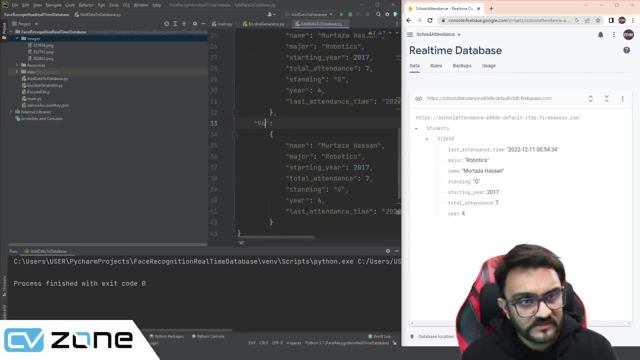 for emily blunt, we have 852741 and for elon musk, we have 963852. so here we are going to write the names. so emily blunt and her major is, let's say, economics and she started in 2018. total attendance is, let's say, 12. standing is bad. she didn't. 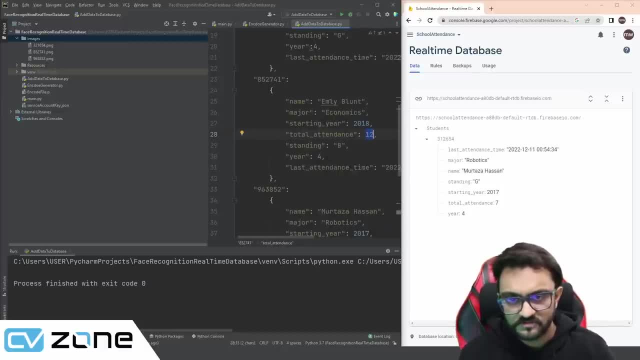 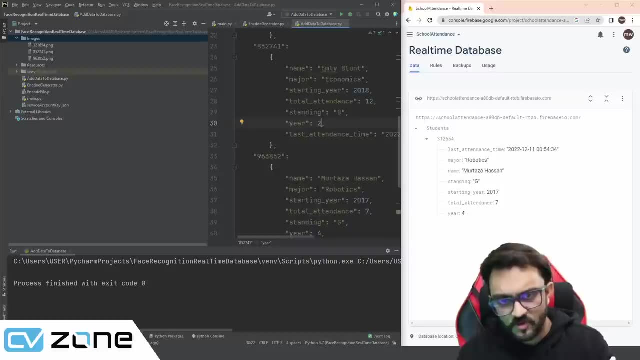 attend a lot, but what? or let's say, okay, it's bad, I'm not going to go into too much detail. so here is number two and last, and this time we're going to keep the same. here we will write: Elon Musk. Elon Musk and his major is, let's say: 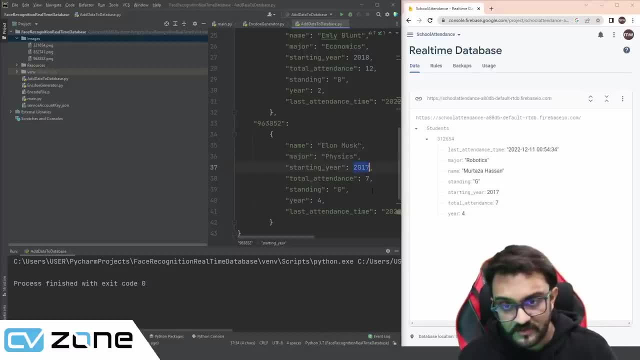 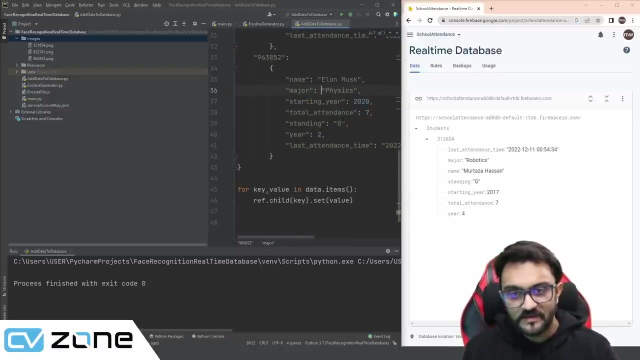 physics and he started in 2014 and this is is okay, that will be too much. let's put 2020 and he- his ear- is second year as well, so she started in 2018. about wrong 2021 and the ear will be one quite bad, and his standing is good as well, and 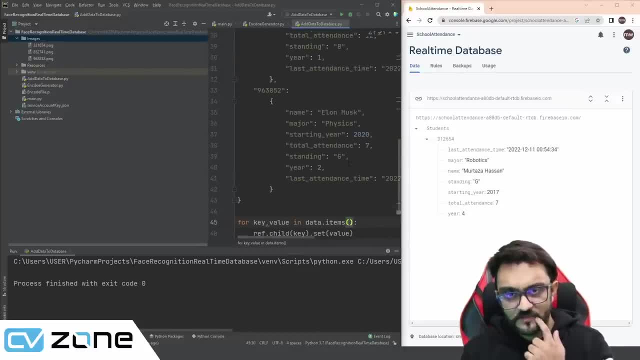 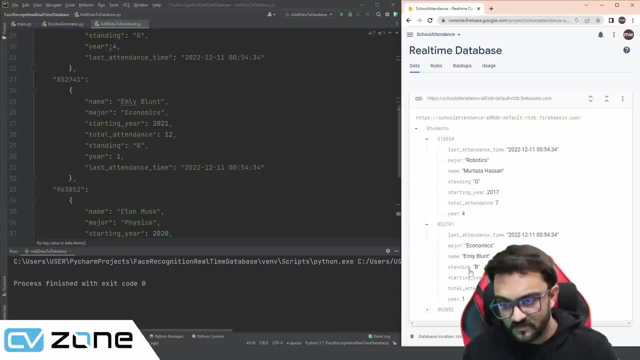 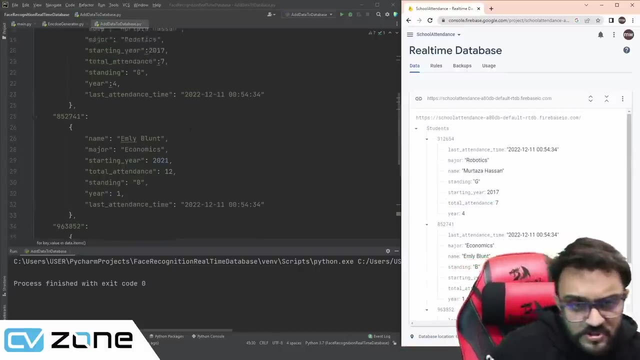 attendance is this, then it's time. so now, if we run this, it will automatically update it and we will be more students added. so we have the Emily Blunt and we have Elon Musk. so all the data has been added to our database. so anytime you want to update the basic. 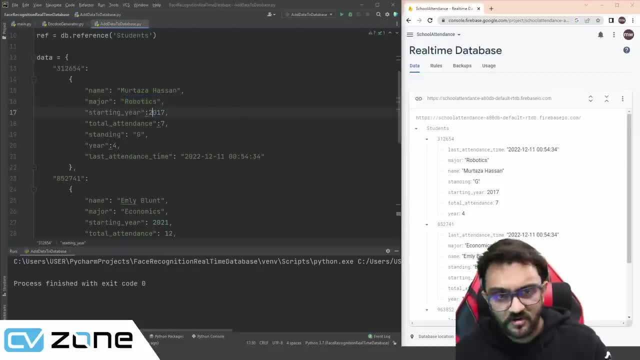 parameters: the name, the major, the year or something like that. you can come back here and update it. otherwise, the attendance, total attendance number and the last attendance date time, we will update it, and then we will be able to update it. and then we will be able to update it. 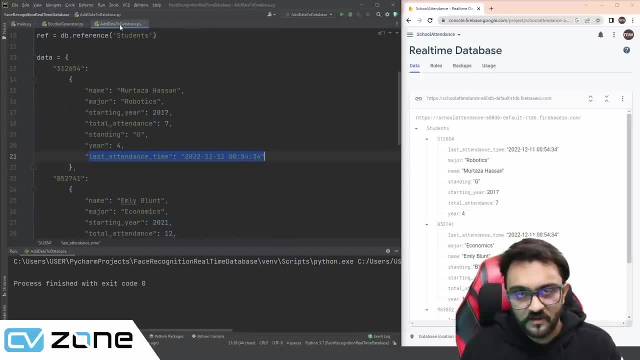 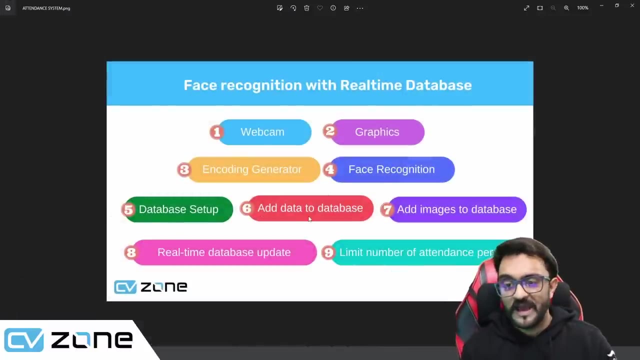 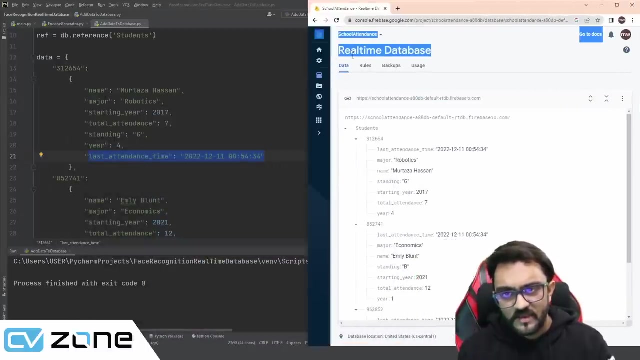 from our main code that will update whenever we have detected the face. so that's the basic idea. so this is good. now we are done with our step number six: add data to database. so we have done that. now we will add images to database, not the database, the storage. so let's go here and, as you can see, we have our 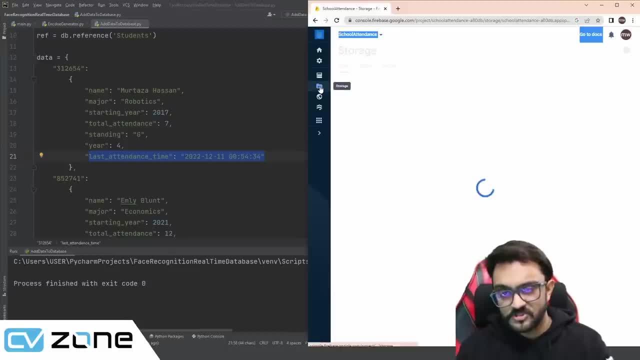 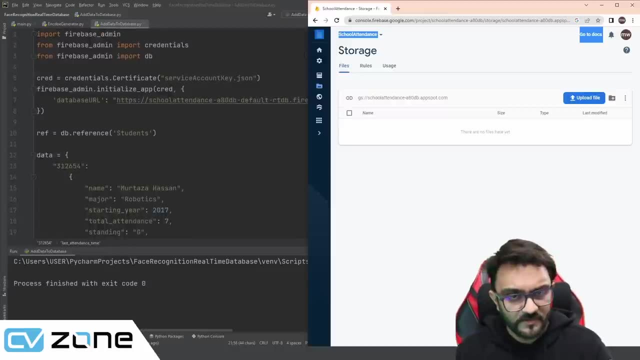 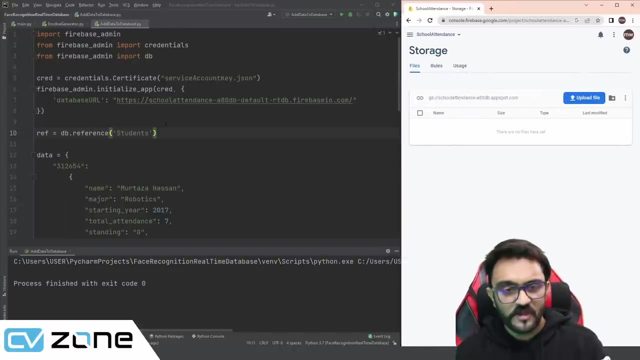 project over here overview storage. so we'll click on storage and this is our storage. so pretty much, uh, what we have done with our database, we will do with the storage and it will give us something similar. so we have to add the images and then we have. 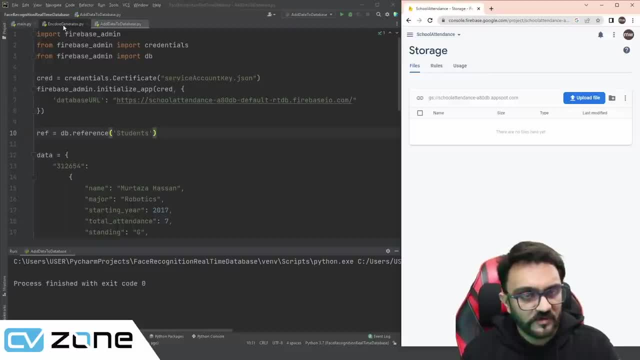 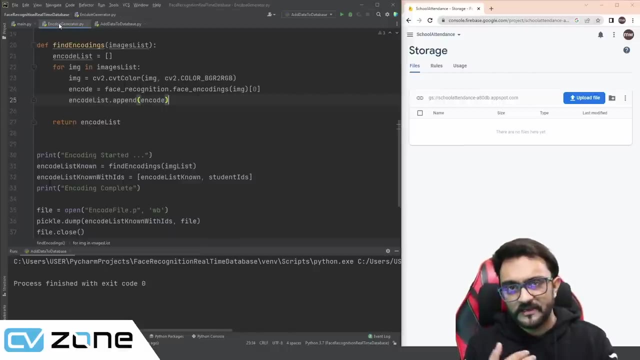 to upload it, then we have to download it and all of that. so we have to create a bucket now the images. we should not create another file to upload the images. we should do it with the same file over here. so what, we are running the encodings, we are automatically adding the images. we are 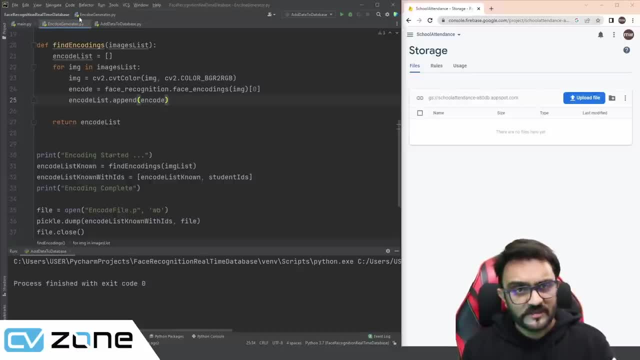 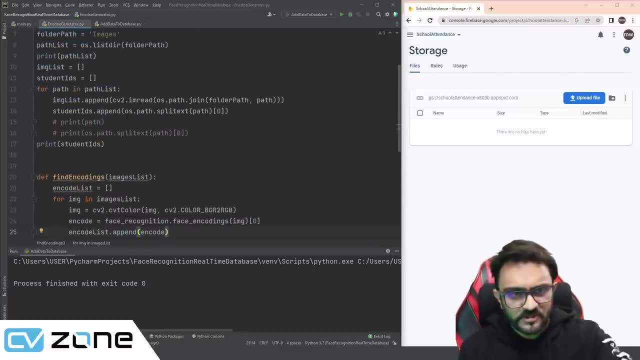 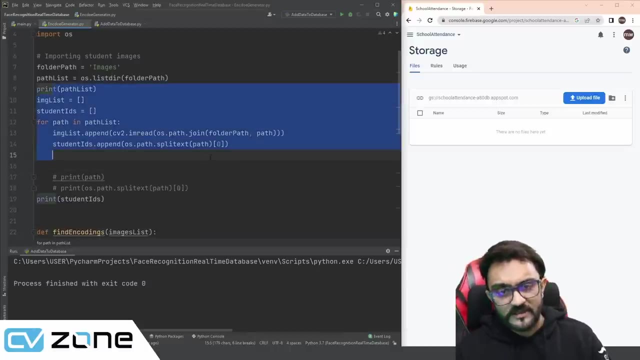 importing them, so why not upload it then? well, you can do it in add to database as well, or you can do it when you are generating the encodings. so let's do it here, because the code is pretty much done here. so let's just be lazy and add it here, so we are already getting all the images. 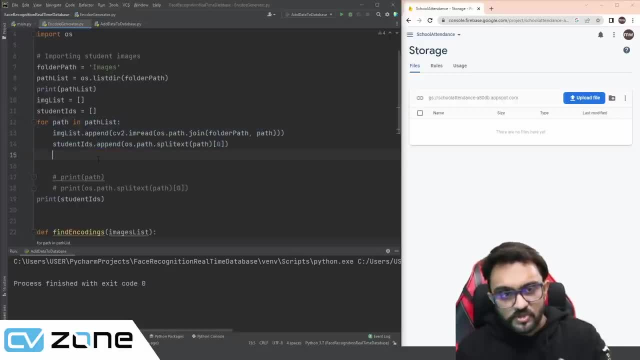 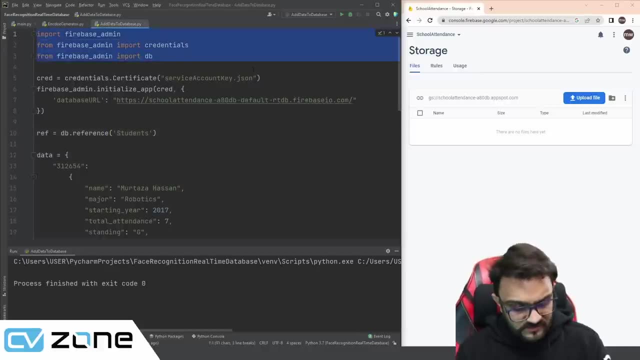 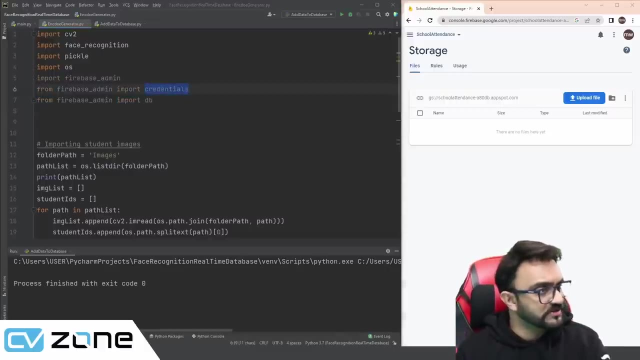 and we are storing it one by one, so why not, one by one, send it to the database as well? so here we are going to copy this firebase admin, all that stuff. uh, we need the credentials and we also need, we also need the storage. so we will write here: uh, 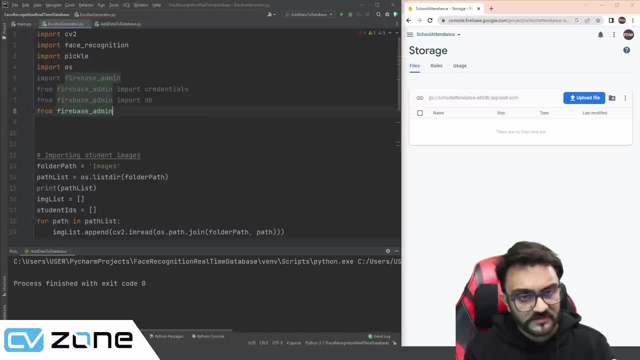 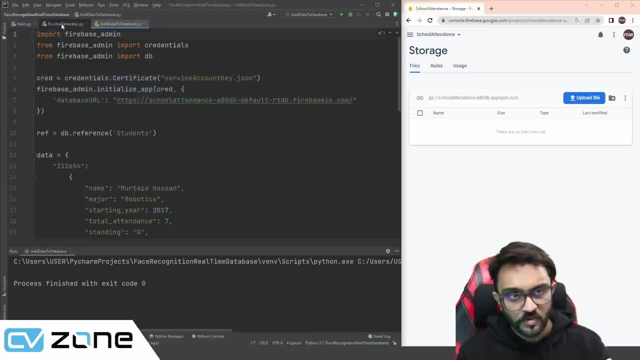 import from from firebase admin import storage. so we are not going to use credentials, I believe we are just going to use storage. so, uh, we are going to pretty much use the same code. we are going to copy it from here. we are going to go to encode generator, we are going to paste it here now in the credentials. 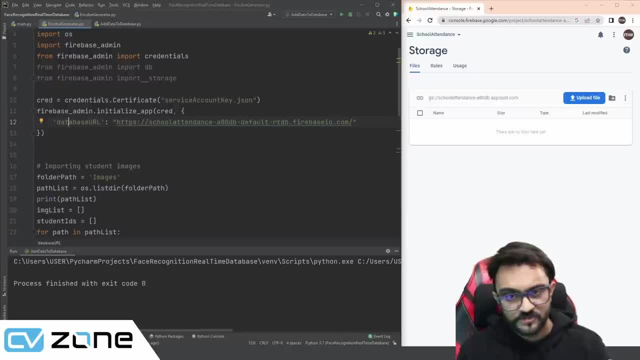 we have given the database, but now we need to give the storage. so here we will write: storage- uh, what was it? bucket b, u, b, u, c, k e t. the link to the storage bucket is again. we will copy it from here, but this time around we have to remove. 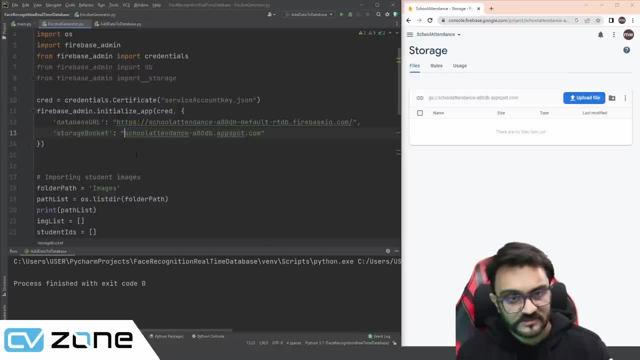 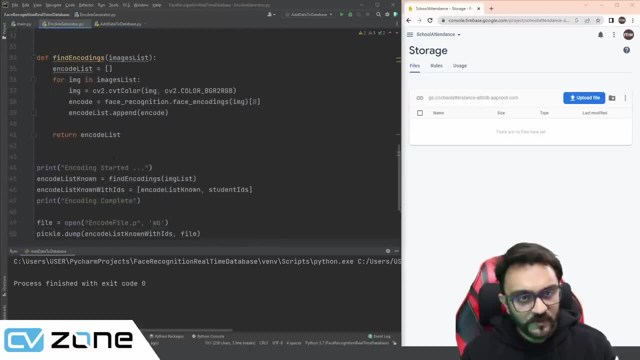 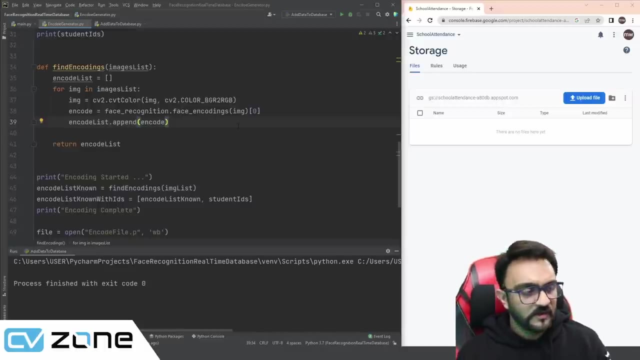 some parts. so we will remove the gs dot, slash, slash. so we are going to remove that. so once we have this, we are going to go into our loop, the loop in which we are going through all the images. so what we can do is we can put inside this code: uh, the, the name list, basically, uh, or we can write: 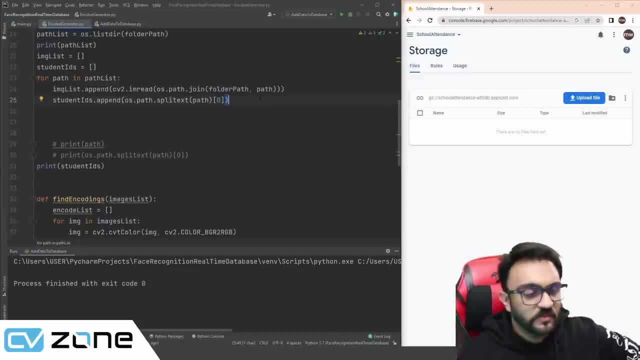 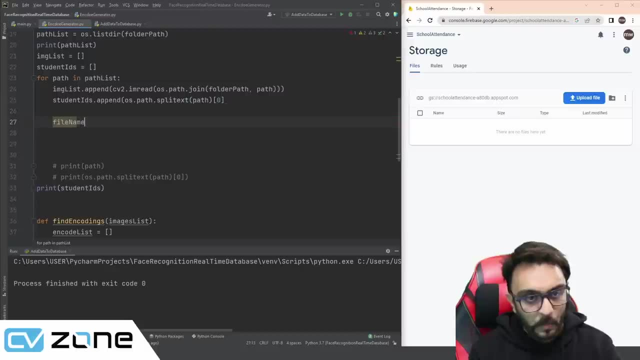 it here? where should we write for path? actually, we can write it here as well. so here we will write five. file name equals. uh, we will write os, dot, path, dot, join, right, and this is the folder path and this is the path. okay, I've removed something from here, so this will give us the file name. 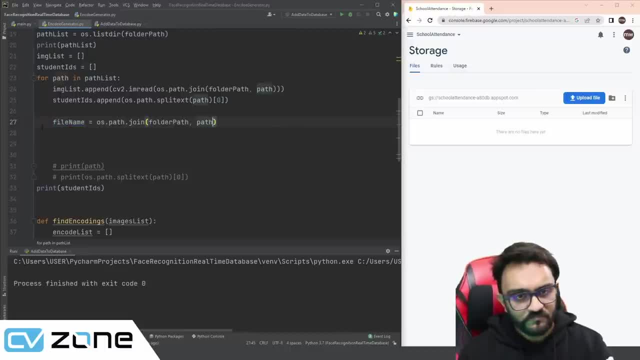 so once we have, uh, the file name, uh, then what we can do is we can create a bucket, so buckets v, u, c, k, et equals storage dot bucket, and then we will write blob. we are going to create a blob to actually send it. blob is equals to bucket dot blob. and here we are going to write the file name. 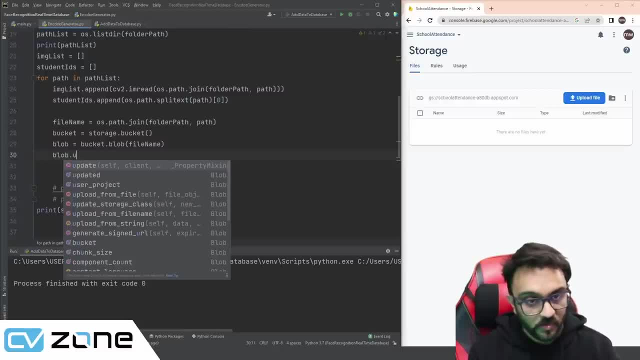 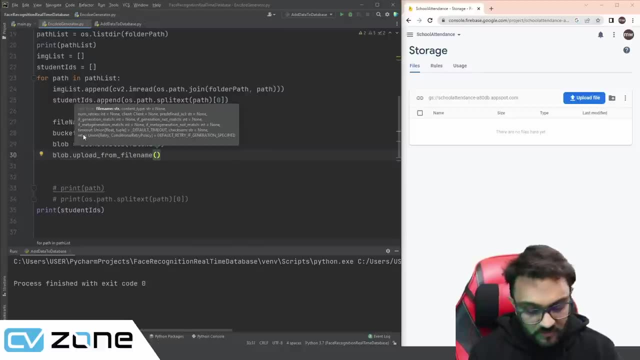 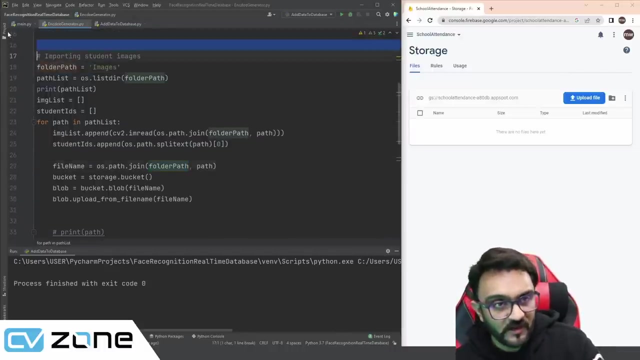 so we will write blob, dot, upload, upload from file name, and then we are going to give in the file name. there we go. so this is going to send the data over here. so what exactly do we need to send? so what it will do is it will create a file, it will create a folder called images, because that 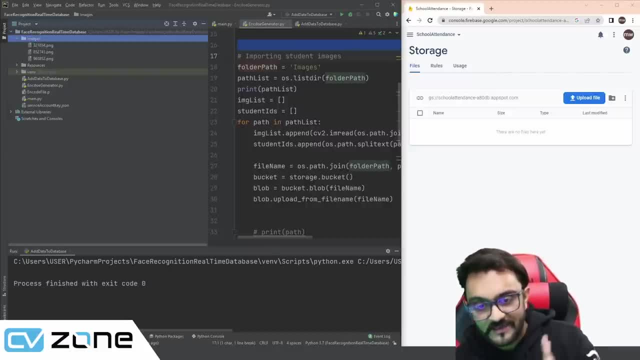 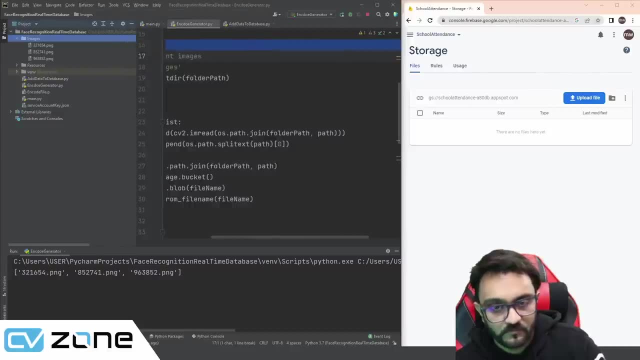 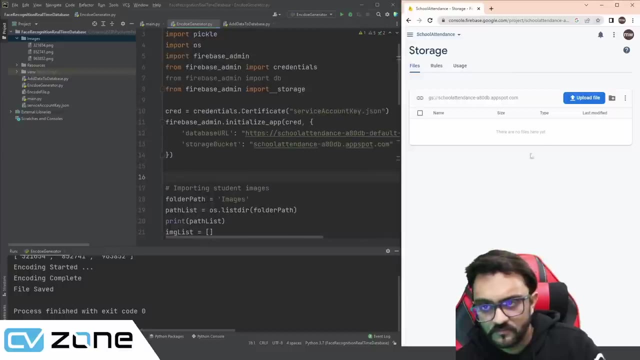 is included in the path, so it will create a folder called images and in that images folder it will add all these images. so if we run the encode generator, did it work? let's refresh, because this is not real time, so you have to refresh. and there you go, so you have. 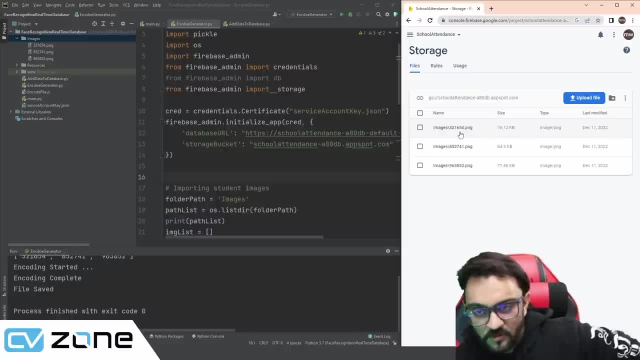 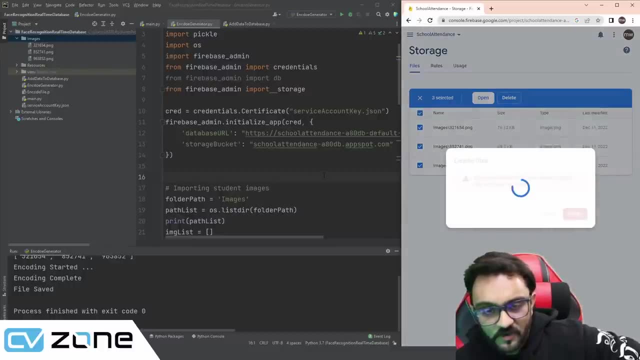 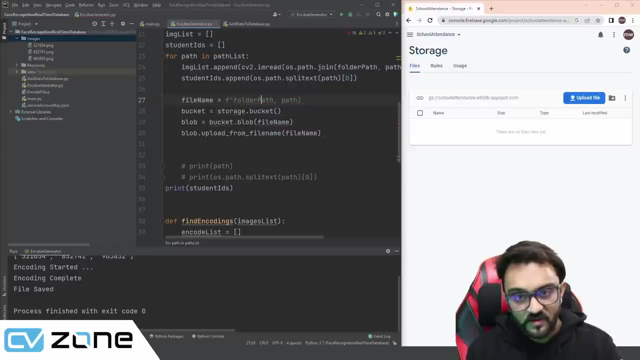 the folder images inside that. you have this or did it do it wrong? i think it did it wrong. uh, no, let's delete all of them and we are manually going to write the will not use osjoin, so here we are going to write f, then this will be within our brackets, then we are going to put slash. 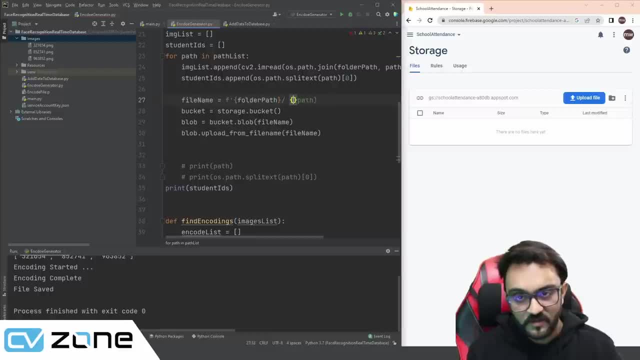 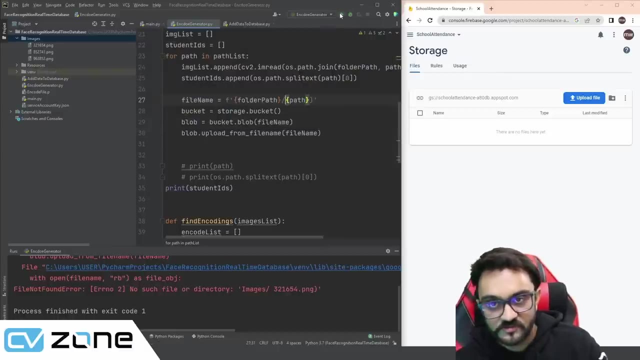 oh, come on, we are going to put slash and then we will have our path. there you go. so, yeah, that should work. now let's run it. uh, okay, there's a space. there should be no space. images slash dot png does not exist. why is that? uh, images dot png. yeah, it does exist. what is the issue? 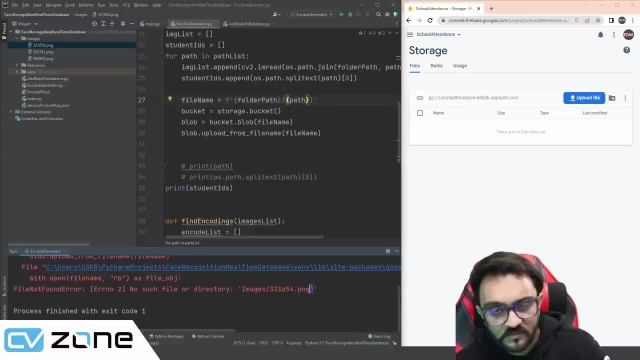 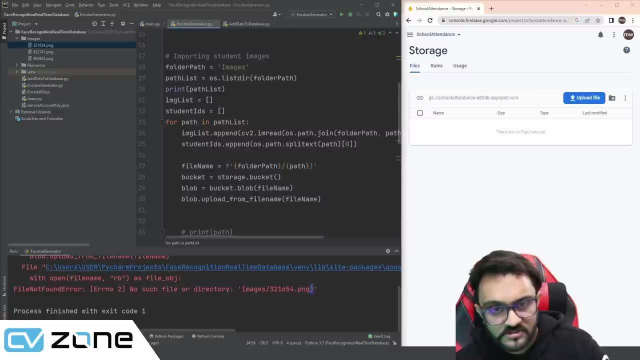 okay, there is a bracket here. why is there a bracket here? something is wrong. why is there a bracket? uh, okay, let's write here: uh, student id, whatever we are getting here. let's try this and we will write manually. oh, okay, okay. okay, my bad, there is this, my bad. okay, let's run that again. and there you go. so no errors and refresh. 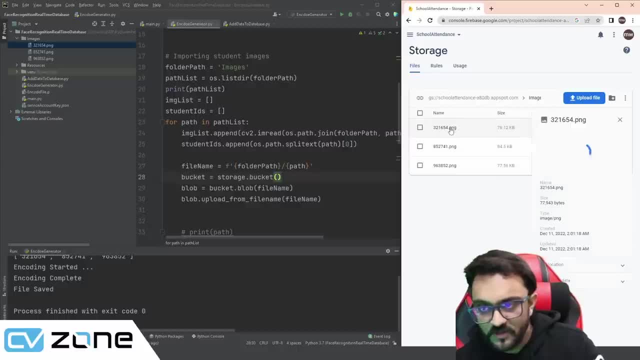 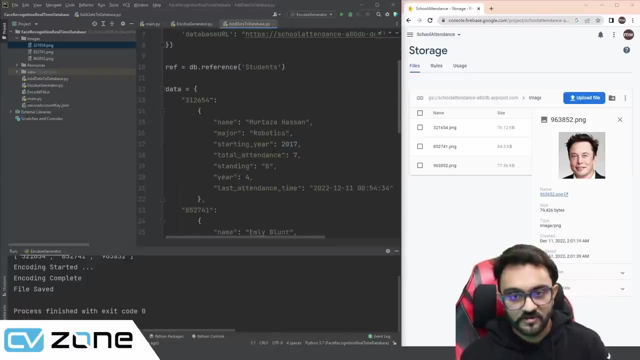 there you go. now we have a folder images. inside that folder we have all these images. so these images we have uploaded and then we can download them whenever we require them. whenever the face is detected, we can download the specific image and then we can use it in real time. 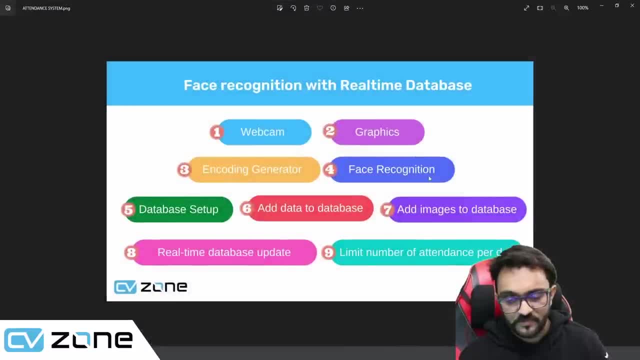 so how can we do that? let's look at the next step: add images to database. we have done that. now we need to update the database in real time whenever the attendance is increased, and we need to fetch all the data from the real-time database and add it to our graphics. so let's 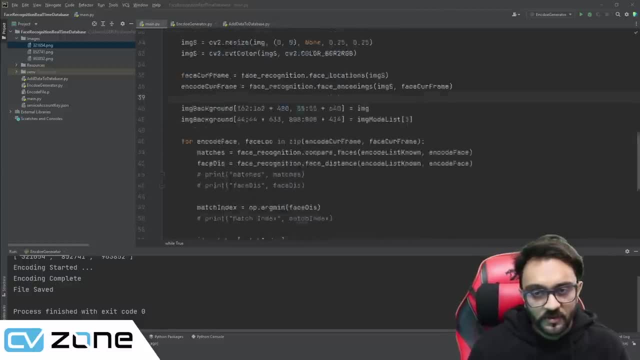 go ahead and do that. so here in our main file, let's go ahead and do that. so here in our main file, let's go ahead and do that. so here in our main file, we are going to do, we are going to add the code for the database. so we will go to the encode. 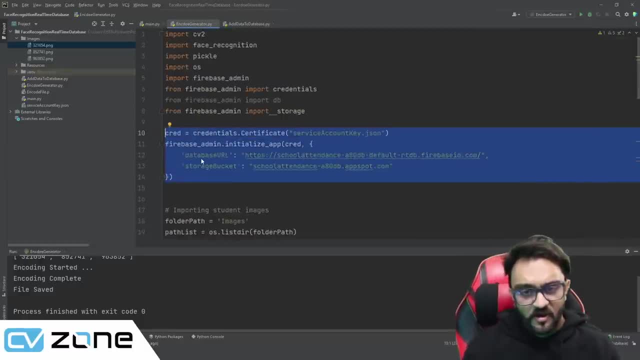 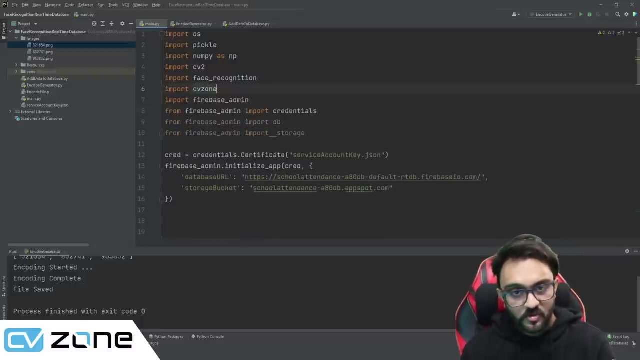 generator. so we need the credentials for the database and we need the credentials for the storage bucket. so we will copy both of both of those. actually, let's just copy all of this and we'll go to main and we are going to paste it here. so now we have our storage storage and we have our 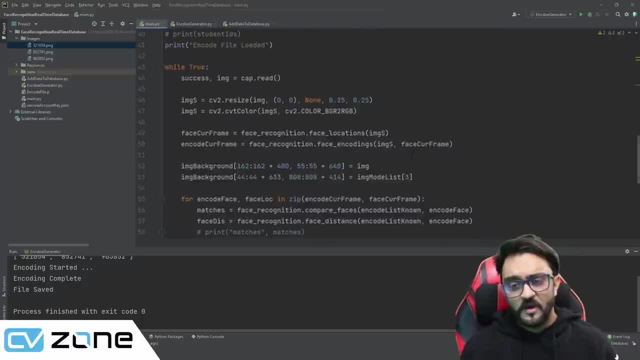 database url as well. so now what happens is that once you detect the face, once you recognize the face and we know that it has been detected correctly, now we will fetch the data, we will download the data from our database, the real-time database, and then we are going to display it. 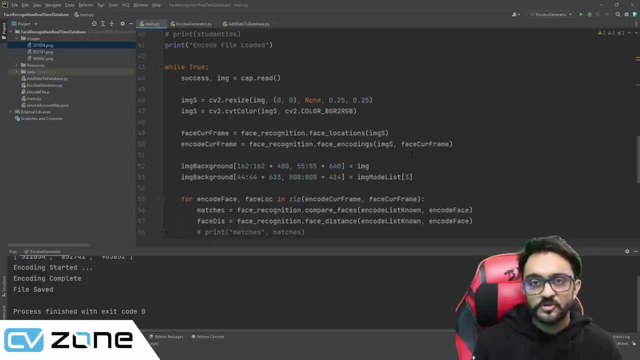 for a few seconds. once it is done, we are going to show marked for a few seconds and then we will go back to active. so this is how it will work, and then we will go back to active. so this is how it will work. so if we open this up in explorer, 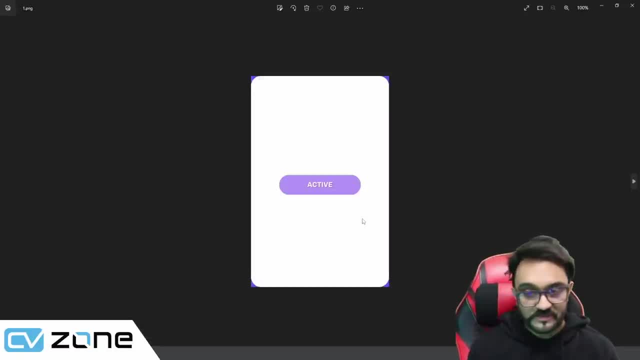 so the first thing will happen is it will show active. right now it's active. then, when it is detected, it will download the data, it will put it on this and then display it, and then, once it's done, we will wait for a few seconds, maybe one or two seconds. 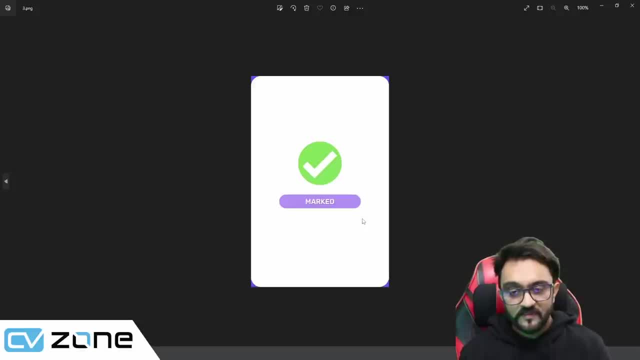 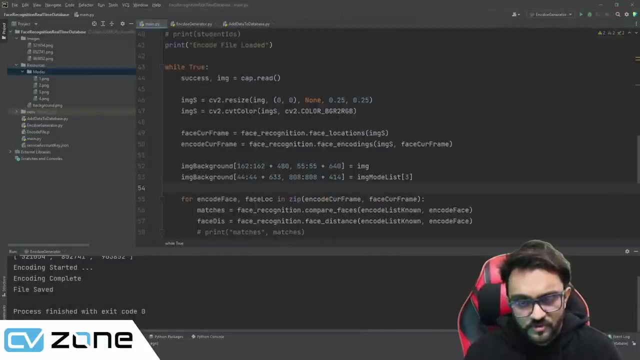 and then after that we will show marked and then once it is marked, we will go back to active and then if the student comes back again, then we will say: already marked, you don't have to mark it again. so, uh, the first thing is that we have to show that it is active. so to show that, 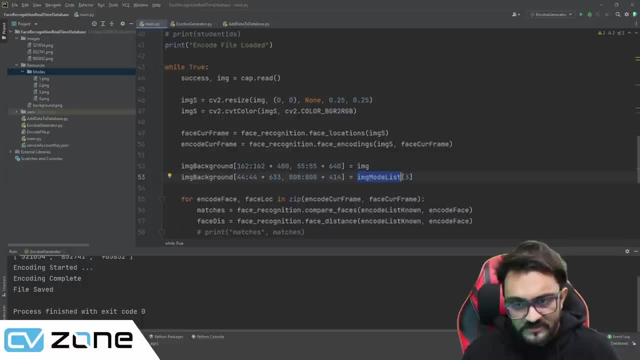 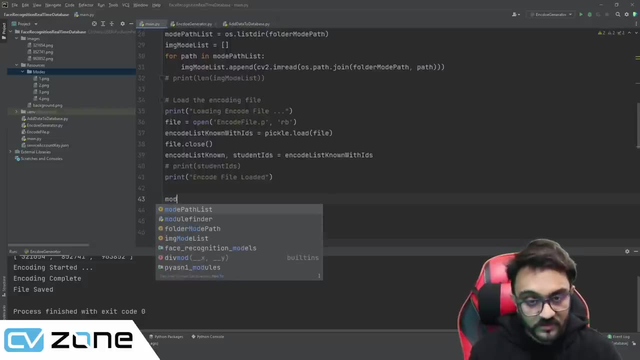 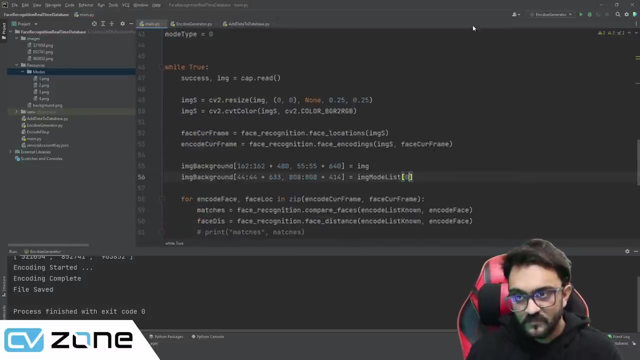 we will simply write image mode list. we will write here mode type. so here we are going to create a new variable. we'll call it: mode type equals zero. so when it is zero it will show that it is active. so if we run this now, we will see that it is active. so if i run this now, if i run the main, 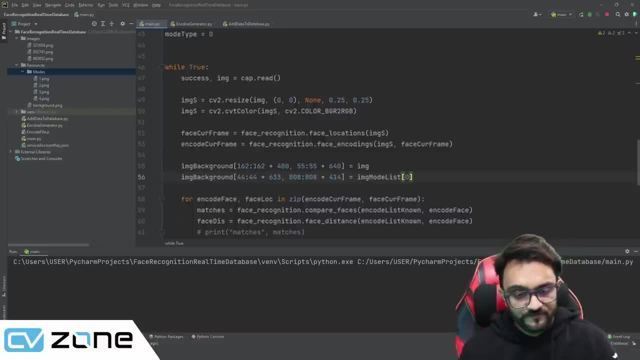 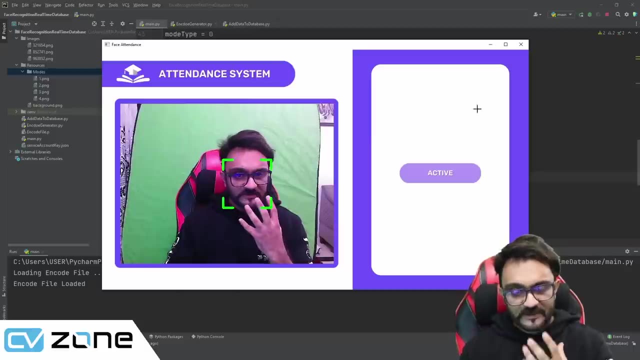 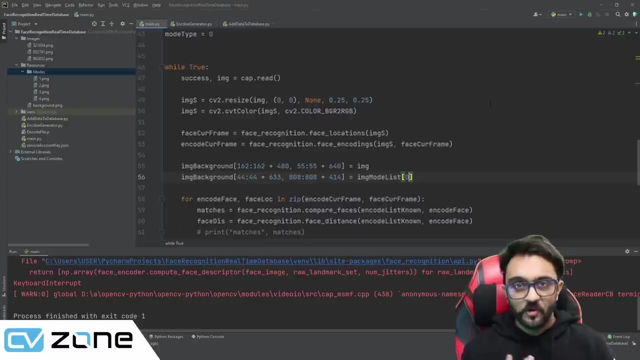 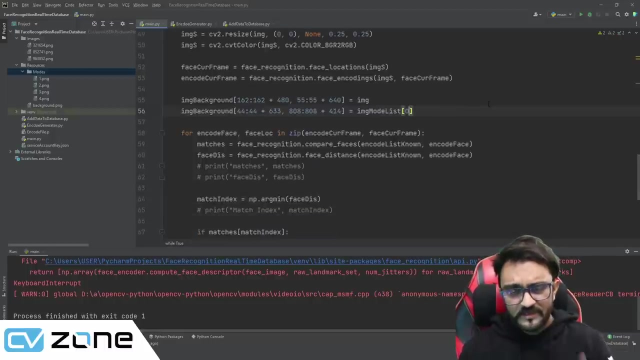 it is supposed to show us active, there you go. so it is showing us that it is active once the face is detected. we only need to download the information in the first frame. we cannot keep downloading because it will be very inefficient, so we have to download it only once in the first frame and then we will see that it is. 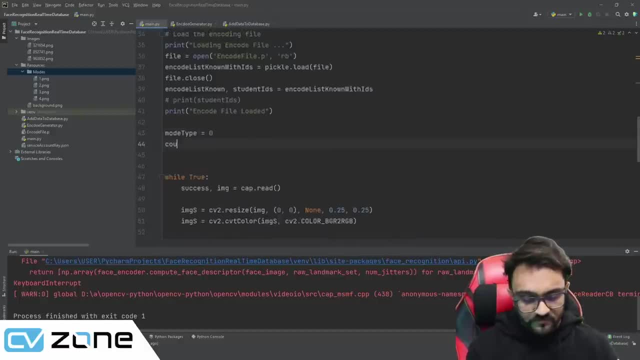 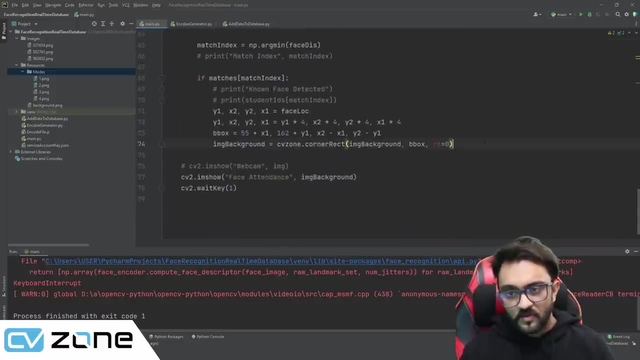 active in the first iteration. so to do that, we are going to add a counter. so counter equals zero. so once we detect it, we are going to write that if the counter- i'm writing it in english- if the counter equals zero, if the counter is zero, then make the counter equals one. 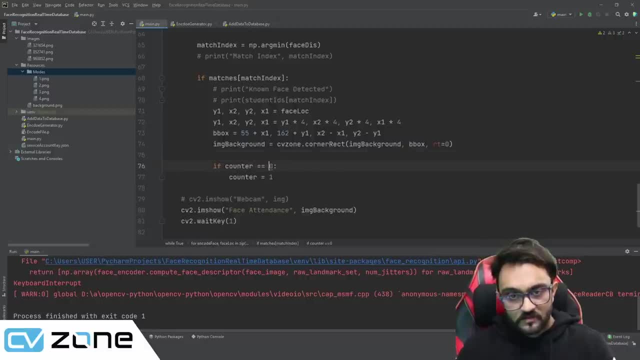 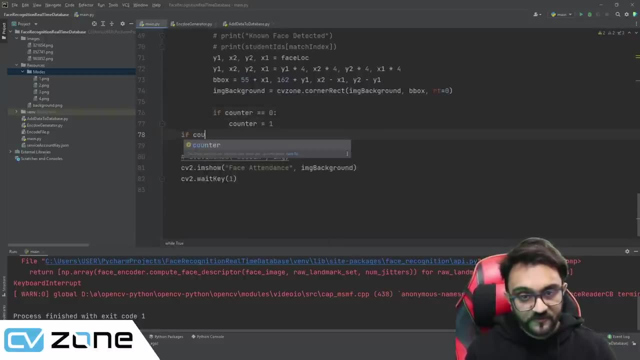 so if it was previously zero, make it one right. so that is the main idea, and once it is one, here we will check. if counter is not equals to zero, then we are going to do something. then we will write: counter plus equals one, so it will keep. 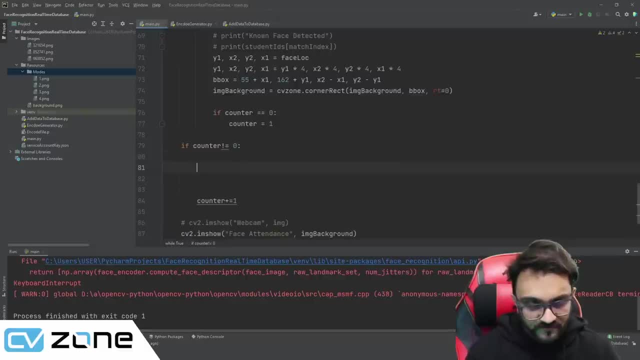 counting. so for the first frame, for the very first frame, we are going to say: if counter equals one, that is the first frame, then what is happening? then we are going to download all the data. we will download it and we will show it at the same time. so how can we download it? 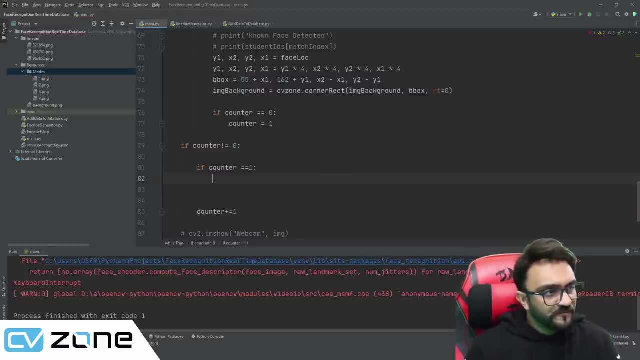 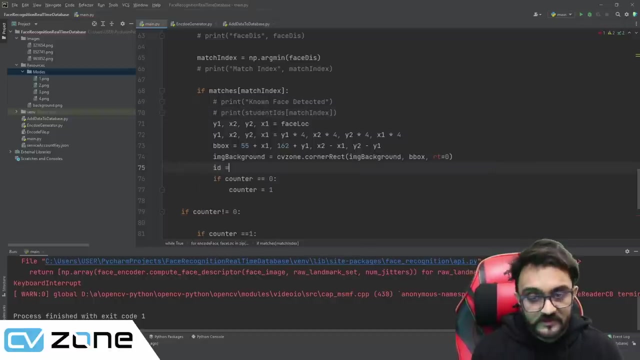 it's very simple. first of all, we need to find the information of the student. once we get it, so we are going to save it in an id. so here we are going to call it. id equals- uh, what was it? id equals student ids, ids at match index. 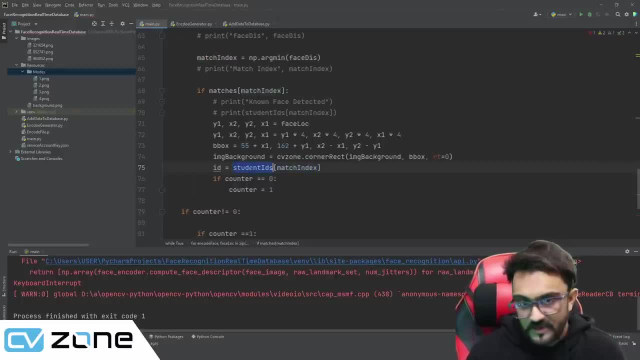 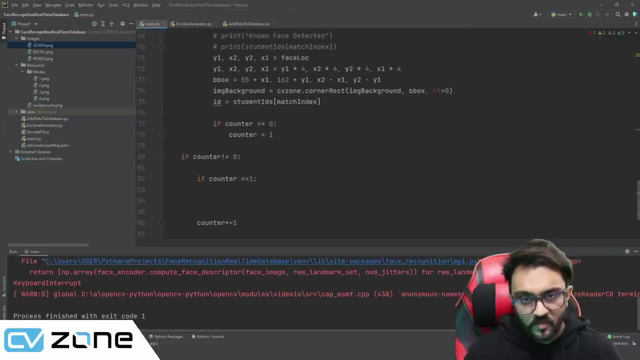 so, uh, whatever index was matched, we need the id for that. so this is our id. for example, it will be 321654, it will be saved. so if, if you want to make sure that we have an id, you can put 0 over here and then it, once it gets it, it will show an id. it will show it. so we smoothen it. and if you schneider b ii, it will. 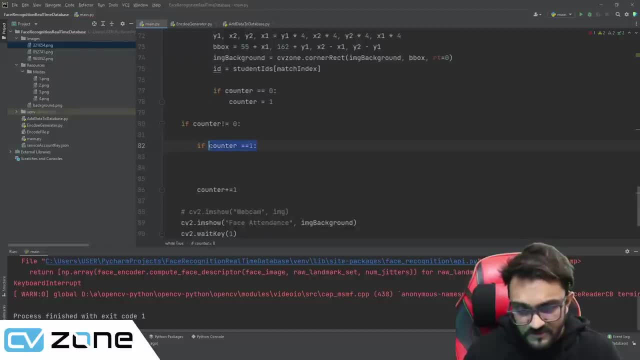 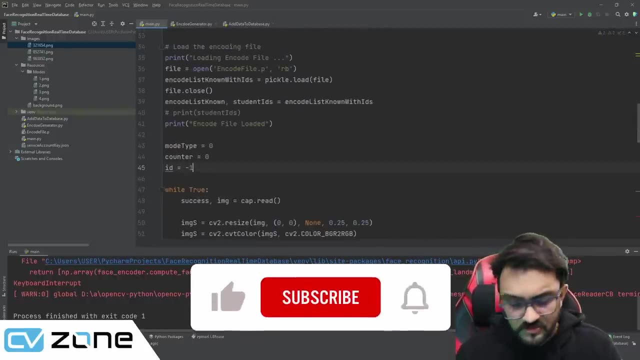 either match or beessenland. so whatever is matched, you can put 0 after that and then it. once it gets it, it will show an id and once we have the first iteration, we are going to use that id number to get. actually. let's write minus one, because zero is also an id, yeah, so here we are going to write: counter is one. 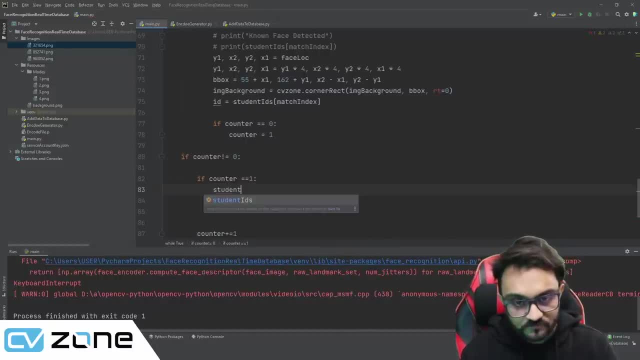 then we are going to write students info equals. this is the part where we are going to download. so how can we download? we will create a reference, we will write db dot reference and in this reference we are going to give a string. we know that the first one will be students. so this is. 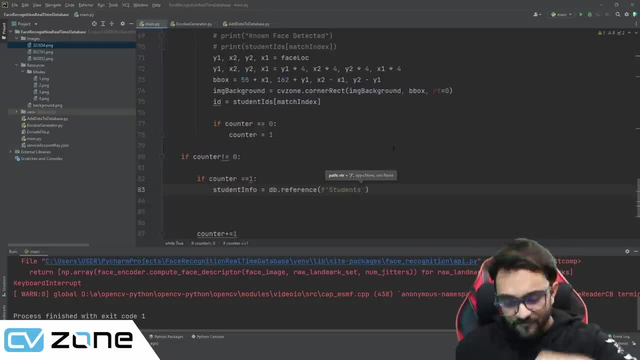 our main path, the main folder. in that folder we need to get the information of the student and inside that we have an id. so this id is the one that we got, so we need that id and and then, once we have that, we want all the information of that right. so here we are going. 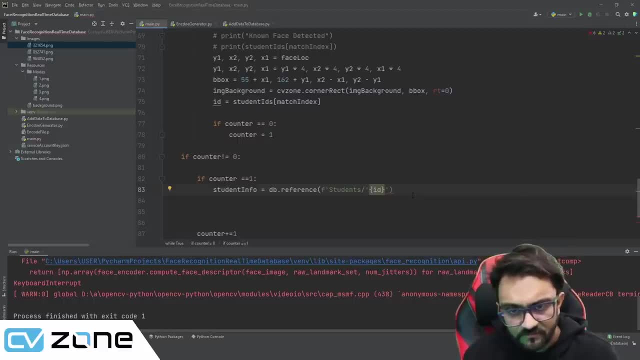 to write what's what's going on. why is it like that? oh there, there needs to be another one. no students id. why is this here? sorry then. uh, what we need, we need to get dot, get that's it. so we need to get all the information. so here we will print it out. 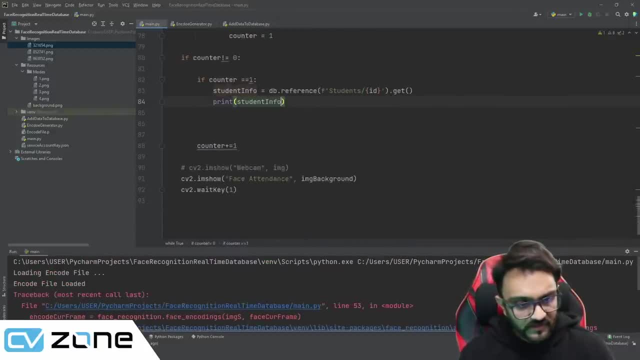 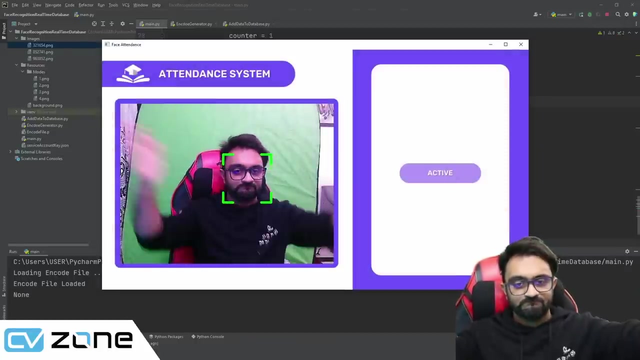 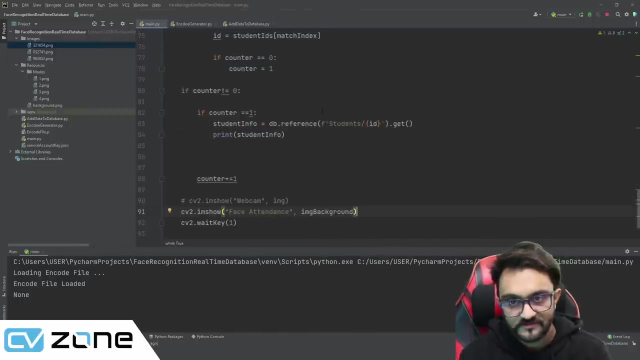 the student info. are we printing anything else? nothing, okay, so only on the first frame. it is going to download all the information and let's see if it downloads correctly. there you go. it has downloaded none. excellent, so there is a mistake somewhere. db reference: is it student or students? 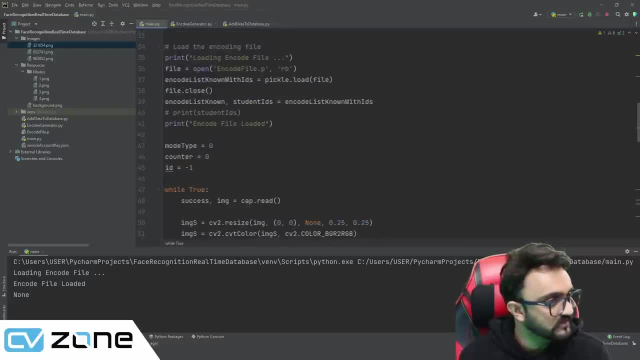 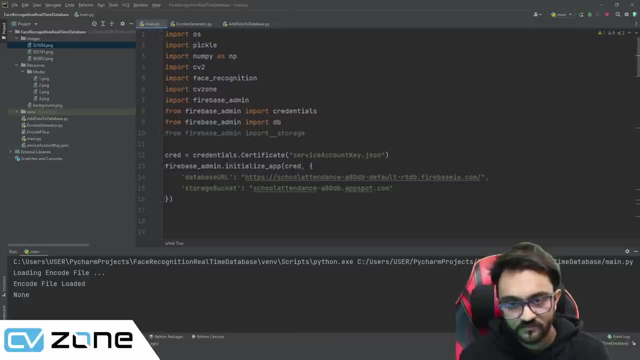 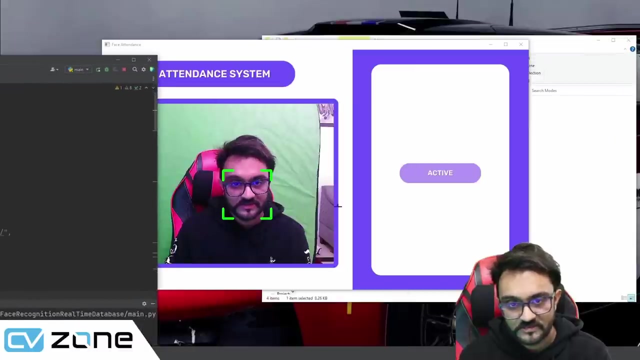 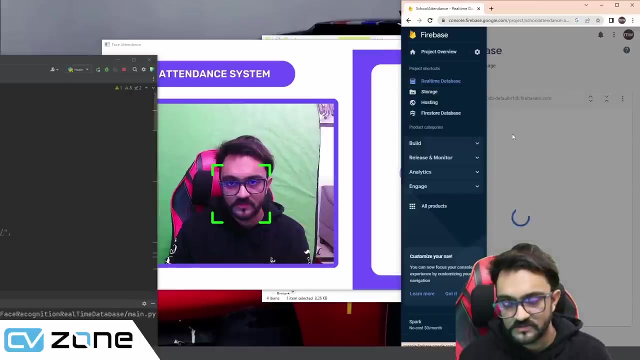 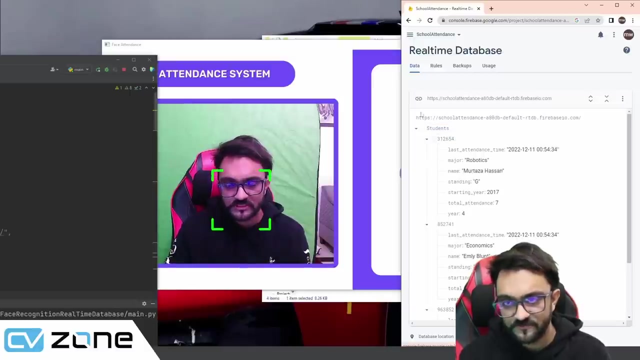 um, do we need to give any reference other than that? not really, okay, let me check again this part. is it students or student? we need to check that in the database. so in the real-time database it is students one, two, six, five, four. maybe the id is wrong. let's check the id first. 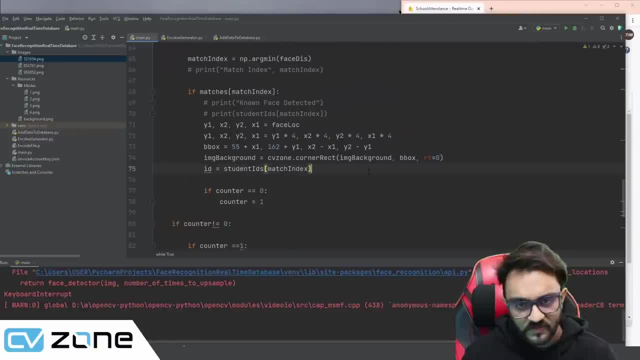 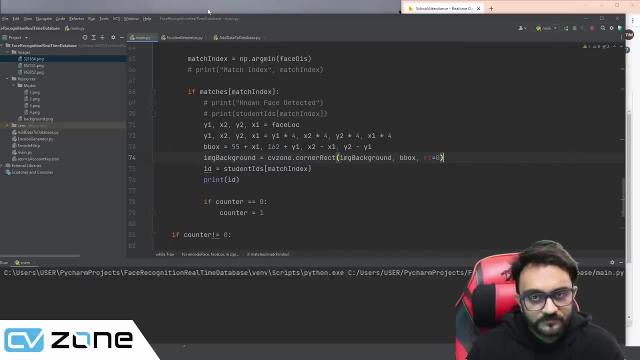 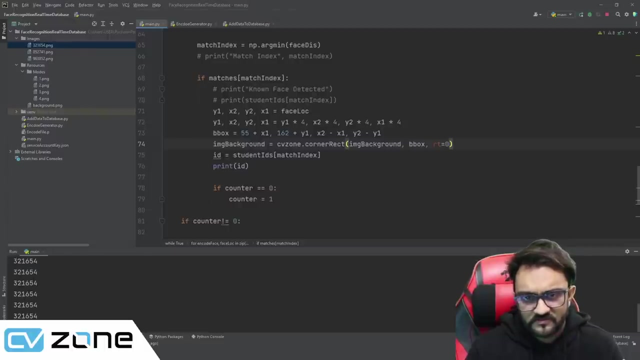 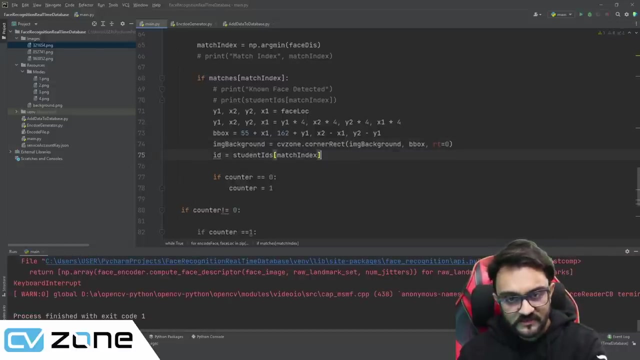 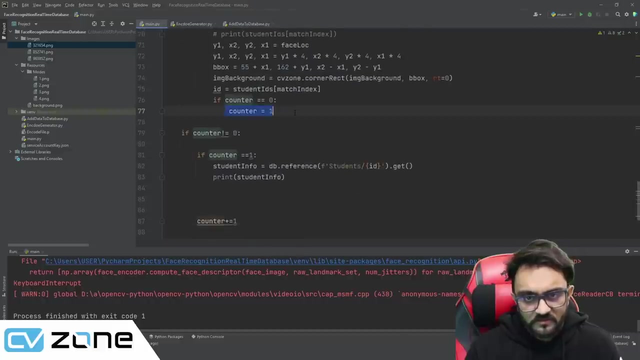 uh, so here, once we are getting the id, we are going to print it out, prints id three, two, one, six, five, four. it is correct, the id is correct. so once we have this id, if counter equals zero- which it is, counter is zero, then it makes counter one. if counter is not equal zero, where is this? yeah, it's in the right. 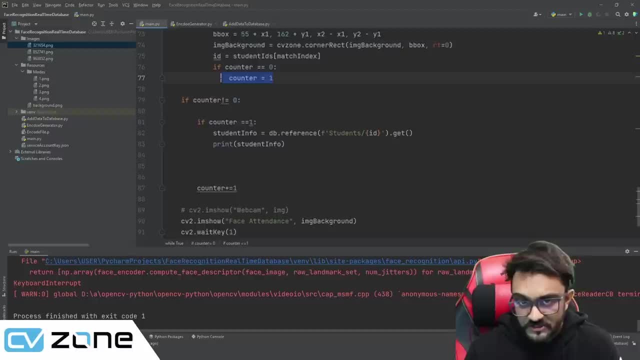 loop. if counter equals one, which it is, then student info equals db dot reference f. students slash id dot gets f students slash id dot get. forget that is the eposu we are adding at the total. well, i am going to automatic. kırm is going to have to send this in this stuart ns. student dot reference f students slash id dot get. 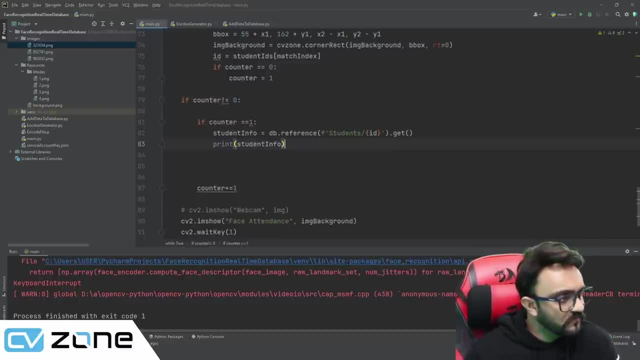 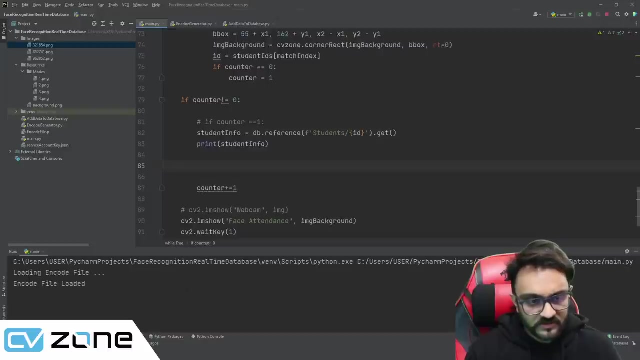 What is the issue over here? Okay, let's just remove this And we are going to go back and let's see if this works. Is it only for the first frame, or does it recognize the data at all? None, So the student ID was what? 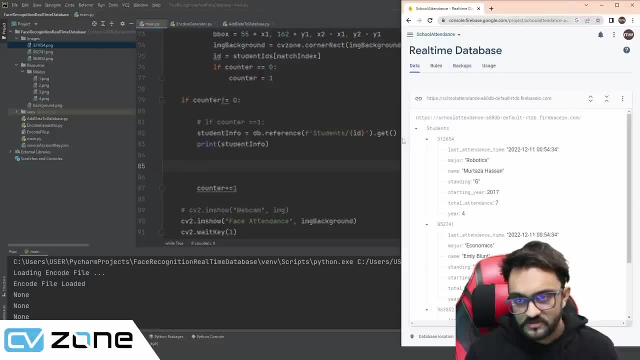 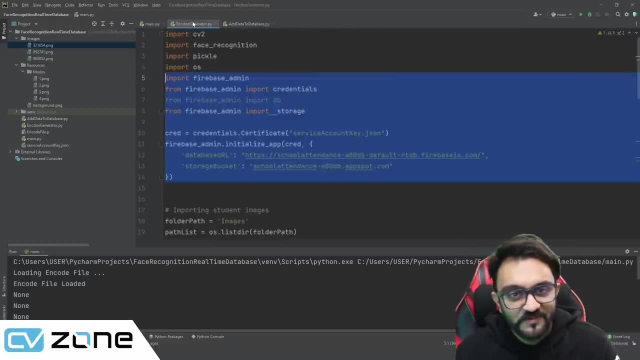 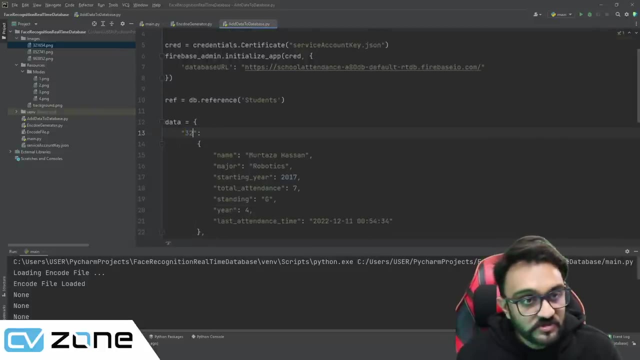 321654.. And over here it's 312.. Oh, oh, that's the okay. so that's the problem. The problem is my typing. So the data where we added the data, I wrote this wrong: 321654.. 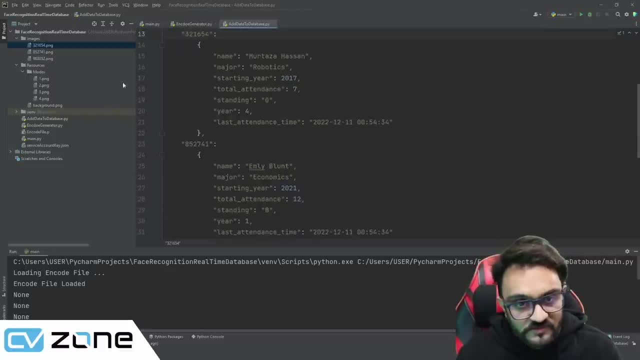 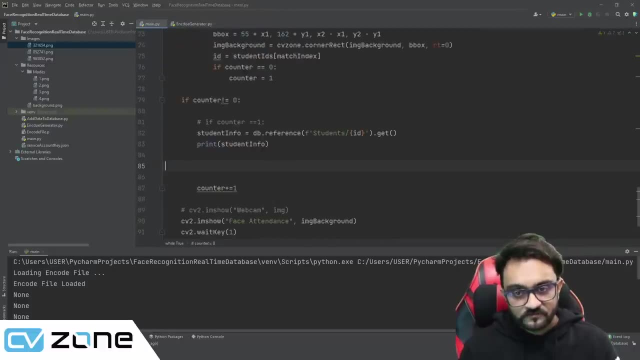 That was the digits. So 852741,, that is correct- 963852.. Okay, So this is fine. now, Actually, we need to do this again. We need to run it. We need to run this because I changed it here. 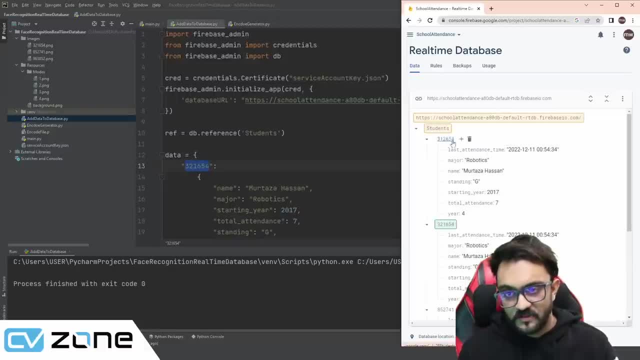 So let's run that. Let's see if it updates here. There you go, It's updated. So these are now two different students, So we are going to remove this one. So there you go, We have now the correct student. 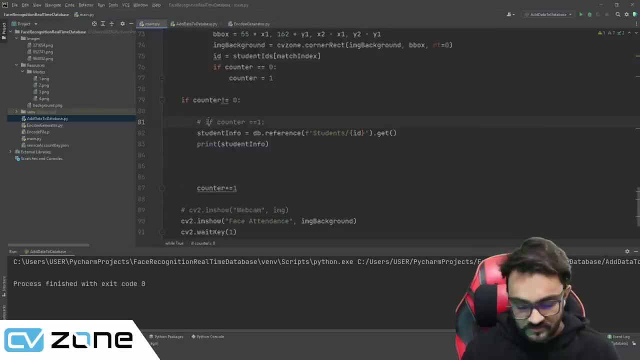 And if we go to main, and I think we can put this, it should work fine. So if we run that now, we should get this. So let's run the main again. There you go, So last time. attendance: major name: standing starting year. total attendance year number. 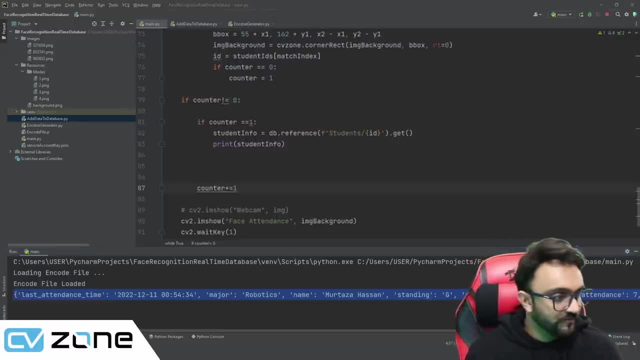 everything. we are getting it directly from our database, So that's perfect. That is exactly what we wanted, And we have it in the first frame only, And in the first frame only, we are going to update, But before we do that, we need to change. 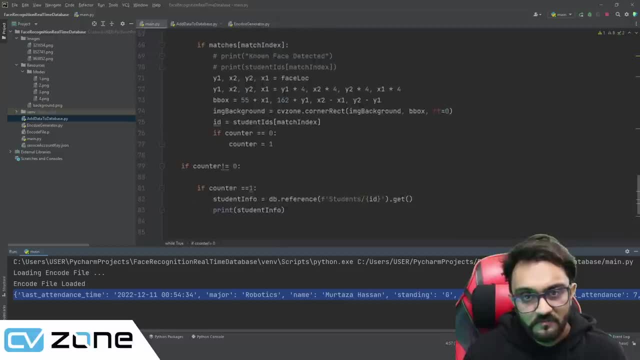 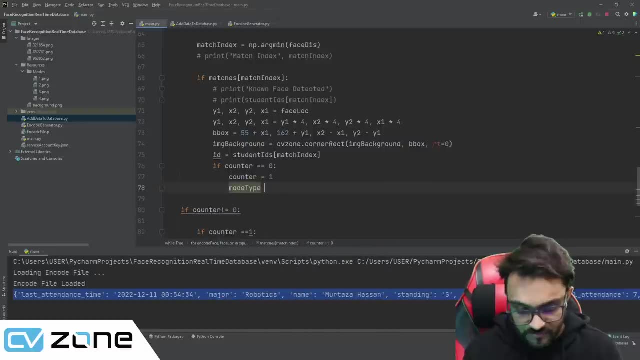 We need to change the image, We need to change the mode, So we will make the mode type equals 1.. So here we are going to write: mode type equals 1.. Because we need to update the mode, which will go over here. 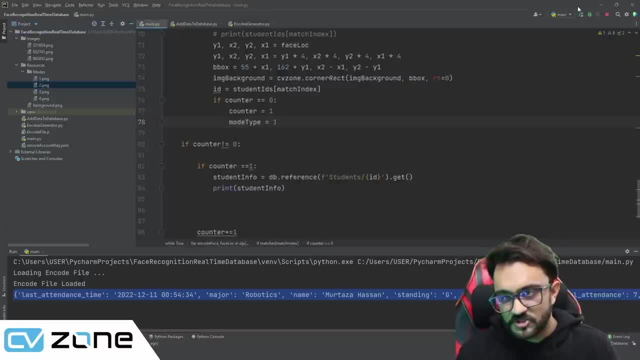 So once it is mode type 1, but will it show before or after? We'll have to check. I'll tell you what I mean by that, But let's just try it now. So once we have the student info, 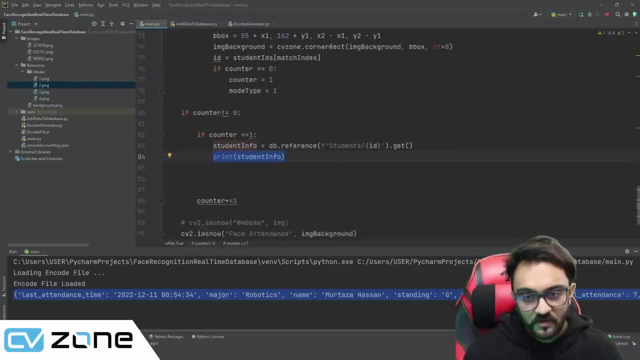 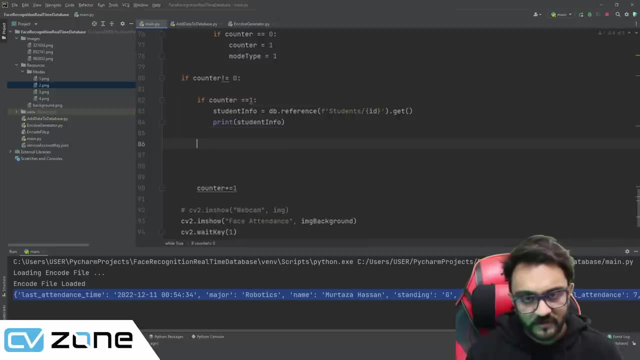 All we have to do is we have to put it in the correct areas. So how can we do that? So we can do that by writing here. Now, this should not only be displayed when the counter is 1. It should be displayed at 2,, 3,, 4,, 5,, 6, and so on. 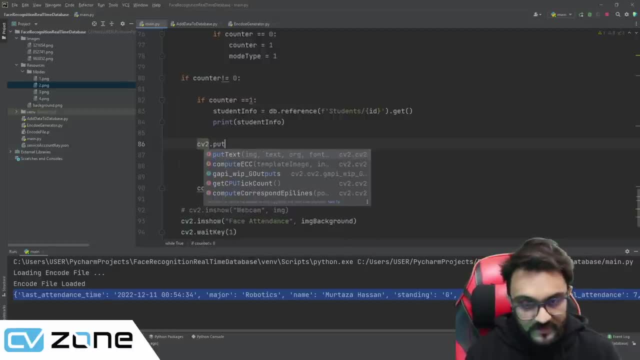 So what? we will write here cv2.puttext, And we have to put it on the image background And then we have to put in the string. What exactly is the string? The string will be student info. At what information? 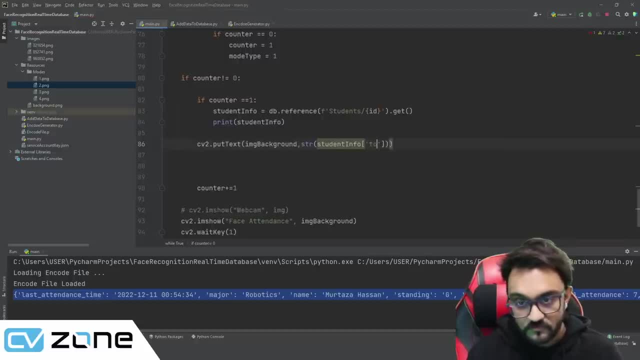 The information let's say is total attendance. Total Because this is a dictionary. you can just reference it like this: Total underscore attendance, And that's how you can get it. So total attendance is this, And then you have to give in the location. 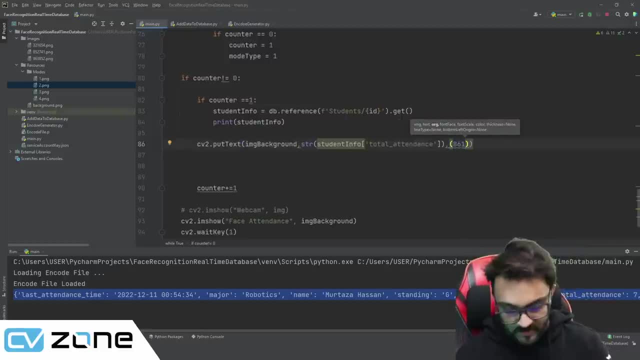 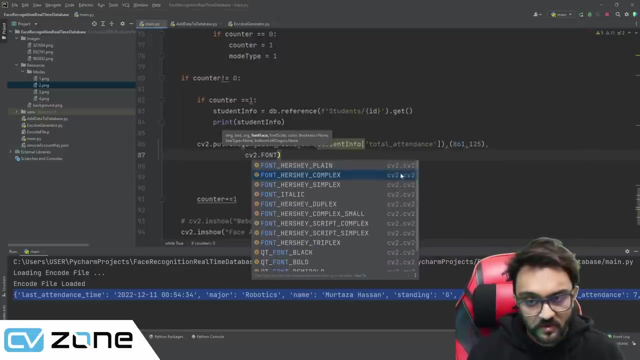 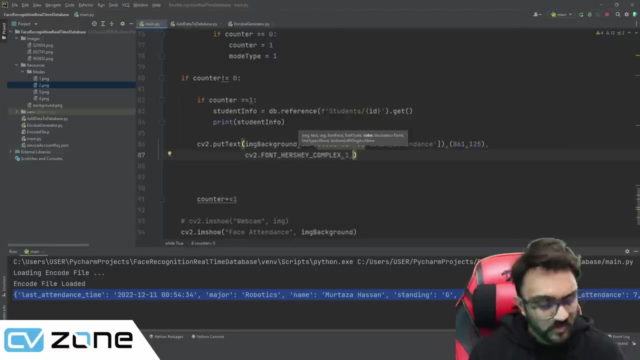 So location? I have already checked: It's 861 and 125.. For this particular text, Then we will give in cv2.fonthersheycomplex, And then we will give in the size, which is 1.. And then we will give in the color, which is 255,, 255, and 255, which means white. 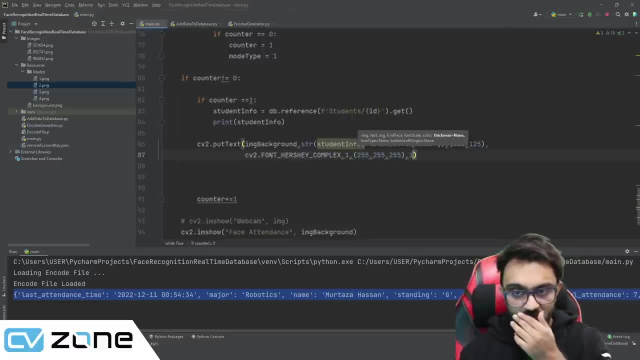 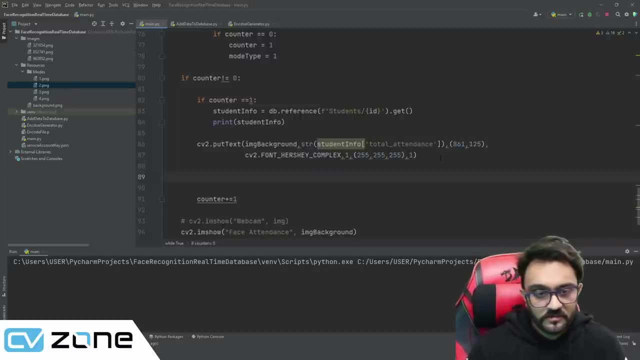 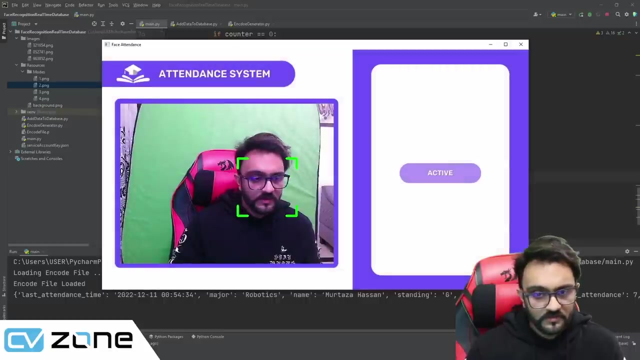 And then we will give in the thickness, which is 1.. So if we, So if we run this now, we should get the total attendance. Okay, we are not getting anything. Why is that? So here we have changed the mode to 1.. 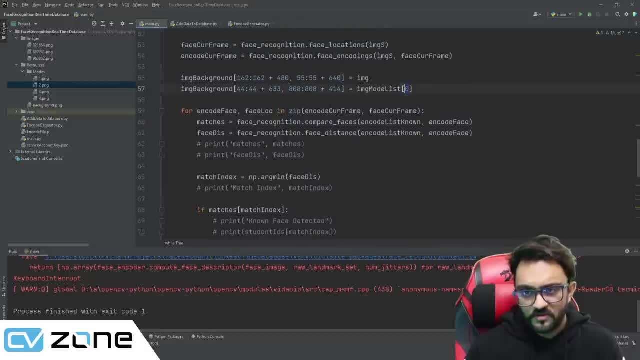 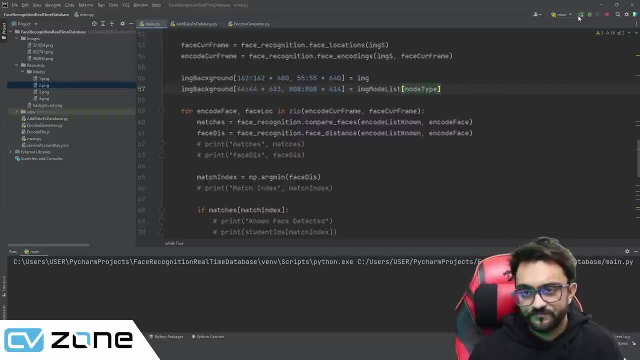 Mode type is 1.. So over here, Oh, it's 0.. Why did I put 0? Here it should be mode type. So that's why, dynamically it should change. So let's run that. So let's run that. 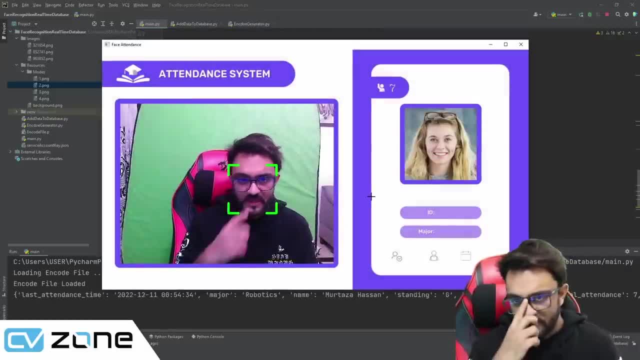 And there you go. So this is First it was active And now it is. The mode type is 2,, where it shows all the details, And here you can see it shows 7.. So the total attendance is 7.. 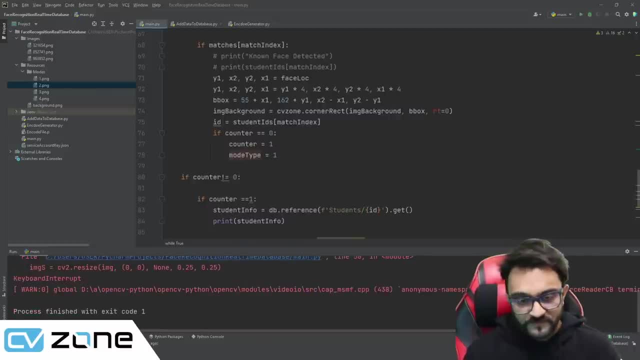 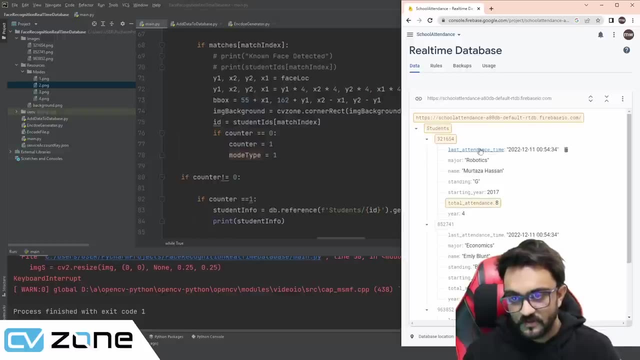 And it has taken it from our database. Now, to prove this, that it has taken from our database, we will change this total attendance. We will click on it. We will change it to 8.. so now my attendance has changed. if I click on this now, it should give me the. 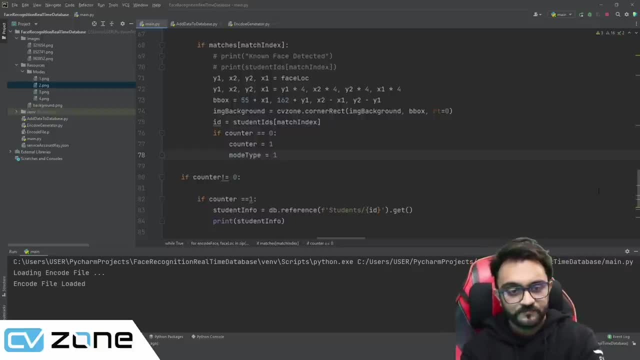 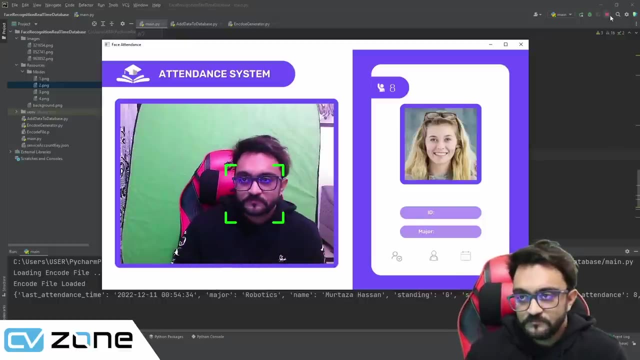 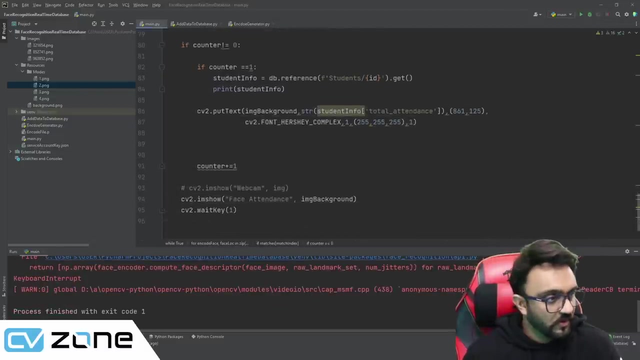 updated attendance number, which is 8. there you go. so now it's showing me the attendance number as 8. so this is all good. now we have to add it to all the other. what do you call values? so here we have to add name. so I will copy this. 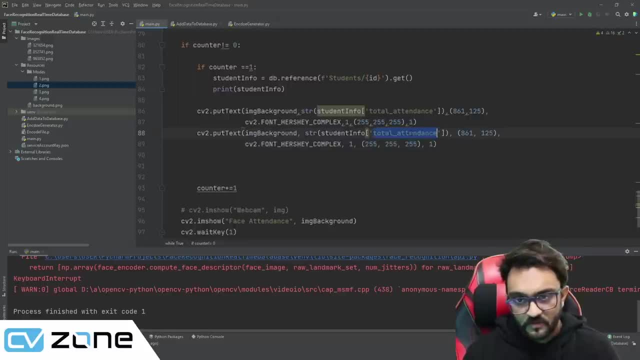 paste it here. we will just change it to name and for the values, the values. it is 808 and 445. now the name is a little bit tricky because the the length changes a lot. we have to Center it and we have to Center it automatically. so I will tell. 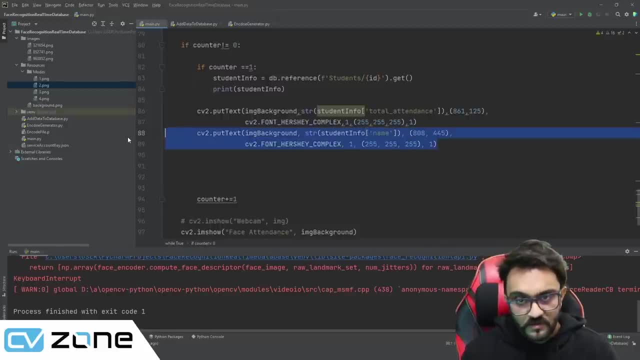 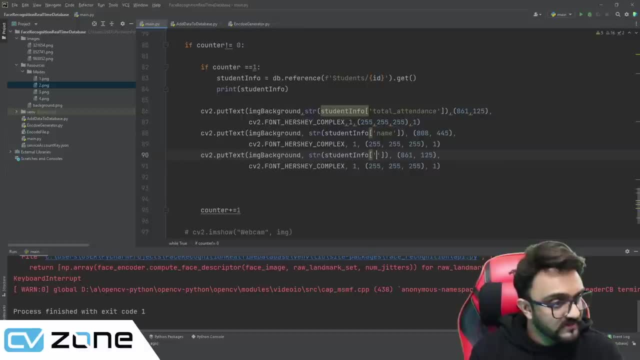 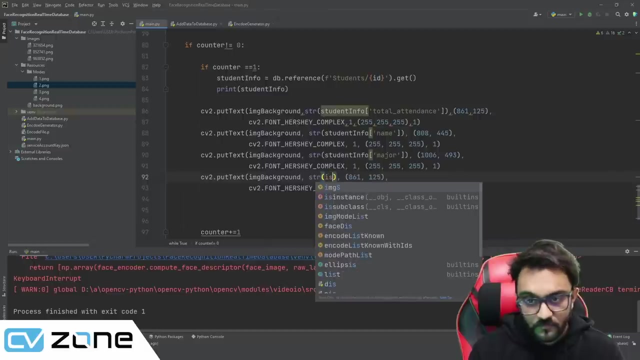 add. let's add major. so the major is 1, 0, 0, 6 and 493. then we are going to add: let's say the ID. so here we will write ID. the ID is at where is it. say the ID. so here we will write ID. the ID is at, where is it? 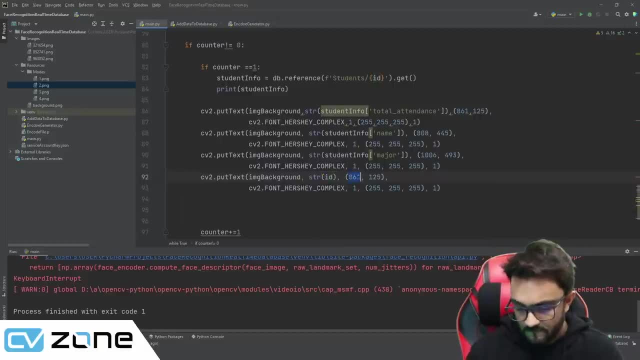 say the ID. so here we will write ID. the ID is at. where is it? 1 0 0, 6. 1 0, 0, 6 and 493. okay, I wrote 1 0 0, 6. 1 0, 0, 6 and 493. okay, I wrote. 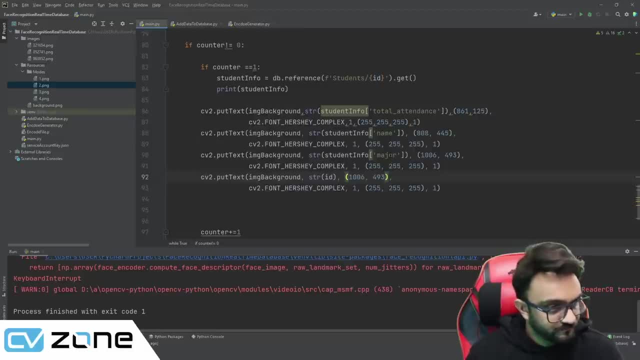 1 0 0, 6, 1 0, 6 and 493. okay, I wrote one of them wrong. major is supposed to be 1 0 0. one of them wrong. major is supposed to be 1 0 0, 6 and 5 5 0. my bad. and then we are. 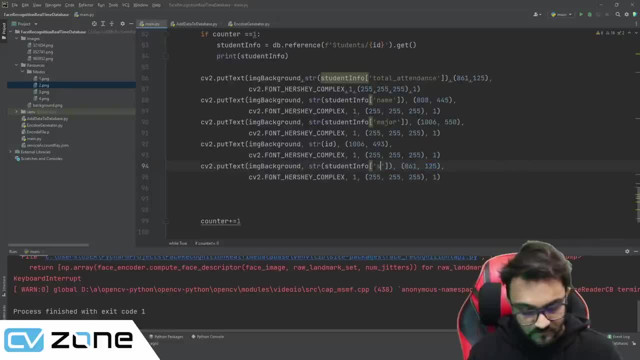 one of them wrong. major is supposed to be 1 0, 0, 6 and 5 5 0, my bad. and then we are one of them wrong. major is supposed to be 1 0, 0, 6 and 5 5 0, my bad. and then we are going to write after major, the standing. 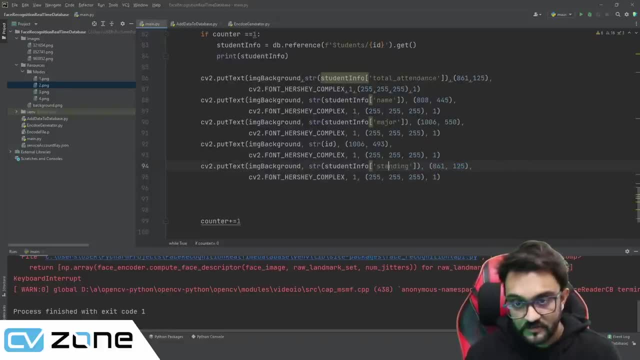 going to write after major the standing. going to write after major the standing: standing: standing. standing standing is 9 1 0 and 6 to 5 is 9 1 0 and 6 to 5 is 9 1 0 and 6 to 5. then we have to write here: here is 1 0, 2, 5. 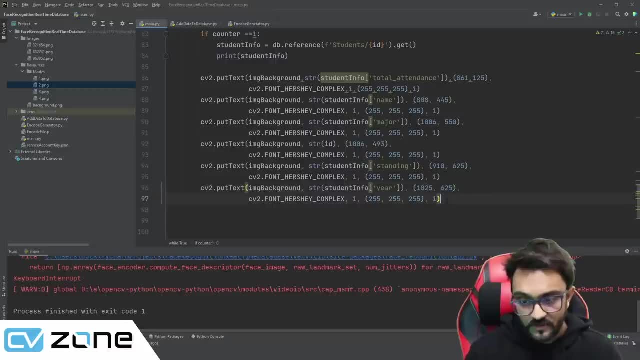 then we have to write: here: here is 1, 0, 2, 5. then we have to write: here: here is 1, 0, 2, 5 and 6 to 5, and then we have to write and 6 to 5, and then we have to write. 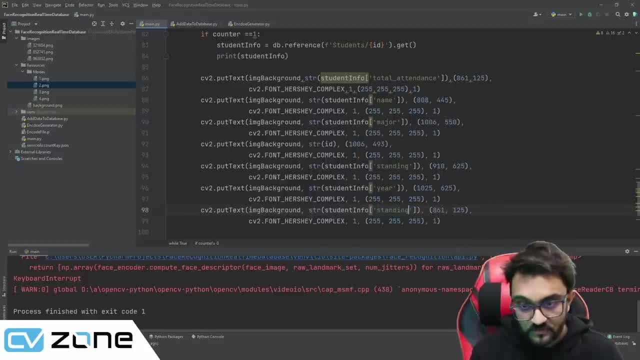 and 6 to 5. and then we have to write: standing here, standing, standing here, standing standing here, standing, starting here. sorry, what is wrong with starting here? sorry, what is wrong with starting here, sorry, what is wrong with me today starting here? so starting me today, starting here. so starting here is 1, 1, 2, 5 and 6 to 5. 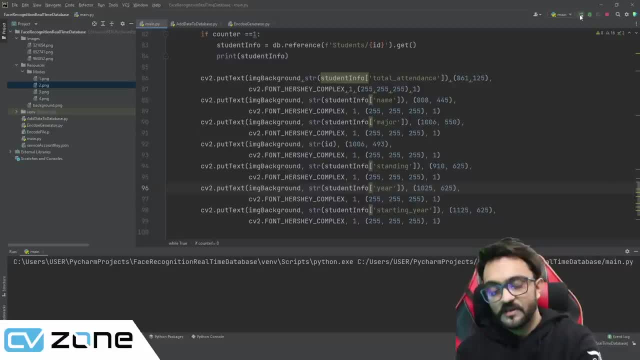 here is 1, 1, 2, 5 and 6 to 5. here is 1, 1, 2, 5 and 6 to 5. so let's run this and see if we are getting. so. let's run this and see if we are getting. 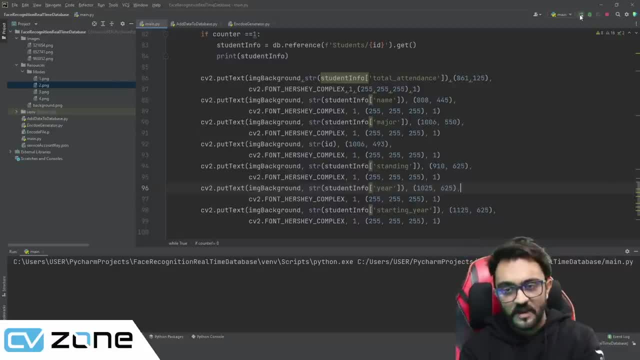 so let's run this and see if we are getting all the positions correct, except all the positions correct, except all the positions correct, except for the name. i'm going to tell you how. for the name. i'm going to tell you how for the name. i'm going to tell you how you can. 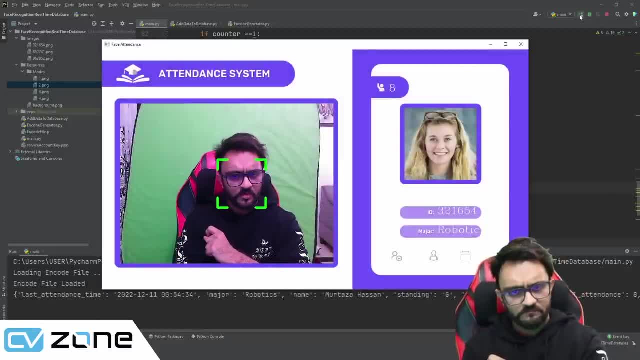 you can. you can write the name as well. uh okay, write the name as well. uh okay, write the name as well. uh okay, the the sizes are wrong, the the sizes are wrong, the the sizes are wrong, and i believe the colors are wrong as. and i believe the colors are wrong as. 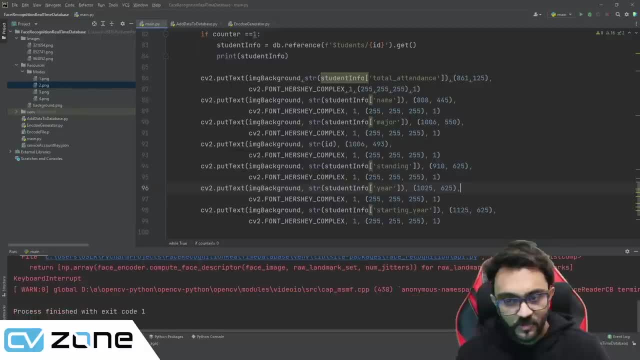 and i believe the colors are wrong as well, because we can't put white here. well, because we can't put white here. well, because we can't put white here, let's put hundred, let's put hundred, let's put hundred, hundred and hundred. hundred and hundred, hundred and hundred. let's copy that. 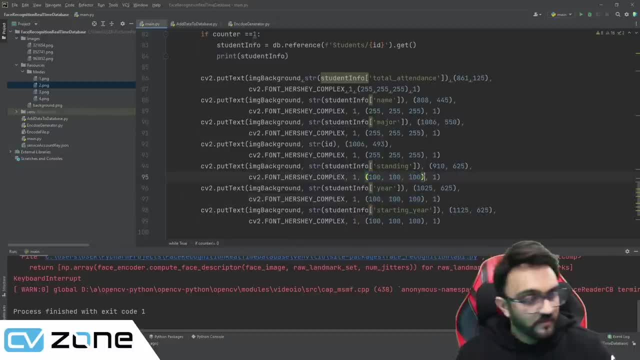 let's copy that. let's copy that and we'll paste it here, and we'll paste it here, and we'll paste it here. and paste it here for the sizing for the and paste it here for the sizing for the and paste it here for the sizing for the last three. it is 0.6. 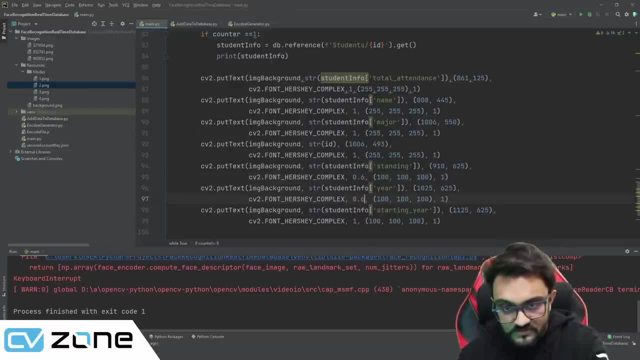 last three, it is 0.6. last three, it is 0.6, 0.6, 0.6, 0.6, 0.6 and 0.6, 0.6 and 0.6, 0.6 and 0.6 and uh, for the ones before, that is 0.5. 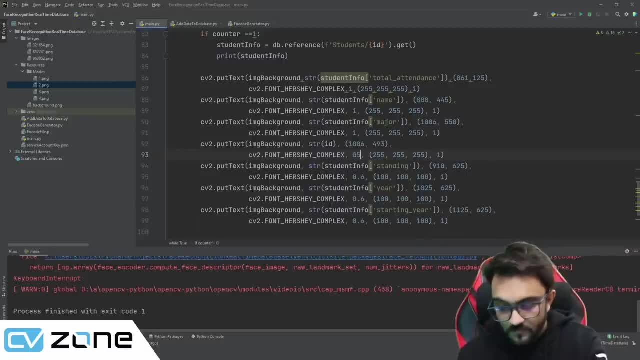 and uh for the ones before that is 0.5 and uh for the ones before that is 0.5 and 0.5, and 0.5 and 0.5 is for major and the colors. the colors is for major and the colors, the colors. 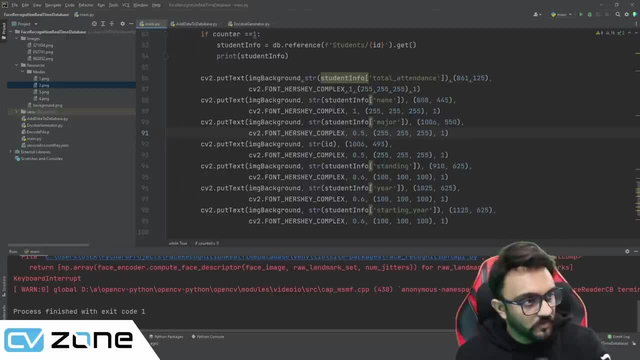 is for major. and the colors: the colors are same. i believe are same. i believe are same. i believe, yeah. and one more thing: we have to, yeah, and one more thing, we have to, yeah. and one more thing: we have to change the name, change the name, change the name. the name again will be: uh, we'll make it a. 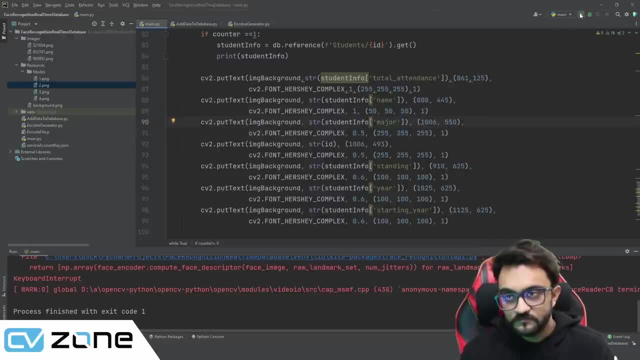 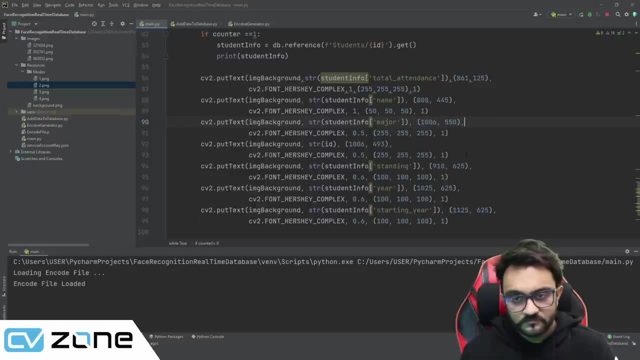 the name again will be: uh, we'll make it a. the name again will be: uh, we'll make it a little bit darker: 50, 50, 50.. little bit darker: 50, 50, 50.. little bit darker: 50, 50, 50.. so let's run that. 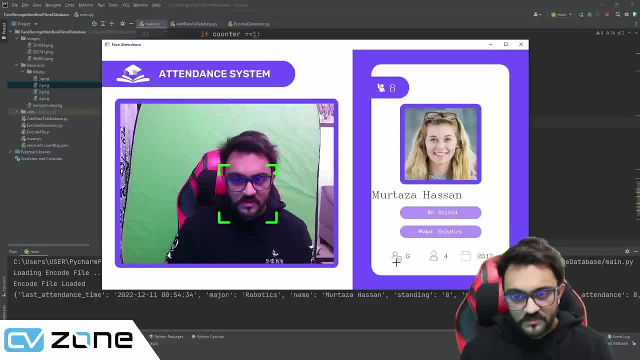 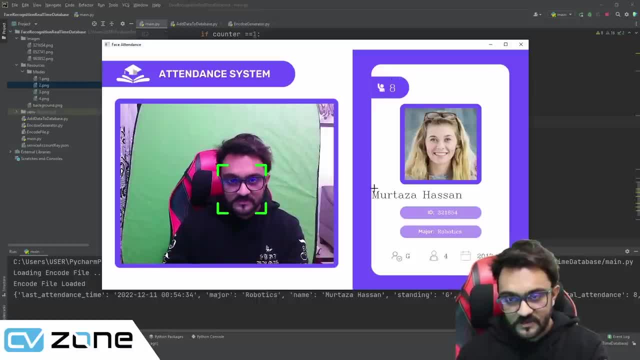 number of years is correct. number of years is correct, the starting year is correct and the. the starting year is correct and the. the starting year is correct and the attendance is correct. attendance is correct. attendance is correct now. the name is wrong because it is now. the name is wrong because it is. 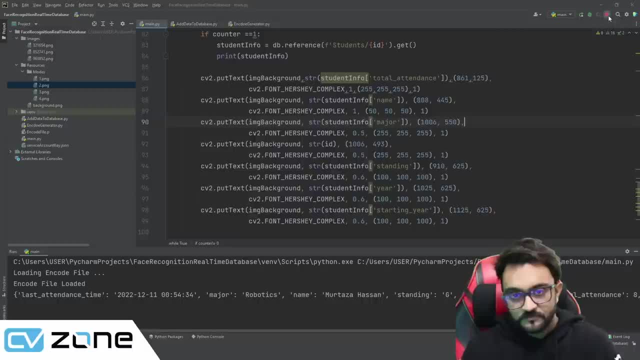 now the name is wrong because it is starting at the very edge, starting at the very edge, starting at the very edge, and we need to center it. so, and we need to center it so, and we need to center it. so how can we do that? so let's put the 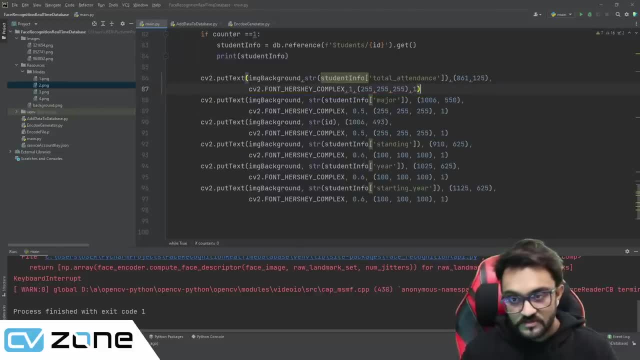 how can we do that? so let's put the. how can we do that? so let's put the name name name at the start, or let's put it at the end, at the start, or let's put it at the end, at the start, or let's put it at the end, so that. 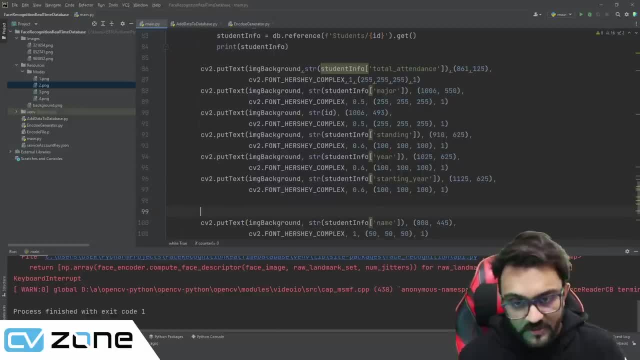 so that, so that we have something separate for it, so we, we have something separate for it, so we, we have something separate for it, so we will write it in, will write it in, will write it in. so what exactly do we need to do? so, what exactly do we need to do? 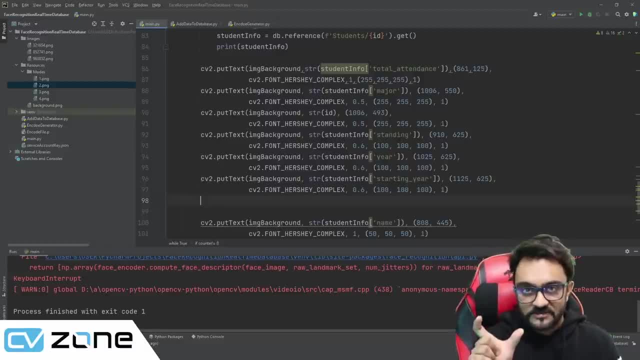 so what exactly do we need to do? we need to find the width of this text. we need to find the width of this text. we need to find the width of this text. so if i'm writing murdaza hassan, i need. so if i'm writing murdaza hassan, i need. 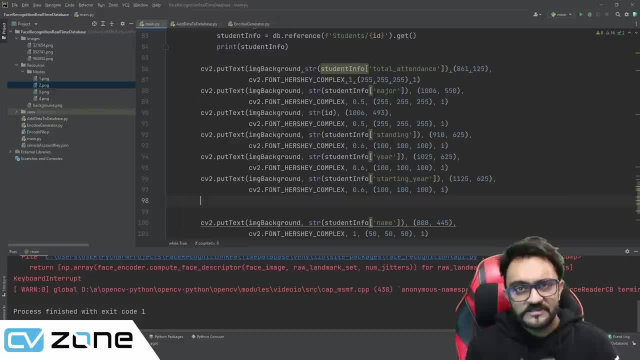 so if i'm writing murdaza hassan, i need to find the width of this text, to find the width of this text, to find the width of this text. so the width might be, let's say 50. so the width might be, let's say 50. 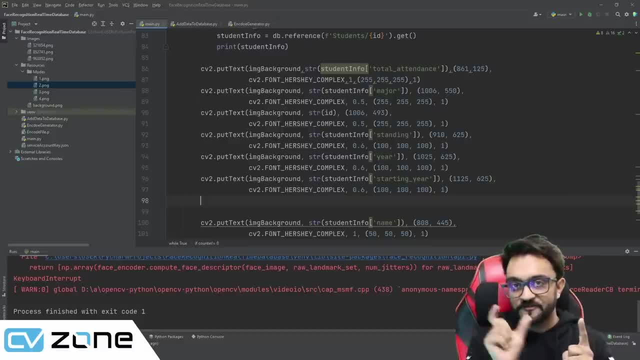 so the width might be, let's say, 50 pixels. so i will take the total width pixels. so i will take the total width pixels, so i will take the total width minus 50 pixels and then i will divide minus 50 pixels and then i will divide. 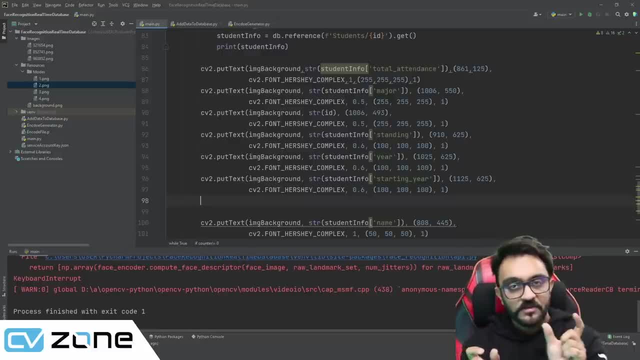 minus 50 pixels, and then i will divide it by two, it by two, it by two and start it from there. so i will push and start it from there. so i will push and start it from there. so i will push that 50, that 50. 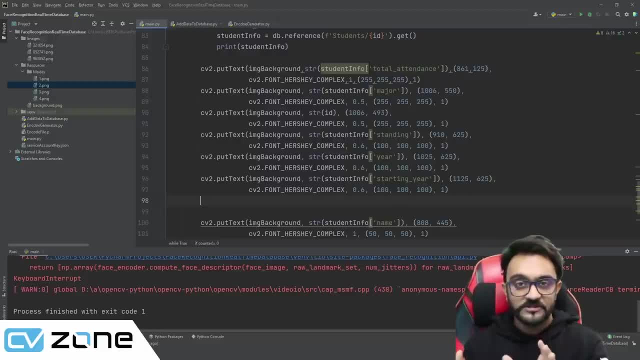 that 50 or 50 percent value a little bit, or 50 percent value a little bit, or 50 percent value a little bit further, and then it will start it from further, and then it will start it from further, and then it will start it from there, and then it will center. 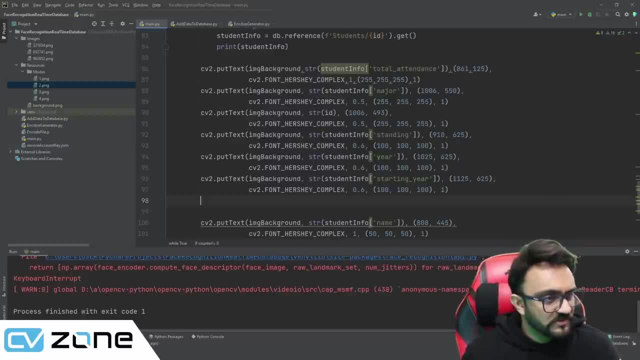 there, and then it will center there, and then it will center automatically, automatically, automatically. so i, i think it's pretty straightforward, so i, i think it's pretty straightforward, so i, i think it's pretty straightforward, so, so, so i hope i don't have to explain it further. 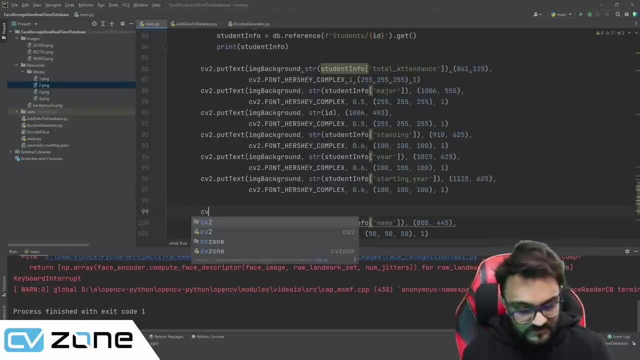 so how can we get the size you can get? so how can we get the size you can get. so how can we get the size? you can get the size by cv2 dot, the size by cv2 dot, the size by cv2 dot. get size, get. 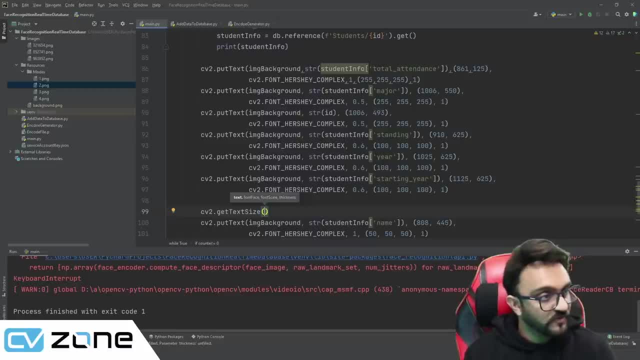 get size, get, get size, get size of the text, size of the text, size of the text and you have to give in the text so and you have to give in the text so and you have to give in the text so. student info, student info, student info at. 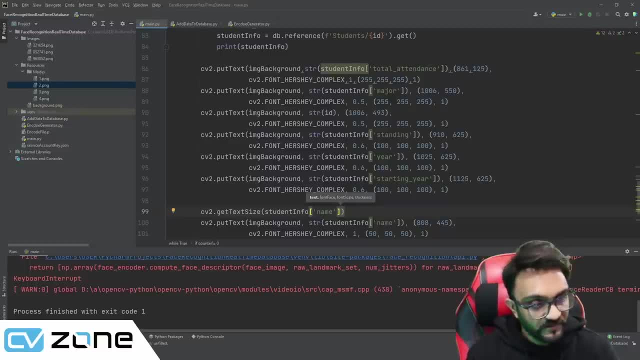 at at name, name, name, and then you have to give in the, and then you have to give in the, and then you have to give in the font cv2 dot. font cv2 dot. font cv2 dot. font hershey complex. so this should match. font hershey complex. so this should match. 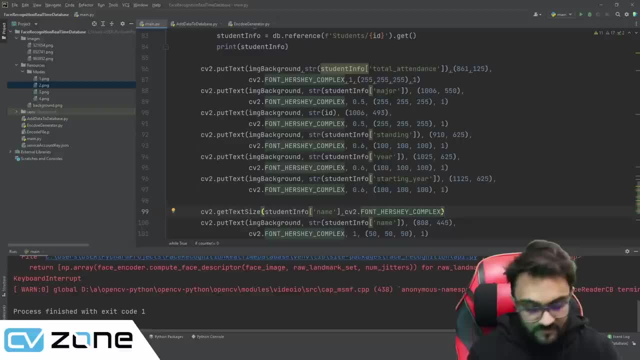 font: hershey complex. so this should match. all of this information should match. all of this information should match. all of this information should match, otherwise it will be wrong, otherwise it will be wrong, otherwise it will be wrong. and then we have the scale, and then we have the scale. 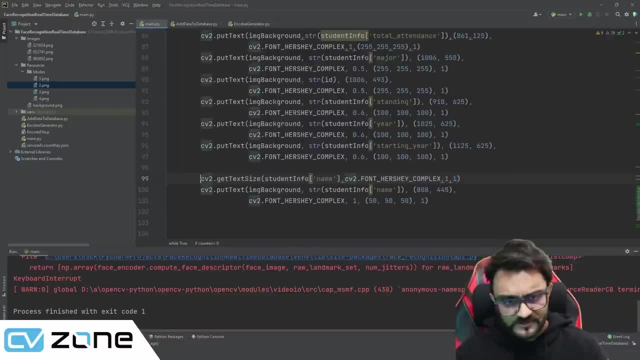 and then we have the scale and the thickness, and the thickness and the thickness. so this will give us the size. so what it so. this will give us the size, so what it so? this will give us the size, so what it will give us? it will give us the width. 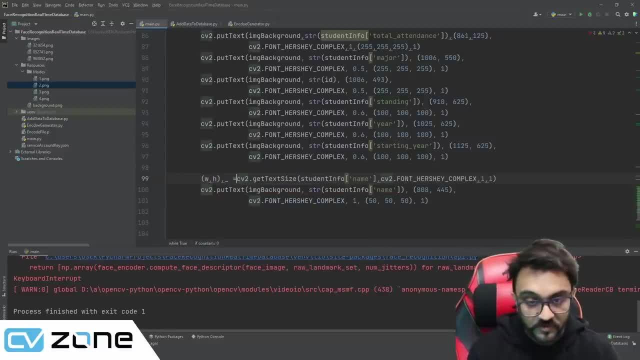 will give us. it will give us the width, will give us, it will give us the width and the height, and it will also give us and the height, and it will also give us and the height, and it will also give us another thing that we do not require. so 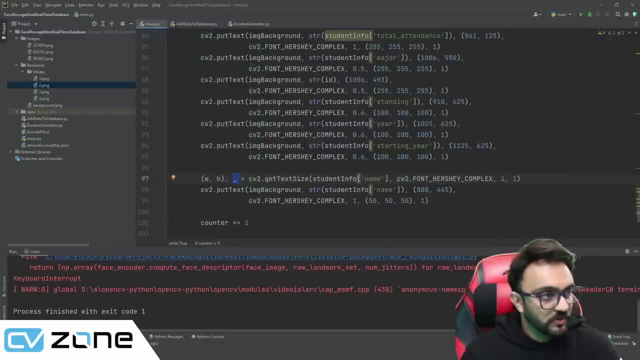 another thing that we do not require, so another thing that we do not require. so we'll put, we'll put, we'll put. so we will add this underscore because we, so we will add this underscore, because we, so we will add this underscore because we don't need it. 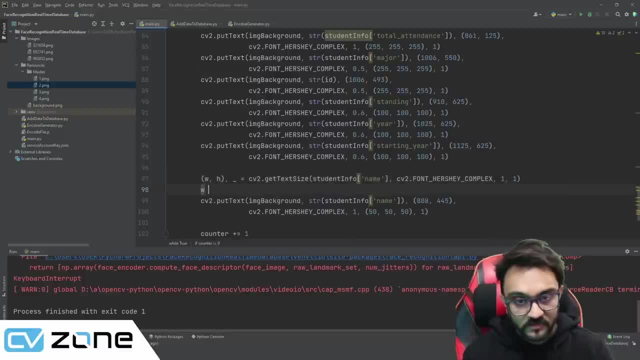 don't need it, don't need it. so once we have that, what we can do, is we so, once we have that, what we can do is we. so, once we have that, what we can do is we can write that our width can write that our width. 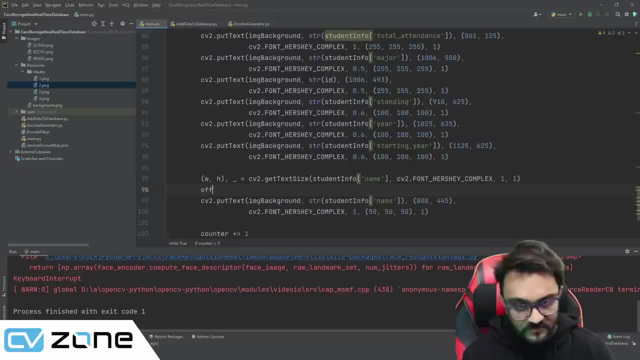 can write that our width- uh, let's say: offset our offset. uh, let's say: offset our offset. uh, let's say: offset our offset- equals width, equals width. equals width minus. this is the total width minus. this is the total width minus. this is the total width. no, this is not the total width, my bad. 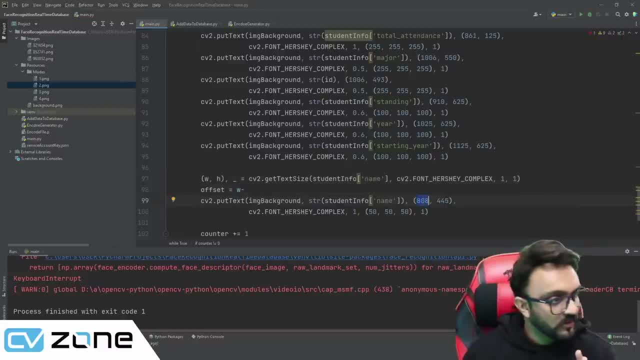 no, this is not the total width. my bad. no, this is not the total width. my bad. the total width, it is the total width. it is the total width. it is. the total width is 414.. how do i know this? the total width is 414.. how do i know this? 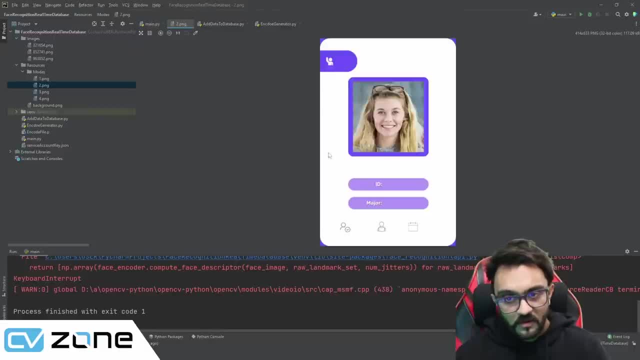 the total width is 414.. how do i know this? because what we are getting is the. because what we are getting is the, because what we are getting is the width, width, width, uh, starting from this point till the uh, starting from this point till the uh, starting from this point till the end point. so the width of this image is 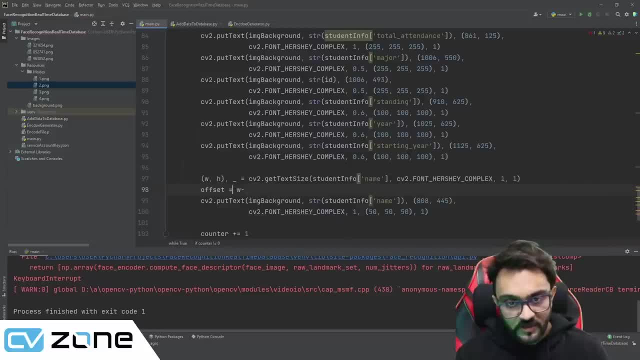 end point. so the width of this image is end point. so the width of this image is 414.. 414. 414.. so that is what we are writing. so here we. so that is what we are writing. so here we. so that is what we are writing. so here we will write. 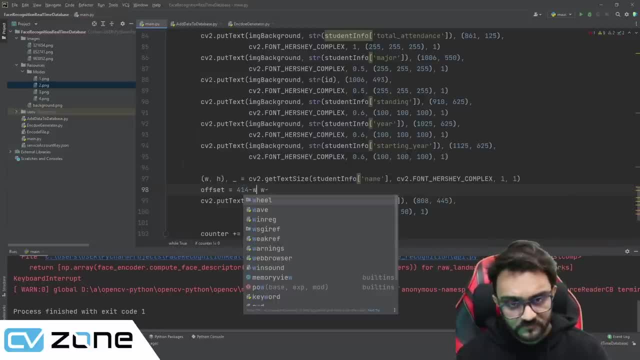 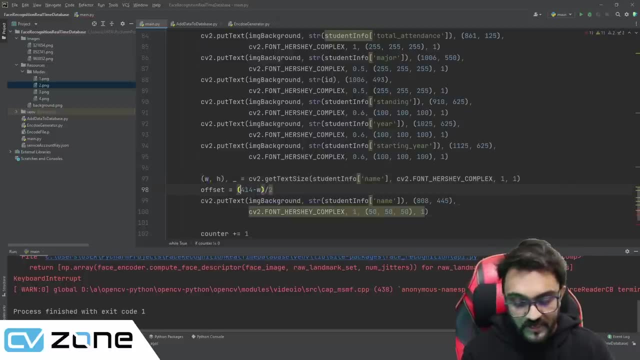 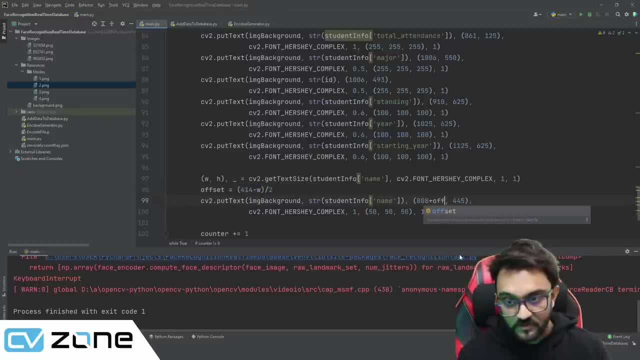 so that will give us the offset. so that will give us the offset. so and over here we will add it to the so and over here we will add it to the so and over here we will add it to the offset. the width will add to the offset. 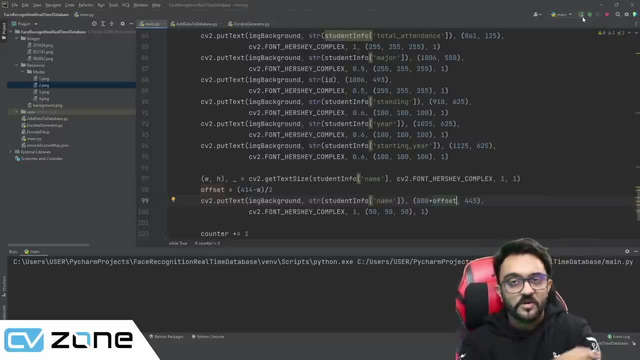 offset: the width will add to the offset. offset: the width will add to the offset. so if we run this now, it should center. so if we run this now, it should center. so if we run this now, it should center automatically. so if we check in for automatically, so if we check in for 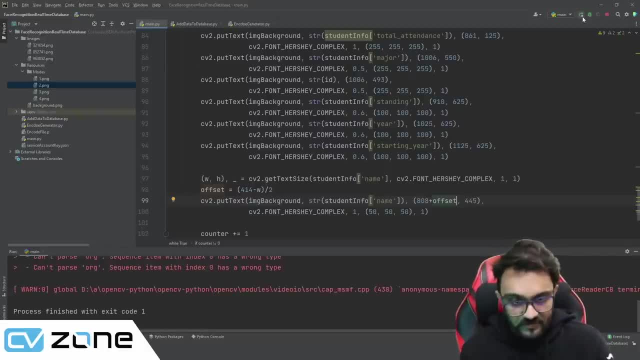 automatically. so if we check in for emily blonde for elon musk, all of them. emily blonde for elon musk, all of them. emily blonde for elon musk, all of them should center automatically. so here we should center automatically. so here we. 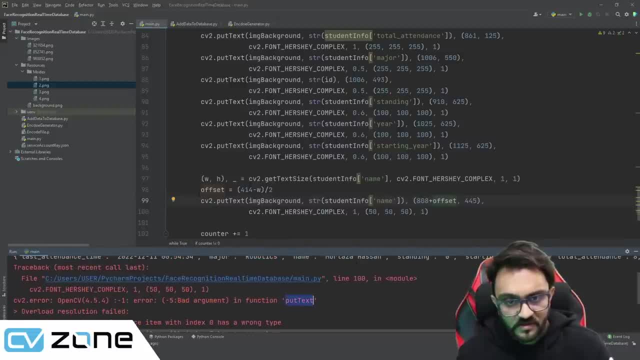 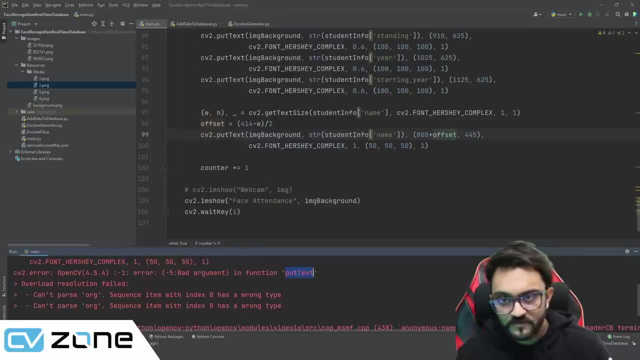 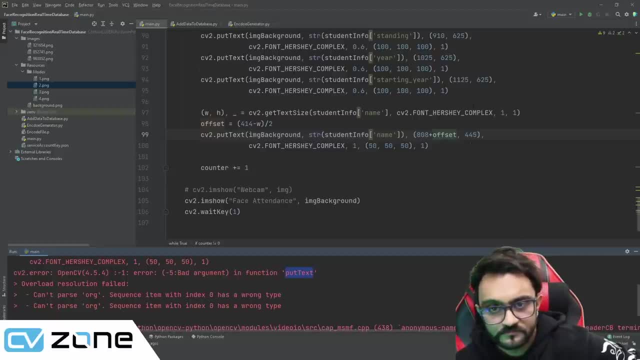 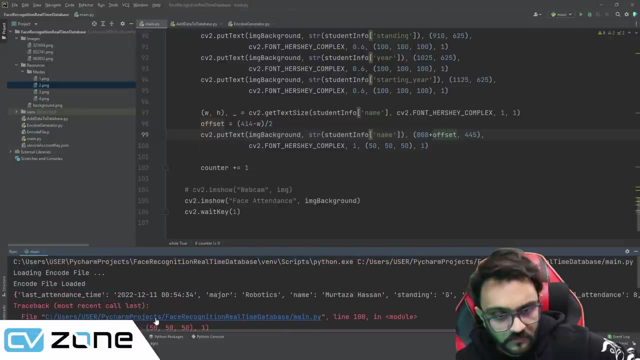 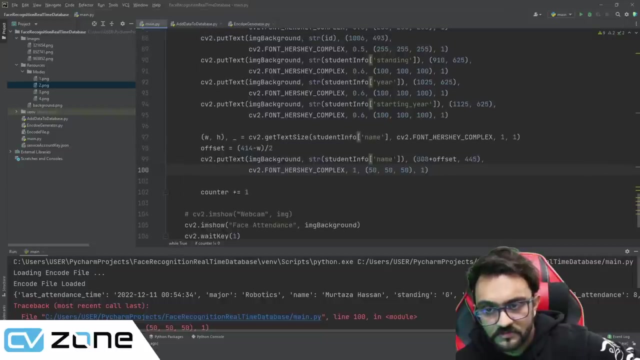 what exactly what? exactly? what exactly is wrong here? the type is wrong. okay, um, over here in its background. oh okay, so we have to put double slash. oh okay, so we have to put double slash. oh okay, so we have to put double slash because it might not. 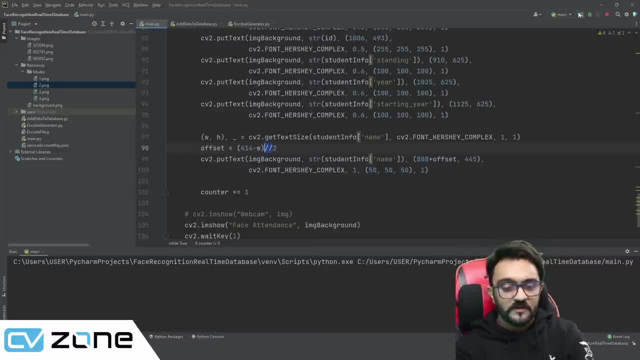 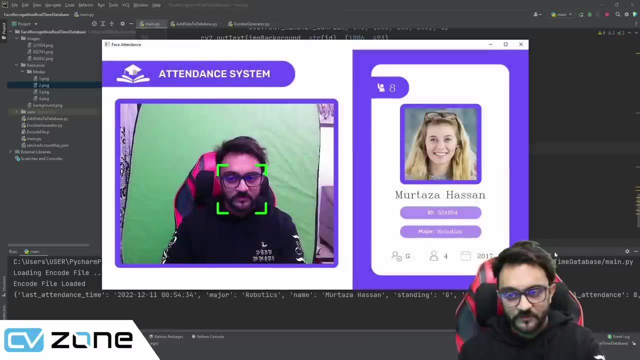 because it might not, because it might not be an integer. it might be a float, so that's be an integer. it might be a float, so that's be an integer. it might be a float, so that's why it's giving another. there you go, so now it's automatically. 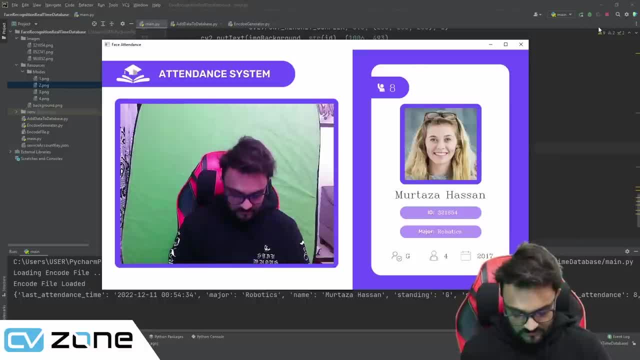 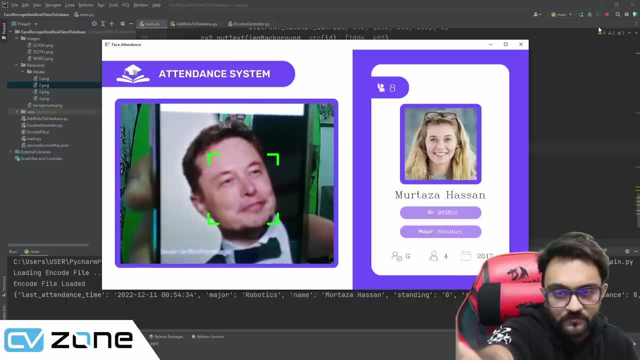 there you go. so now it's automatically there you go. so now it's automatically centered. so if i bring in centered, so if i bring in centered, so if i bring in, let's say, uh, let's bring in elon musk, is it not detecting elon musk? 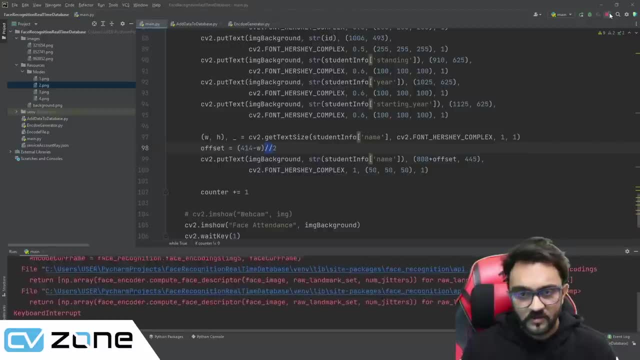 is it not detecting elon musk? is it not detecting elon musk? oh no, it will not update it. oh no, it will not update it. oh no, it will not update it a second time, because right now it's a second time, because right now it's. 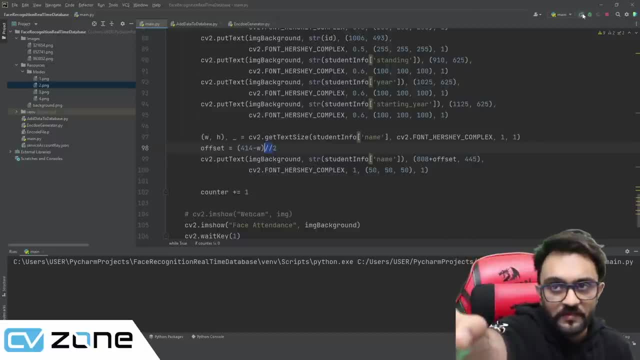 a second time, because right now it's already only updating for the first, already only updating for the first, already only updating for the first frame. so i will bring it before it frame. so i will bring it before it frame. so i will bring it before it starts. 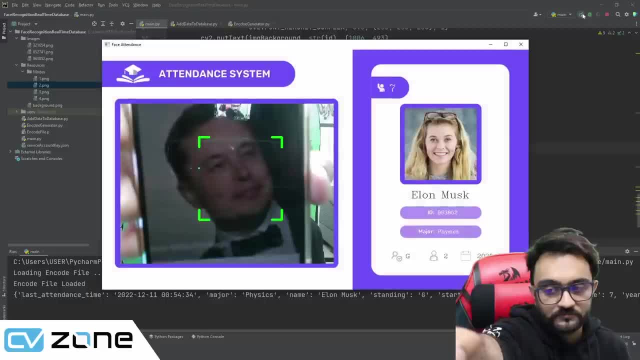 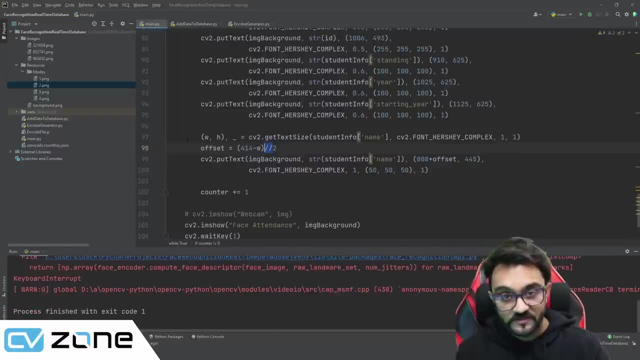 starts, starts, so that it checks for elon musk. there you go. so now even the elon musk, there you go. so now even the elon musk, there you go. so now even the elon musk is centered, is centered, is centered because, um, we have this code, that is. 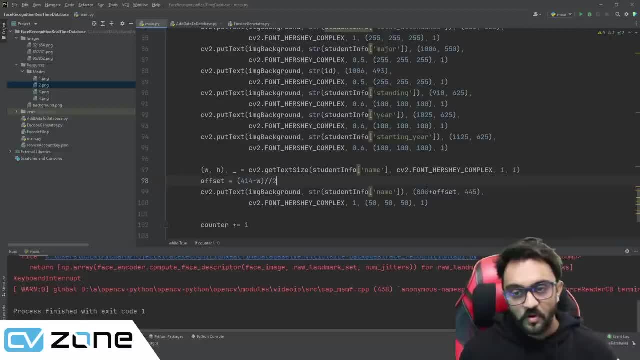 because, um, we have this code, that is because, um, we have this code that is checking automatically, checking automatically, checking automatically how to center it. so all of the how to center it, so all of the how to center it, so all of the information is information is information is being received, the data has been. 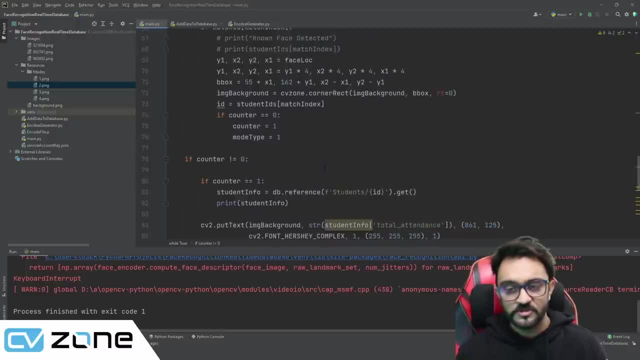 being received. the data has been being received. the data has been received, but not the image itself received. but not the image itself received, but not the image itself. so now, what we need to do is we need to. so now, what we need to do is we need to. 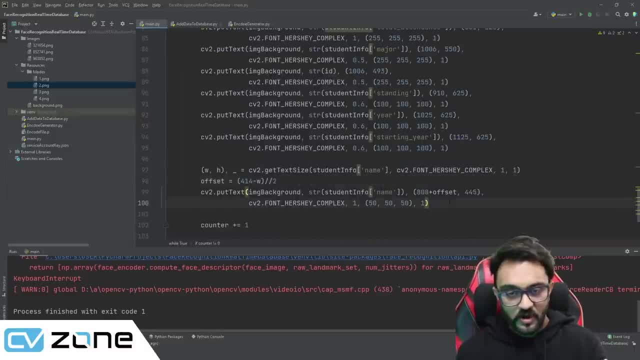 so now what we need to do is we need to get the image and we need to add it. get the image and we need to add it. get the image and we need to add it uh to our, uh to our, uh to our graphics as well. so how can we do that? 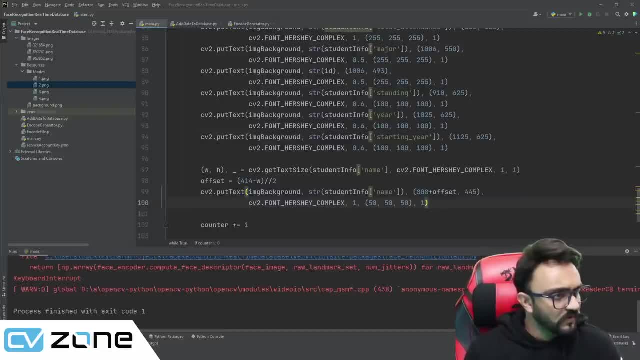 graphics as well. so how can we do that? graphics as well. so how can we do that? it's fairly simple. so, uh, where are we getting the data here? so uh, where are we getting the data here? so uh, where are we getting the data here? we are getting the data over here, so we. 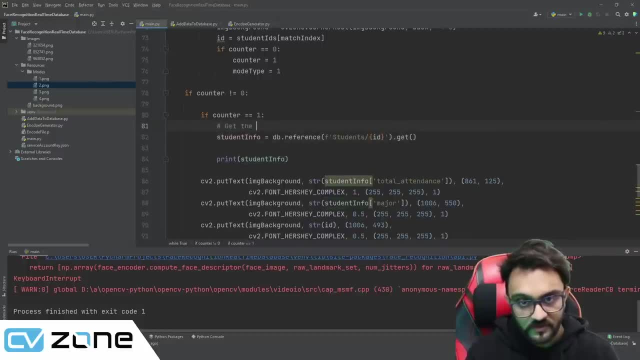 we are getting the data over here, so we we are getting the data over here, so we will write here: get the data will write here. get the data will write here. get the data. so here, so here. so here we will write, we will write, we will write. get the image. 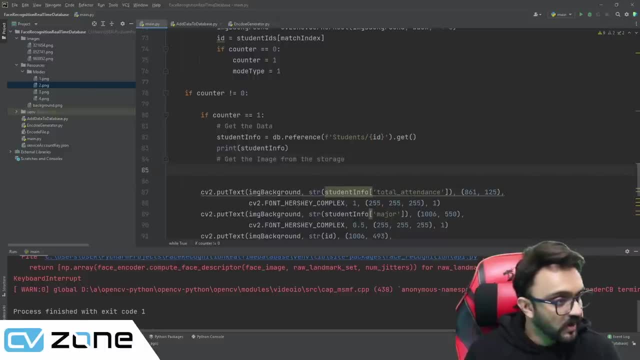 get the image, get the image from the storage, from the storage, from the storage. okay, so how can we do that? okay, so, how can we do that? okay, so how can we do that? uh, we are basically reversing the. uh, we are basically reversing the. uh, we are basically reversing the method. we are writing here, blob. 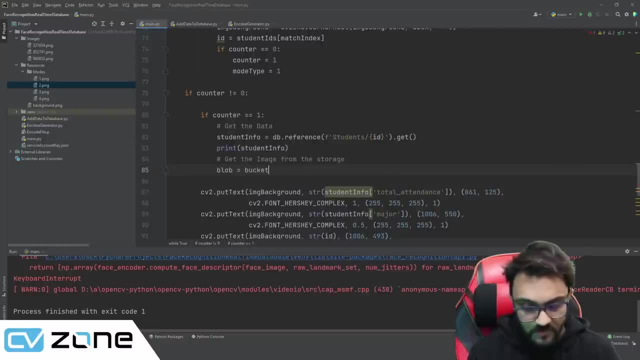 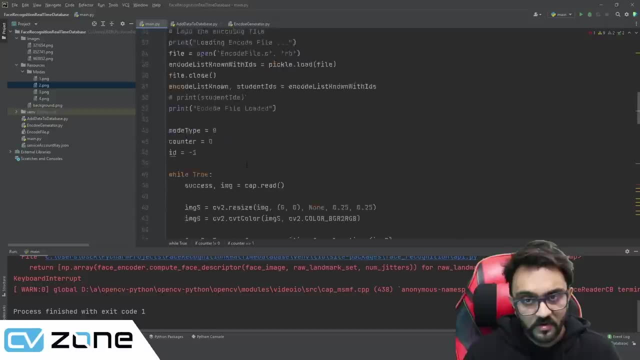 method. we are writing here blob method. we are writing here: blob equals, equals, equals: bucket bucket, bucket bucket dot. get bucket dot. get bucket dot. get underscore blob: underscore blob, underscore blob. so so so bucket is not defined because bucket is not defined, because bucket is not defined, because we didn't create any bucket. so here we. 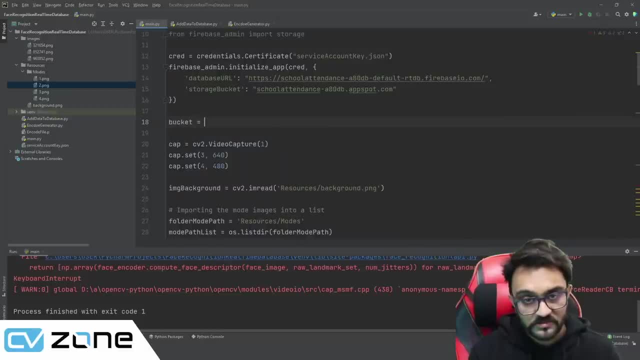 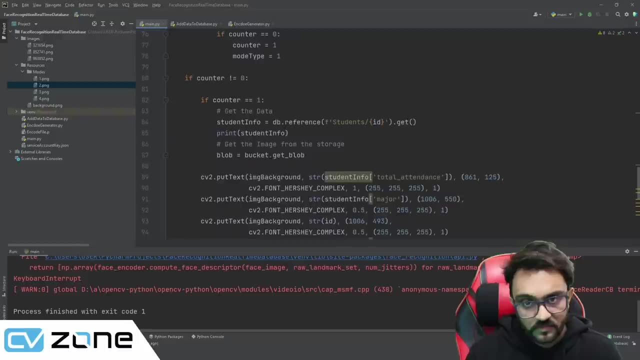 we didn't create any bucket, so here we. we didn't create any bucket, so here we will write, will write, will write. buckets equals storage buckets, equals storage buckets, equals storage, dot bucket, dot bucket, dot bucket. and then here, and then here, and then here we will write. 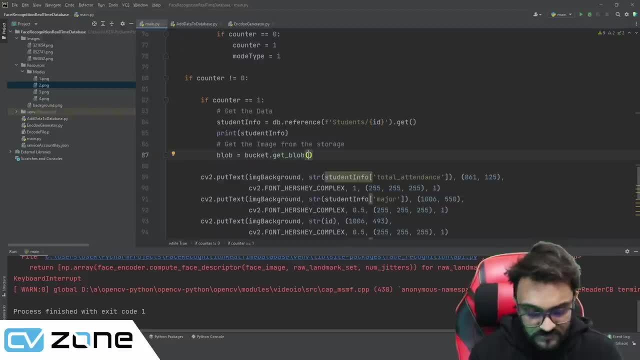 we will write. we will write: get blob, get blob, get blob. and we are going to give in the reference and we are going to give in the reference and we are going to give in the reference. so it will be f, so it will be f, so it will be f, and then we have the images folder. if you, 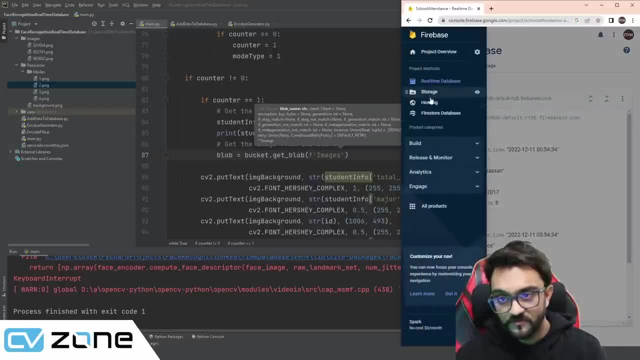 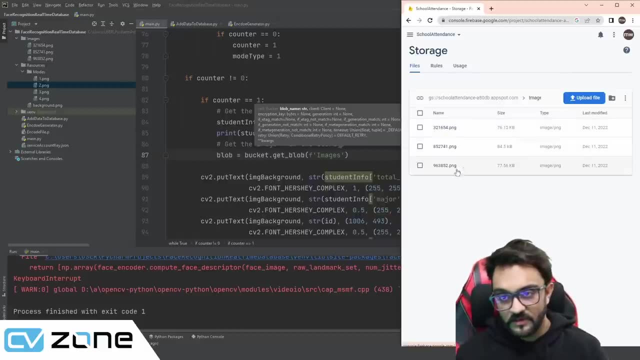 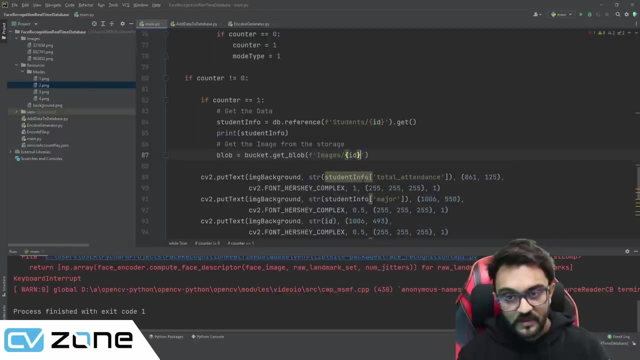 and then we have the images folder, if you, and then we have the images folder, if you remember, remember, remember in our storage, in our storage. so if we go to storage we have the images folder first and inside that images folder we have our images by their ids. so again we have to do the same thing. we will write slash, we'll put id and. 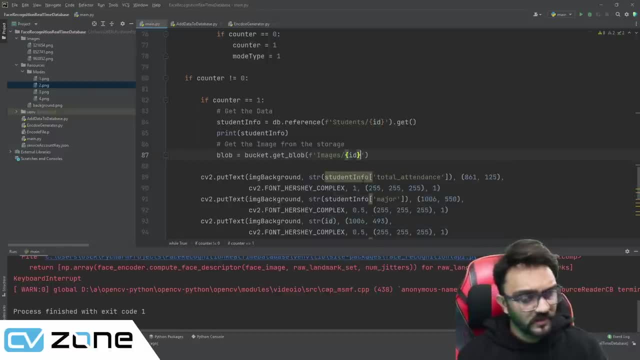 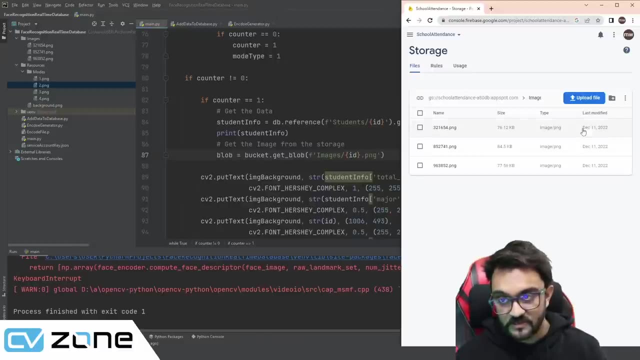 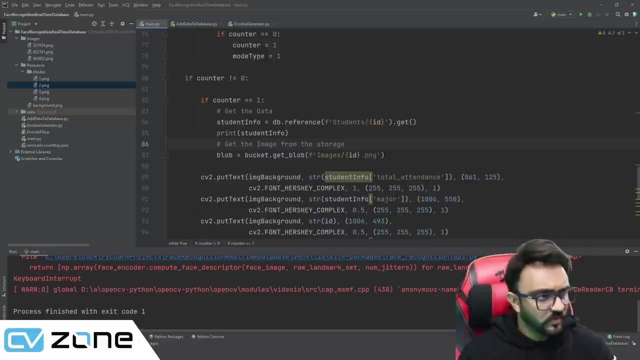 that is pretty much it. and then, uh, we don't have to write png, do we? no, we do have to write png dot png, because that is the complete name. it is stored with the png name, so we have to write that as well, otherwise it will not work properly. so then we have to create an array from: 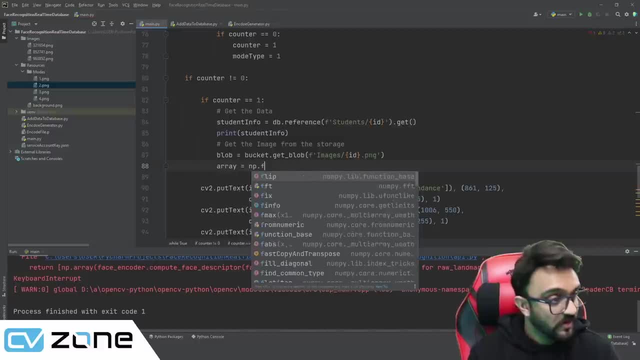 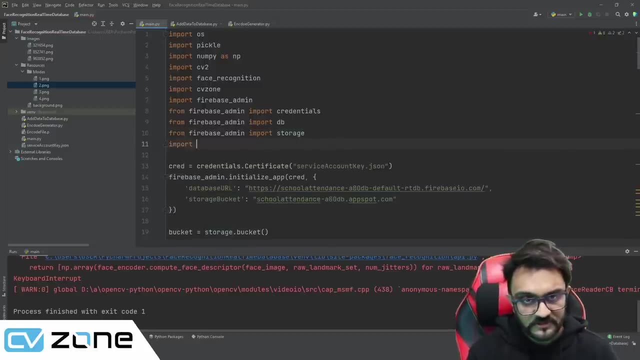 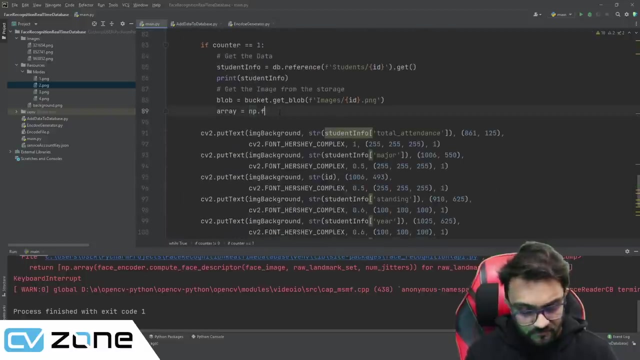 this array equals numpy dot from buffer. so just think of this as a standard method of converting. don't have to go into too much detail. import numpy as np and from from buffer, buffer, buffer, and we will write blob dot download as string and then we have to give in the numpy dot. 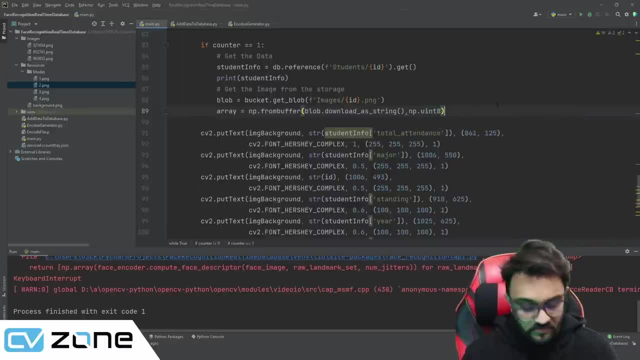 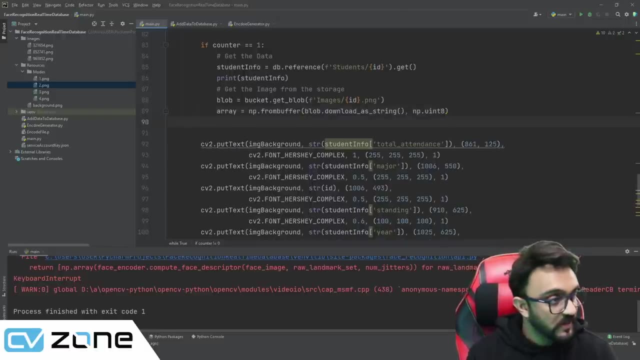 unsigned integers of 8 bits. so that's the idea. and once we have that array, now we need to convert it so that we can use it with opencv. so we will write here: image student equals, uh, cv2, cv2 dots, uh image decode, and we will give in the array and we will give in the. 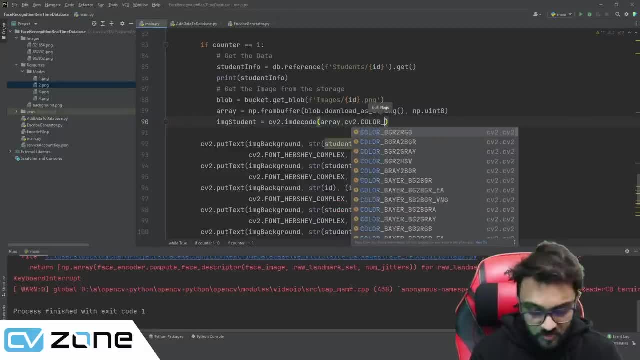 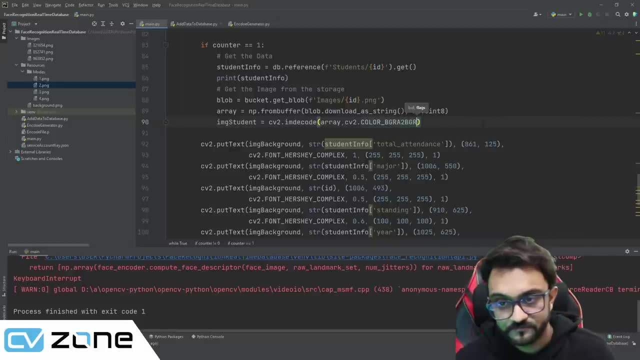 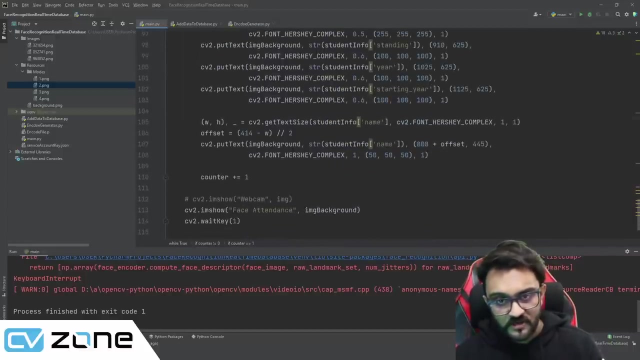 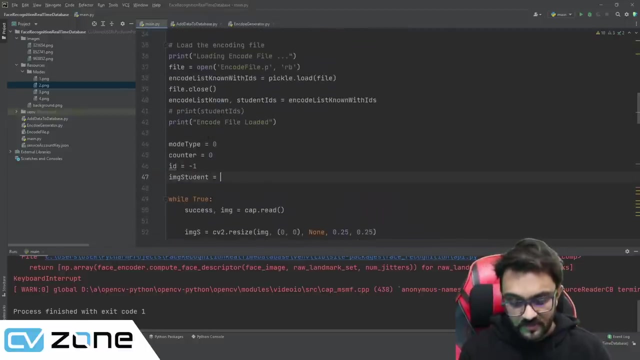 conversion: cv2 dot. color underscore: bgr, bgr, a2, bgr. so this will give us the image and now what we can do is we can use this image outside here to display. so let's just to make sure that it works. we can put here image: student equals empty, and later on we will keep adding it. 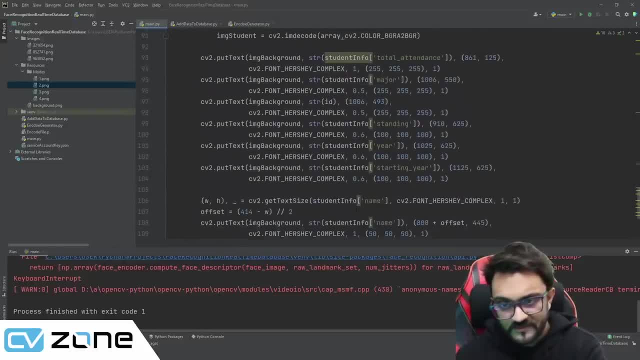 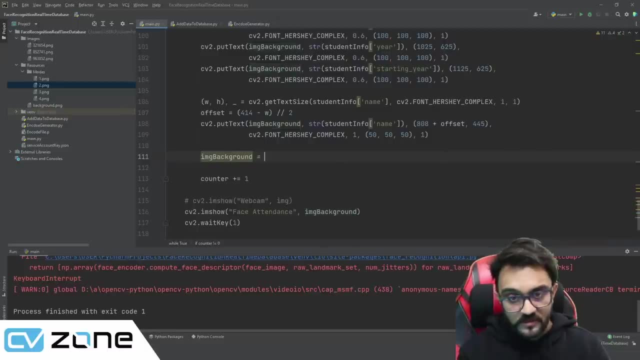 so here, um, after all of the text is done, we are going to put in the image, and to put in the image we'll write image background. at what values equals image student? so what are these values? again, i have done the math already and it is 175. 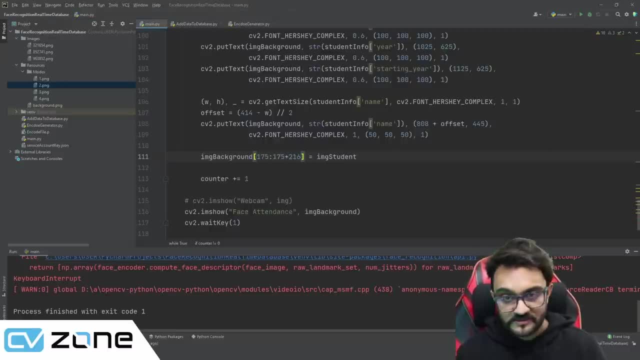 and 175 plus 216, because 216 is the size of the image and these this is the offset, so the offset in the width is 909, and then we have 909 plus 216.. so if we run this now again, it will download it once. 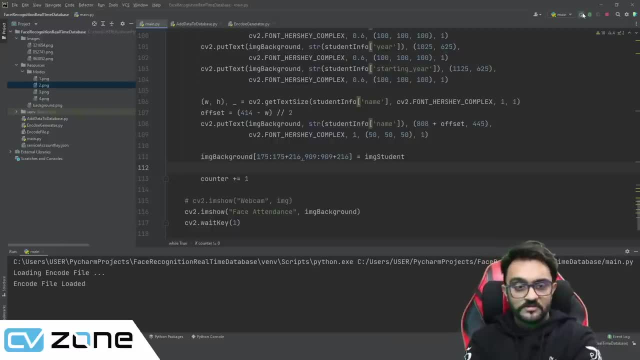 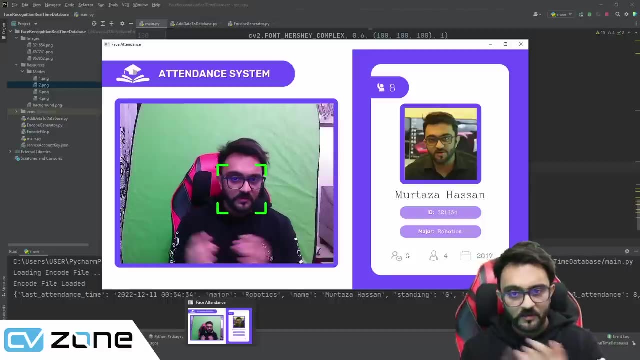 but it will display it again and again. so let's find out. and there you go. so now you can see my image is downloaded. number of attendance: id number, major good standing year number. total number of years in the university. so that is the main idea. so it is. 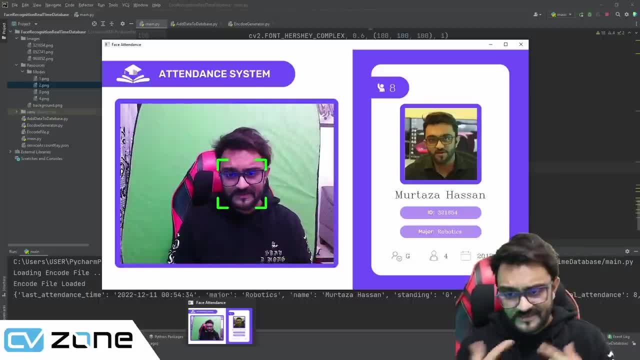 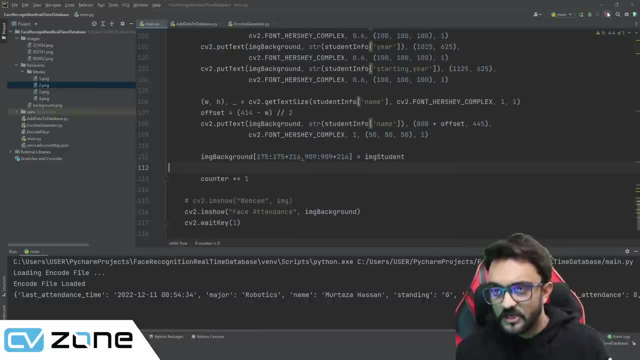 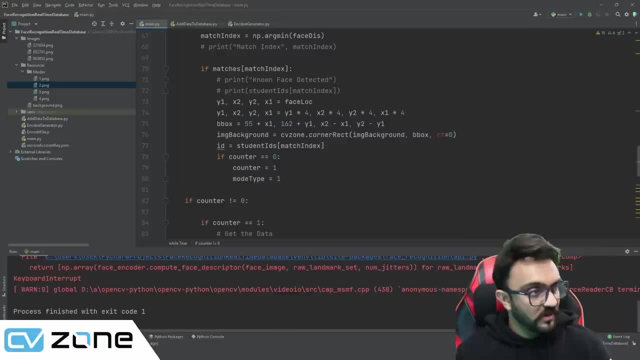 working very well right now. so, uh, the next step is to update the attendance. so every time it is, uh, we detect it, it should update the attendance. so we have to send the data, and this we will only do once because, uh, we don't need to keep doing that every iteration. so how can we send it? 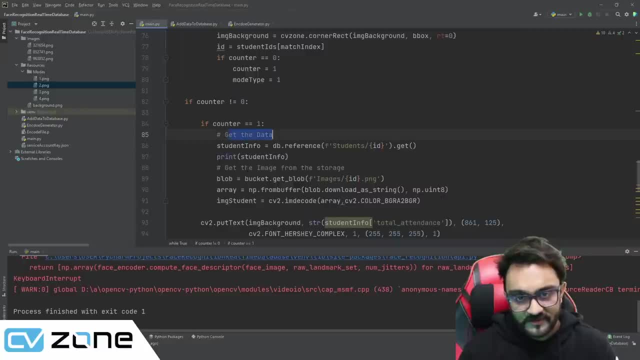 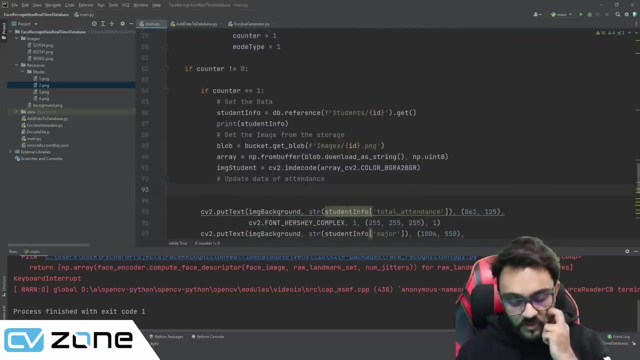 ticking through. it is very simple. i will just see if i can irgendly recall how to do that. so yeah, iorden, the data is very simple. so here, after getting the data and getting the image, we are going to update the data. so here we will write: updates- data of attendance. 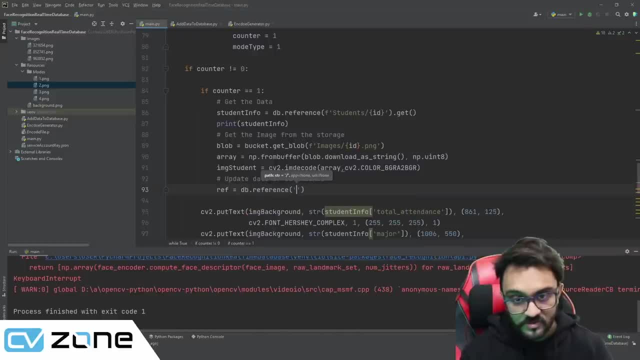 so here we are going to create a reference reference equals db, db dot reference- and we'll give in the path over here like this: and now, using this reference, we are going to send in the data. so here we will write that first of all we need to update. so student info at total underscore: attendance: 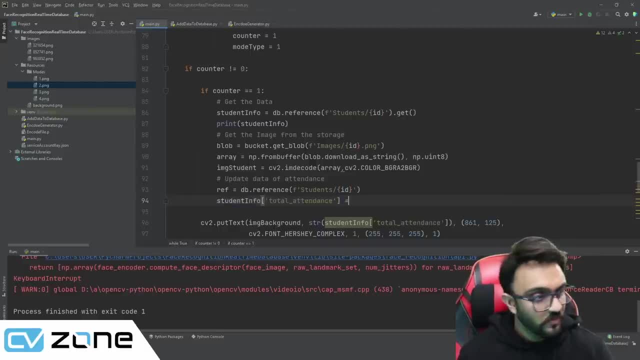 equals. we are going to update, so we will write plus equals one. and now we are going to update this value in our server, in the database. so here we are going to write ref- dot child. if you remember, when we were sending the data we wrote ref dot, child, dot set. 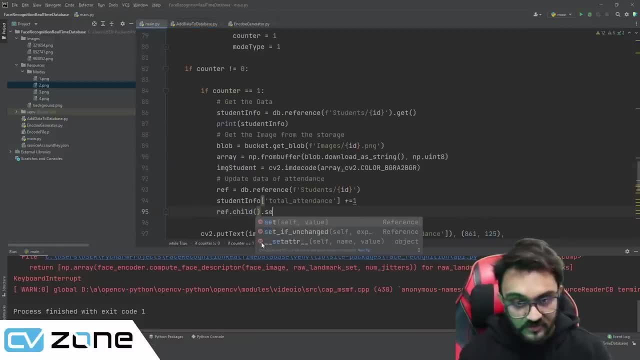 so we are going to do the same thing: ref dot, child dot set and child. what value we? we need to update total attendance and we need to update it with this value. so, whatever the updated values, we need to update it with that. so let's run that and see if it works. 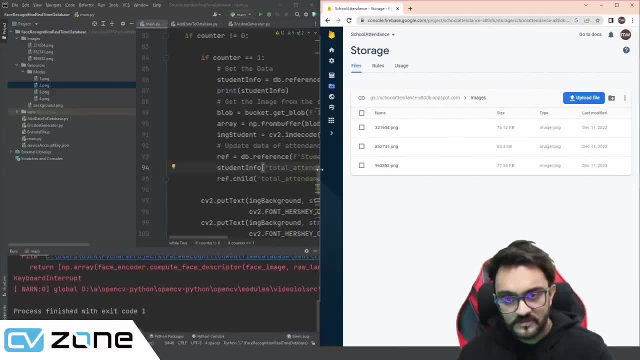 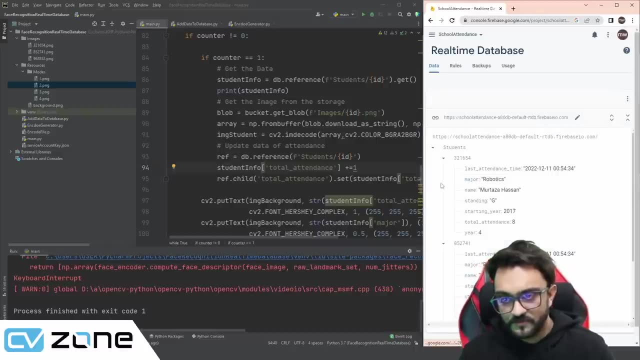 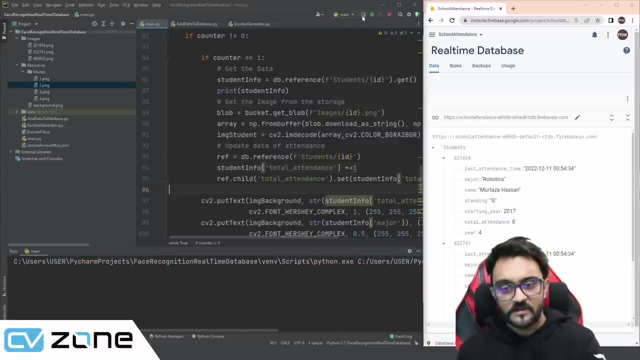 so i'm going to put this on one side and this will be on the other side. so let's go to the real-time database and i will open up my own. there you go, and here the total attendance is eight. so if i run this now, it should update to nine as soon as it is. 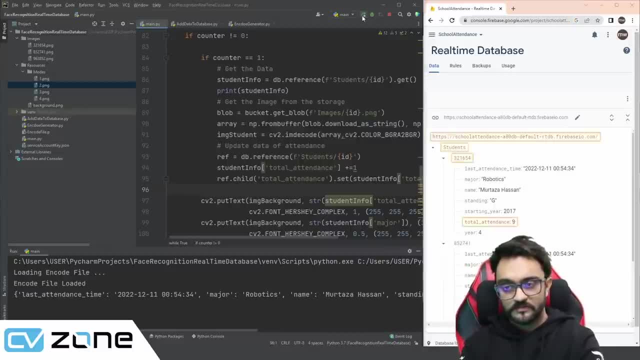 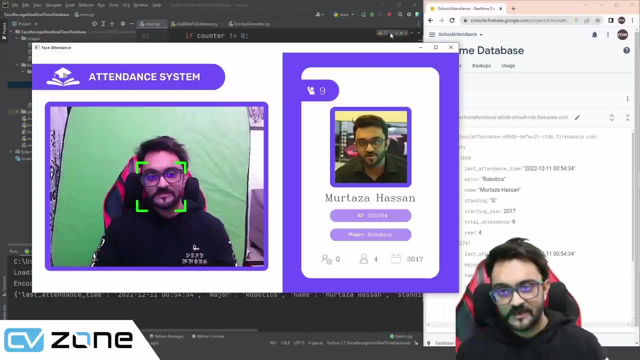 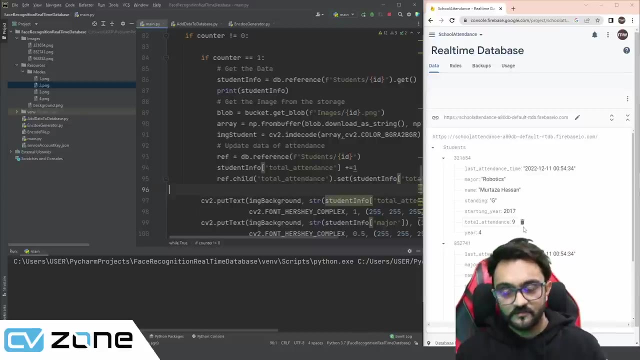 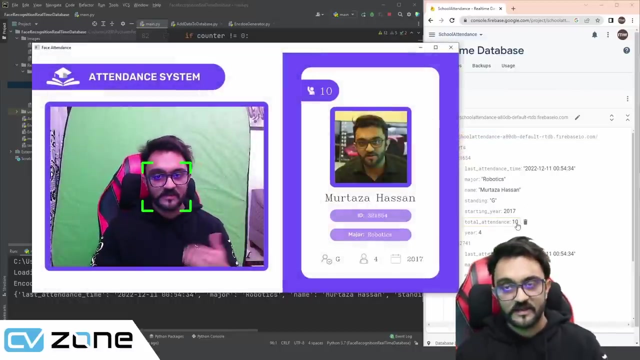 detected. there you go. so it is updated to nine, and it is also showing nine over here. so it means it is correctly adding the values to the database and if i run it again, it should update it to ten. there you go. so now the total attendance is 10. it has been updated. so this is the basic idea of this. 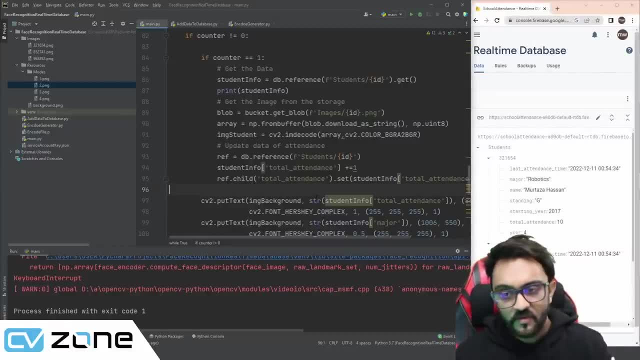 and then what else do we have to do? now? what we need to do is we need to create this timer thing so that once it is detected, it will detect. okay, we need have updated, we have marked, and then it will go back to active to detect for a new student. so how can we do that? so the counter is already. 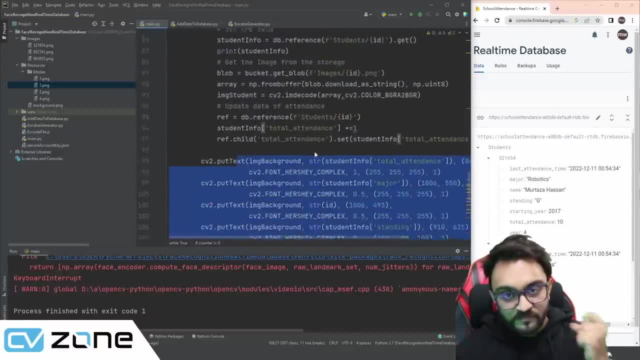 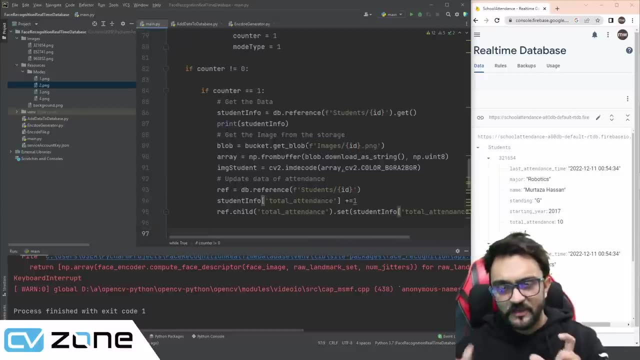 running. so we will show all of this only when the mode type is two. so what we will do is we will say that we will show all of this only when the mode type is two. so what we will do is we will say that we will give it some certain values. so over here, uh, i believe it is from 0 to 10, then 10 to 20 and then. 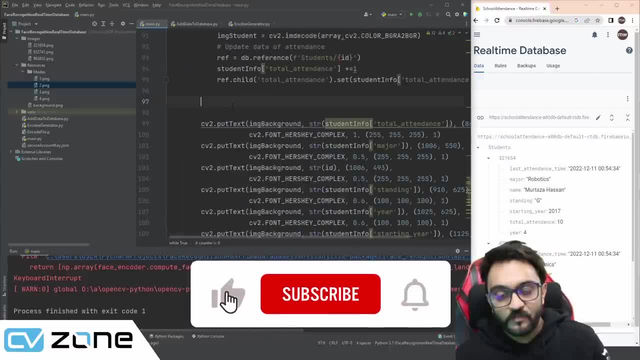 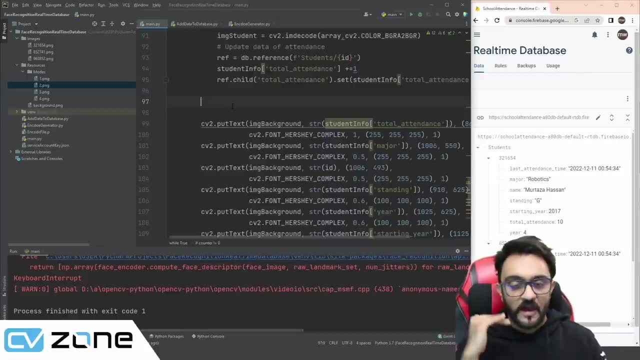 20 to 30. yeah, so greater than 20.. so here it's a little bit tricky because we have to add it based on certain formatting. if we add the if statement above another if statement or below the other if statement, it will change the effect, so we have to make sure it is in the correct format. 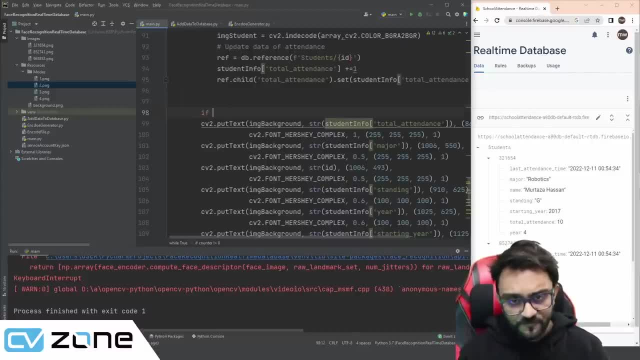 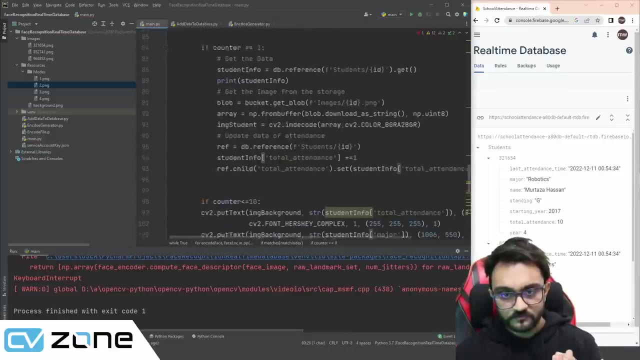 so the first thing we have to do is if, uh, our counter is less than 10, less than or equal to 10, then we are going to display all of this. the mode type will be 1 and we will display all of this. so we are going to do all of this. 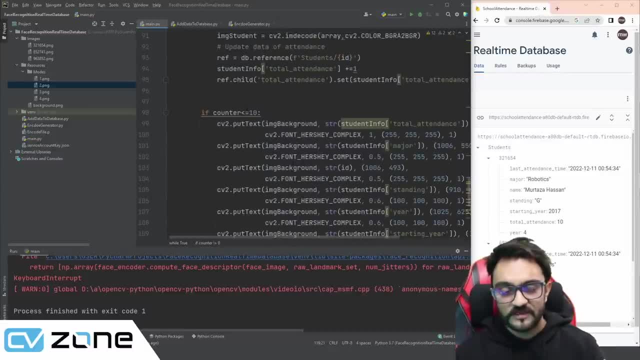 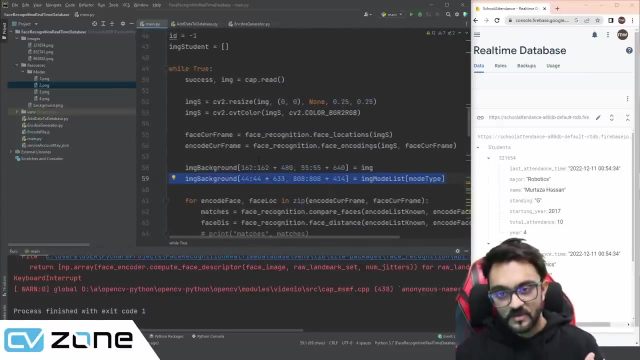 there you go. but if that is not the case, if the counter is between 10 and 20, then we are going to display marked value. but that is supposed to be done before this. otherwise, because the the only time it's updating the image is here, so it will be too late for us to update. so we have to update. 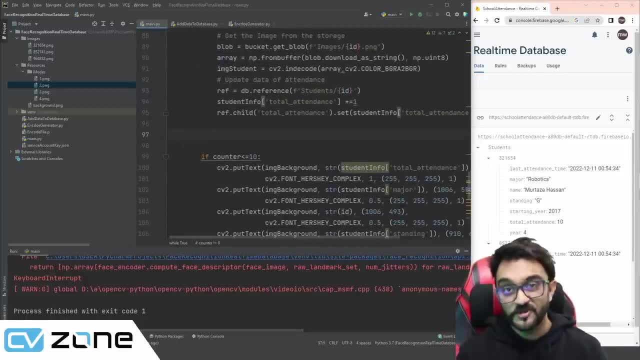 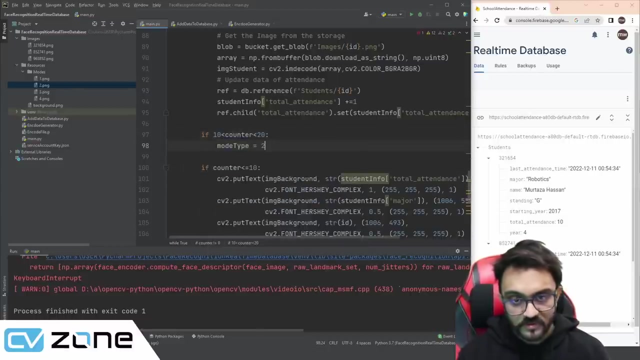 it again. so here we'll first check: do we need to update? we need to update it when if counter is in between 20 or- let's remove that- 10 and 20. so if it's between that, then we have to make mode type equals 2 and if we may change the mode type, we need to update the image before putting. 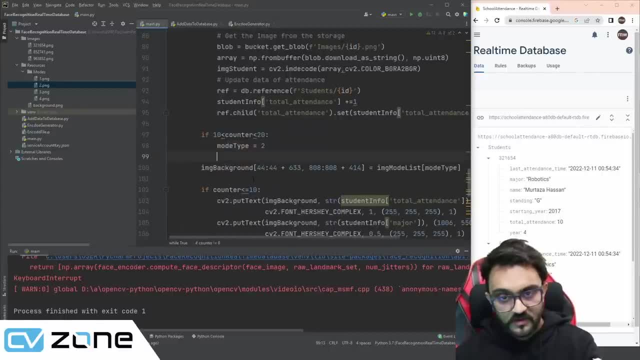 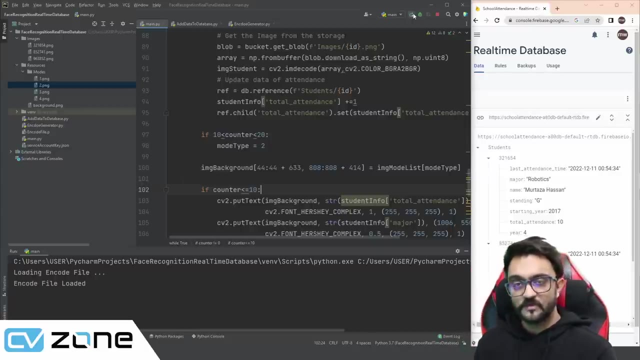 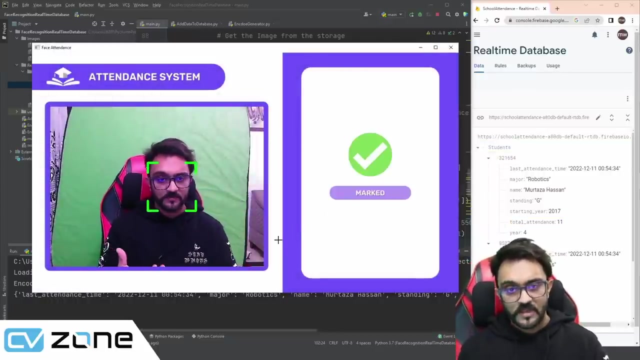 everything on it. so here we will write image background, here will be more type, so so. so let's run that and see if it works. so the first 10 frames it is supposed to show the image and all the data and then it will say marked. there you go, it's showing, and then it says marked. now, once that is done, we did not say 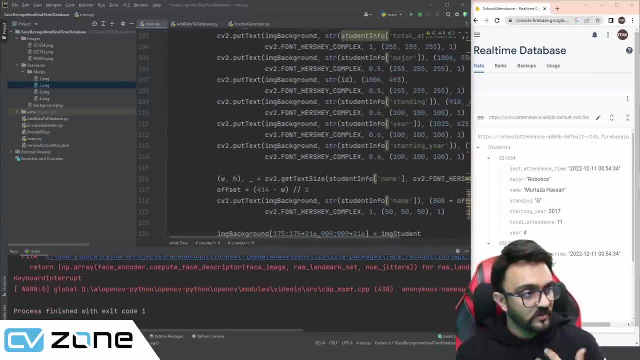 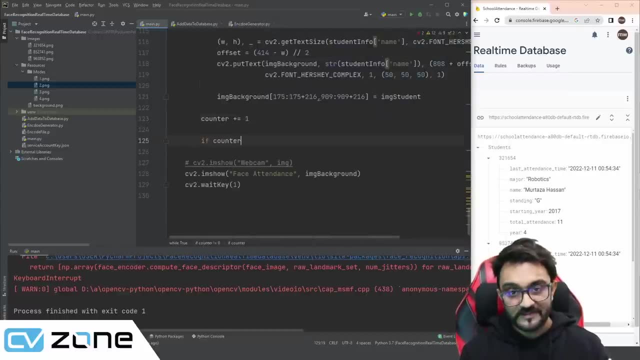 what to do next. the next part is when the counter is completely done, when it is above if the counter- and this has to be below the counter plus one- if it's above the counter plus one, there will be one wrong frame, so add it below the counter. 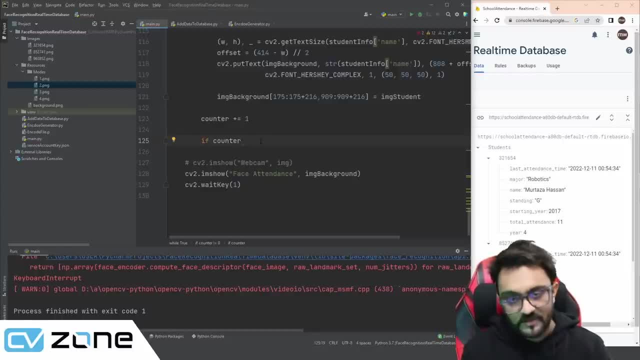 you can try it out to see what happens. but i have checked it and that's why i'm telling you: if counter is greater than or equal to 20, then we are going to write counter counter equals zero, then mode type equals zero. basically, we are resetting everything. then the student info equals empty and the image 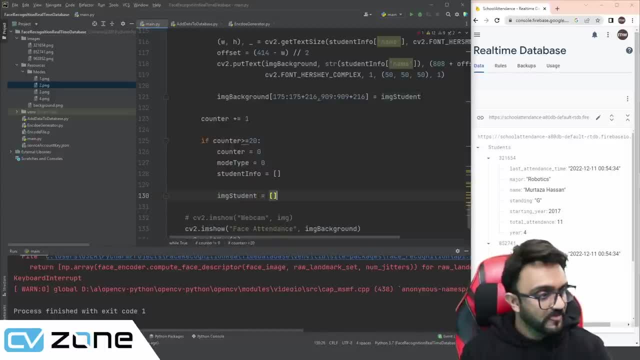 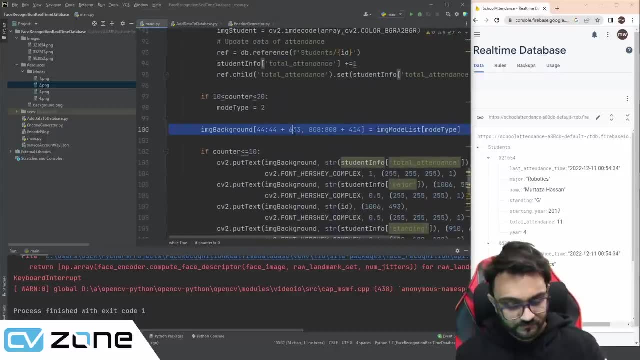 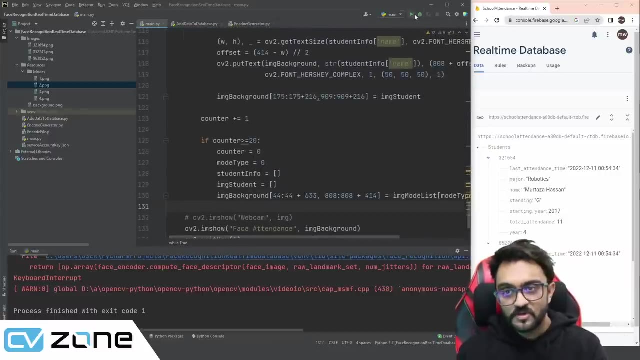 students. and then we are going to write counter- counter equals zero. and then we are going to write counter equals empty and we are going to update the mode type again. because we updated the mode type, we need to reset it quickly at the same spot. so let's run that and see what happens. so it should reset all of that. 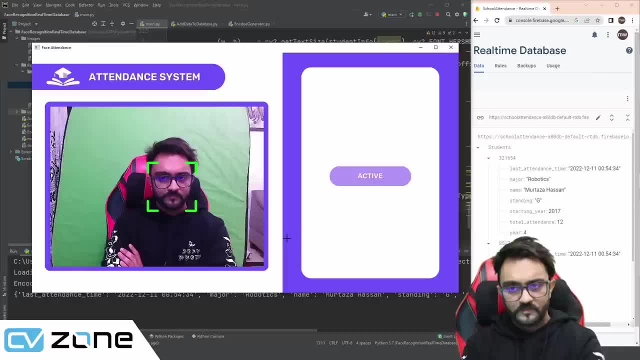 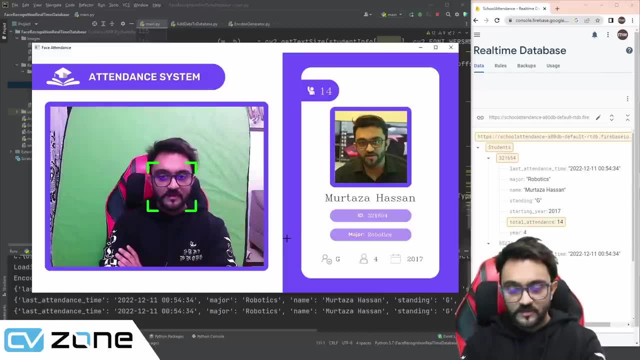 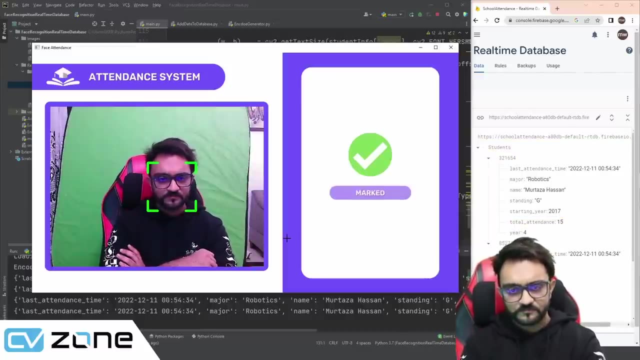 there we go: marked active, then it will start again. marked active, then it will download. it will show. you can see the attendance is updated. last time it was 14, now it will be 15 and then it will go to 16.. so again, that's not the right way. you should not keep adding the attendance values. so what we need to 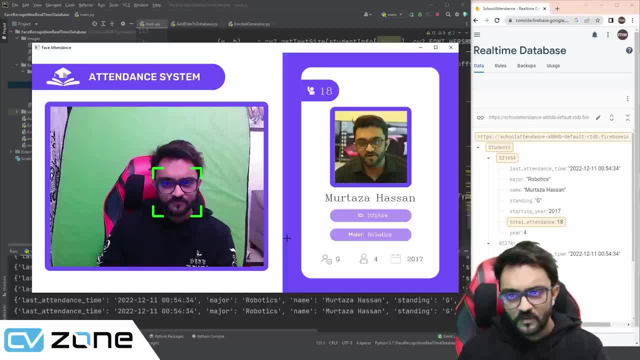 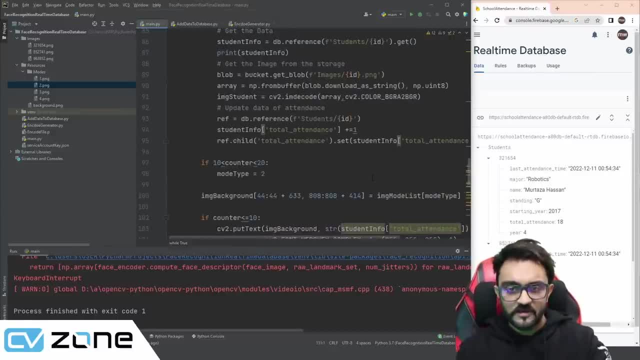 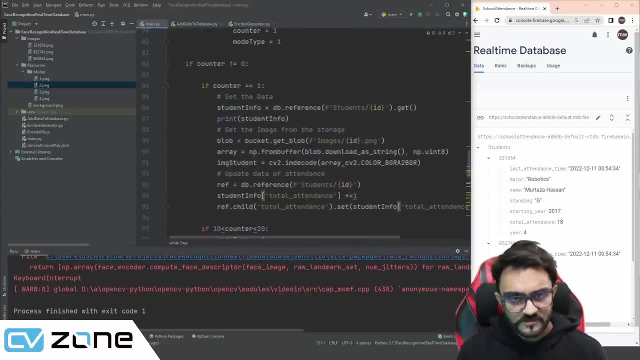 do is now: we need to pause and we need to check whether you are, whether the attendance was done an x amount of time after the previous attendance. so to do that, what we will do is, it's very simple: where did we update the attendance? where are we? 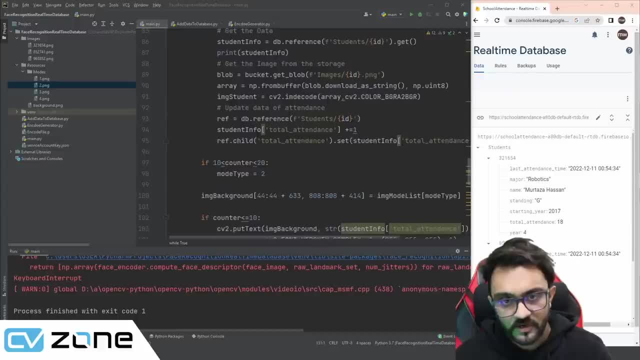 updating the attendance. okay, so here we are updating the attendance. so here we are going to say: if the student time was more than 30 seconds from the previous attendance, then we are going to mark attendance because we are testing. otherwise you will put the total amount of seconds as the actual hours. for example, you 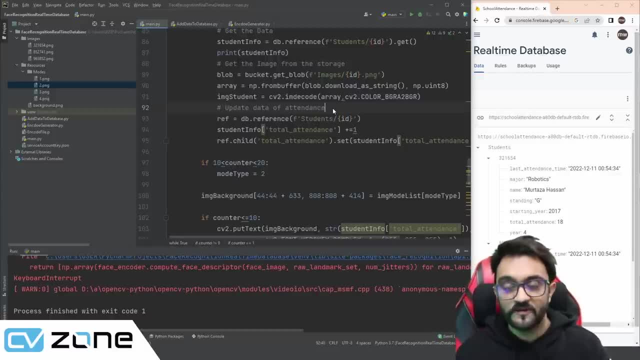 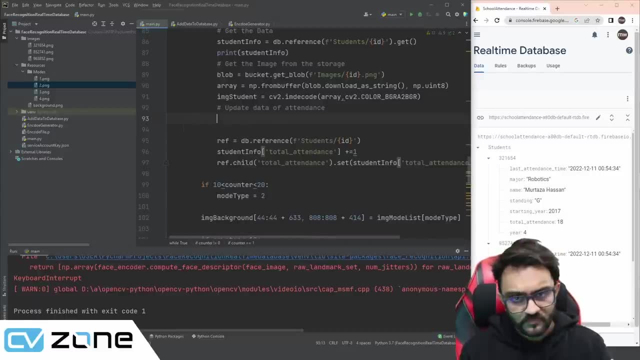 want it after 12 hours or the next day, so you want it after 24 hours, so we'll add it in seconds instead of hours. so here we are going to write that our dates underscore date time object equals date time. dot string to time. now why are we doing this? because the time over here is basically string. 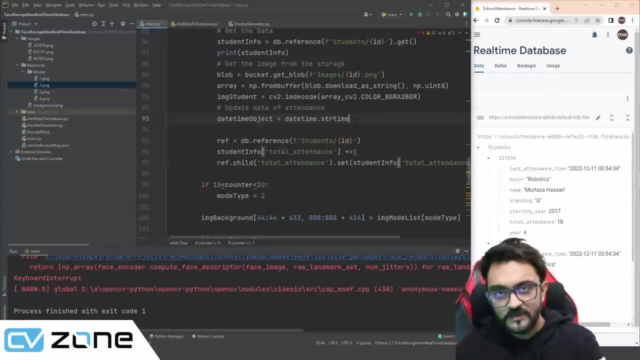 whatever we are getting from the database is string. we need to convert it into an object that the date time understands. so we will tell the date time what is the time right now and minus it from this time. so when you minus it it is not string minus string, it is object minus object. so that's why. 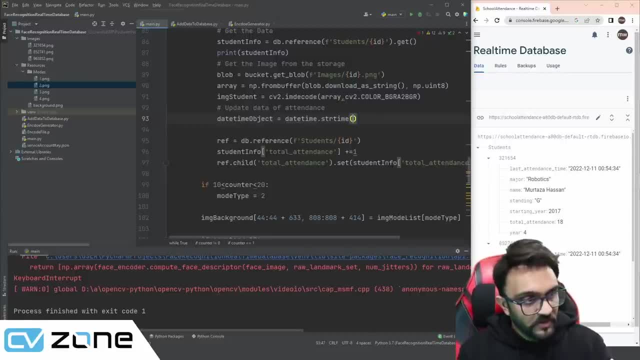 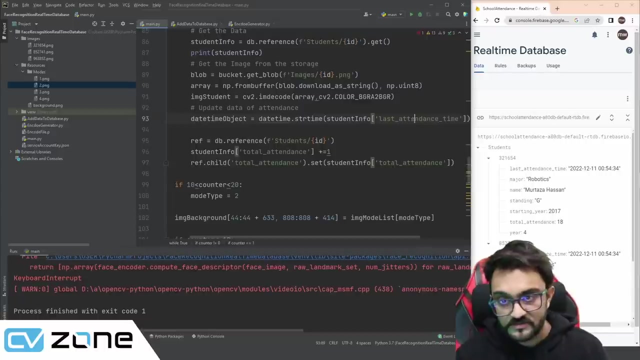 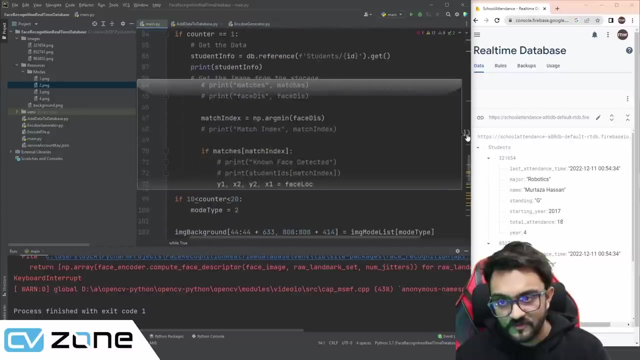 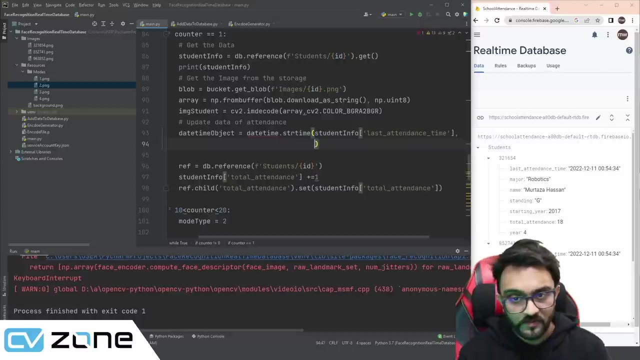 we have to convert it so string time. we have to give in the student info of the last underscore attendance underscore time, so the last attendance time, and then we have to give in the format. where did it go? then we have to give in the format. uh, the format we are using is basically- i will write it down. 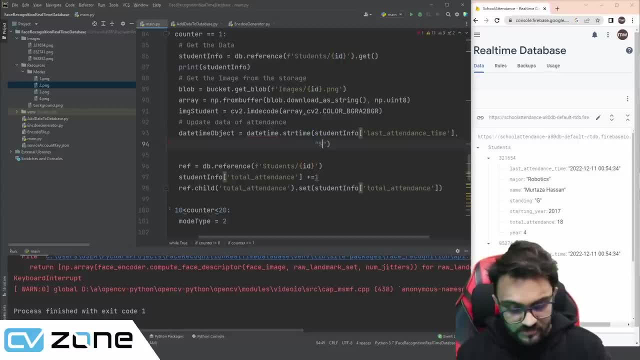 here it is percentage. first of all we have the year, then we have percentage month, then we have the percentage day, then we have a space, then we have hours, then we have colon, then we have minutes and then we have colon and then we have seconds. so this is the format basically. you can see it here. 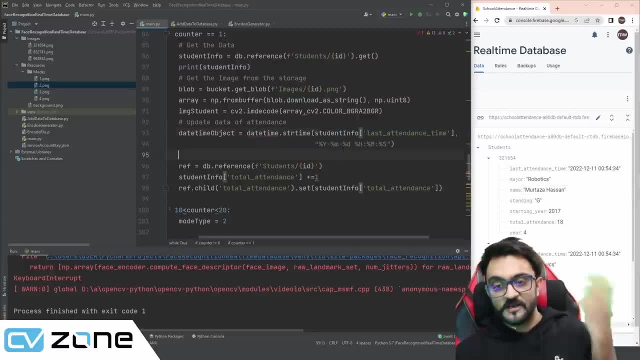 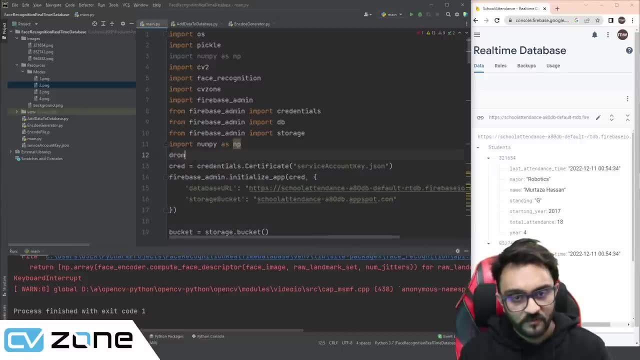 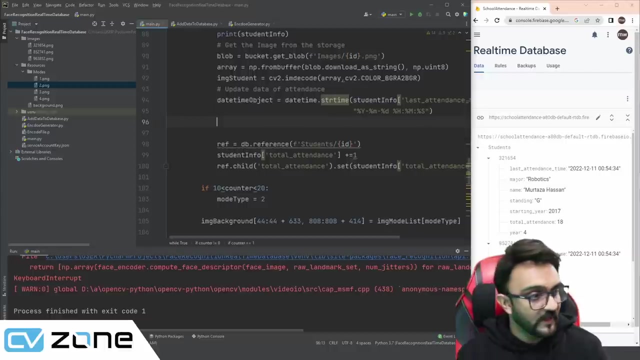 this is what we are writing it, that, uh, when you are creating the object, create it in this format: from the string, date time is not added because we did not import it from. from dates time imports date time. okay, so now it will have that. now it is converted and now we need to find the date time right now so we can write that date time. 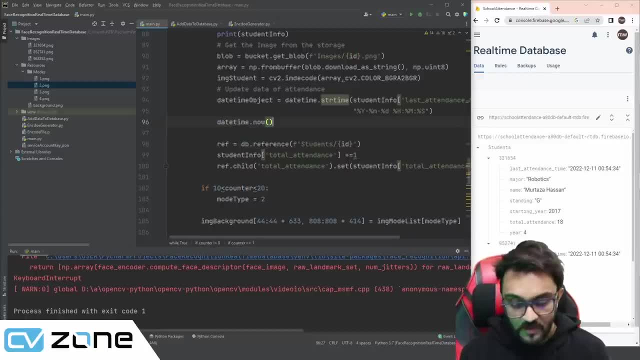 dot now it will give us that time minus date, time object. this will be the seconds. uh, elapsed equals this, but this will not be in seconds. it will be still in this format. so we need to convert it into seconds. so we will write dot the method. we will call it dot: total seconds, so it 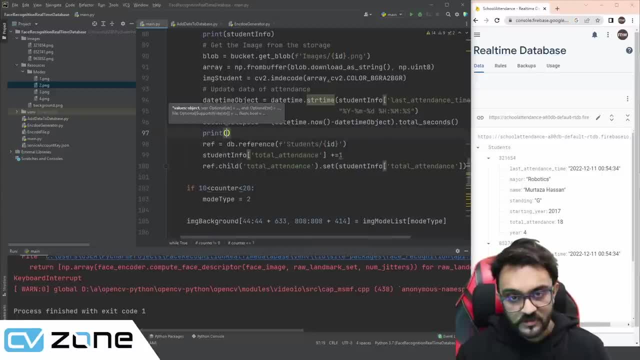 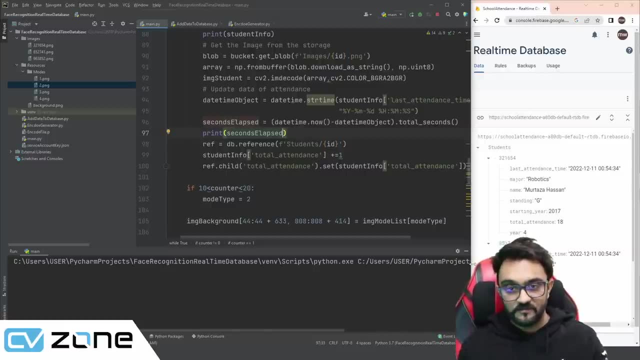 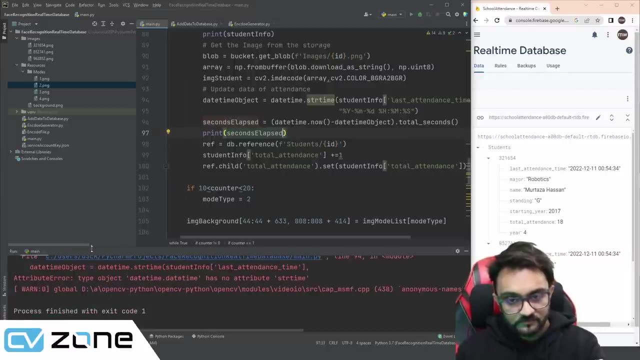 will give us the seconds elapsed. so if we print it out, we can print out the seconds elapsed. so if we run this now before updating, it will give us the time, the seconds that were from the previous one. so here we are, getting a warning. so this is the string time. 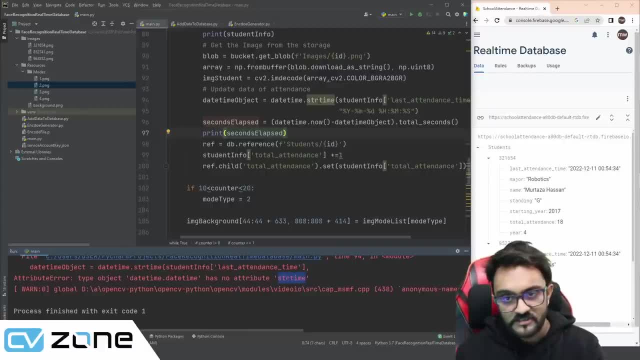 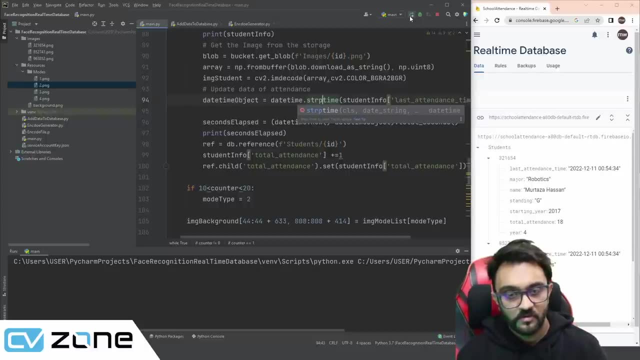 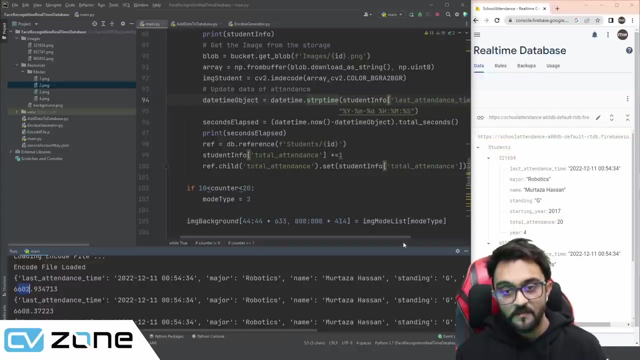 the string time is not there, so it's strp. my bad, so string p, so let's run that. there you go. so six, six, six, uh, sorry, six thousand, six hundred and two, then six thousand, uh, six hundred and eight, but now it's not updating the, uh, the the state, um, so it's not updating the. 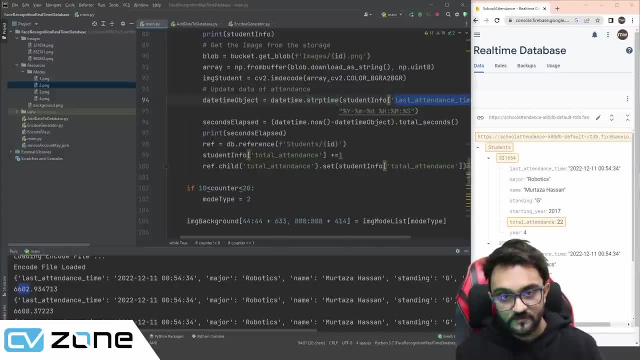 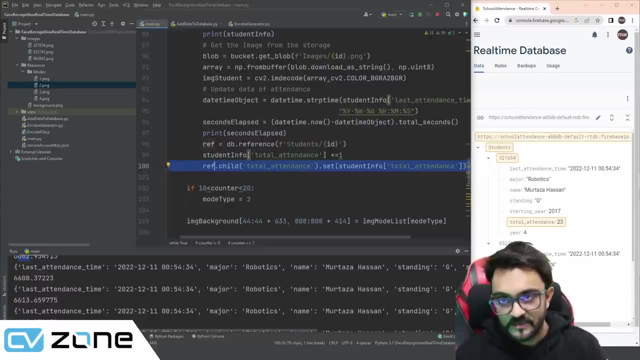 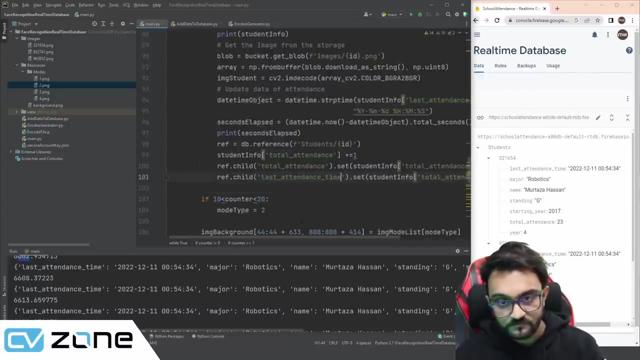 the last attendance time. so we need to update it right away so that next time it should not be six thousand second, next time it should be five seconds or six seconds, whatever time it's taking. so we will put it here reference style: uh, total attendance time and here the the time will be the date time right now. 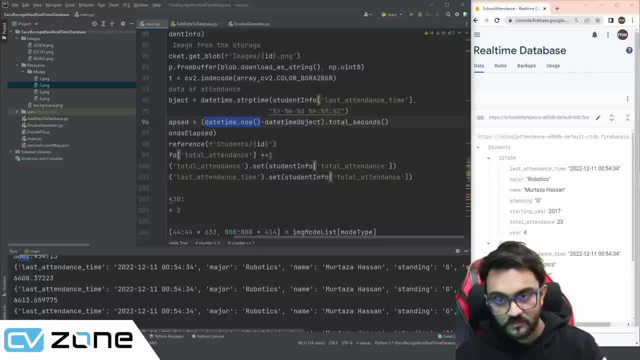 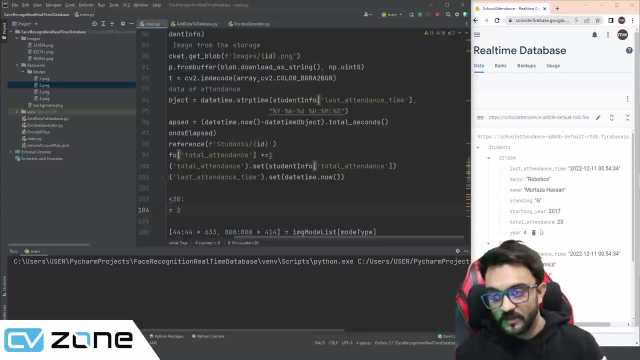 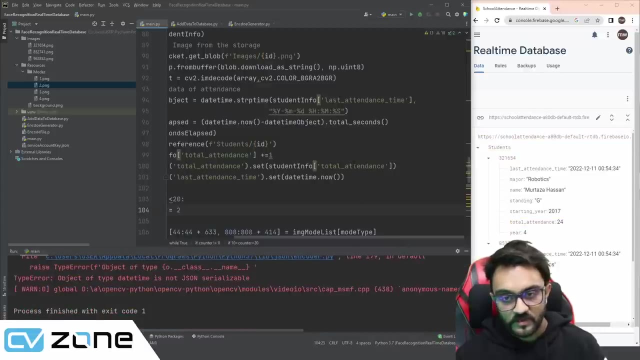 now the date time right now. there you go, so let's run that. so now it will update the last attendance time as well, so that will give us the correct. okay, there is a problem. date time dot now. uh, we need to convert it. okay, okay, okay, okay. so we need to convert it. 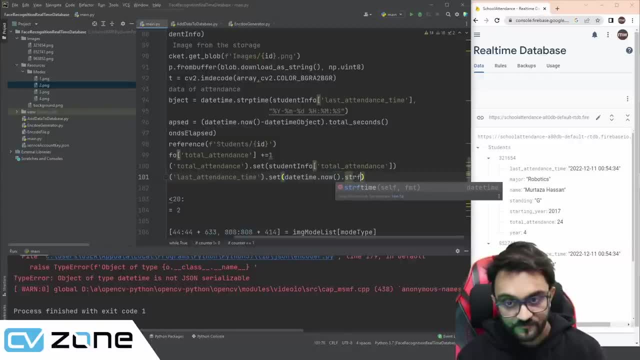 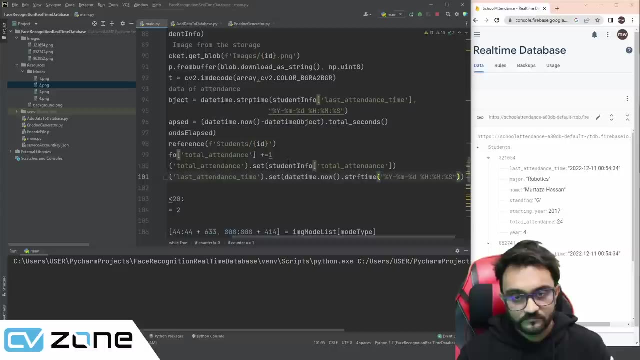 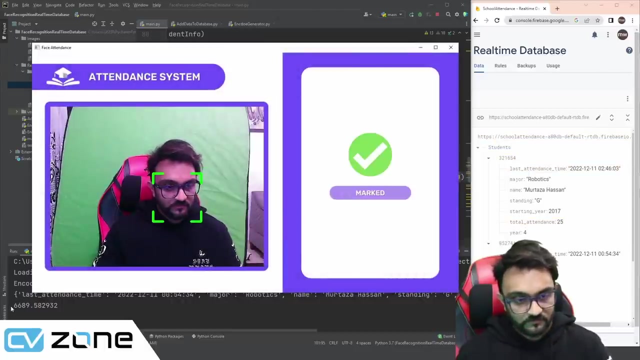 dot string, strf time and we need to give in the format. this is the format that we need to convert it into and then we can run it. let's run that. so here it should update. there you go, you can see it updated. so now, the time elapsed was six seconds rather than six thousand. 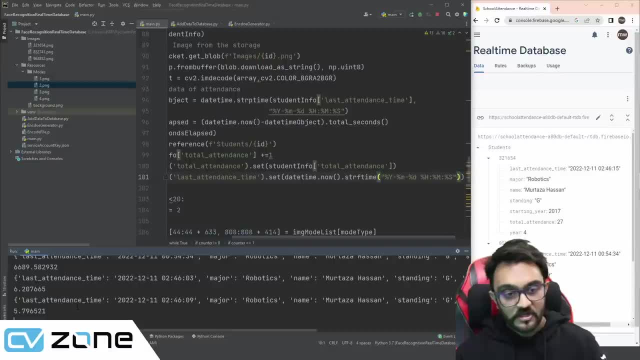 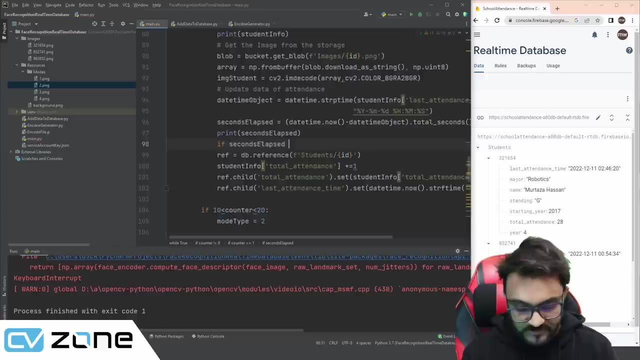 so next time it will be again five point seven. so now we can check how much time has elapsed, so that, uh, whether we should update the person or not. so here we can simply write. after second lapse we can write if seconds elapsed is greater than 30. so this will be 30 seconds. but if you want to do it in real, 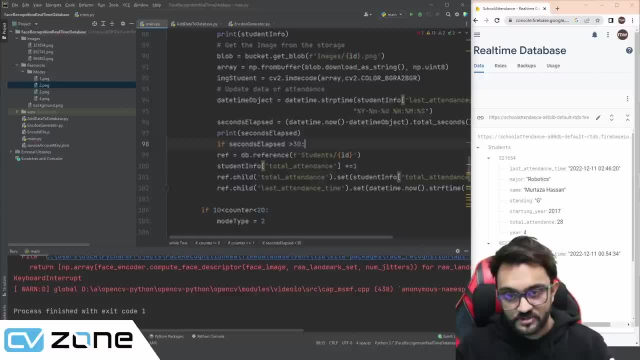 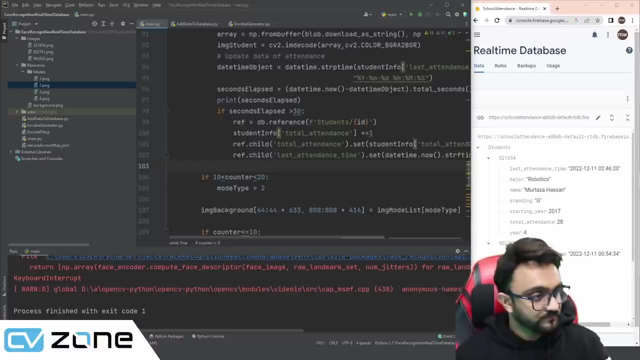 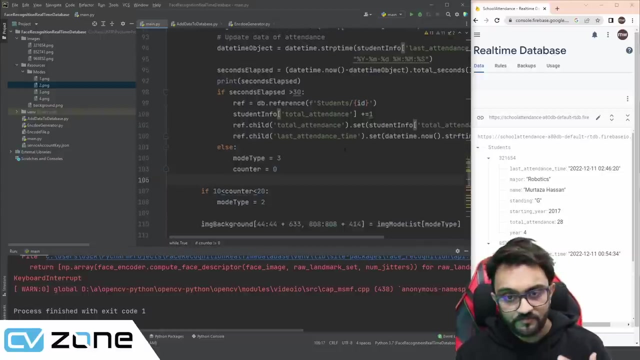 time you should do it. for how many hours or seconds? you have to convert it into seconds, as i mentioned earlier. so if that is the case, then we are going to update and add. otherwise we are going to uh give in the mode number three, so else else, mode type equals three, counter equals zero and uh, we will still um update our image. so 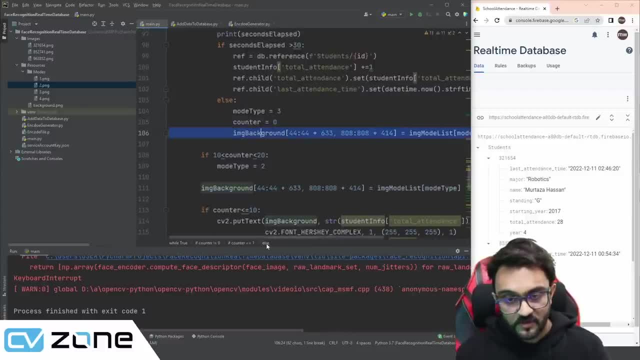 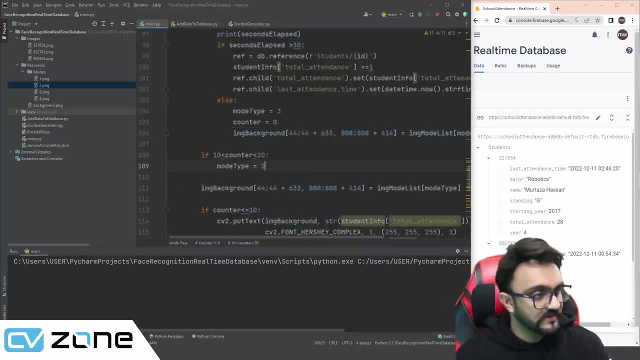 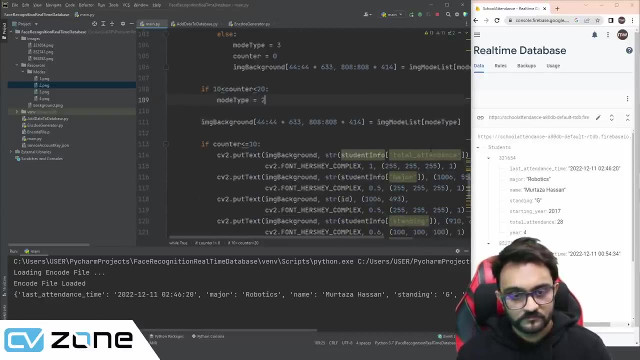 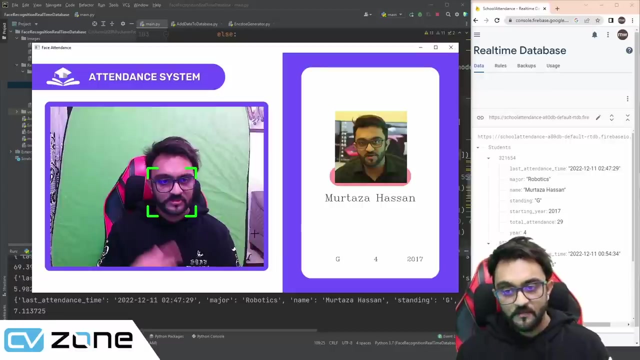 whenever we change the mode type, we need to add the image background, uh, this code, so that it updates in real time. so that is the case, and then if we run it, let's see what happens. so there you go. so it is marked. now it's showing active, but now it's showing the. 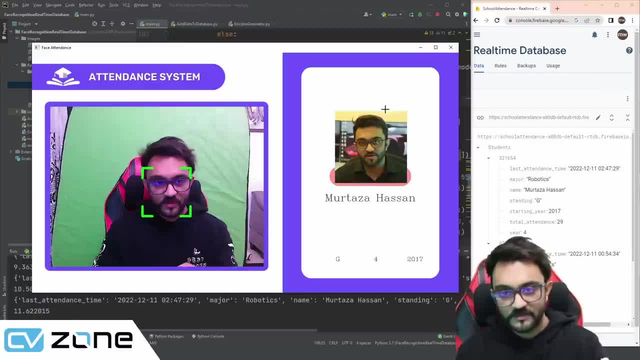 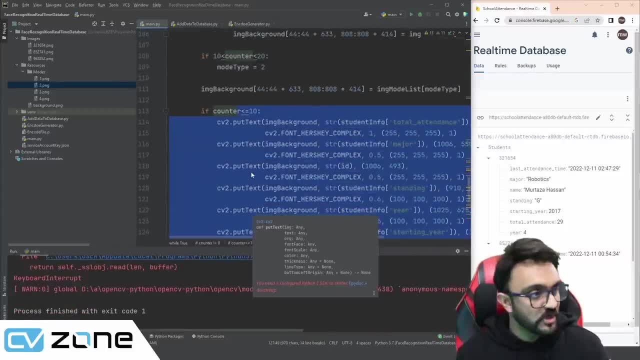 image and all of that it's showing, already marked, but now it's showing the image, the text and all that. we need to stop that. so here, this is the part where it's showing all of this. so all we have to do is- uh, we have to write here. 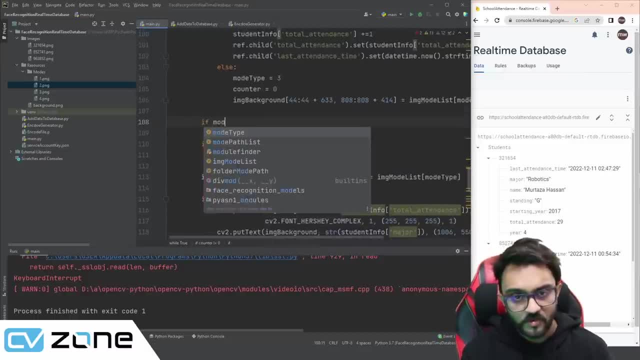 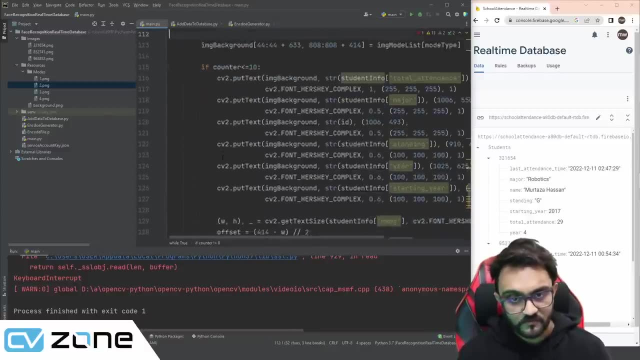 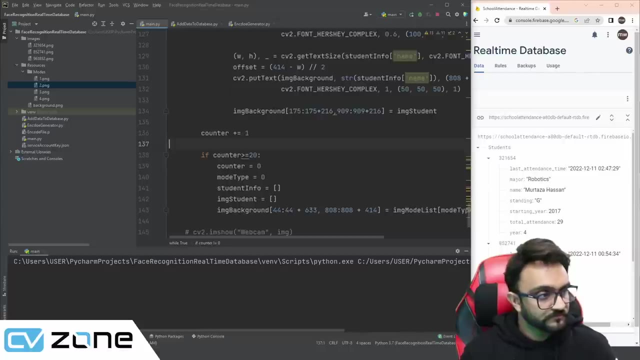 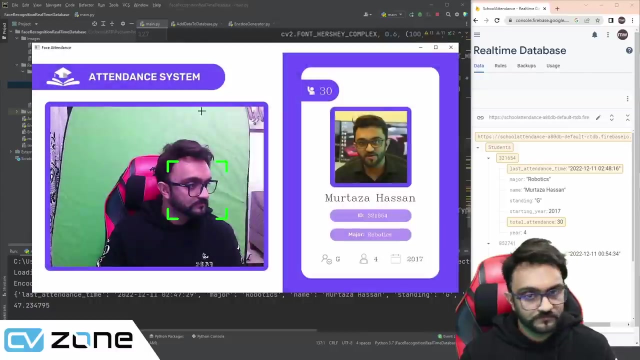 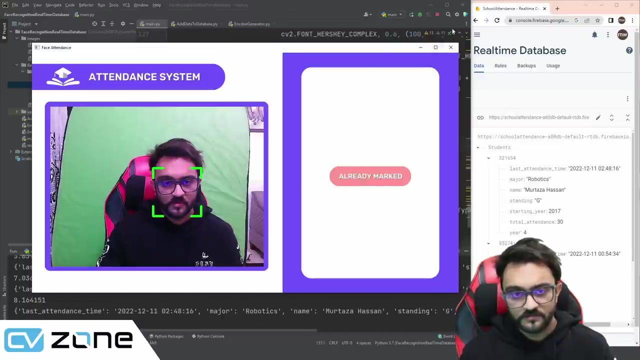 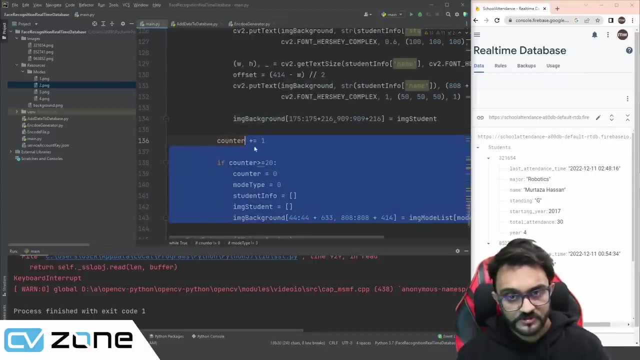 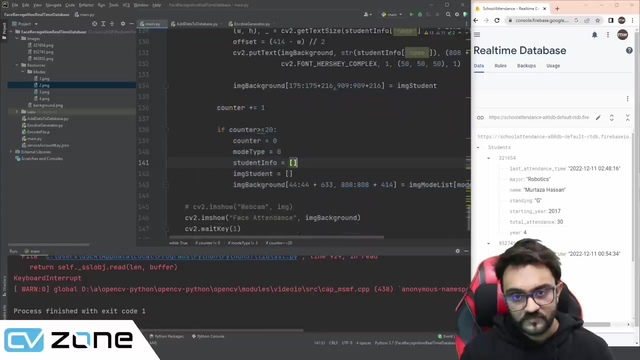 that if the mode type is not equals three, then you can do all of this. otherwise don't do it all of this. so there you go. now it says already marked and then you have to push this in counter plus one. it checks it here. yeah, so when the counter is above 20 it will go back to active. so you just had to push it in it. 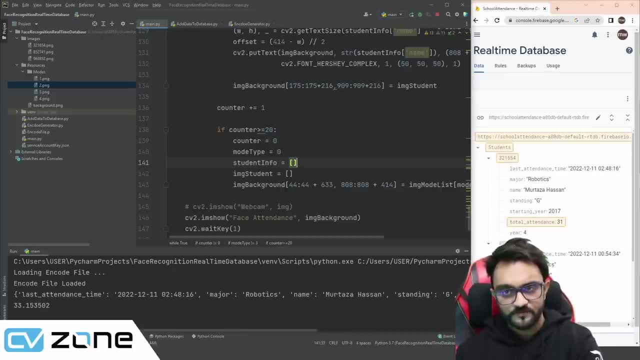 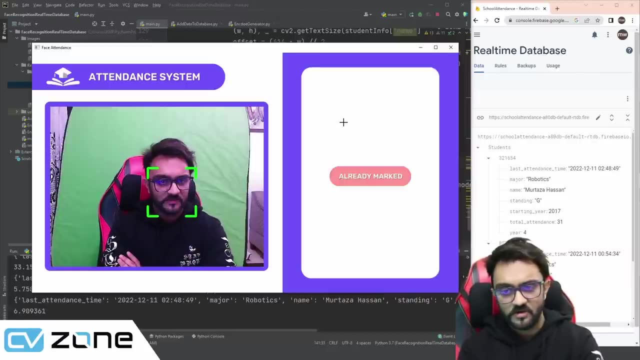 was in the wrong loop. so let's run that and, as you can see, the time and the attendance is automatically updated. so it says already marked, but, uh, before it says already mark, it shows active. and then, after already marked, uh, if i remove my face it should say active again, but it's. 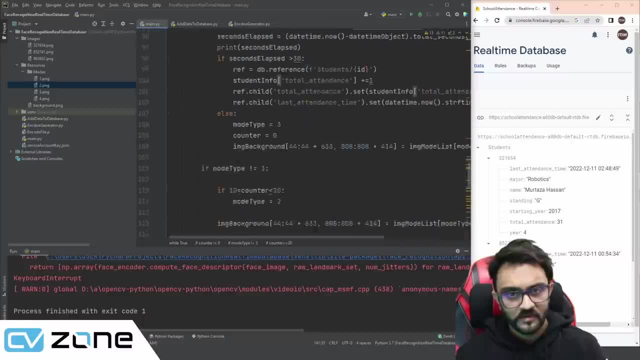 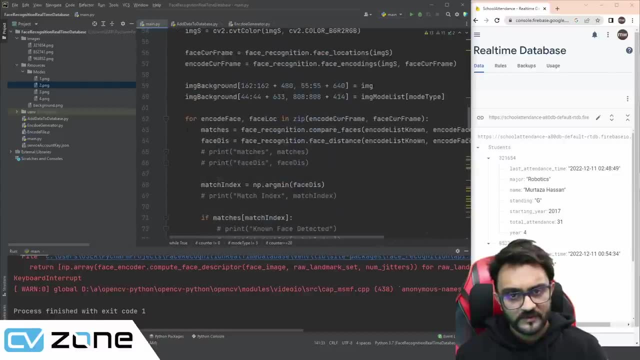 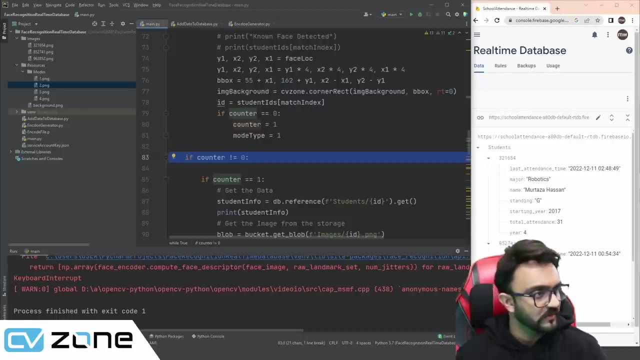 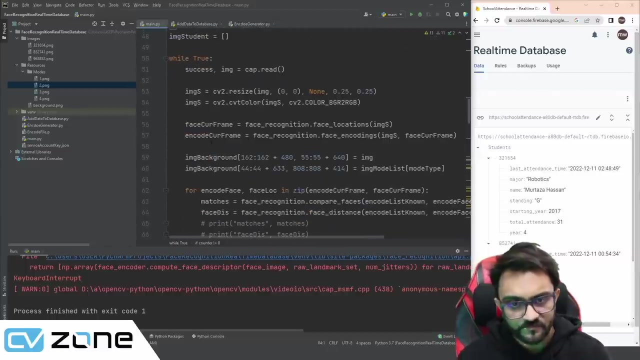 not doing that, so we need to fix that. so, if mode type is three, so in this case, if nothing is detected, uh, no, not in that case if counter is not equal zero. if that is the case, let me just recheck it again. okay, yeah, so we need to add another if condition, that if the face is detected. so here we will write. 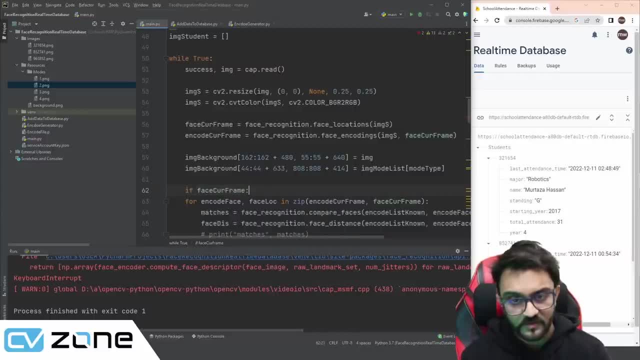 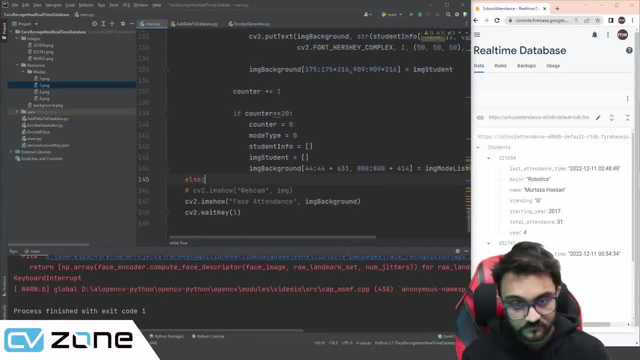 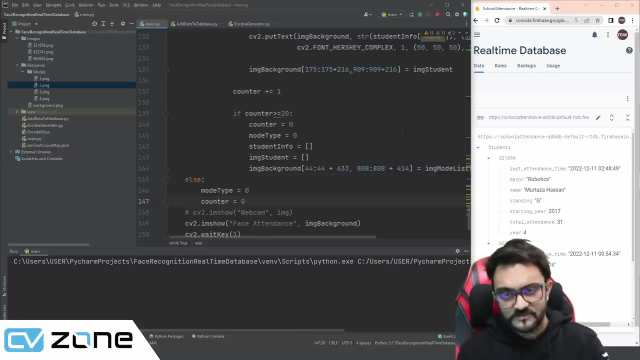 if there is anything in the face current frame, then do all of this, all of this else mode type equals zero and then counter equals zero. so if we play that again, then we should. when i put my face in, it should remove the already detected or already marked. 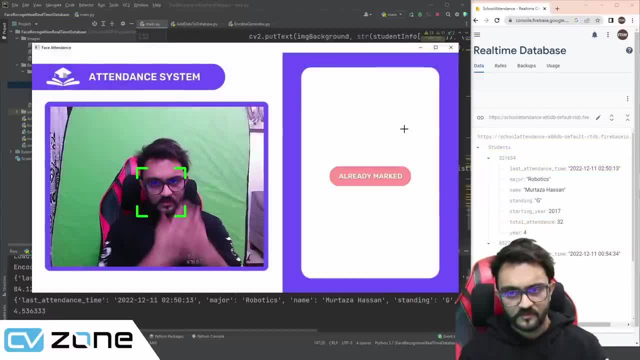 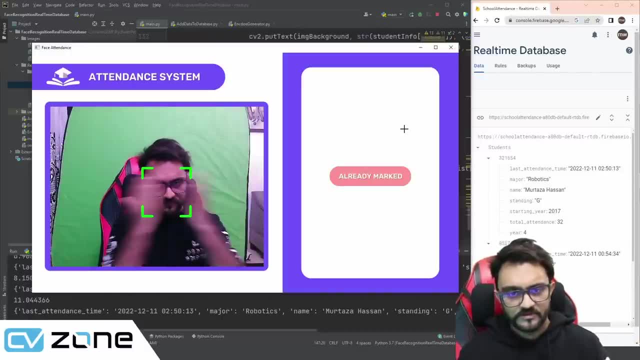 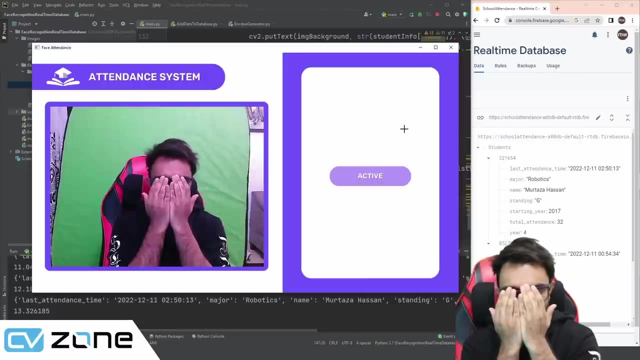 so if i put my hand in, it shows active, then already marked. and if i put my face here, it shows active. if i remove, it says already marked. so i need to wait 30 seconds. so i'm going to block my face and hope for 30 seconds. then, once the 30 seconds are up, uh, it should say: 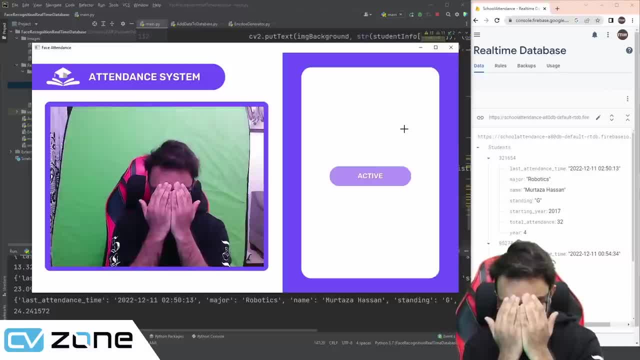 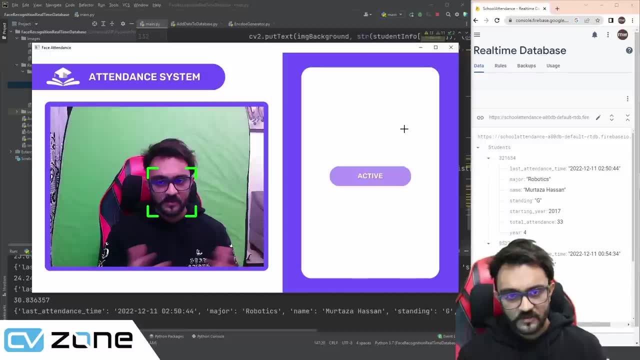 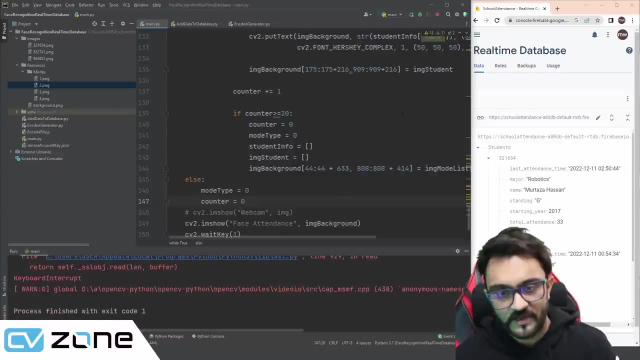 uh, marked. so let's wait, wait, wait, wait, wait, wait and let's try it. there you go, go. now it marked again, and now it's marked active and now it will say already marked. so after 30 seconds we were able to mark it again. now one more thing we can add, which is a little bit um: 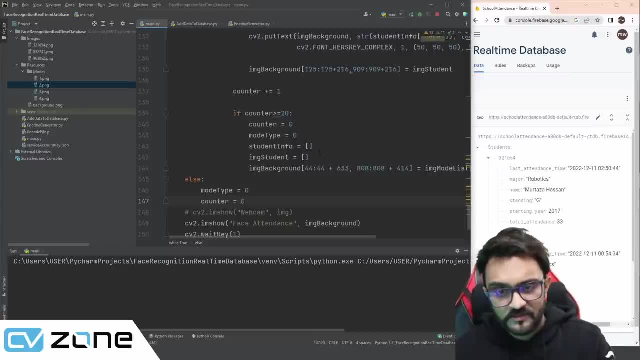 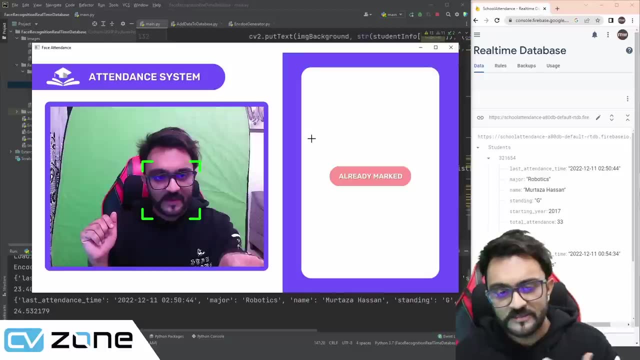 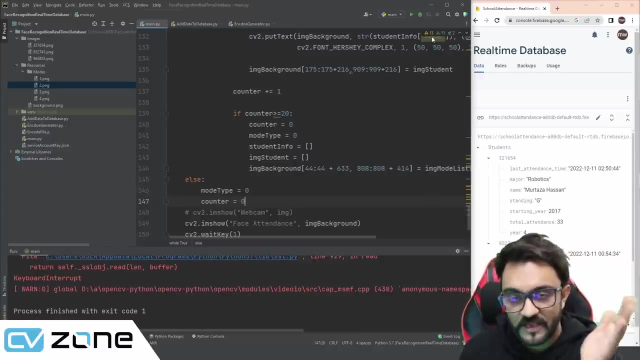 for for the aesthetics of it. once the object is detected, once the face is detected, you will see here. it delays, it lags. so this is because it is downloading the data from the database. if you want to remove this lag, you have to use asynchronous functions, so we are not going to go into that. 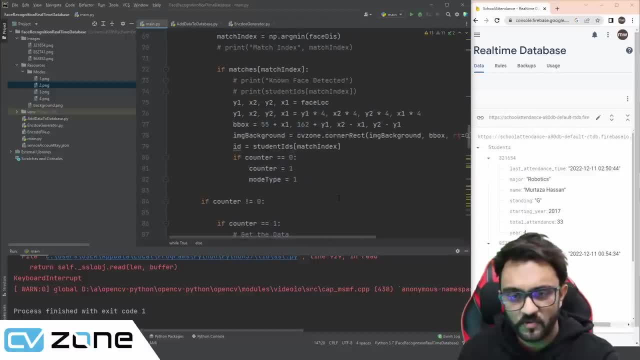 much detail. we have covered this in our web development course, in which we will create all of this in our website and once we have done that, we are using asynchronous functions, so it will show the video in real time and it will update and download the code. download the database. 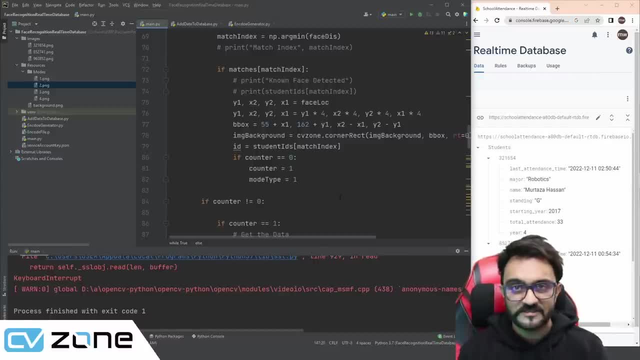 at the back end, so it will not delay as much, it will not get stuck. so in order to avoid this as a problem, in order to make it better, what we can do is we can just write loading once it is detected, so that way it will not look that bad, it will not look like it's stuck. 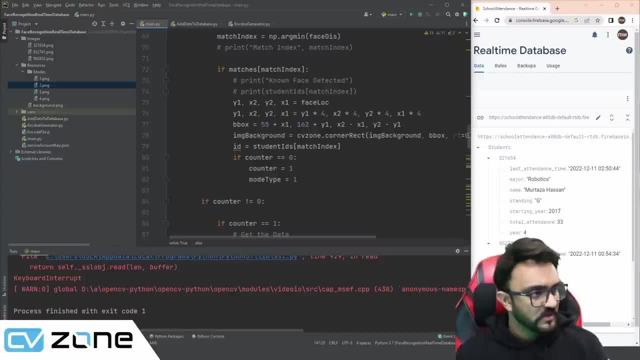 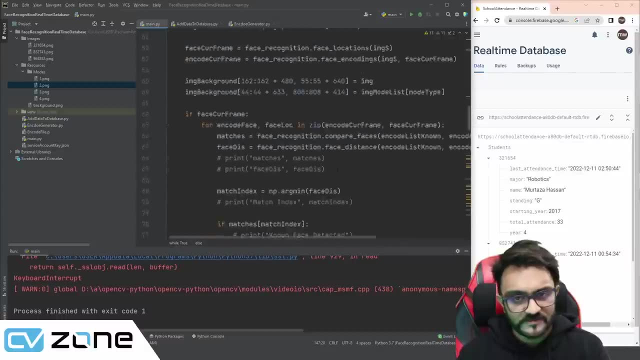 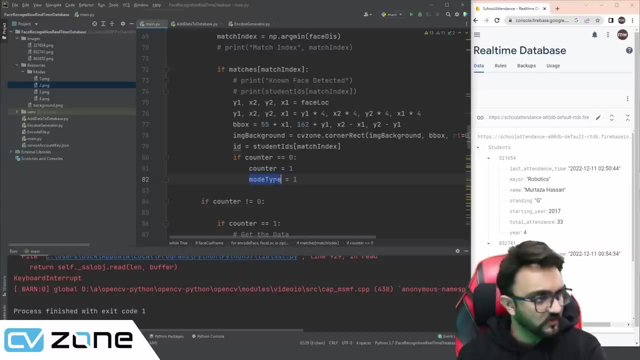 it will just think that it's encoded, it's loading. so in order to do that, let me check where do we add that? yeah, if the known face is detected, if the known face is detected which is over here as one, and in this, when the counter is zero, what we will do is we will write here: cv zone. cv zone. 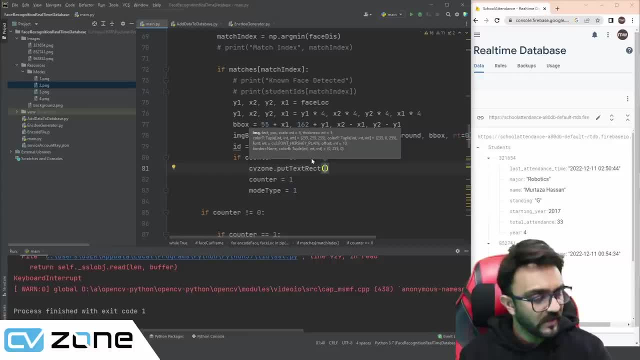 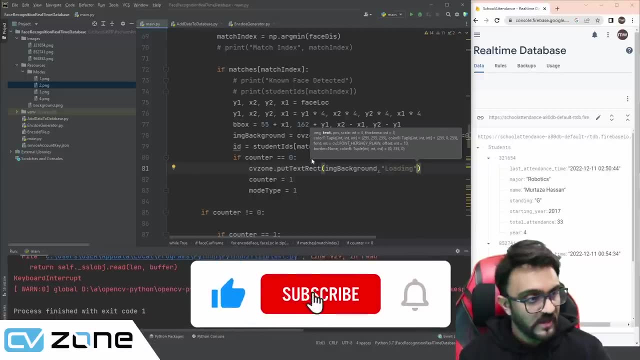 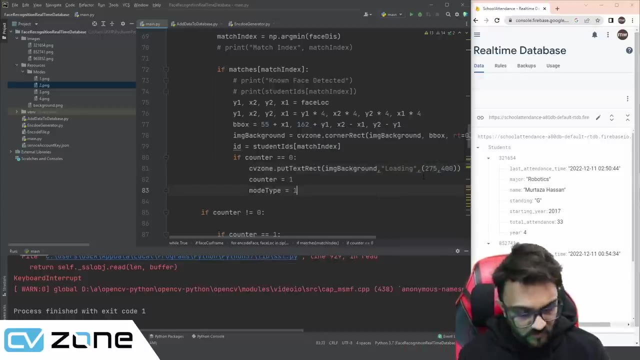 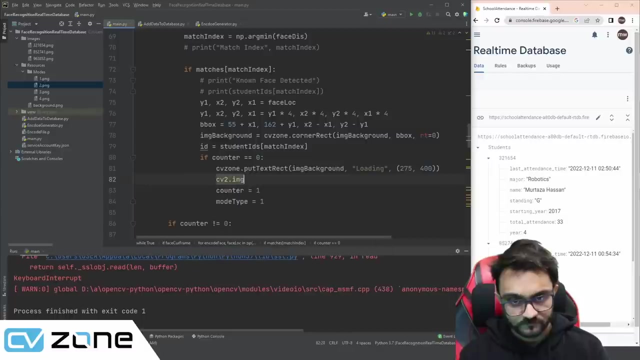 dot, put text rect and then we will put it on the image background and we will put loading l-o-a-d-i-n-g and we will put it at the position 275 and 400 and then we will update the image. we will not show it as it is, so we will write cv2 dot. i am show. you have to write the exact name. 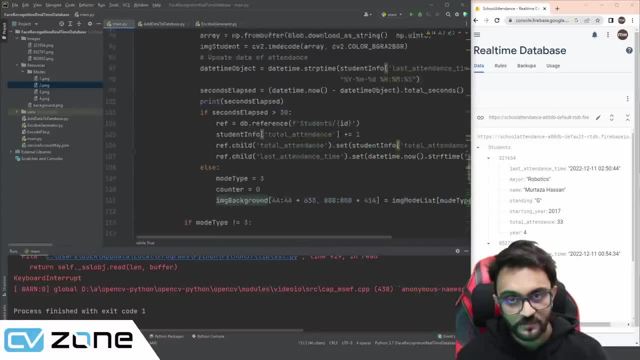 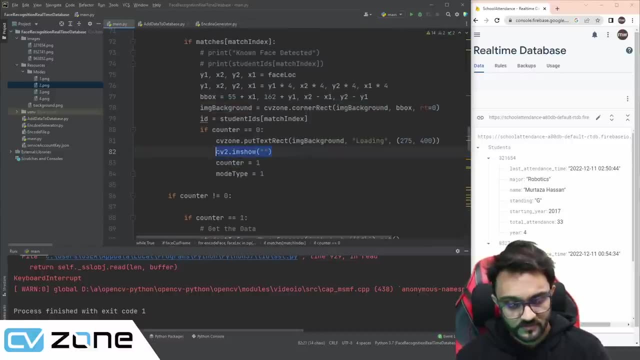 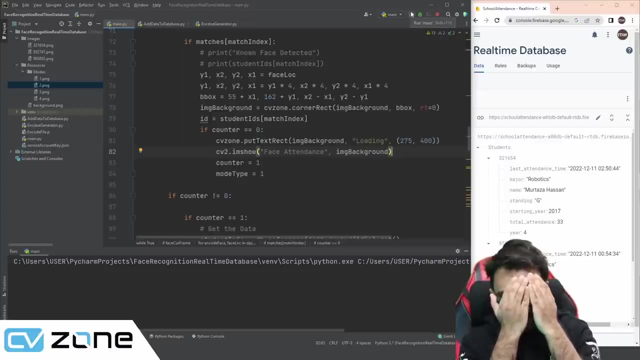 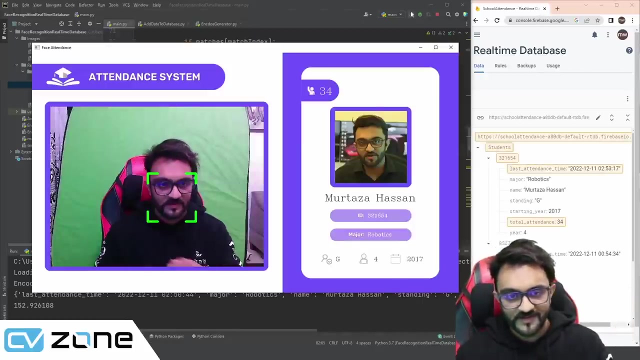 so we used face attendance so we just we can just copy this and we can paste it here. copy this part and paste it, there you go. so now, once it detects, it will say loading. so i will cover my face. uh, now it's running. running if i remove. no, it's not saying loading. that's not good. why is it not saying loading? 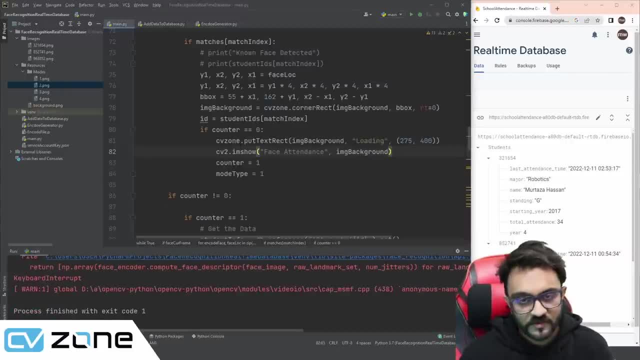 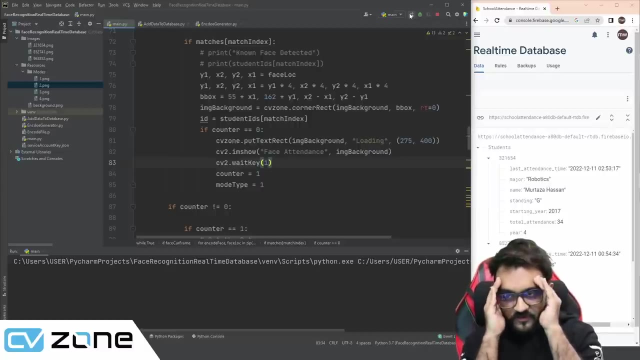 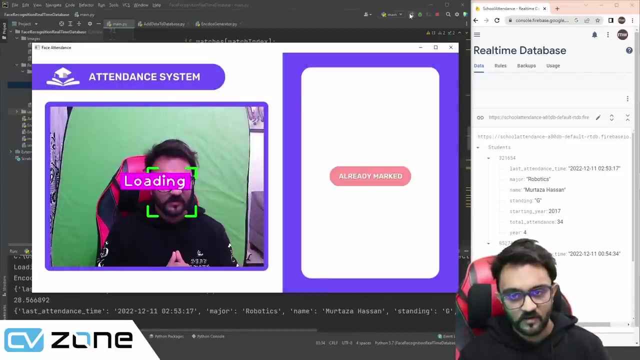 uh, counter is zero. oh yeah, we need to add the weight key, cb2.weight key. we need to add a delay of one millisecond and then it will update. so let's hide my face again. okay, if i put that, it says loading and then already marked, because i just did it. that's why. 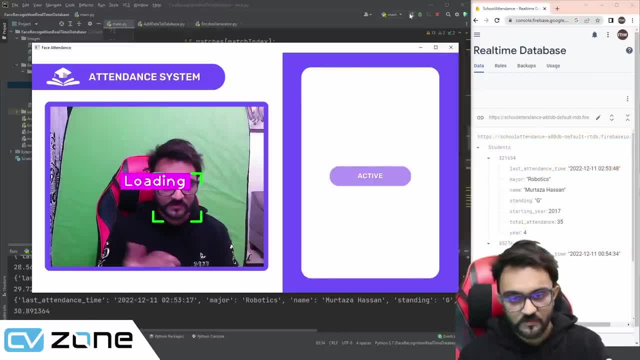 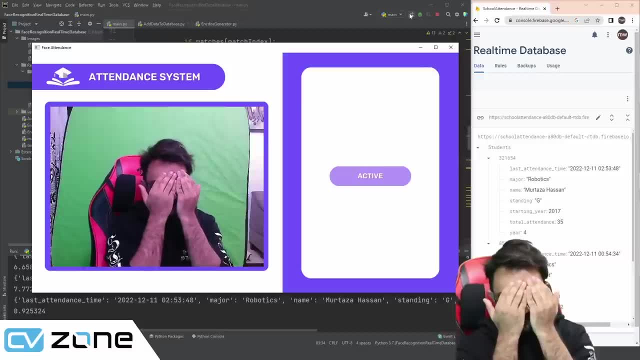 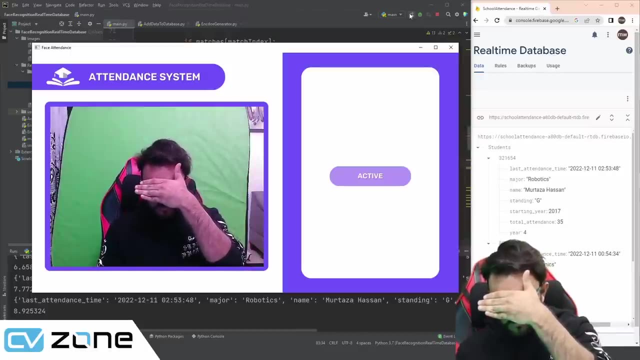 there you go. so now 30 seconds were up, so now i can mark again. now it says loading and already marked. so if i hide it, the loading is gone and now it's active, and then we can mark others as well. so if i wanted to mark, i can mark. for example, let's say, i want to mark elon musk.